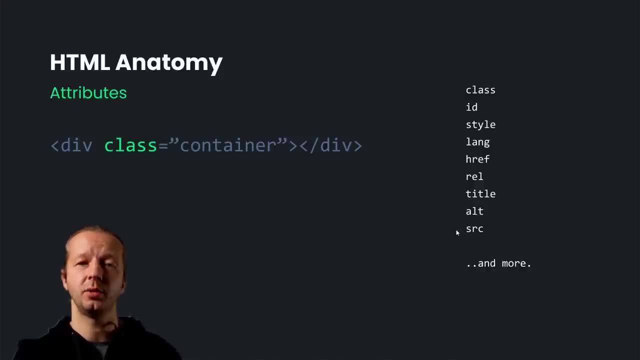 here are other attributes that you have that you can add to your html element or html tag. and then, finally, we also have i the concept of self-closing elements, and, for instance, this right here is not a self-closing element, it has an opening tag and 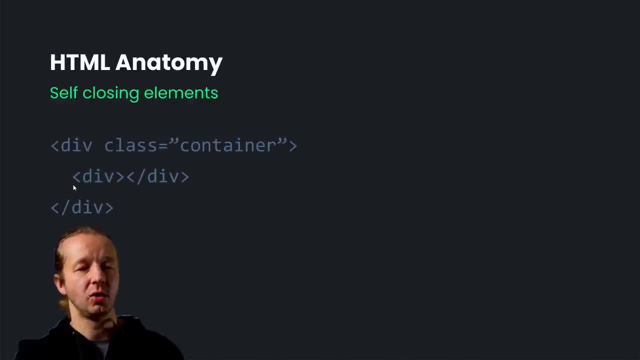 a closing tag and, of course, with these types of elements, you can nest them inside each other and you can have nest upon nest upon nest, etc. etc. this here is a self-closing element, all right. so image source whatever, we don't see a closing tag and there are a variety of different html. 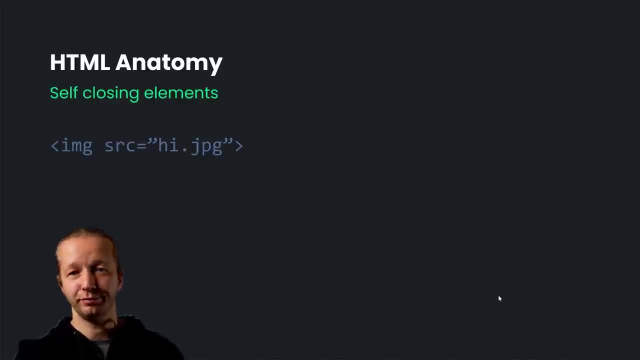 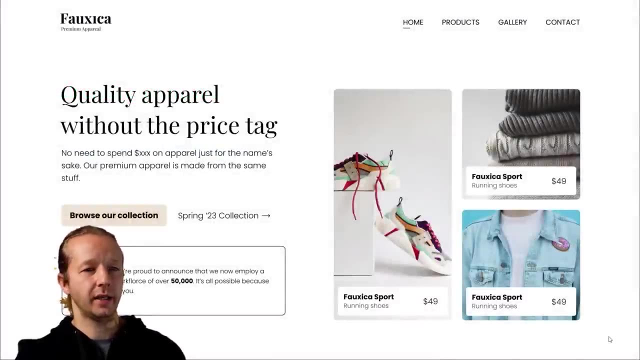 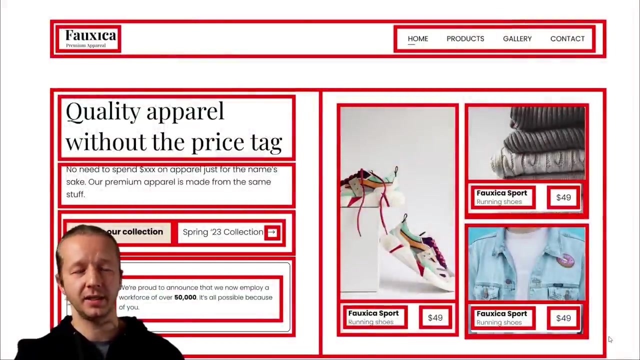 elements that are self-closing and otherwise all right. so you may be asking yourself: what is the purpose of html then? well, looking at the design that we're going to build here in a second to provide you with a visualization of kind of what html is doing, this is what html is basically doing, at least in the respect of 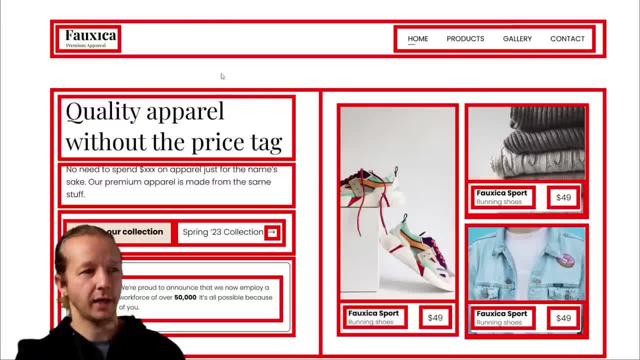 helping you structure a layout. i, all of these red rectangles have to be accounted for in html code in some way, shape or form, and we're going to talk about this i ad nauseum, throughout i writing the html for this particular layout. so this is what we get in the browser. this is what everybody. 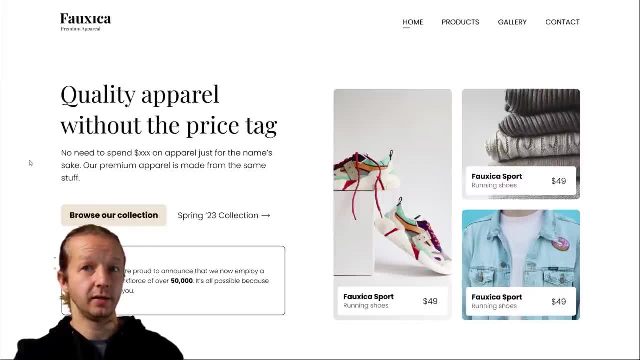 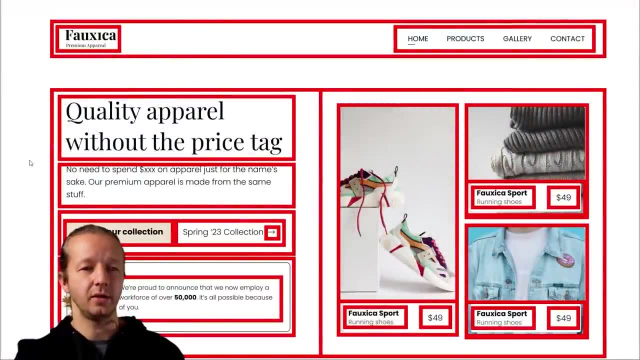 sees, but in order to kind of provide a literal, visual visualization of the responsibility of html. this is kind of what's happening here, and you can think of it in an analogy such as: html is your skeleton and then css is the aesthetics, it's your skin, it's what everybody sees, all right. so 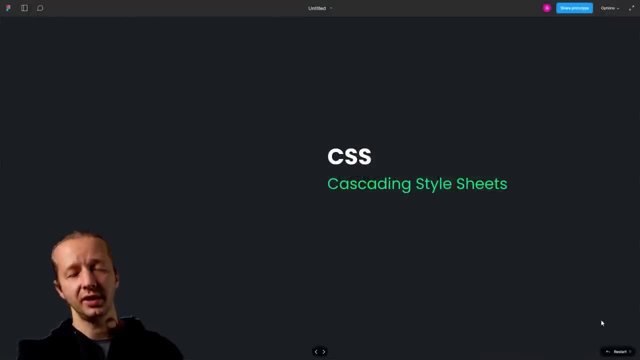 now, with that said, let's talk about actual css. okay, so that stands for cascading style sheets. if you walk into work for the first time and you tell people, let's write some cascading style sheets, they're going to make fun of you, all right. so let's take a look at. 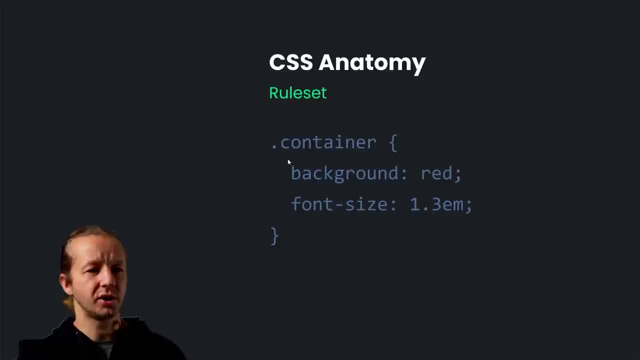 css anatomy, and what we have here is a rule set. typical projects have multiple rule sets. they have many, many, many, many, up to hundreds or even thousands of rule sets. this is one rule set, right here, this whole thing, right there, all right. so, first off, we have what's called the selector, all. 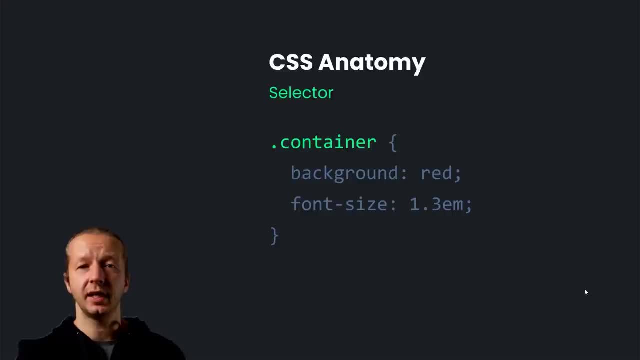 right. so this is a rule set, and this allows you to basically say to css: what html element or elements do we want to style? simple enough. next up, we have the declaration, and that's defined by all the stuff that happens within these squirrely braces right here. then we have properties, as you can see in. 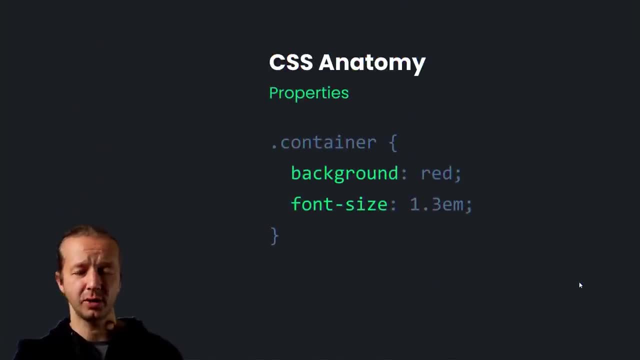 this context, this particular rule set has a declaration of two properties. by the way, people don't know about declarations and stuff like that. this is just, uh, you know terminology that most people don't use, but we do have properties here. there's two properties: background and font size. 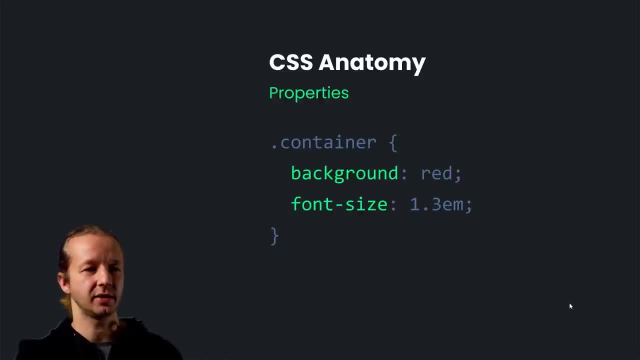 and, trust me, there's a ton of properties that you can use in css. next up are the values. so we have the property name with a colon with the value, and then we end that property, or that that particular declaration, with a semicolon: all right. and then finally we also have 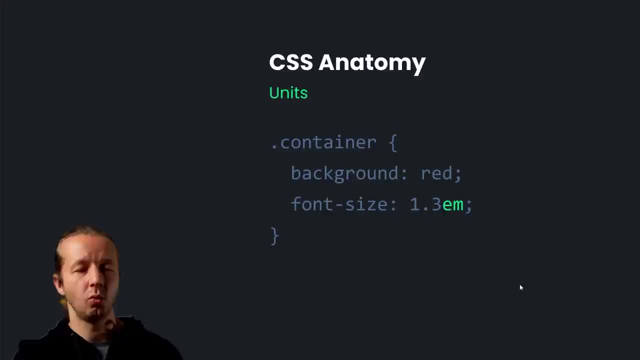 units. sometimes some properties will have units fixed to them and of course there's, you know, probably a dozen or so different css units i that are categorized into absolute and relative positioning, and we'll talk about that as well. all right, so that is it. i told you it wasn't going to. 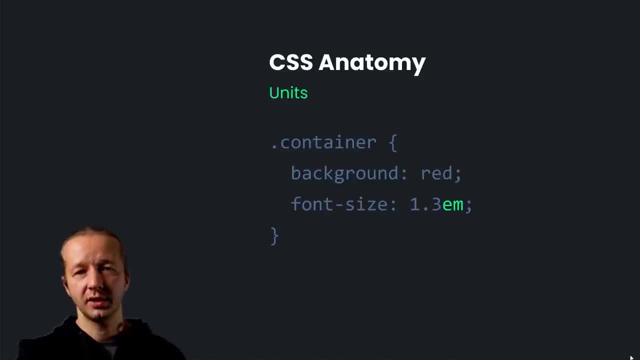 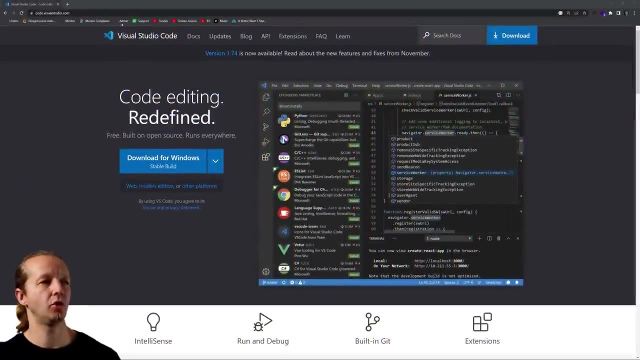 be that long for just outlining general concepts now, because this is a crash course. we are going to jump right in, all right. so i want to show you a couple of things that i want to talk about here once you go here to code dot visual studio, code dot com. all right, and this is the web page from. 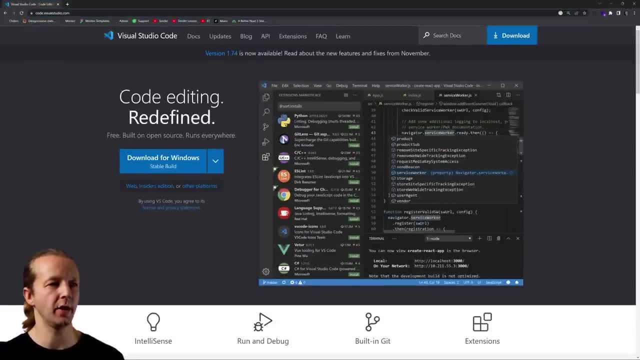 which you can download a code editor in order to write the html and css to complete this project today. this is a free code editor from microsoft, and it's also the most popular, and has been for several years now at least, and so, depending on your os, uh, you're gonna, you know, download the, the software package, install it and then run it. 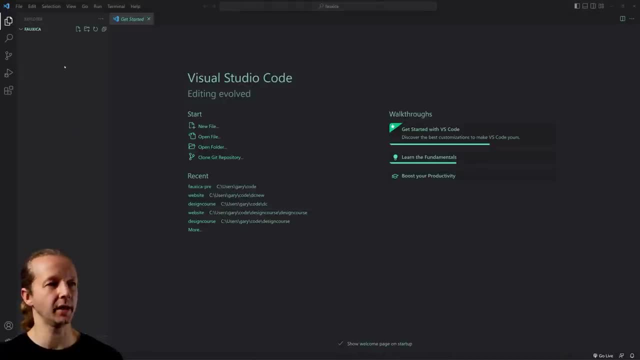 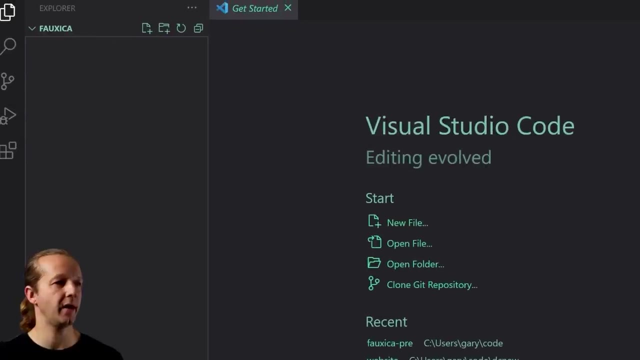 and then, once you run it, you'll see something like this: now your, your color scheme might be different. no big deal, but over here we can see that we have this thing called foxica, which is the name of the fictional, you know service that we're designing a landing page for. 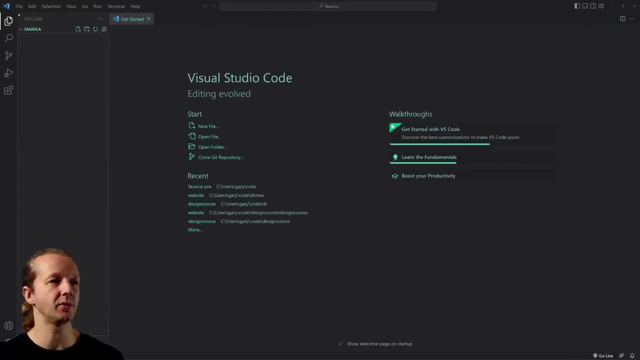 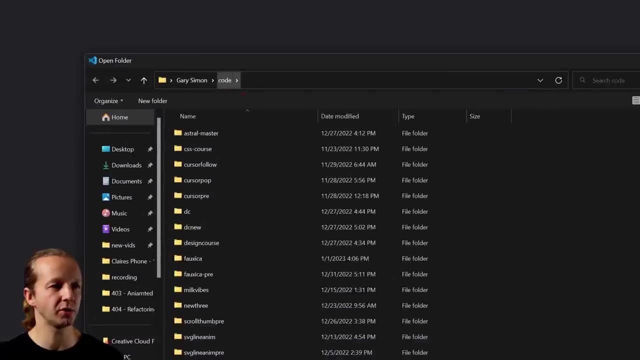 so that is basically an empty folder that i've already opened up. so if you go like to file open folder, i right here. i'm in gary simon code folder, so i've created a code folder where i store all my uh projects in and you'll see foxica right here. so, um, you know you can right. 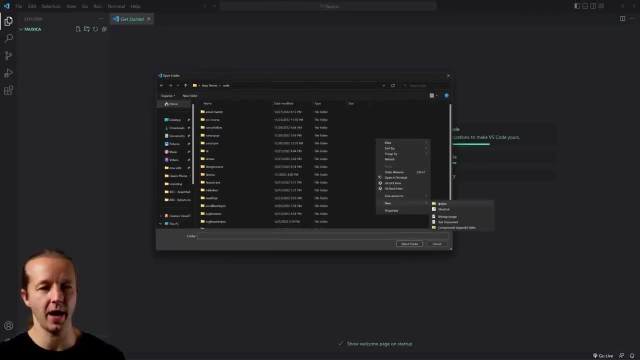 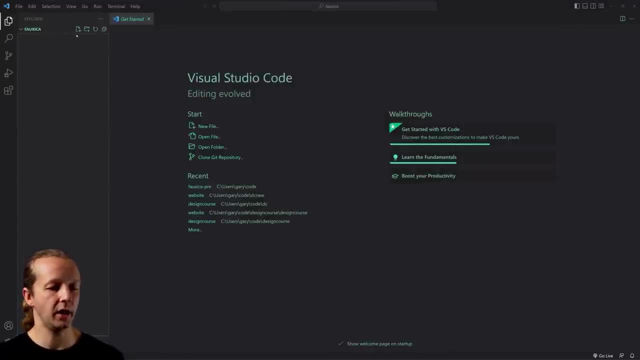 click new folder. this situation might be different for mac, but just you. you have to open up an empty folder, essentially to get where i'm at right now. um, and so now we're going to go ahead, and we're going to go right up here and we're going to click this button, which will create a new file. 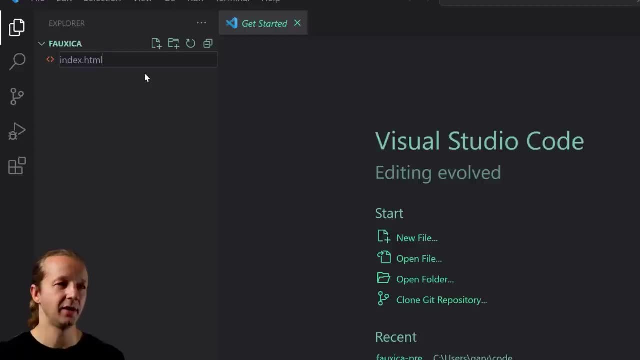 and then we have to give it a name: indexhtml. all right, so indexhtml. very typical starting point. whenever you go to like whatevercom, it's probably loading in the actual indexhtml. of course, if they're using frameworks it could be different, but for us, uh, where we're not using any type of javascript framework or platform, we're we're just. 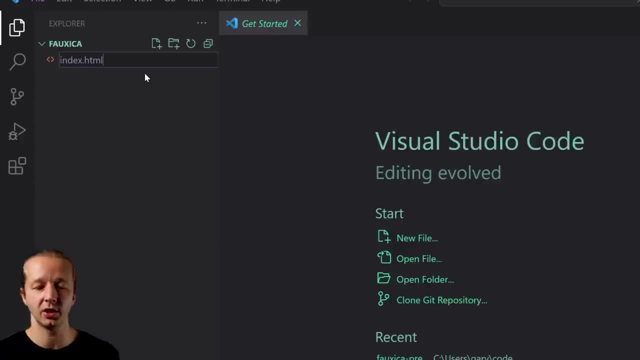 going to name this indexhtml, which is going to be the actual home page or the starting page. when somebody goes to a fictional site like foxicacom or something like that, hit enter and you can see now that it's opened up here in this code editor where we can start writing. 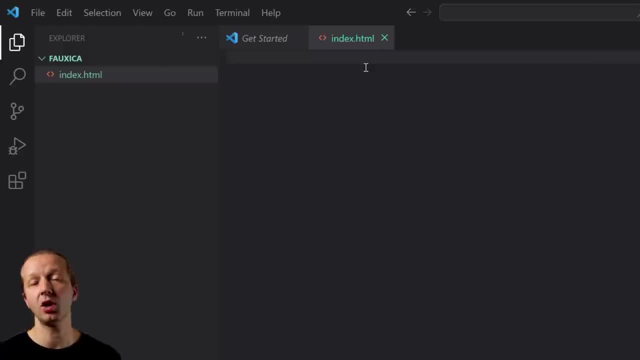 our html. um, there's something called emmet, e-m-m-e-t, emmet abbreviations. now i've done a whole course on this. it's really simple. there's basically a few shortcuts that you can use that can speed up the process of writing html, and the very first one that i use every single time. 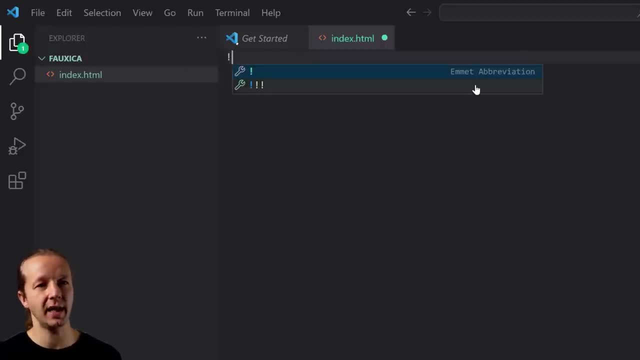 is exclamation point. hit that and now you can see it says em abbreviation right here and then hit enter and it gives us a bunch of our starting html elements. so it gives us the very opening html and closing html tag. it gives us the head element with the various meta tags in here. this stuff right here, you really pretty much for the. 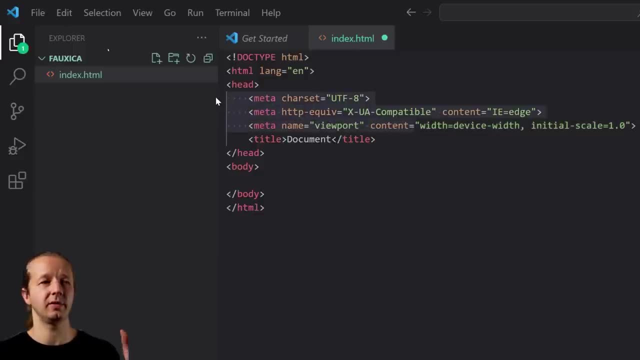 most part, you don't touch. you don't touch these, just ignore them. if it looks scary, don't worry about you, don't have to touch them. uh, the title is important because that's kind of the title of the page that shows up on the browser title and also shows up like with people search for. 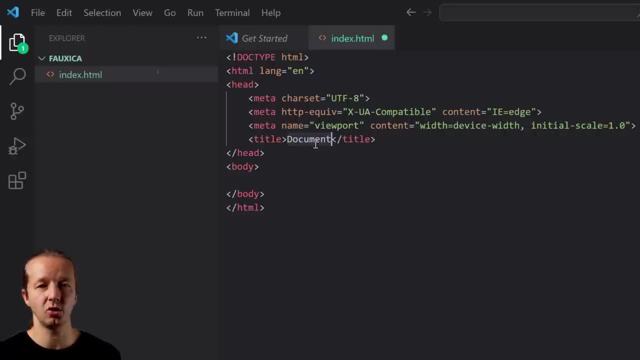 the company name or us, a keyword, and if you you rank in google, you'll see the little blue link or whatever that's. that's where it gets this from as well, so we'll just call this foxica, just like that, all right, and we'll hit save. and, of course, then we have our body element, and this is where 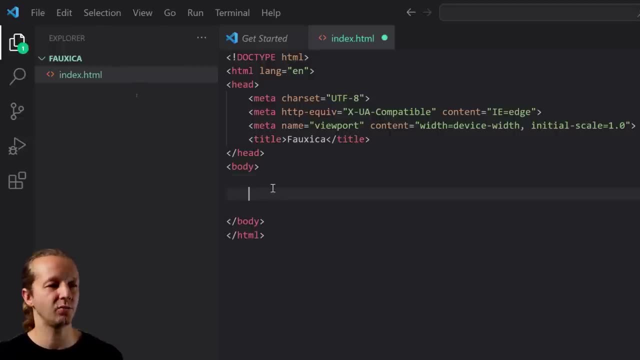 all of our html is written right smack here in the middle. so 99.99 of the time you're writing within these body, uh, the the closing and um the opening, rather in the closing body tag. so with that saved, um, we're going to also outside or just underneath the title. 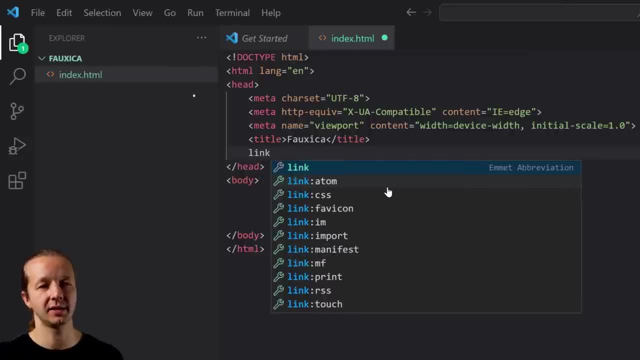 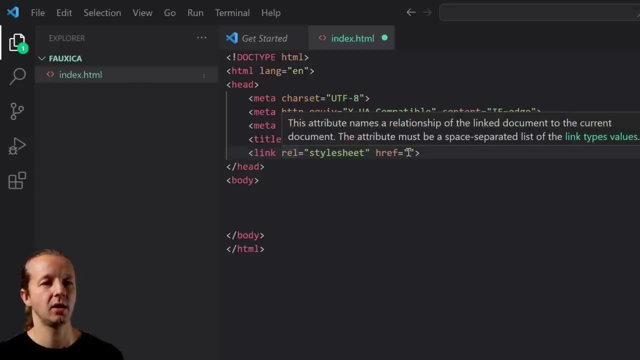 tag. here we're going to type link, and again this is an em abbreviation- enter so that opens up the link element rel stylesheet href attribute in this, href basically means gives us a place to go. what we're doing now is we're going to reference a css style. all right, so we're just getting that. 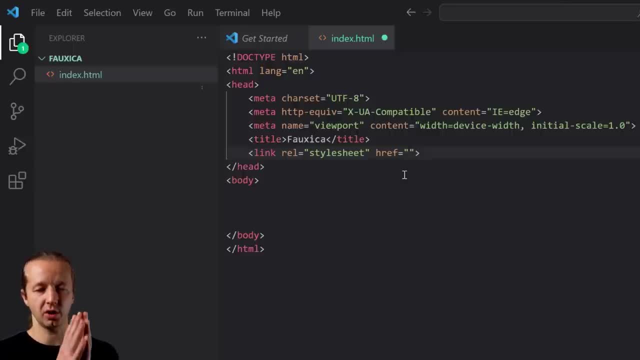 out of the way. initially, there it is because it's part of the HTML process. First we're covering HTML, then CSS. But I wanna link that up And typically I put it in a folder called CSS- forward slash- maincss. All right, so we'll save that. 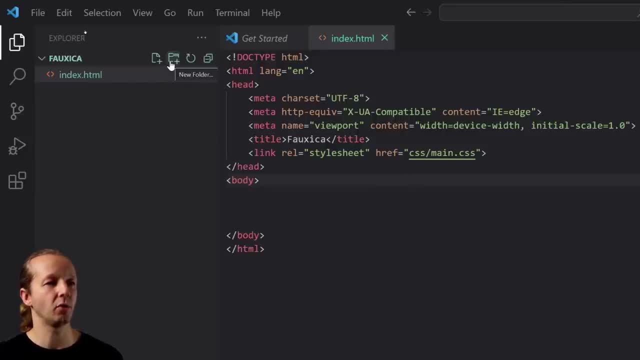 Control S on your keyboard And then we're gonna go ahead and create that folder. So we're gonna click this, which creates the folder CSS, And then we're gonna click this, the file maincss. And there you go. you can notice it opens up a new tab. 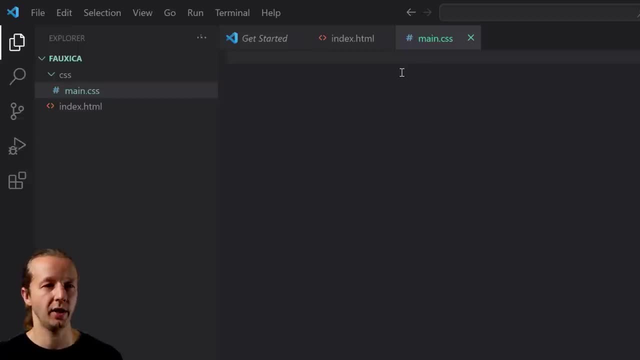 with maincss. when we save that or hit enter And we're ready to write our CSS in here and it will get communicated automatically. Note- and this is something I never do, but just understand- you could do that If you didn't want to have to link another file. 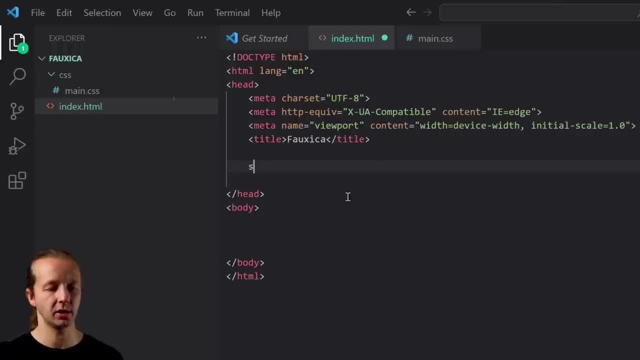 to access your CSS, you could just put in style tags, So style enter, that's an M abbreviation, And then we can start writing our CSS in here as well, in this section, That's to call it. that's inline CSS. 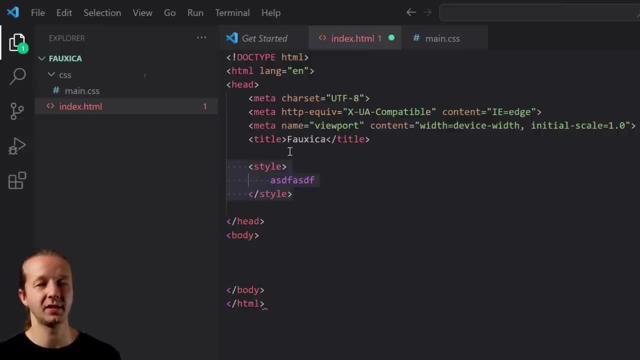 There's nothing wrong with doing it that way, But if it's a serious project, this index to HTML file will become real lengthy in the number of lines of code that has, And that's just annoying. I like to separate my files out. 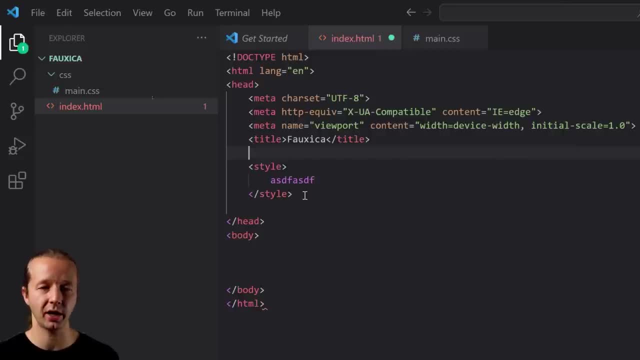 Same thing with JavaScript. We're not getting into JavaScript here in this crash course, but you can do CSS, HTML and JavaScript all in the same file. But if it's a serious project that's gonna be a lot of lines of code. 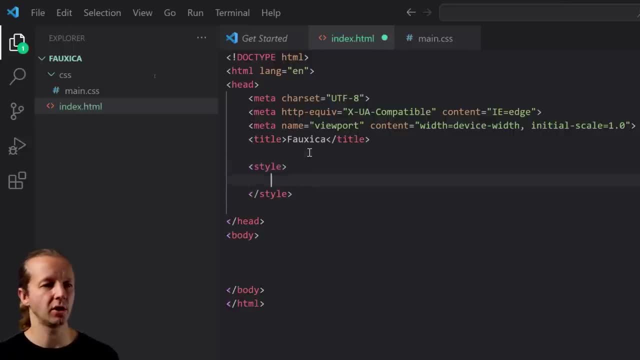 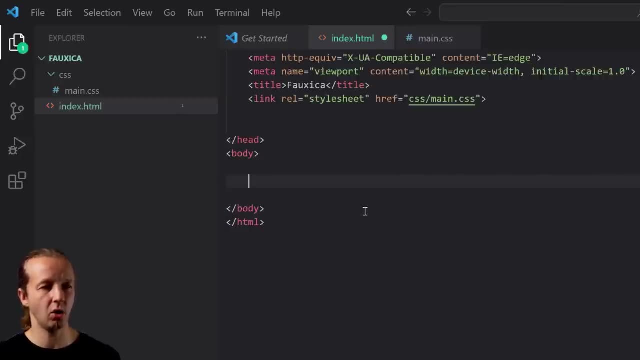 Might as well, just separate them out with individual files. So I'm gonna go ahead and back up, I'm gonna hit the Z a few times and we're ready to rock All right Now before we start writing code. another thing to pay attention to. 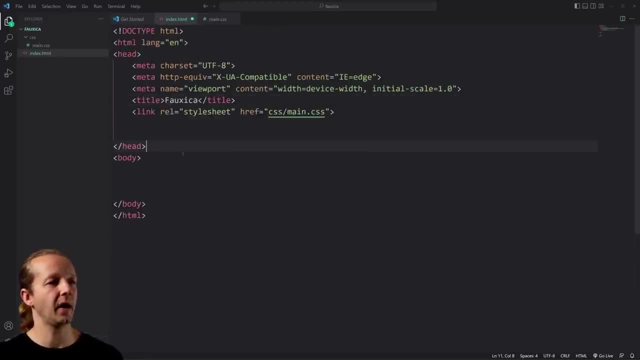 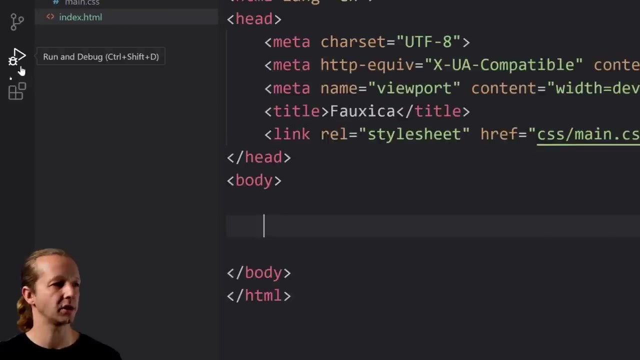 let me get this bigger- is a couple extensions. So Visual Studio Code, like Figma- if you watch the design version of this tutorial you'll know- has plugins or extensions, And that's right over here, right here in this section. 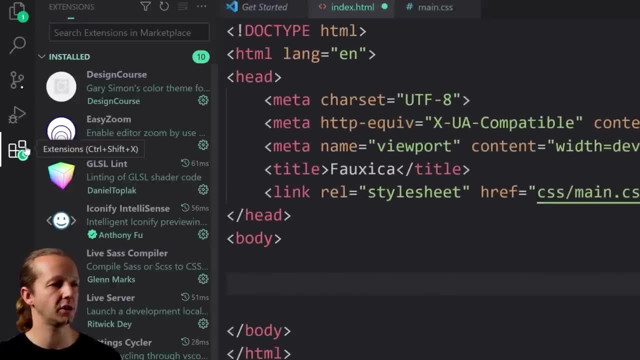 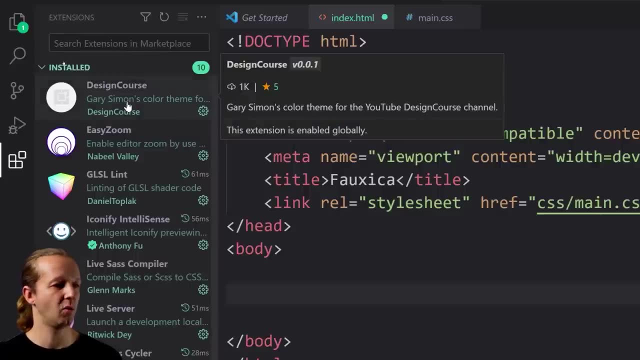 And we're gonna use just one. So if we click on extension, you can go ahead and, by the way, if you like my color scheme that I'm using here, you can search for design course and install that, But the one that we want is live server right here. 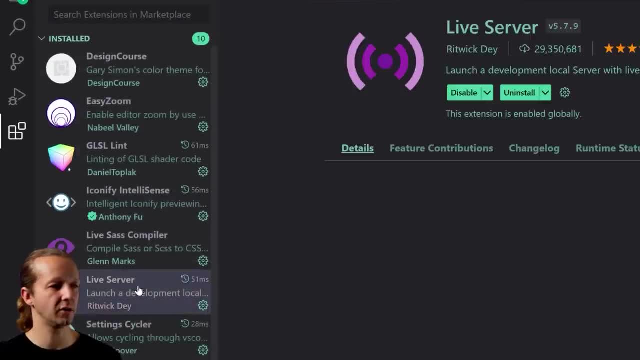 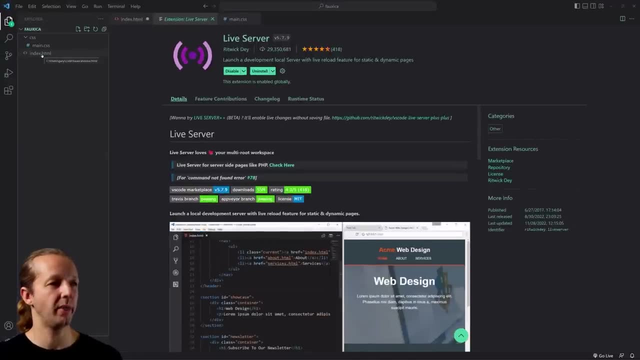 So just type live server in the search and you'll see live server. You click on it. it's gonna say install. go ahead and install that, All right. So after you've done that, then you can come back over here for indexhtml. 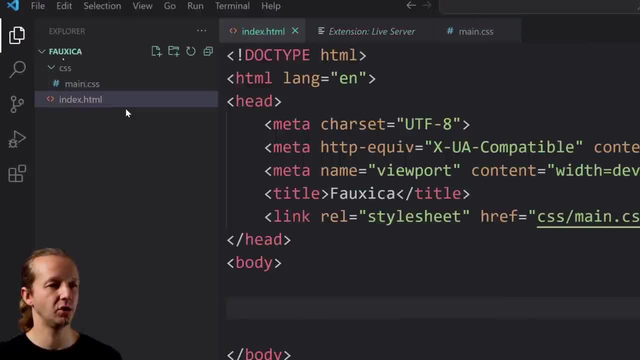 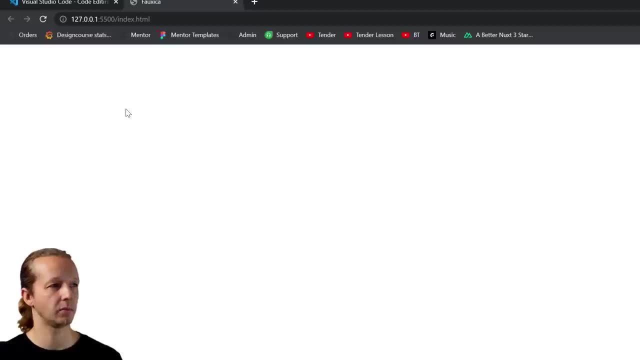 right click and open with live server. What that will do is open up your default browser. in my case it is Google Chrome. Let me get out of here. There we go, And here's our blank indexhtml. It's gonna show us exactly what we have so far in our HTML. 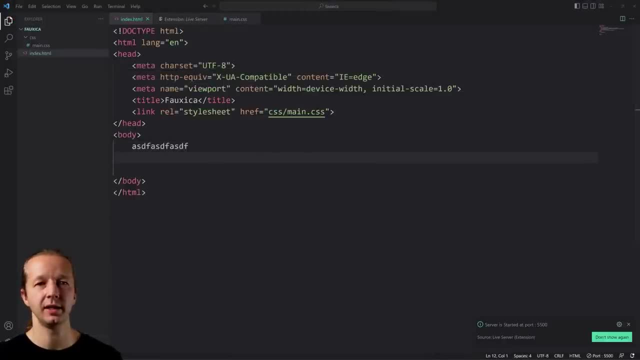 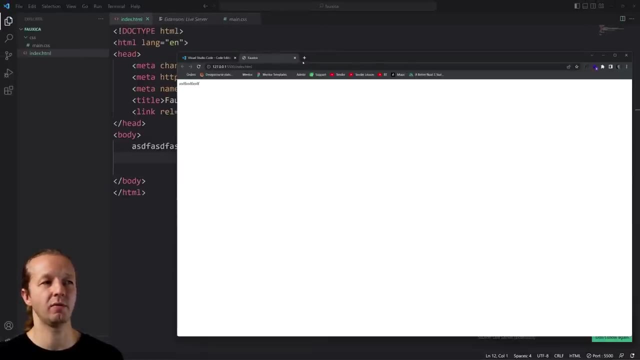 So you don't have to do this. but if I just do that real quick, hit save control S, you'll see right here it automatically refreshes for us And that way we can refer back and forth to the real document in the browser. 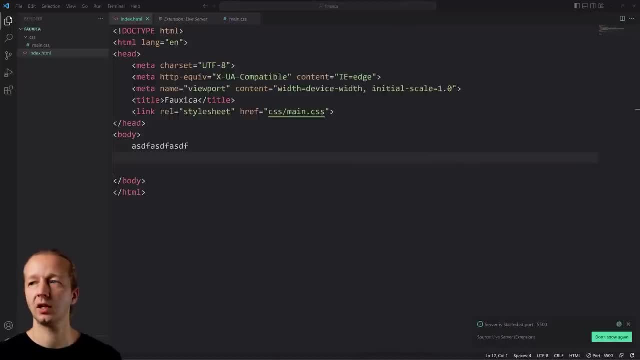 As we're recoding, Okay, So I'm just gonna minimize that or move that off the screen. And now what I'm going to do, rather, is we're gonna start writing our HTML, but that means we're gonna have to refer back and forth. 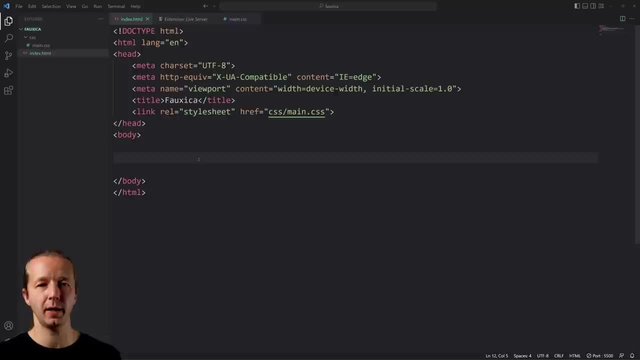 to our design prototype or our mock-up that's in Figma, to start to get an idea of where we're gonna start writing our and how we're gonna need to start writing our HTML structure here. So I'm gonna go back to this Figma document. 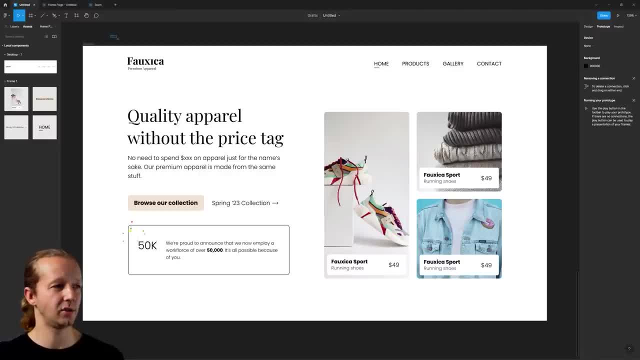 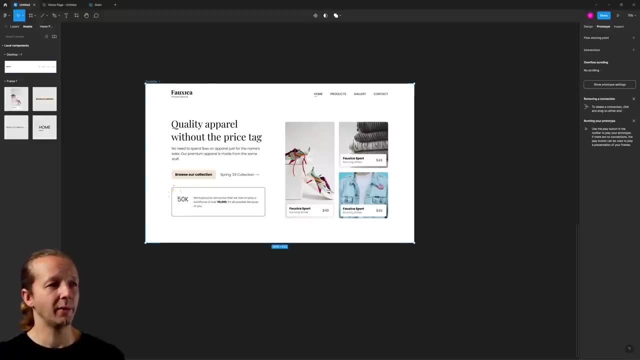 This is gonna be linked in the YouTube description. I advise you to definitely get a copy of this right here. There should be some simple instructions in the YouTube description on how to do that, And we're ready to rock now. Okay, So what I'm gonna do? 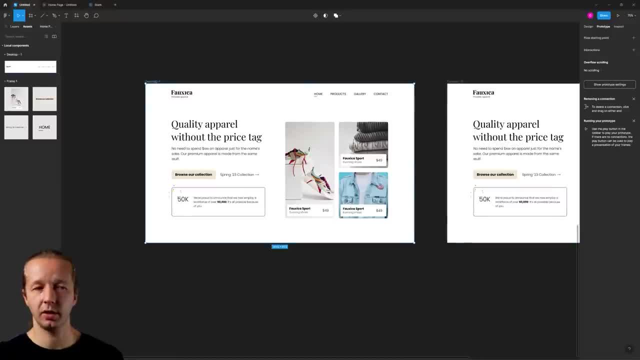 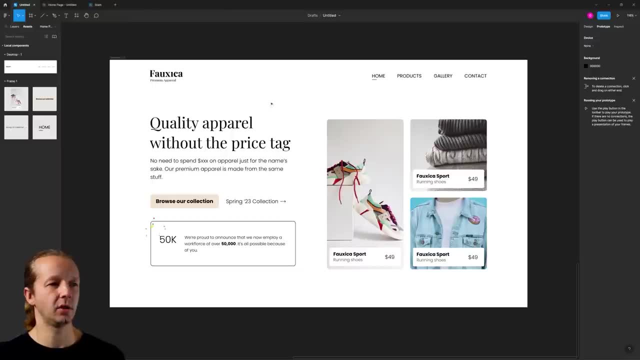 I'm gonna create a duplicate of this, So I'm just gonna take this: you can hit control D or just hit alt shift and just left click and drag over. So now we have a duplicate and we need to think about that too. that is. 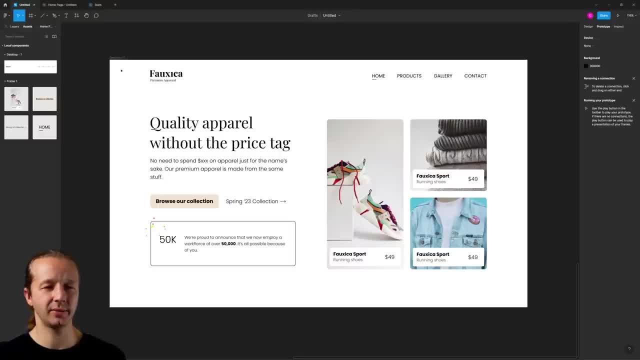 what does this mean? do this, does it mean if I remove theaires? So we're gonna do that. Now, what I'm gonna do is I'm gonna call this the default view. And here's what I'm gonna call this default view. 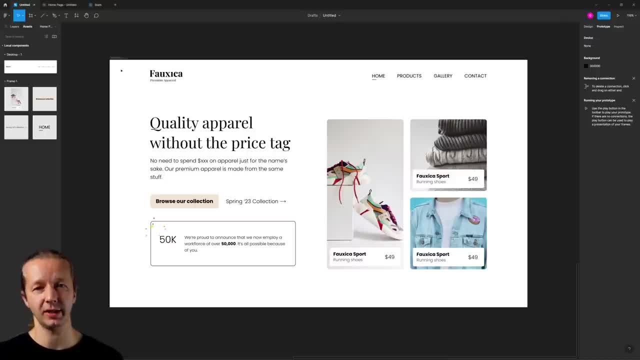 And what I'll do is I'm gonna save it. I'm gonna say: we're gonna call this the default view, because we wanna keep this as that default view And this is how you do it. So what we're gonna do here is we're gonna add: 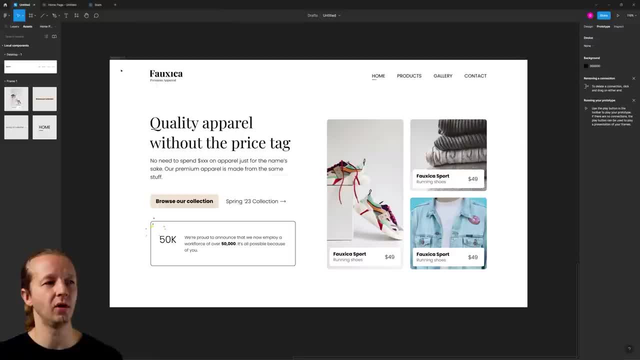 that to our pre-digital document. So we're gonna select that and we're gonna add that, And then we're gonna add this, we're gonna add this. to be able to do anything, it has to have html markup, it has to have the skeletons, so the 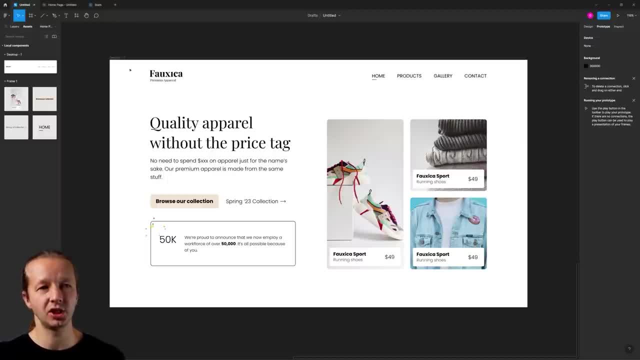 skeleton in this, in the html world, is just a bunch of rectangles, if you think about it. so let me go ahead and get to the rectangle tool. i'm going to hit r. you don't have to do this, but i'm just doing this um just to, to show you how to start thinking when you're structuring your html. 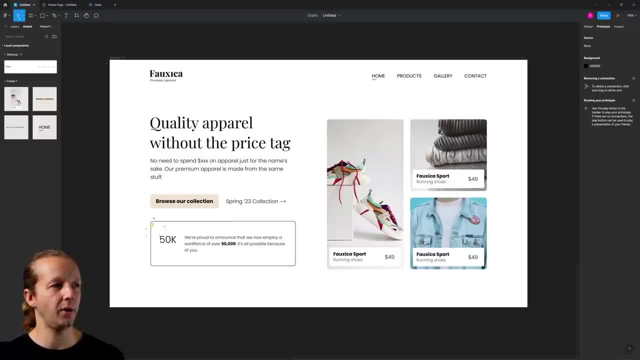 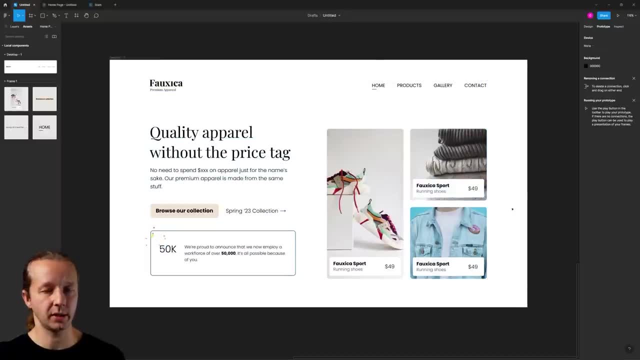 markup. so the very first thing that, um, i start with, and most people do as well, is a wrapper element. okay, um, and essentially notice how this is. this is emulating like a browser window right here. right, and, if i take everything real quickly, group it and center it right here: 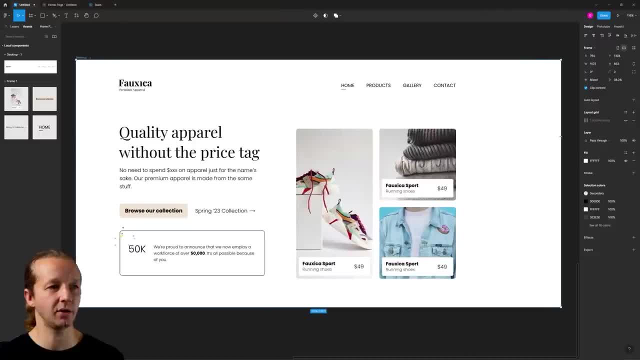 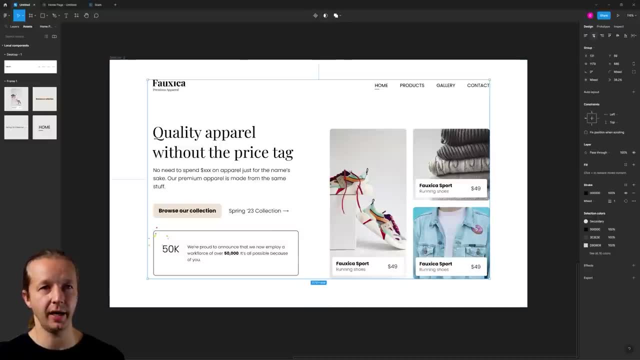 and then i simulate like a large desktop monitor. i just take all the data from the html. well, it's always going to. i don't have it doing it correctly right now, but i you want it to stay in a in the center. at a certain point there's equal white. 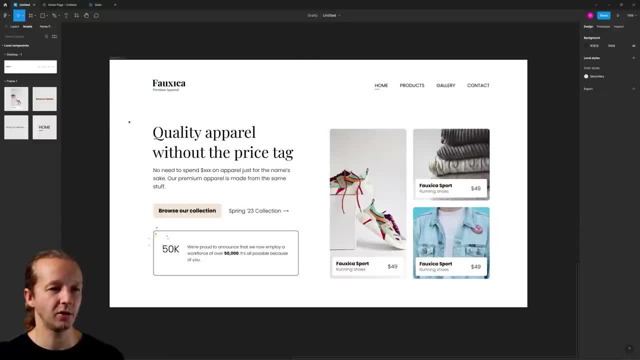 space on the very right and the very left as well, all right. so in order to achieve that, if you kind of think about it, everything is kind of wrapped- i'm going to make this red in a big rectangle, all right, what that wrapper element is, that's going to be our very first element and everything is going to 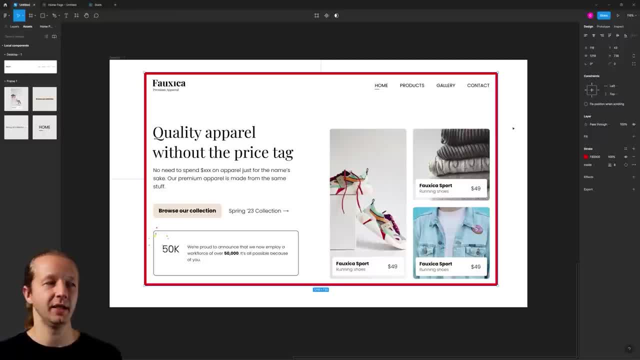 reside within that html element, and so, you'll see, this all comes full circle. by the way, when we get to the css i and finish it up and you'll see, oh okay, so that's why we needed a wrapper element. so we're going to wrap everything in a single element called wrapper, and it's going to be a. 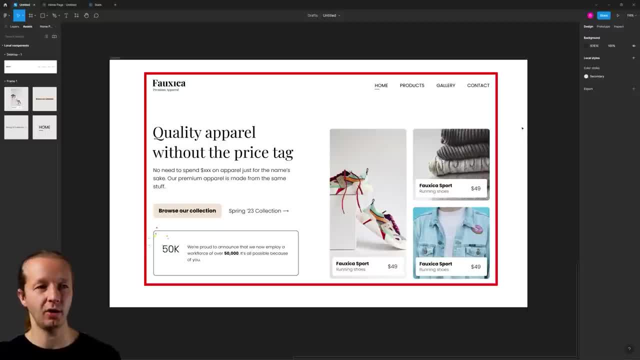 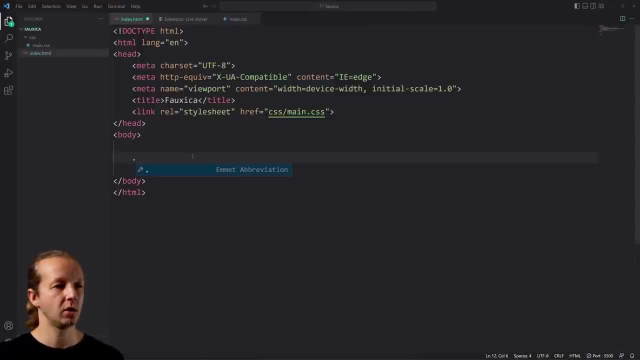 div html element. a div element in html is really for structural purposes for the most part, like creating like this little overall rectangle that you see here. so let's go ahead back to our visual studio code and we're going to type in a oh, and i'm going to use an emmett abbreviation for this. 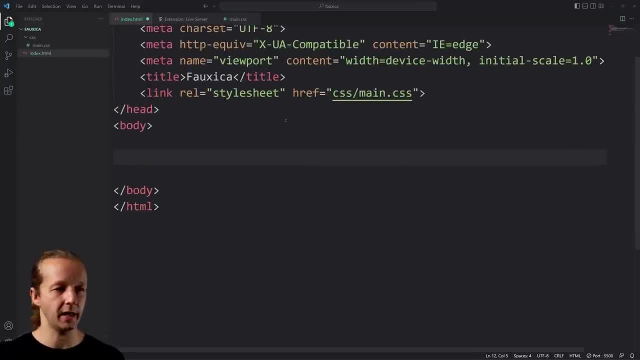 and so let me show you what i mean. i could type this out by hand like: div class equals wrapper, like that, and hit enter. or i could be intelligent and type in period, wrapper, enter. all right, so a period basically means it's going to create a div element as class. now, if you wanted to create 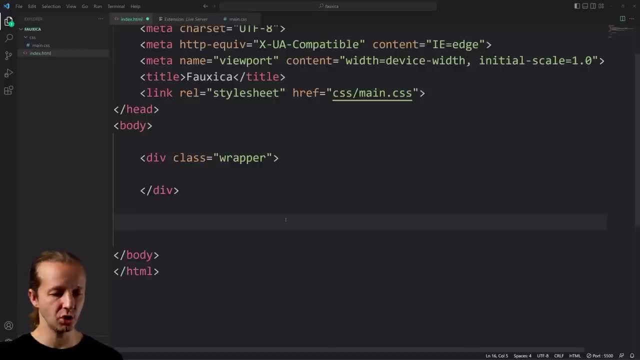 an id like use the id attribute instead. you would just do hash sign wrapper and that gives us an id attribute. but i typically very rarely use id attributes. we use classes. okay, so that's our first element. if we save it and go back nothing, you don't see anything. there's. 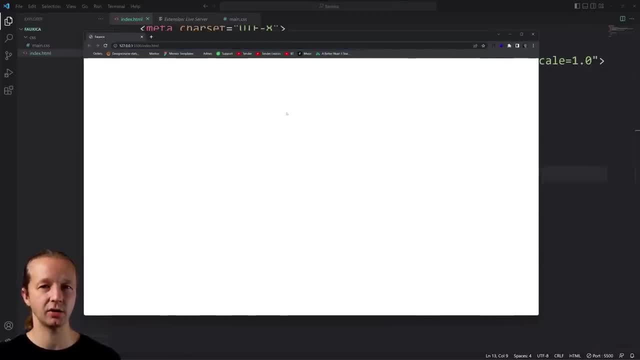 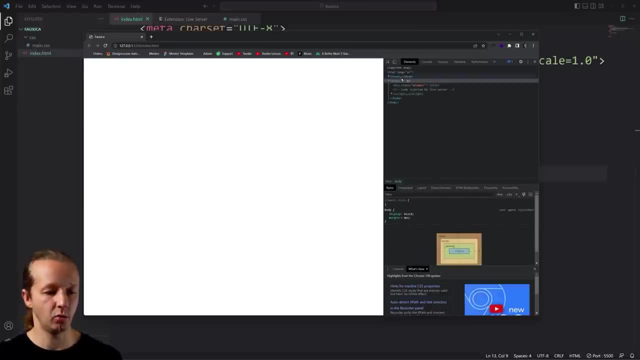 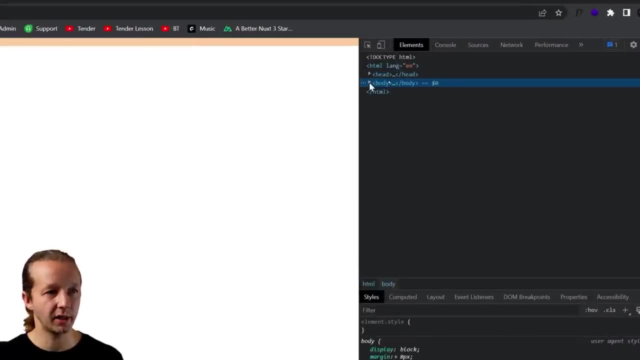 nothing present here, because a div element inherently has no style to it. all right with like css. so if i go to f12 and we look right here, this is the developer console. it kind of popped out here, um, and i we look at the html markup, we'll see div class wrapper. but it's just, it's something. 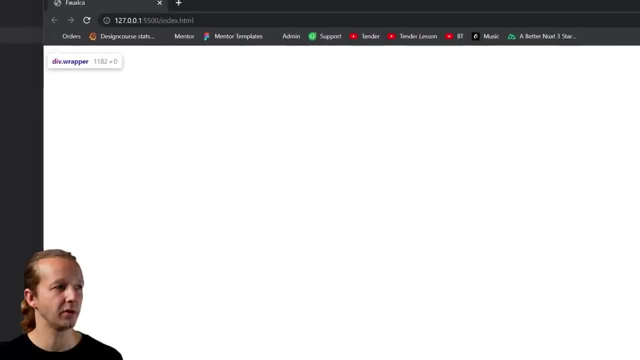 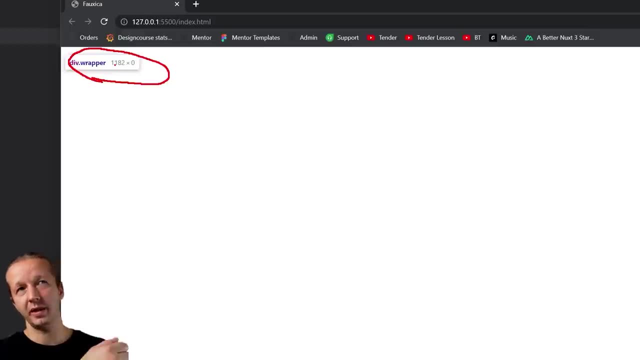 at all. it kind of shows this thing over here: div wrapper has no height but it has 100 of the width because it will. a div element will span by default 100 of whatever its parent container is. in this case it's the body element which goes all the way across, so it's 1182 pixels because that's. 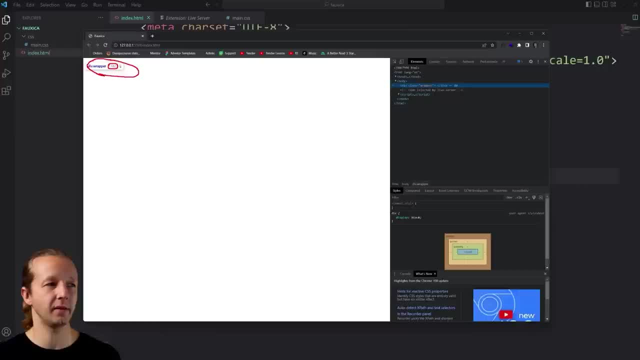 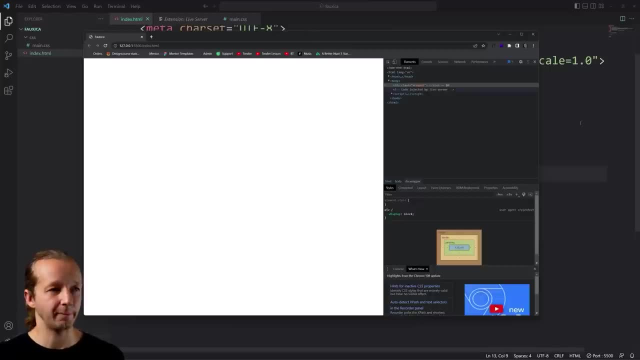 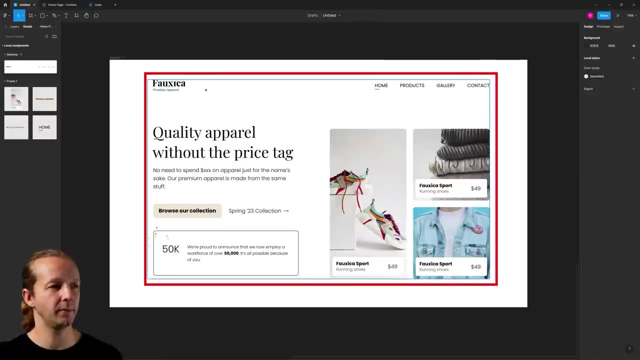 the width of my browser right now, but zero height. we don't see anything, even if we, if it did have height, we wouldn't see it anyways because it's it doesn't have a background color. it just be transparent, okay. so next up, what is the next element we need to count for in our markup? so, going back to figma, 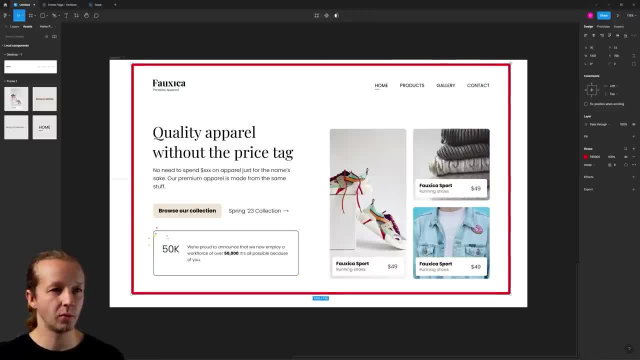 next up inside of this overall uh container, this wrapper, as we've called it. i'm going to duplicate this. the next element is going to be right here, if i can grab it, there we go. so it's going to be this element, and so we need an element that wraps around both the logo at the top. 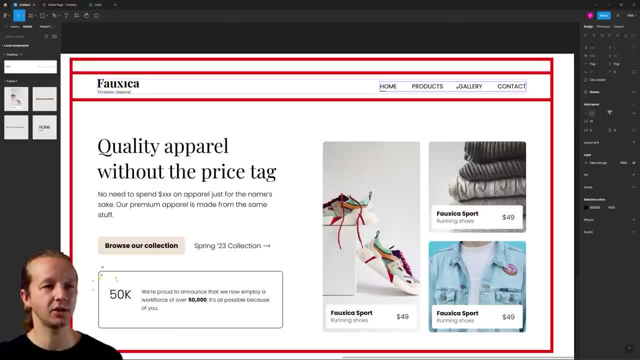 here, all right, and also this navigation. and the reason we we need a element that will wrap around both of those elements is so that, if you notice right here, there are two elements that are there in two columns. they're to the. there's one logo to the left and then a navigation to the right. 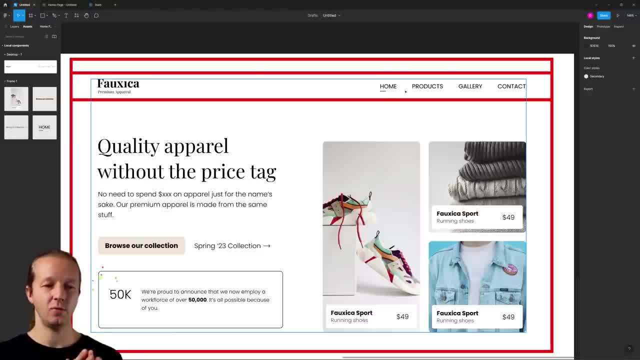 and so in order to instruct the browser to say: hey, we need two columns, rather than the default mode where things will just sit on top of each other into two rows, element around those two elements, and we instruct it with something like display flex and that will put it into two columns. hopefully that makes a little bit of sense at this point. 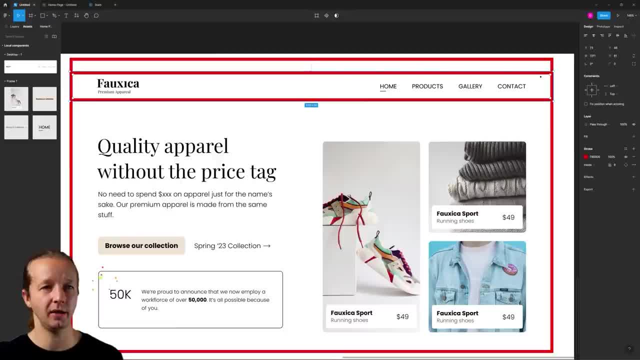 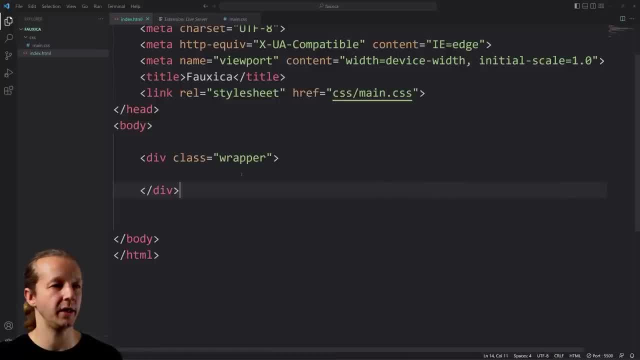 alright, and so we have tags that will accommodate this common pattern for a website- header, slash, navbar, and so that element would be right. here we're going to say header, just type header, enter, and there we go, all right, so the header element in in html. very important to use for good semantic HTML. so now we have to worry about what. 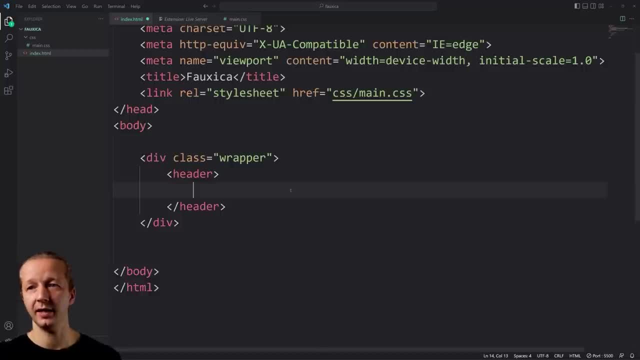 what's inside the header, the logo. alright, so we're gonna go ahead and we have to ask yourself: is the logo clickable? like, if you click the logo with your mouse, like, is it supposed to take you somewhere? yes, it almost always. should people expect to be able to click the logo to be able to go back to the 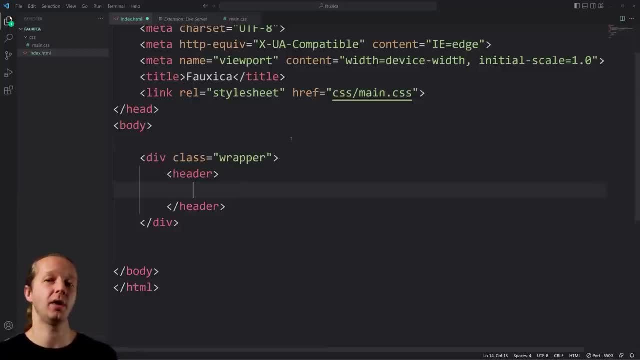 homepage. so if it's clickable it needs to be the HTML a element. so I'm going to type in another little bit of I, Emmett, just hit a enter. there we go href again, me remember, just like up here. that means it needs to go somewhere now. 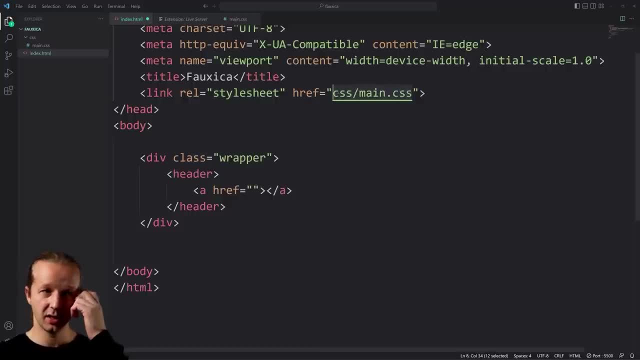 of course, in the case of the CSS right here in the head, that means it's going to go somewhere locally to like a file that's hosted on the server. in this case, we don't want that per se. we we want it to go actually nowhere, and that's because this isn't a real 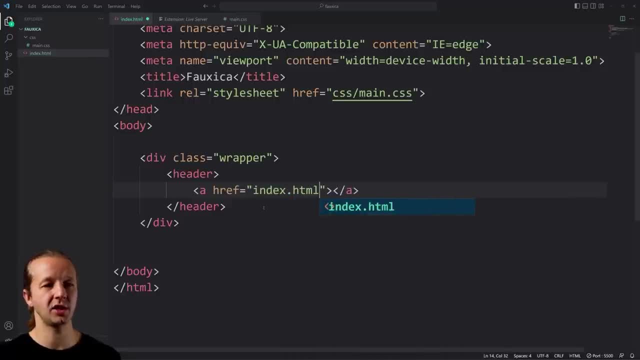 project. typically you could just put index dot HTML, if that's where your home page resides, or you can go. you could actually go like HTTP colon slash slash, oops, HTTPS colon slash slash. my eye like foxycacom. you could do that, but for us we're just gonna put the hash sign, which means you click it, nothing's. 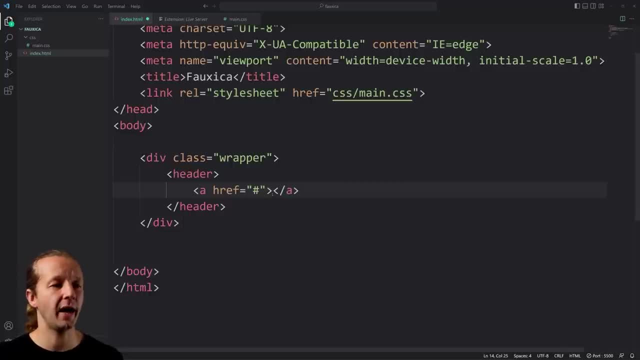 gonna happen. all right. so inside of here we have you what's called the anchor text. now notice: this is not a self-closing HTML element. we have an opening and then we have a closing tag here. that means we could put something in between it. you could just put some type like foxyca, but chances 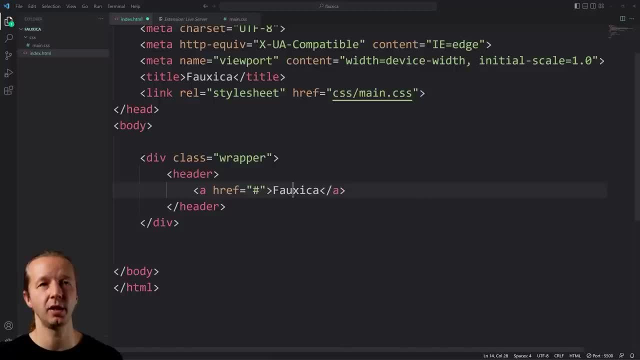 are. if you're dealing with a real project, it's going to be some type of I graphic design elements such like a logo, such as I'm an SVG element, which is the most common and most preferable element to use for a logo, and that's what we're going to do here is we're going to go to our 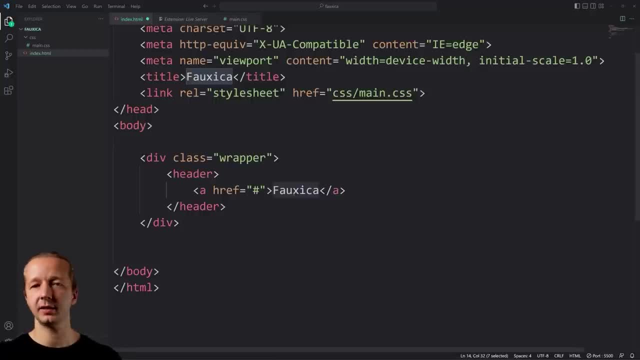 content writer here. so in ourILLTriала section. okay, I had information at the bottom here that says this very important file and I would encourage you guys to do that. going to our system header, right under our ายllt- magazineshtm folder, we are going to go out and 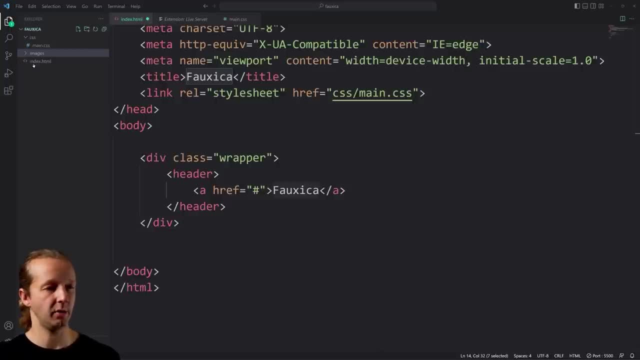 give this a new name. you want to open this up here to download your new file fall. it's going to open up just like this, no matter how big it is, it will never get so we have an empty images folder now pro tip, right click on the folder and 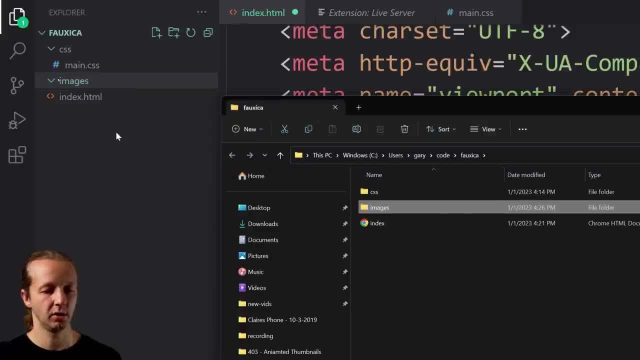 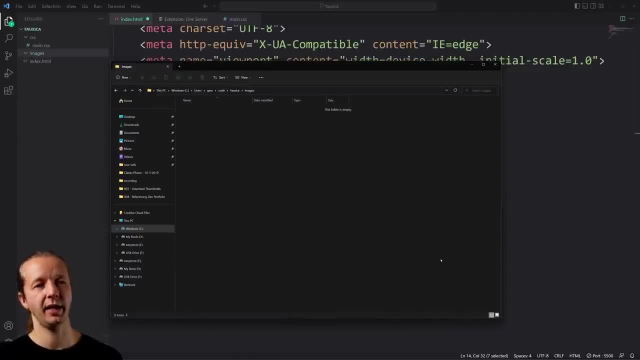 just to choose reveal in file explorer, alright, and we can double click and you can see this is now empty. so wherever you save those project files and go ahead inside the images folder in those that the project files just drag those over here, and I'm gonna do that right now actually, so I'm getting my reference. 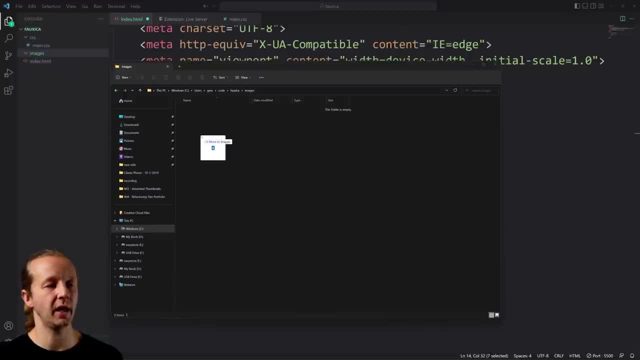 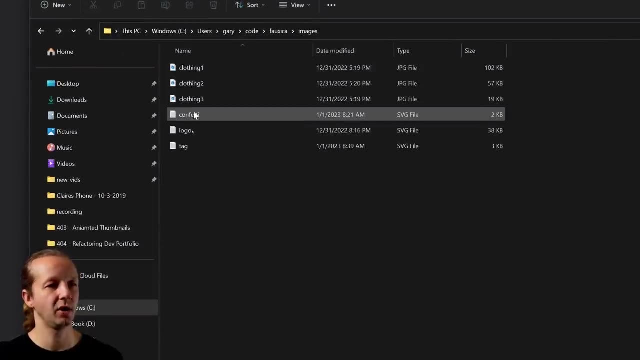 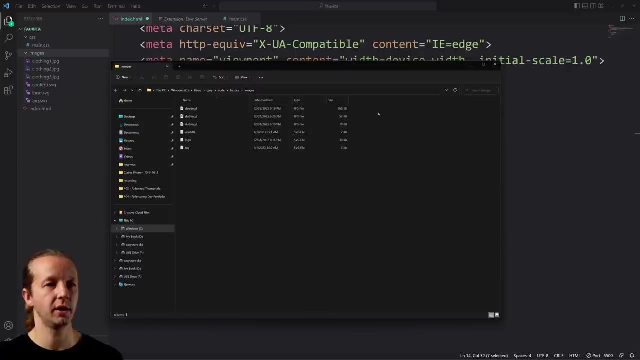 code and we just have a few, six different elements we're going to use. so let me zoom up. we have three JPEG files and then we have three SVG files that you can see right here as well. logo SVG is one of them. okay, so now we can go ahead and close that out and so in this case we're not going to use. 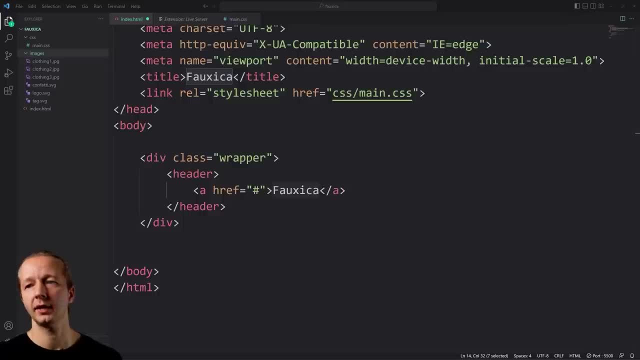 actual text as our anchor text for the a element. instead, we're gonna go ahead and use an image tag, an HTML image tag. so I'm going to type image img. enter again. this is going to have a source is going to point to a file on our server, although it. 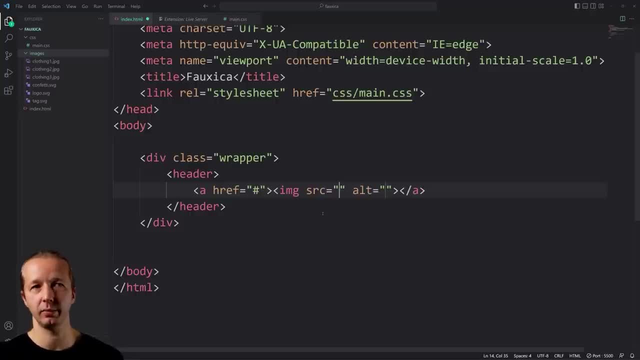 could be external server if another website's hosting, you know, a logo or something like that. for us it's going to be forward slash images, so it's going into the images folder into and specifying logosvg. we hit enter as we saw the little helper selector: alt is a tag, that or an. 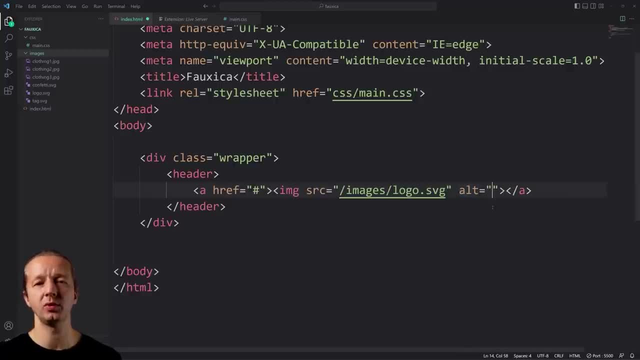 attribute, rather that i is important for people with screen readers, so obviously they cannot see your logo, so they use screen readers, and this is also, by the way, good for seo search engine optimization. uh, so so, for instance, in the case of screen readers, somebody is able to navigate. 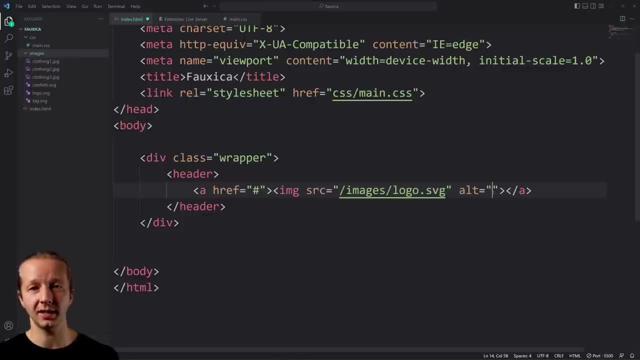 through with the keyboard and just kind of listen to what's happening on a ui, and so the alt will instruct them. what is this element? all right, so the alt is like literally what it will play back to that person via a screen reader. so for us we can say: foxica logo. there we go and hit save. so you can see we have two html elements. 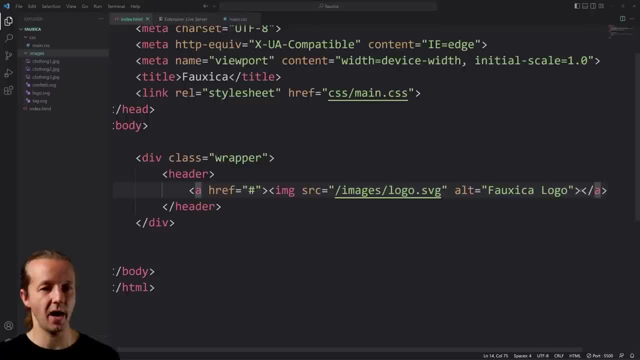 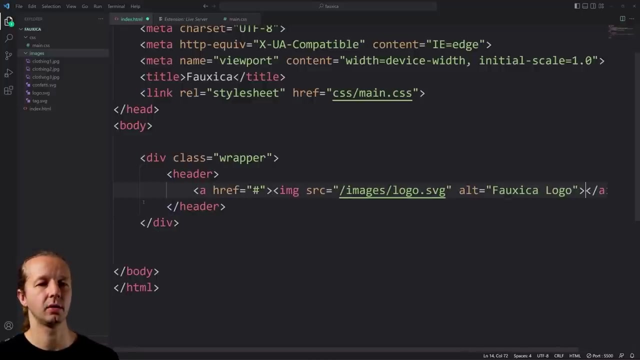 here. uh, we have the, the closing um element for the a element over here. sometimes people will go like this: and that's fine, that's not going to affect anything for me when it comes to simple things like a link, i just keep it all on the same line. all right, there we go. so next up. 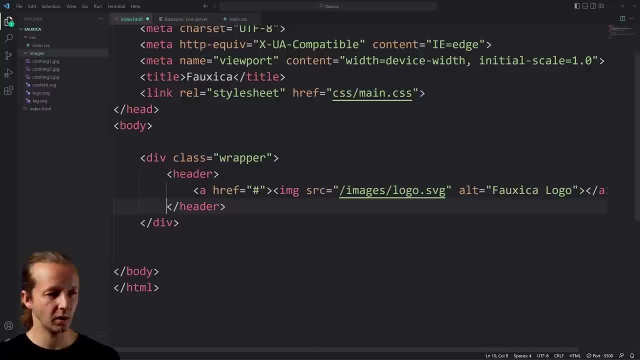 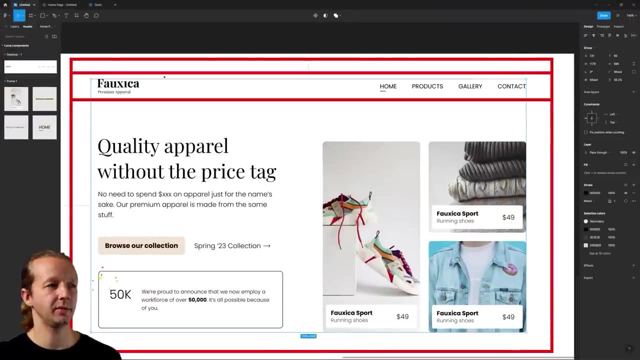 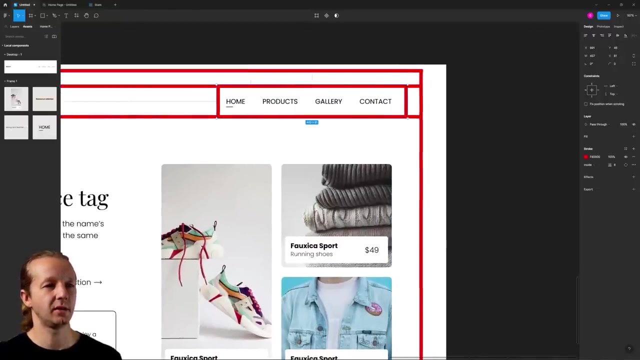 what else is after our logo? well, we have another element, and that is the actual website navigation. let's refer back here to this element, all right, so let me duplicate this. so we have our a element, which is this little block over here. let's duplicate that. now we have another element that needs to wrap around these four links, or these nav items, again, it. 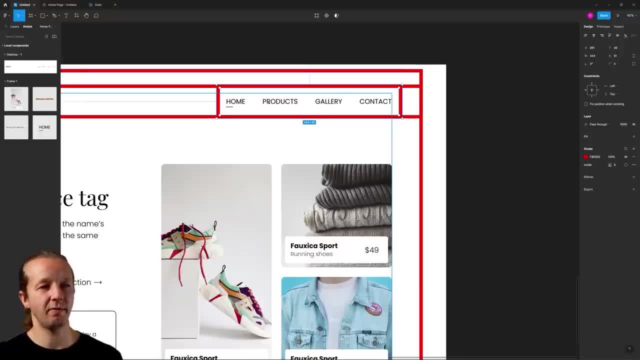 needs to wrap around, because these are, by default, going to be stacked vertically on top of each other. we don't want that. we don't want rows for our desktop. we want, we want columns, all right, and for that to happen, we have to have a parent element that wraps around it so that we can. 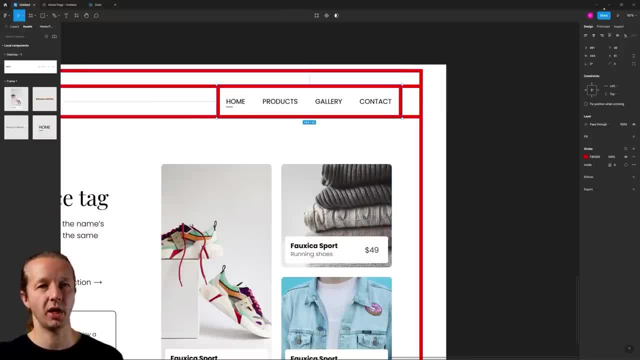 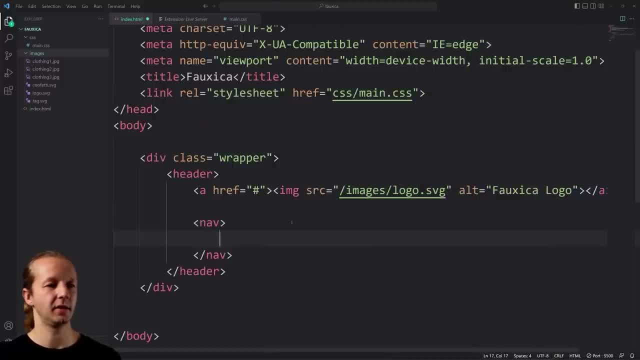 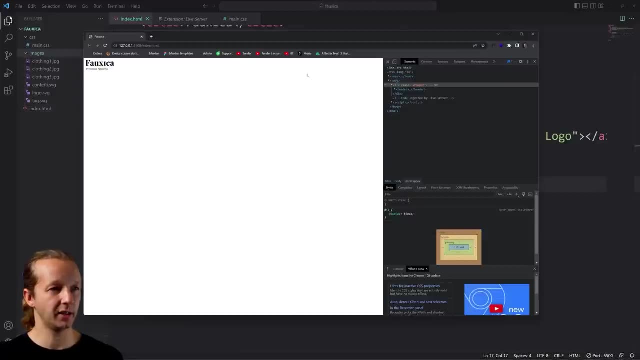 construct a browser to do that. so there's a another semantic html element that we use for this purpose and that is called nav. very simple nav, all right. so we're going to save this right now and we go to look at the result in the browser. i we're not going to see much of anything just yet, just the logo over here. 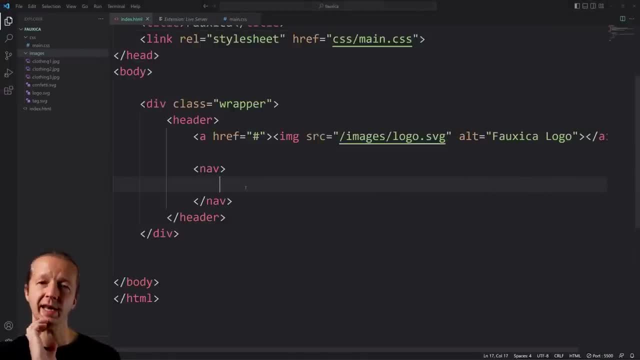 so now, when it comes to nav elements, we use another element inside of the nav element, i for basically structuring the type of data that's present. and the type of data that's present here is an unordered list- ul for short, that's the actual name of the. 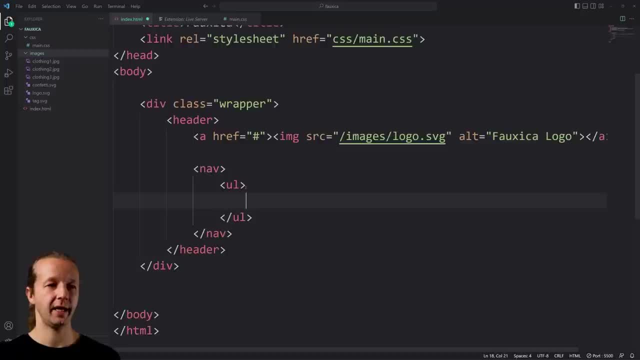 html tag: ul, enter. then inside of there we put our individual list items or li elements. so we hit li, enter. all right, so right now i could type, for instance, home: i'm going to hit shift, alt and down a few times and you know, we could change this to products. you don't have to follow along with. 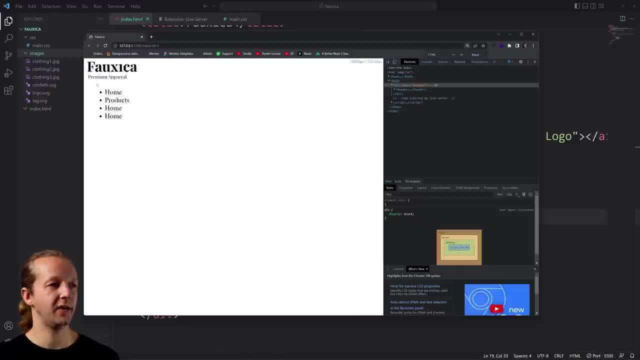 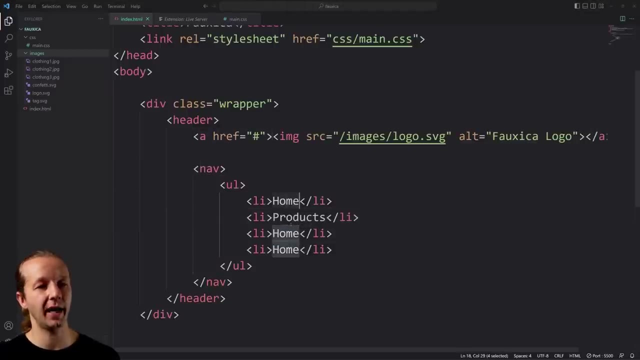 this part and if i hit save and i go back we'll see we have a list but they're not clickable. we don't want that right, so we have to make them clickable. how do we do that? we use a elements just like this in the logo. so we, inside of the li element, we put a enter. it's not going anywhere, so 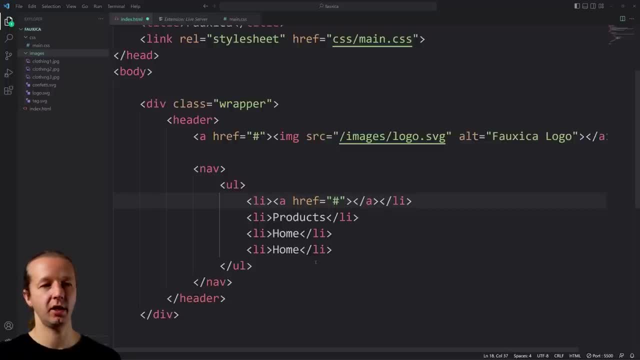 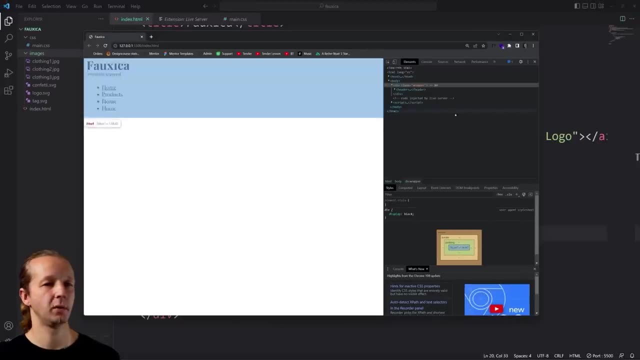 we're going to put in the little hash sign and then we're going to put in home. so now, if we save and go back, you'll see it is now a clickable link. now we need to do that for the other ones as well, so i'm going to go ahead and rate. 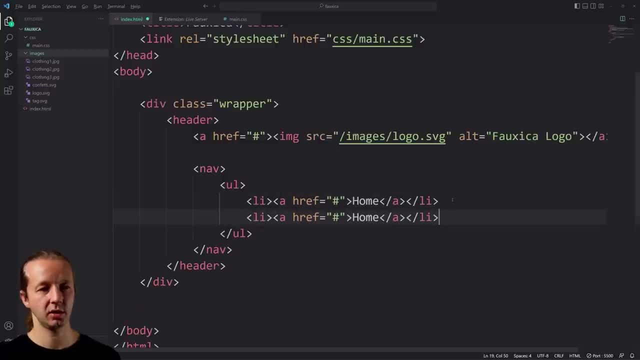 at the end of this line, shift alt down a few times just to replicate it. that way we don't have to sit there typing that out forever. products, gallery and finally, contact. now this is what it should look like in your browser, something similar to this: now notice. 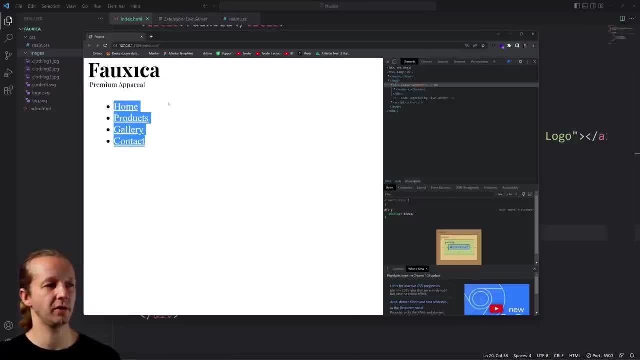 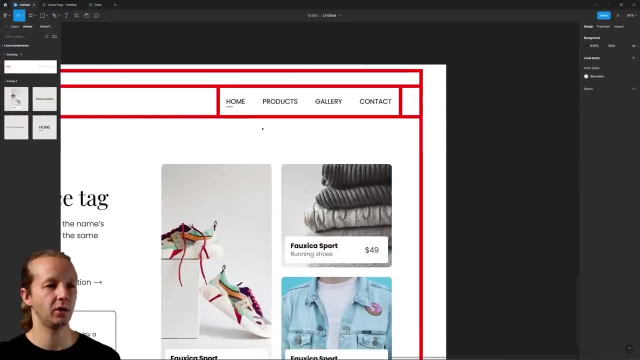 there's nothing that's different about any of these four compared to each other, except for the actual anchor text. you know home products, gallery contact. but if you notice, in our figma file we do have this little underline right here. that's the active state. i've described this. hopefully you 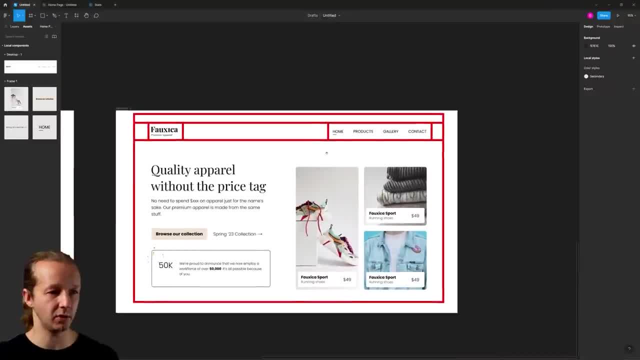 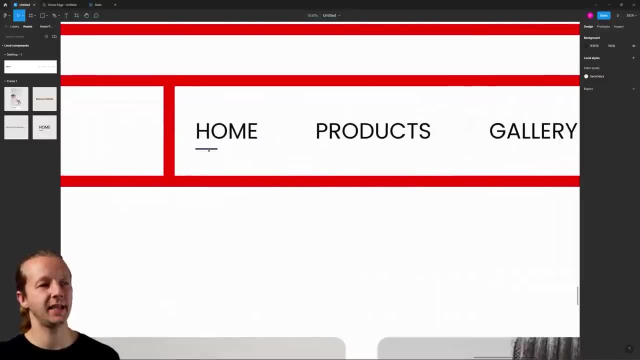 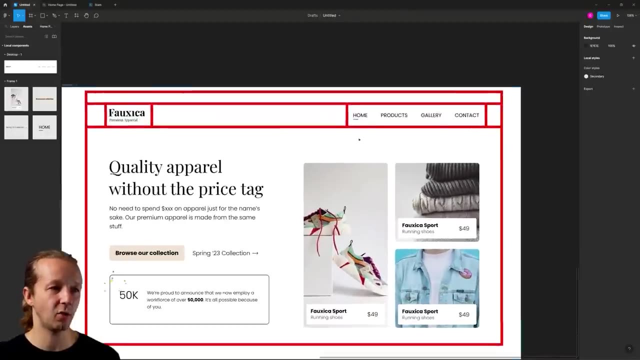 have watched the design portion of this about how to design. you know this whole website layout here, but this right here. we need a way for our css to add this underline based on the currently active page. in this case, we designed a home page, so that's why this little. 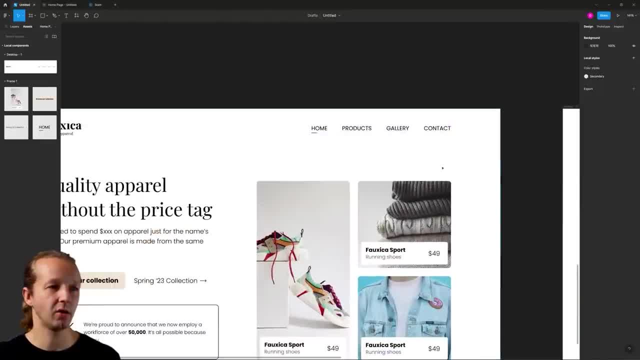 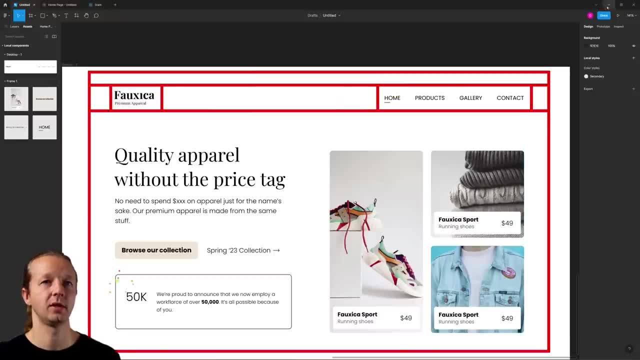 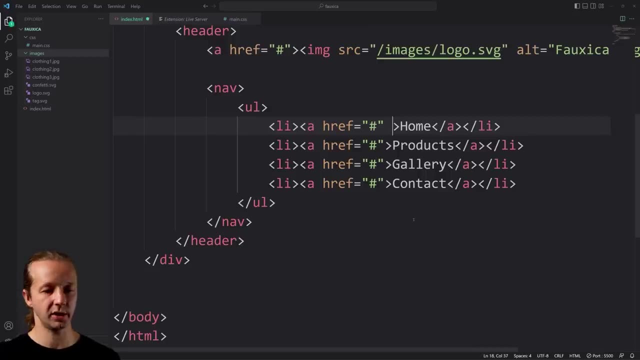 underline, you know, is right there. so to do that, we simply attach a class onto the associated home element. so to do that, we're going to come back here and we're right in the a element. right here, we're going to say: class equals active. all right, now, if we save this again. 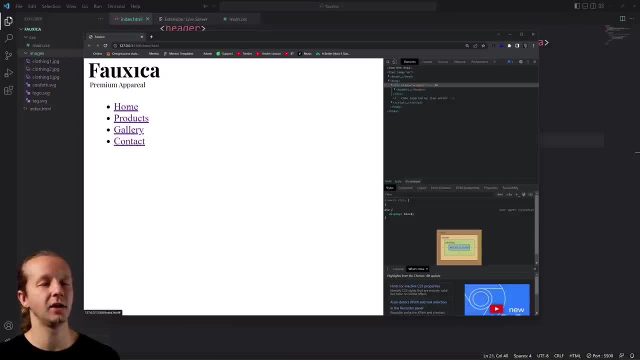 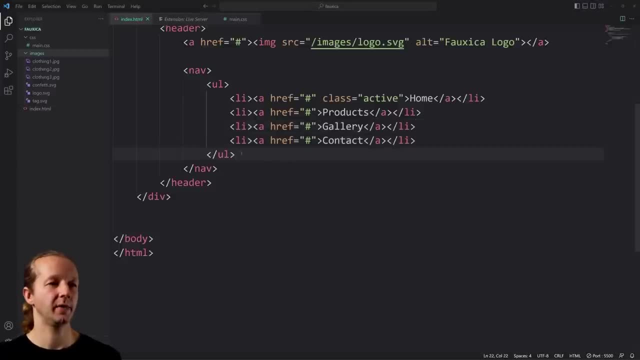 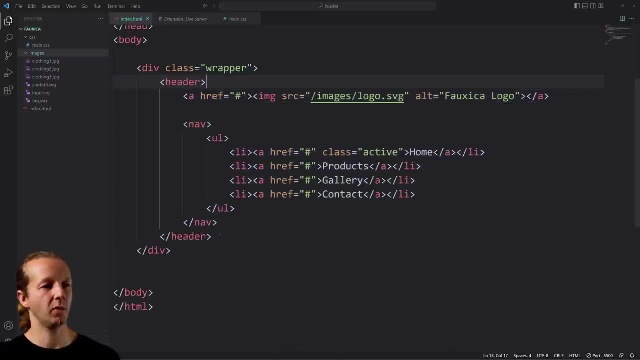 nothing's going to change because we have not yet got to the css portion. so you'll see how the this comes around. i don't expect you to understand it yet. if you're new to this, all right. and so that is the markup for our entire header portion, the top portion of the website. so now remember we. 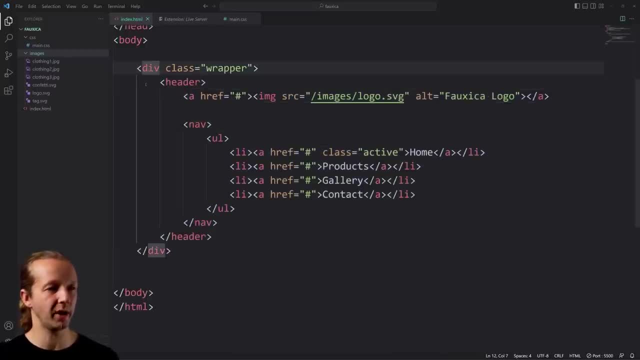 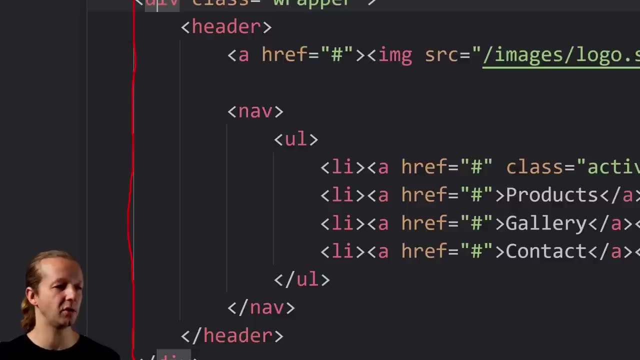 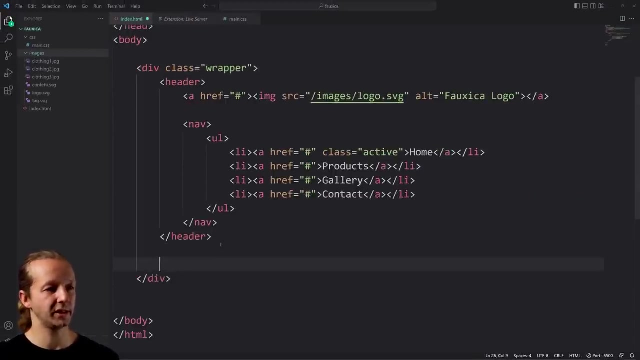 want to stay inside of this wrapper and you can notice, by the way i, this div element, div wrapper has a line that points all the way down to the closing div tag. that's handy, just so you know, kind of, where everything matches up. so we want to come just outside of the 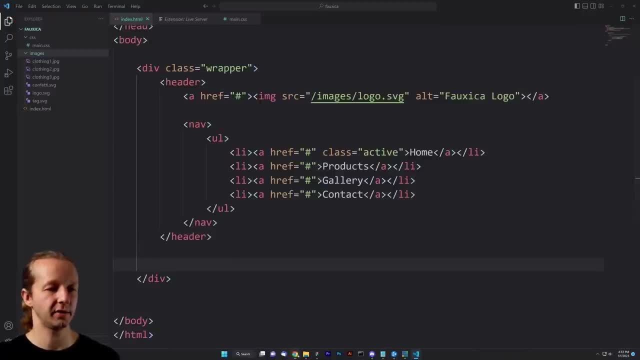 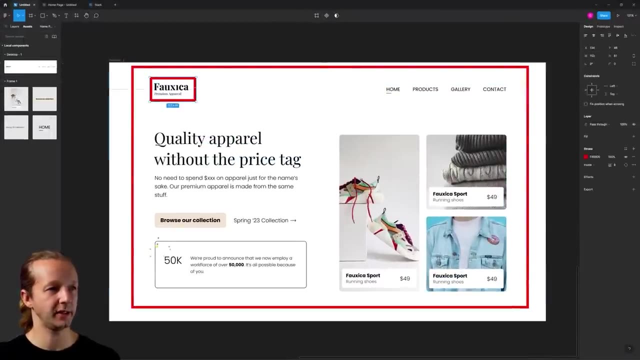 final column. so if this outer element of the label is positions on the outside side of the column, we're going to be able to yawn and zoom in all the way up and down. this is the closing header element to start writing our next element and let's focus on that. 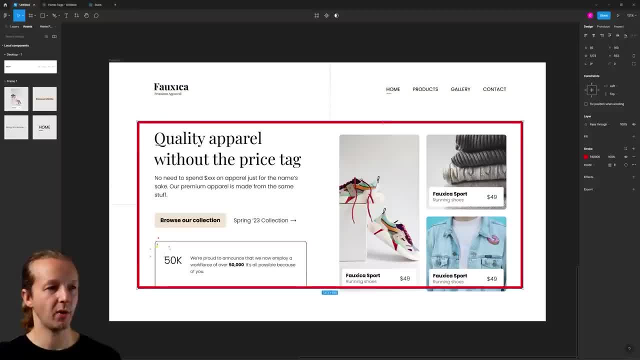 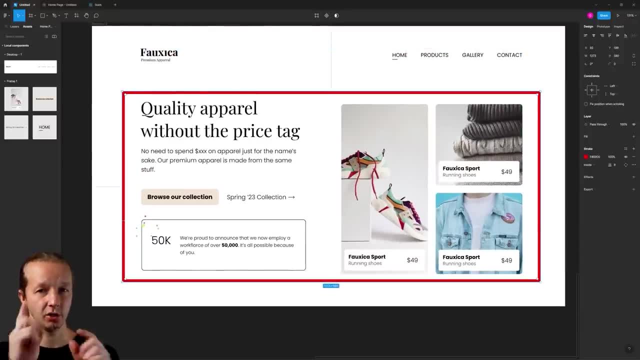 so our next element- and, by the way, i'm going to get rid of some of these because it's starting to really get crazy- so our next element- let's just pretend this one's still here- this outer element is going to be one that wraps around everything here. 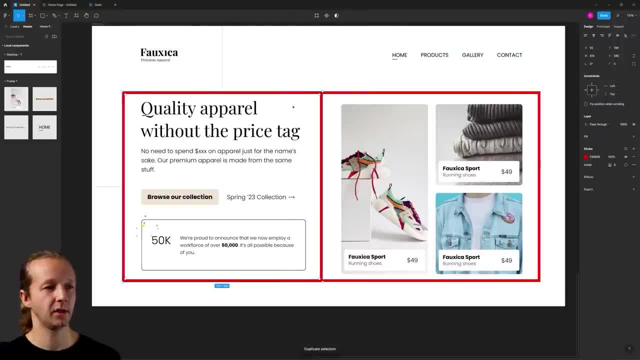 right here in the left And there's also one right here on the right. So you have to think about how you're going to structure and group your elements in HTML. And it's one of those things like once you're done watching this and you think you got it, and then you go to do it. 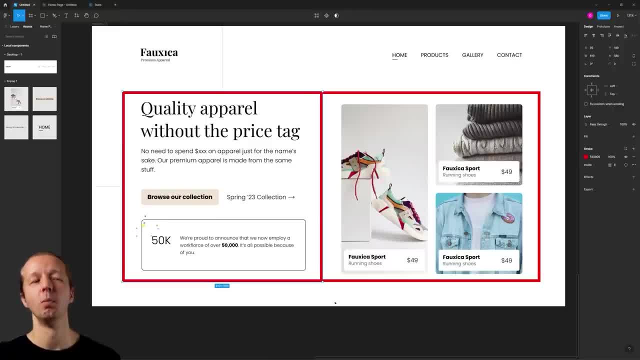 yourself. it will be confusing, It takes time, muscle memory- All right. That's why you should join the CSS course, because that's what it's all about. Anyhow, shameless plug. So we're going to create that. So first we have an outer element and then we have a left column and then a right. 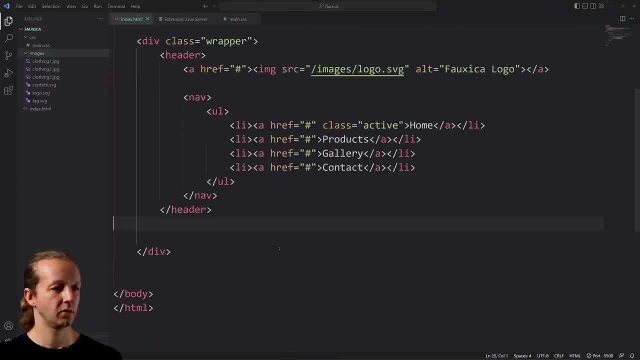 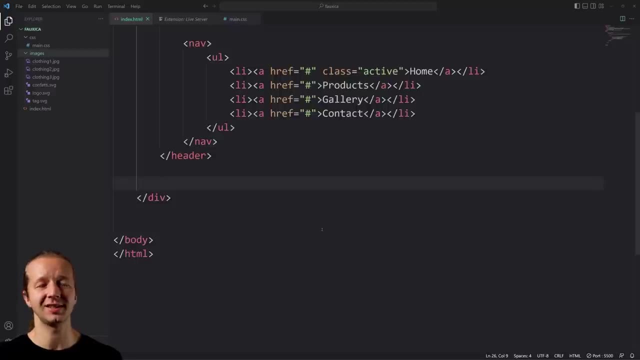 column, So let's create the markup for that. Now there's another semantic HTML element that you use commonly for these types of things. You could use the section element, or you can use the main element. For me, this is the main section of the actual website, So I'm going to use main and hit. 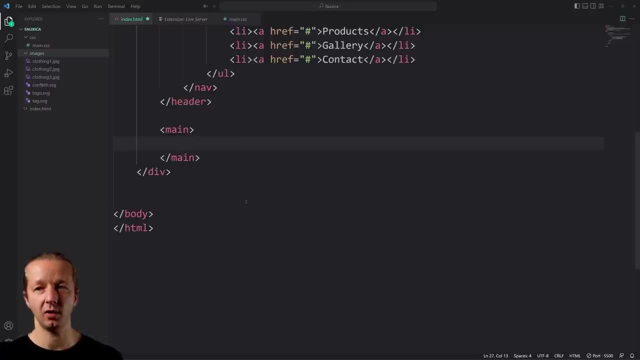 enter. All right. So then we have a left column. So I'm just going to put period Period, because it's going to be a class left hyphen call And then we'll do the same thing right here, Right hyphen call for column. Again, you can just name it left and right, That's fine. 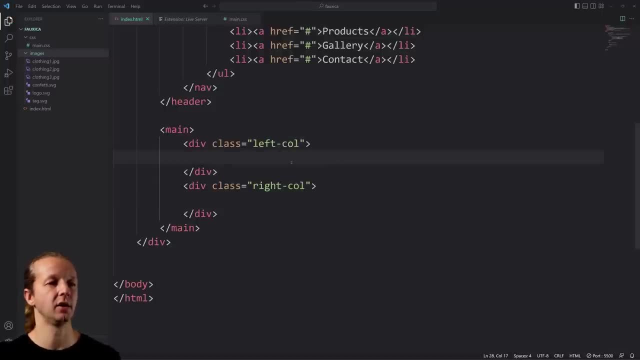 but I'm choosing to add the dash call at the end. Okay, And you can name these classes whatever you want. essentially, for the most part, Okay. So now that we have that, let's focus on the left column because, based on how you read from left to right, it just makes sense to do that. So 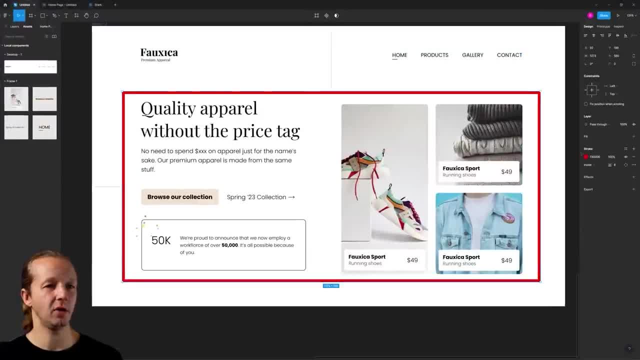 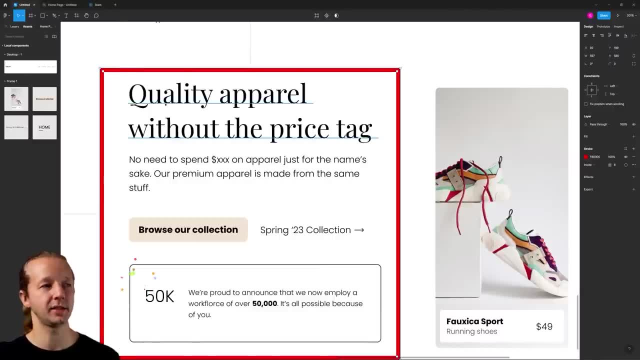 going back here, what do we have in this left column? Well, here is left call. right here, The first element that shows up top, bottom, left to right, it's this headline: quality apparel without the price tag. So headlines. every webpage typically should have a heading or a headline. 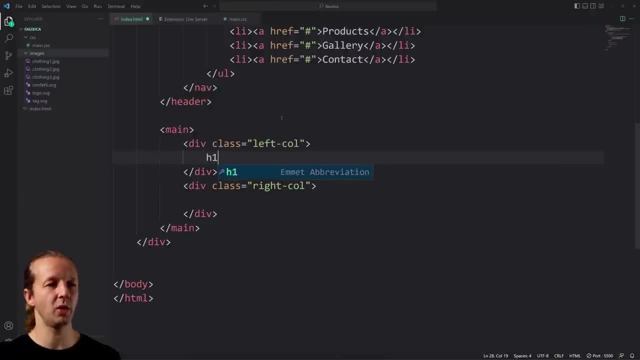 is created with the H1 element. All right, They have H1 all through: H2,, H3,, 4,, 5, and 6.. H1 should be the most important element. as you go and you work through different titles or subtitles, 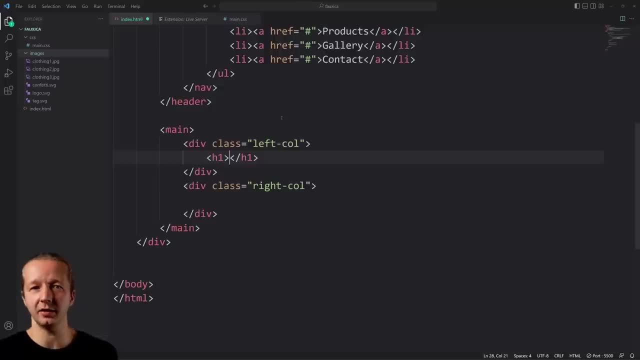 Notice and also note that you can have multiple H1 tags if you deem necessary. So we're going to go ahead and specify quality apparel without the price tag, All right, So let's save that. Let's see what our design looks like so far. Yep, It's ugly because there's no CSS that we've specified. 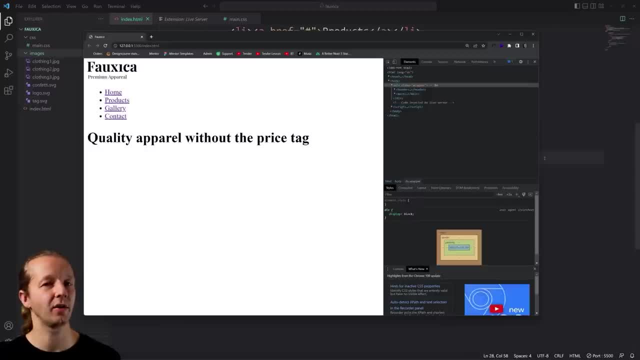 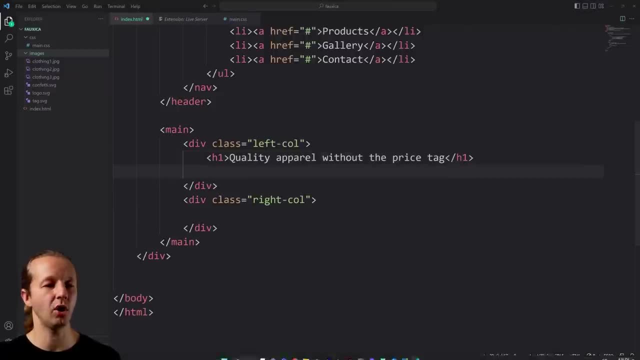 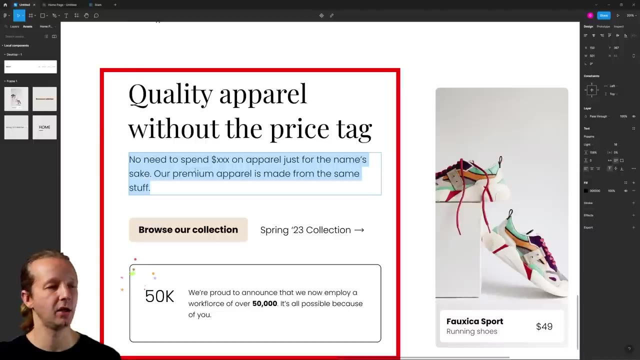 yet It's all going to look ridiculous like this so far, Kind of like the very, very early web and like the mid nineties. So after that we're going to have our subheading. That's this text right here. Go ahead and copy that. Just double click into it and hit control A, control C to copy. 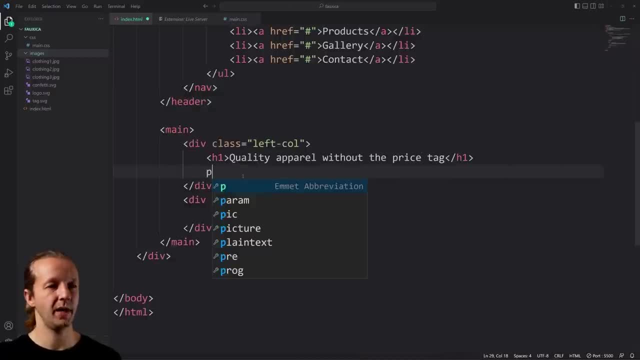 That way we can save ourselves typing. So hit P, enter. This is a paragraph tag. You use this very often, By the way. control B if you want to give yourself a little bit more space to collapse that sidebar, So control B. it will toggle that on and off. So I'm going to. 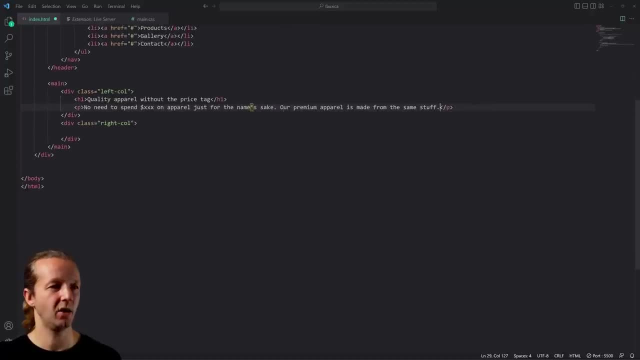 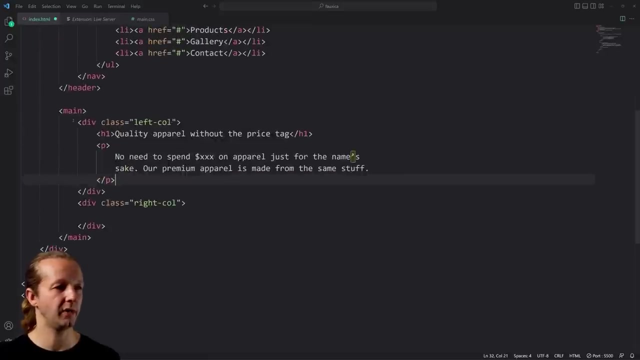 paste that in, All right. So it's pretty long here, And if you want to kind of save yourself from having to horizontally scroll around, you could do something like this: Just hit enter, enter. There we go. So now, if I zoom back up, just hitting enters here in your HTML isn't going to. 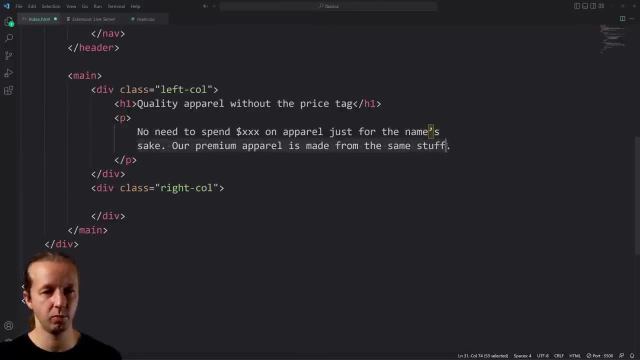 screw up anything. It's not going to like create a line. It's going to create a line. It's going to create a line right before the beginning of sake. So just understand that that you know you can organize things decently if you wish And notice. it'll just keep on going on the same line even. 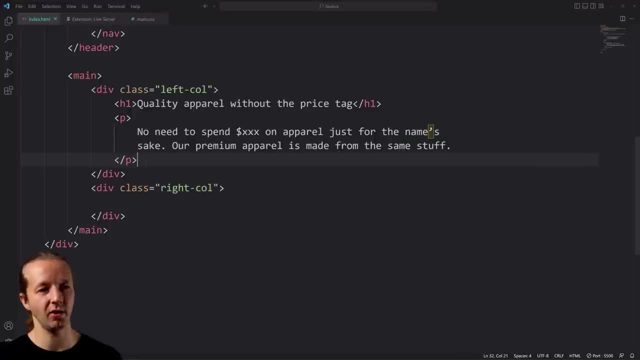 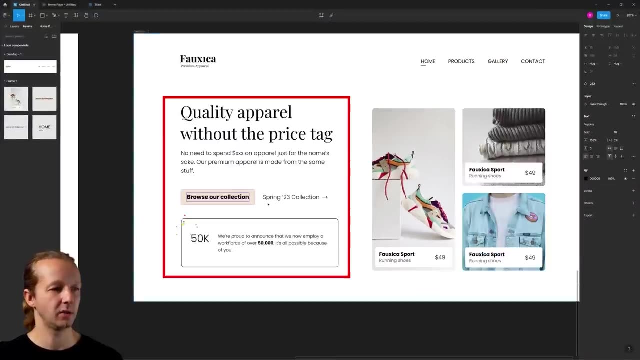 though we put a line break here, kind of in the editor itself. All right, So next up after that is going to be this section. We have two buttons- Guess what? Two columns. What does that mean? You remember? it means we have to put a. 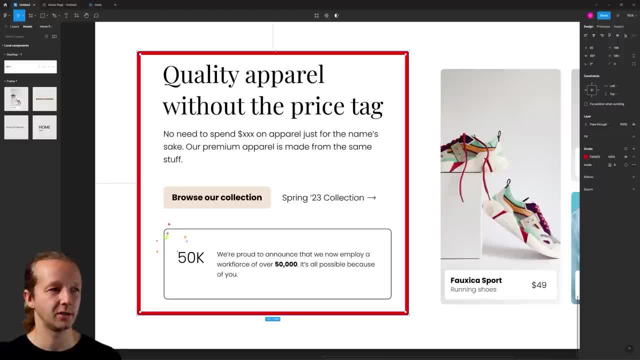 an HTML element around it. So just pretend all of our elements are still here. Again, just to quickly visualize, here's our H1. or rather, let me do this: This is the left column, this outer one right here. This is the H1.. 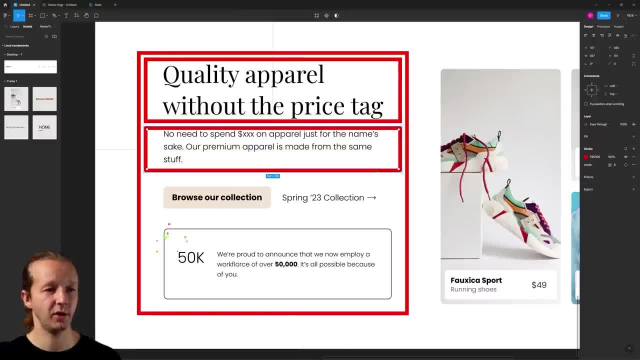 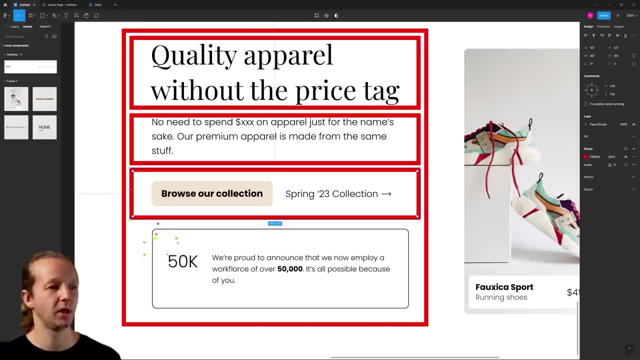 This right here is our paragraph element that we just created, And now we need one that wraps around these two elements to create those columns one to two, And then we have to do duplicate that even further, And then we'll have an element for the button, And then also duplicate that. 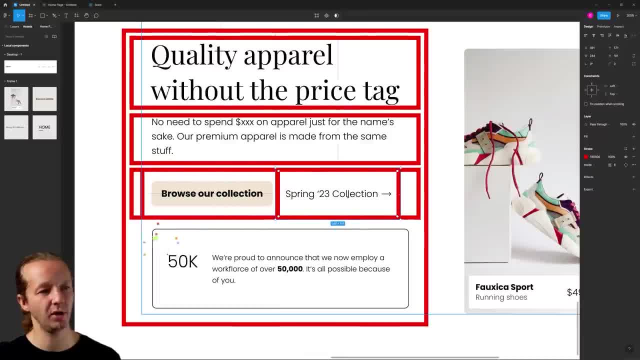 and element for this secondary button right here this spring. See, I'm telling you, it's all just rectangles, Okay, So let's delete some of these and let's create this markup there. Now, sometimes, when it comes to your semantic HTML elements, you can get so specific, like we. 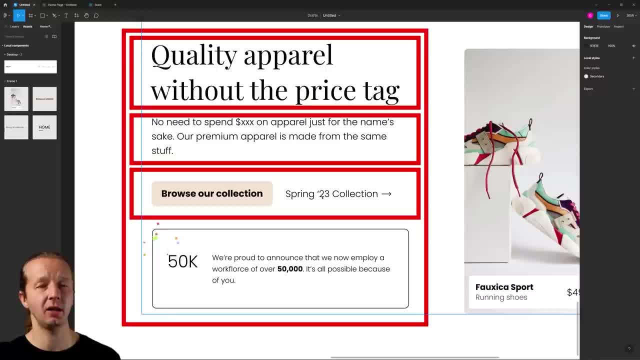 are like two call to actions. Like there's not a HTML element called call to action- And that's what we call these. Like it's the primary thing we want people to do is to click something or do something. There's no HTML element. 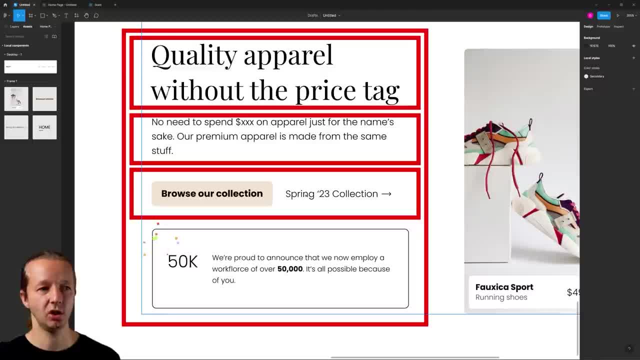 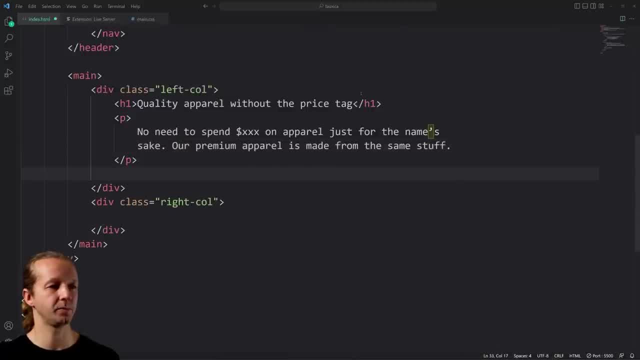 called CTA or call to action. So in that case we can just use our own div class for that. So we're just going to specify right here a class called CTA: hyphen BTNS for buttons. All right, So we just, we just did that overall. 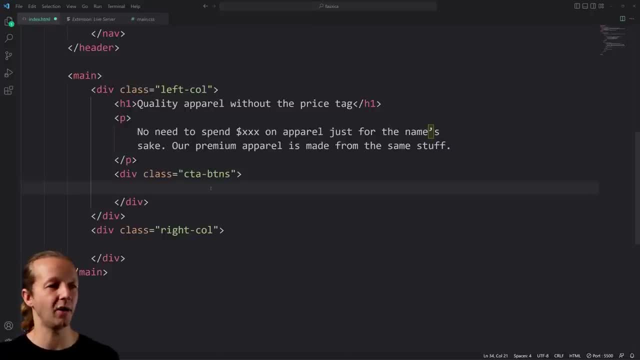 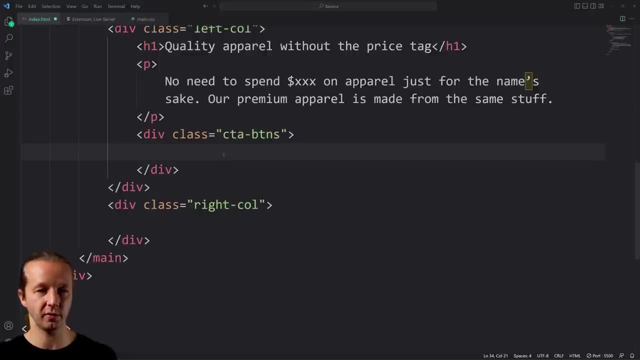 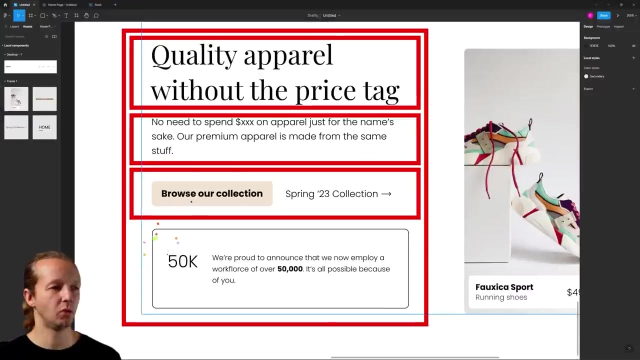 Red sort of fake rectangle thing around those. Now, inside of here we have to specify that primary call to action button, the beige one that we saw first, and then the other one that says bring 23 collection. So if we refer back to the design, we'll see this button consists of an. 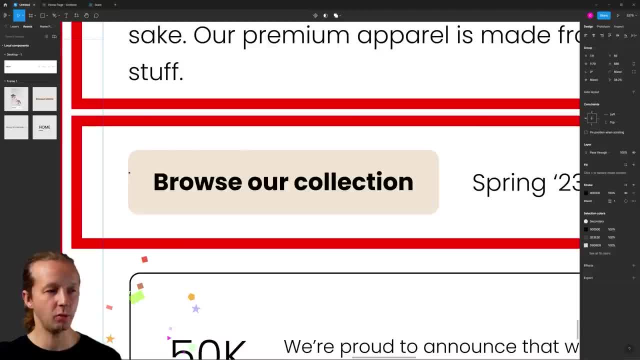 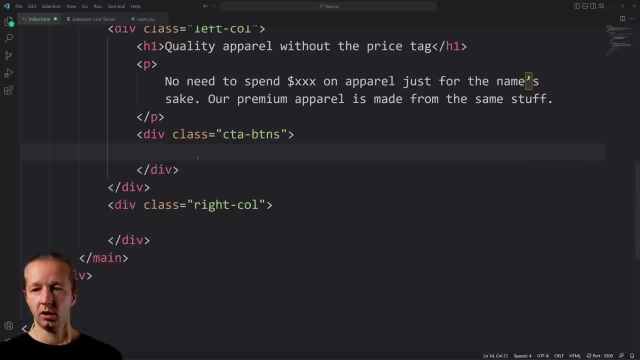 element, this beige sort of a rounded corner thing which we'll achieve in CSS, and then the type inside of it. All right, So here's how we do that. For this, we're going to use an, A element, and we're going to give it a. 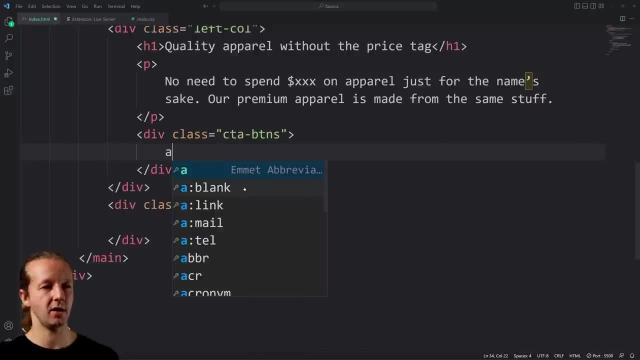 class called primary hyphen CTA, So A period, and this is an M abbreviation- primary hyphen CTA. So if you hit enter, it produces this HTML force, which is exactly what we need. This is fake, So it's just going to go to hash sign And then inside of it we're going to put in the actual 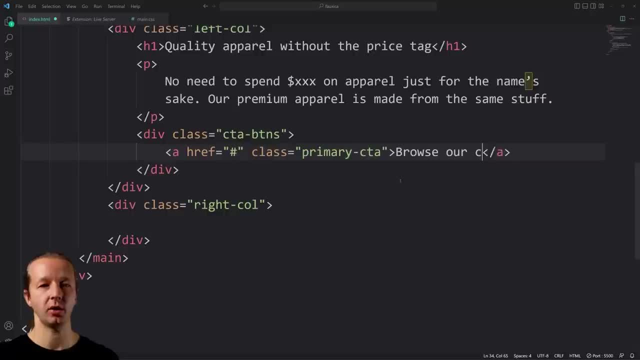 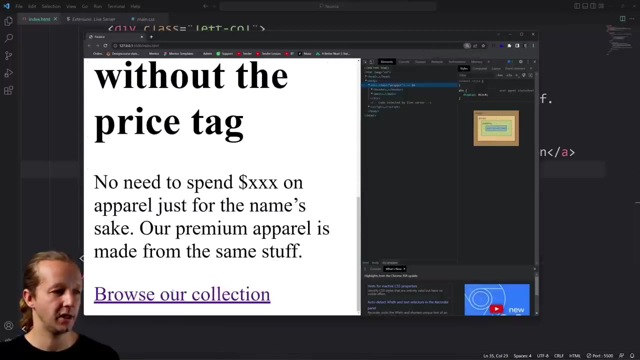 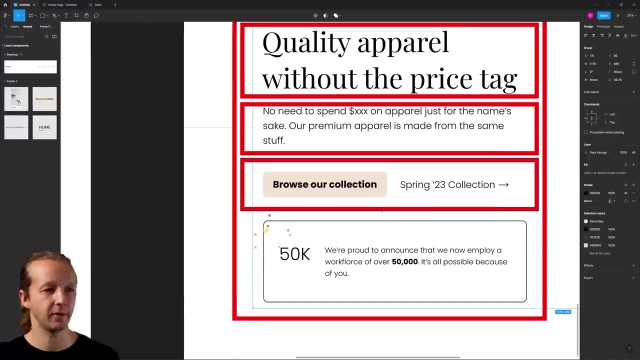 button text. So here's what that looks like. Okay, And then we want to add an element here on top, and then I need to add a hash sign or an A element, and this is going to create the. Now we have to do this one. Now, this one's a little bit more tricky because- notice, it has an associated. 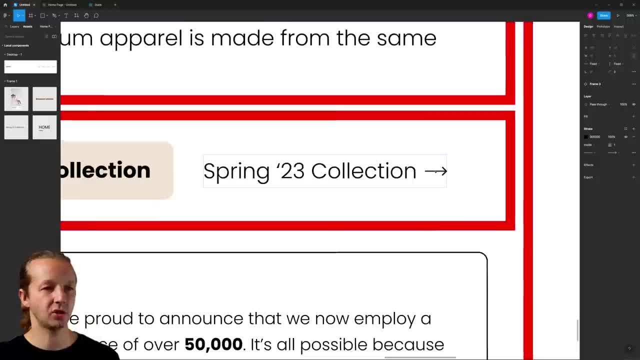 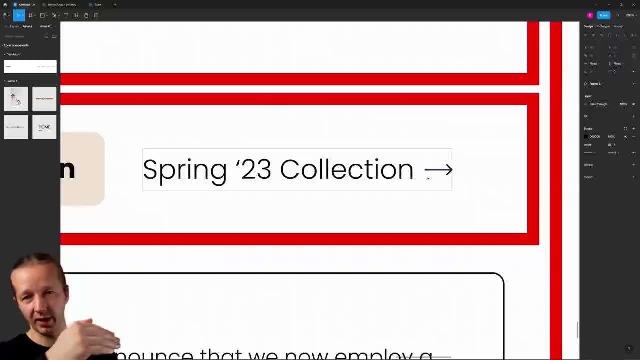 icon, this little right arrow, I so, if you think about it again, columns. what does that mean? we have to have an overall element that wraps around it in HTML. that will provide the structure for this text in this icon to be next to each other in column format, so to do. 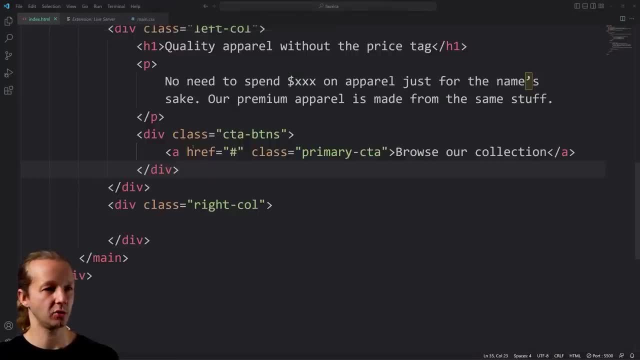 that let's go back, and this will be still inside of our CTA btns class. we're going to specify one called a link, called secondary CTA: hit, enter, hit, enter again, oops, put a hash sign and then come out here between these elements: hit. 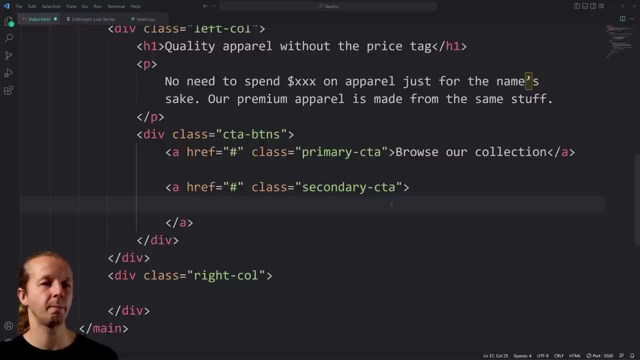 enter again, and the reason this time I'm going to be putting I'm the closing tag beneath it as opposed to on the same line, is because we're gonna have two elements inside of this. a element all right, because, remember, we have two elements. there's a two columns, one and two right. 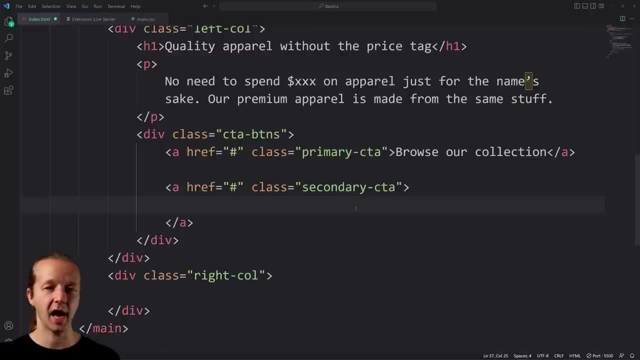 and so that's the text and the icon. so for the text, we need to wrap the actual anchor text in its own tag as well. it could be a div element or a generic span element, and that's what I typically use for this type of scenario. span enter and. 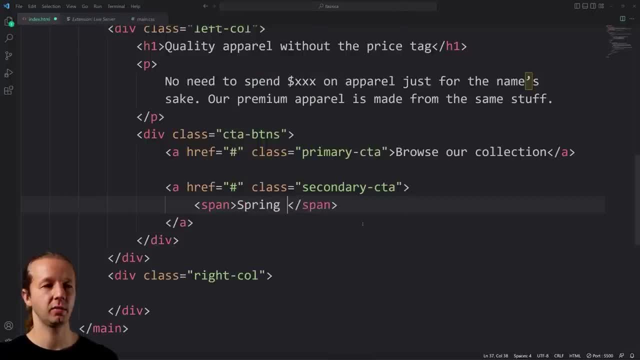 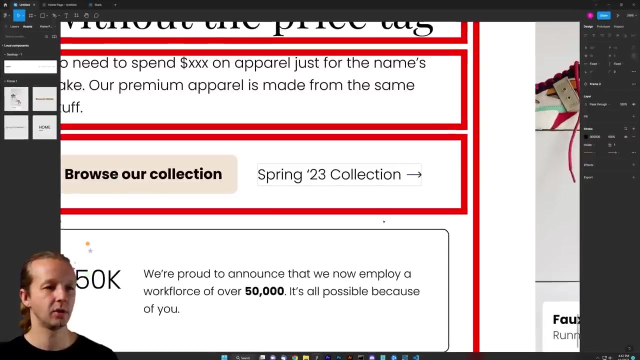 then we're gonna put in spring semicolon 23 collection. so that's our first element. now our next element needs to be that little arrow. so in that case we have a couple options. we have to go back, we zoom up control, screw will, if you will. 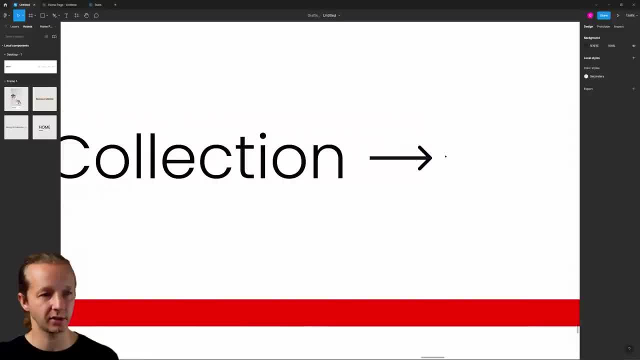 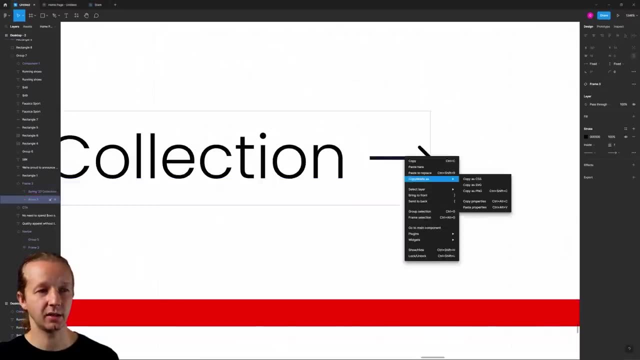 and we need to make sure we're selecting this button or this arrow, to make sure you can hit control, left click to select it and you'll know you've selected it if you come down here to your layers tab and then this is highlighted right here: arrow 1, we right click it. 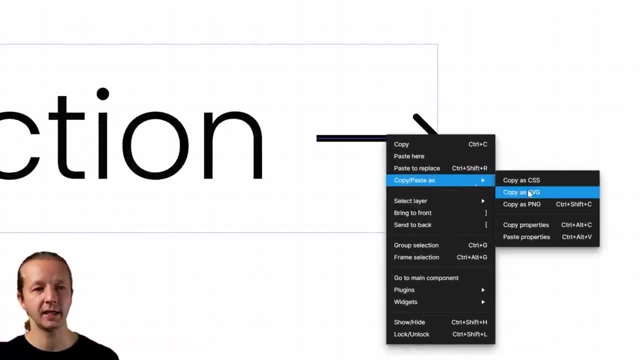 let me zoom up and we choose copy and paste as svg, because this is a svg element. it's scalable vector graphic. anything created inside figma, like with design illustrations, will typically be svg, not png that's rastered in bitmap. you don't want that and not css svg? okay, well, once you have that. 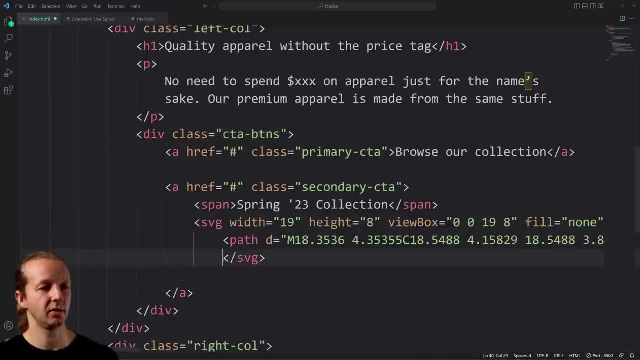 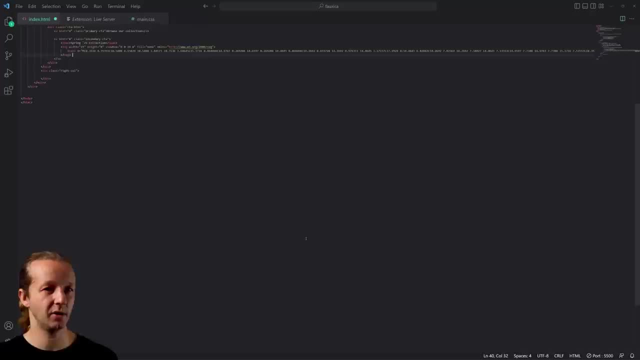 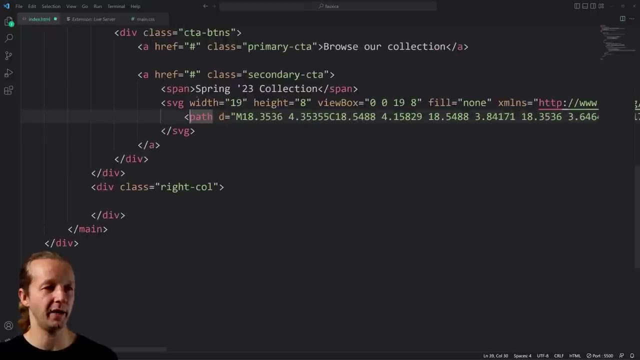 copied. we're going to go ahead and just paste it. so look all this this stuff, this crap. rather that it spit out, i it's long, and in order to create that, look at all this htm html up there. this is basically a mathematical equation that gives us that arrow. um and so, because it's math, 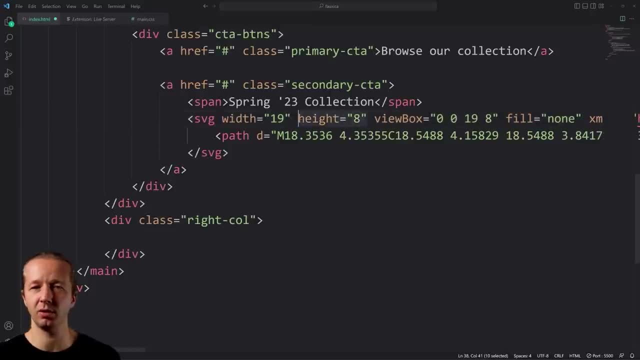 though that's why it's it's. it's not bitmap. it'll never get blurry or pixelated like a blurry ugly, like 2009 iphone photo or something like that. there's a couple attributes in the svg element that i want to get rid of, and that is the width and height attribute, so i'm just going to left click select both of those. 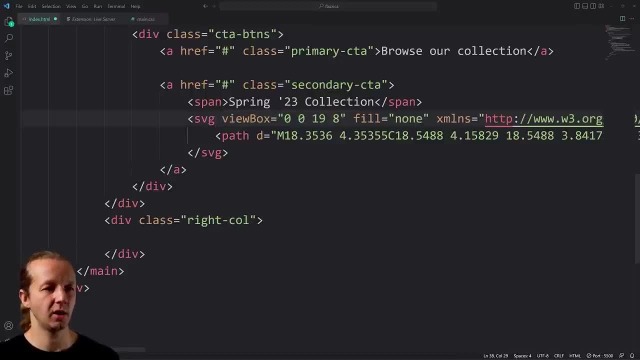 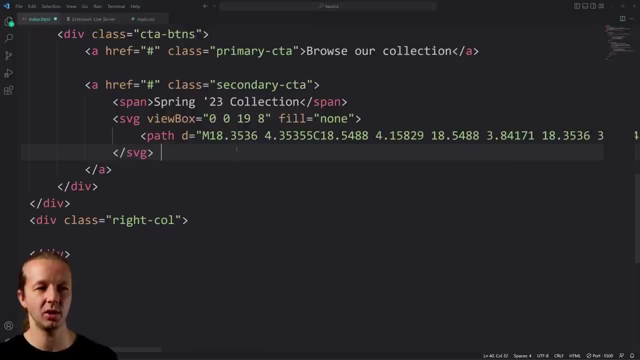 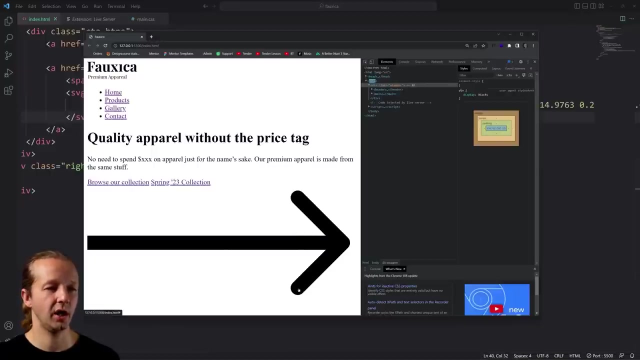 hit delete or backspace. rather, we're going to leave view box and, but we're going to get rid of our xm, xml and s. some of these are just unnecessary. we don't need them now. let's save control s and go back, and there's our huge arrow button. we don't worry about it being this huge because we haven't. 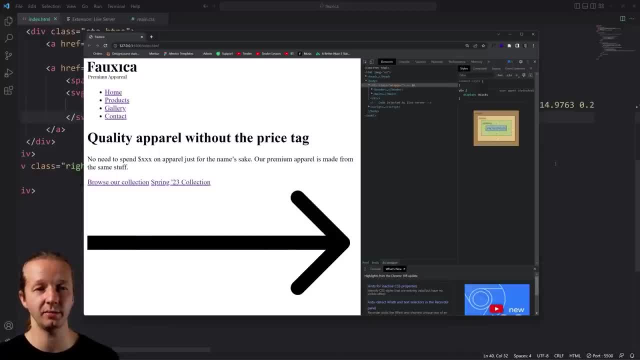 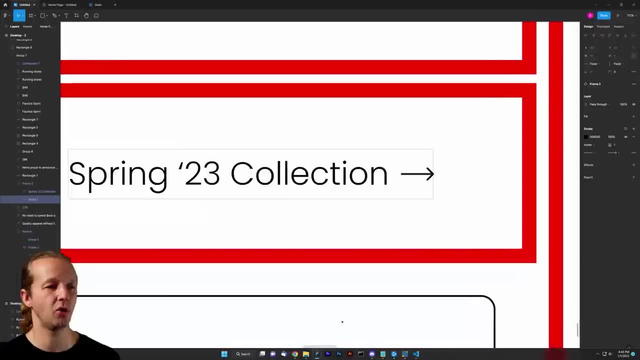 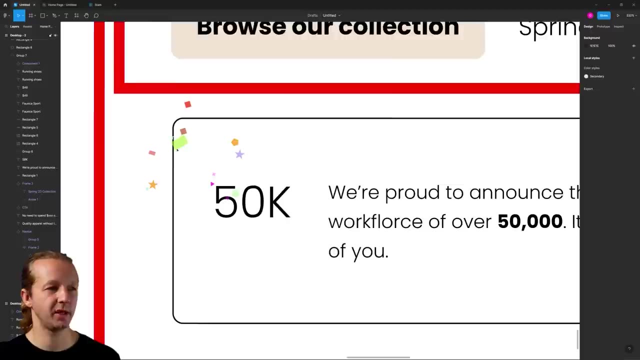 got to the css. we're going to fix that all up when that point in time comes, like ahead of time. okay, going back here. that's it for our cta section. so, going back to the next element, we have this, and this one might trick you up at first, because look at this, what is this? 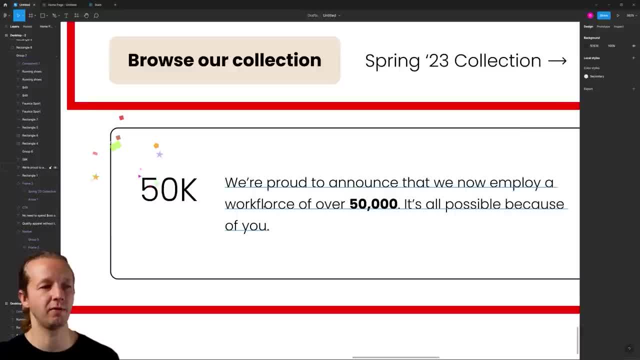 confetti stuff. well, that's because this is like we're proud to announce that we employ our. a workforce should probably fix that. there we go of over 50 000. it's all possible because of you: 50k. that's why i decided to put this little ad for for pay low. until. welcome commenting guys. thank you so much for watching this. we honestly are having a great time coming up. i'm still going to n一 in for more websites will give you a link in the description if you would like to see how i draw your business and some other things about video too, these up�. 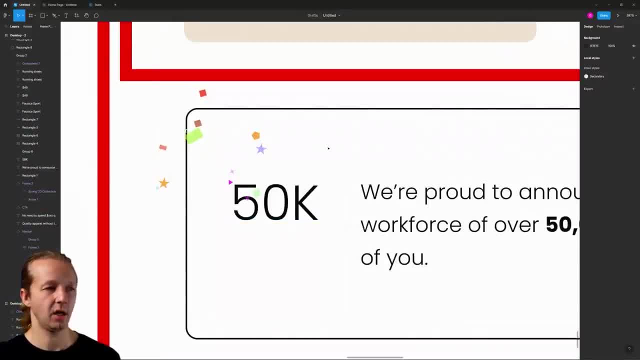 out in the description below this video as well. so if you're interested in making a discussion with me, it's a very asset. set of like confetti graphics over here. ignore that for now. we'll get to that, but we're gonna ignore that, just pretend it doesn't exist. it's kind of on. 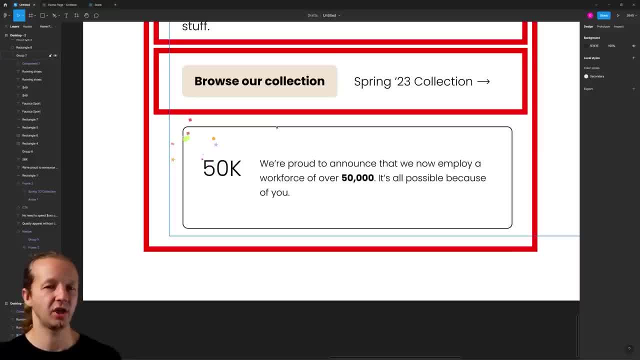 top of stuff. don't worry about accounting for that. I'll show you how to do that in CSS. so really I only want you to focus on just get this out of the picture, this area right here. so we have a div element we could see clearly, because it has that black border and it's wrapping around both of these. 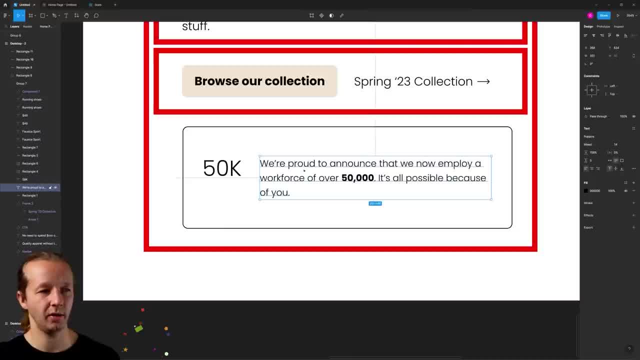 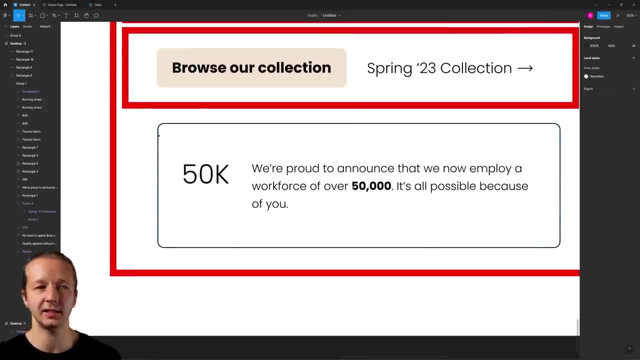 columns, this 50k and this type right here. so let's create the element that will do that for us. almost this element right here is actually visually depicted in our design and it kind of mimics what's happening up here, because we're giving that HTML element a border of one pixel solid in CSS. you'll see in a 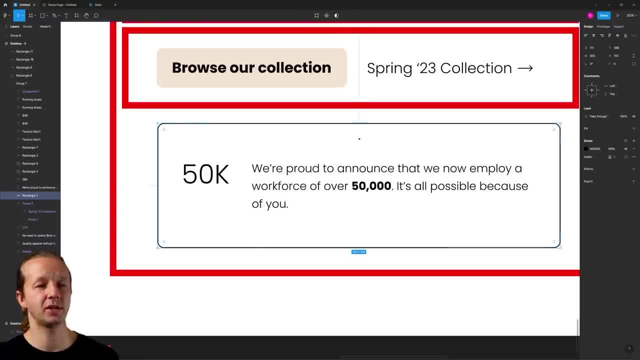 little bit, but it's still necessary. even if we didn't want to visualize this, and maybe we just hid this, it would still be necessary to have an element that wraps around that, and that's what we're going to do here. so we're going to go ahead and 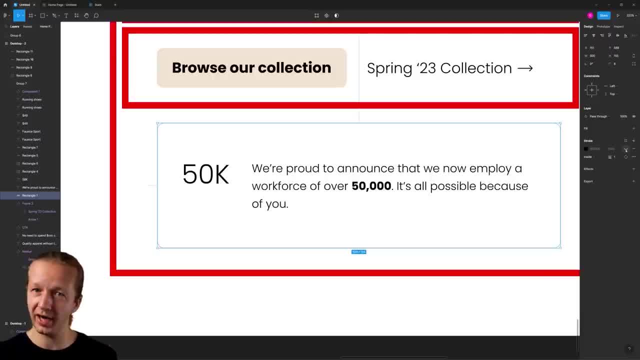 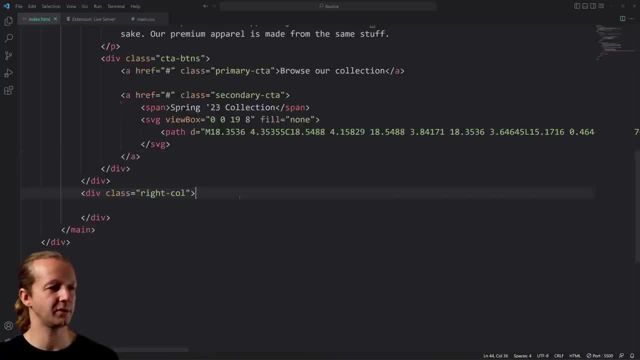 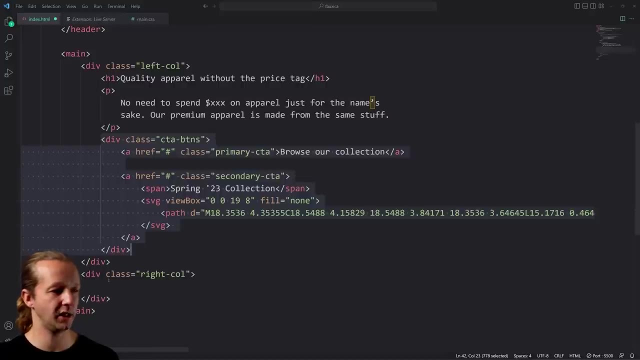 do that. let's go ahead. let's here stop saying: let's go ahead. so much, Gary, and underneath, but inside, oh no, no, sorry, let's get out of here. so we have our CTA buttons section. that ends right there. after this closing div tag, we want to. 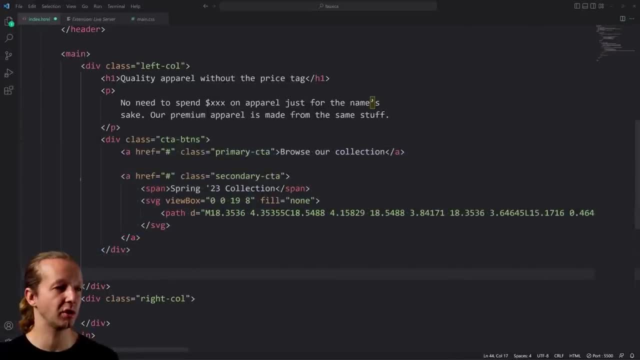 come right after that, right underneath it, but we still want to make sure that remaining we're remaining inside of our left call and this, if you follow it all the way down, we'll point to this right here. so we're still in it. if we start typing our next code right here, this is: 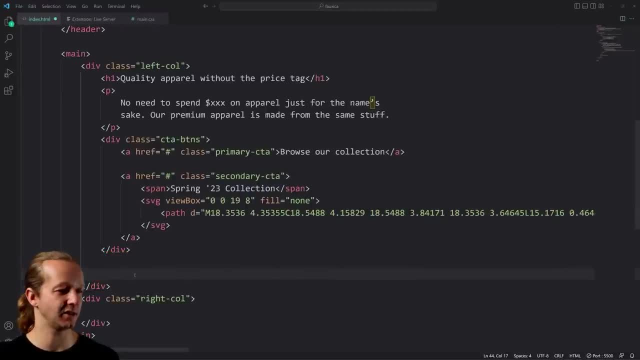 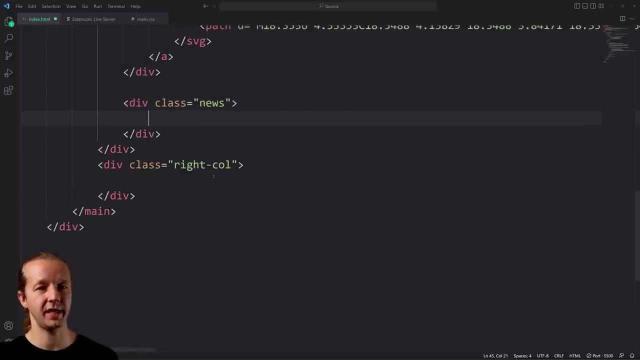 underneath the what do you call? the CTA button section. so for that section we're just going to call that news and we're gonna wrap that in a div class. so period news enter and inside of it gonna have two columns, 50k and then a paragraph. so for that we're just going to use paragraph. 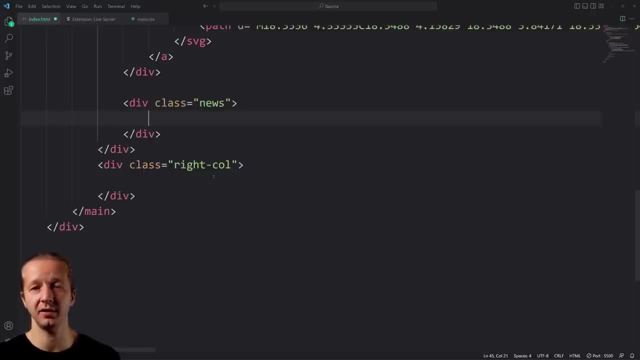 classes for both of them. it doesn't necessarily even have to be a paragraph. even though it says 50k, that's not a paragraph. you could still use the p element. so p dot employees. so it's going to be a paragraph. html element with the p tag with the class attached to it, called employees. hit enter. 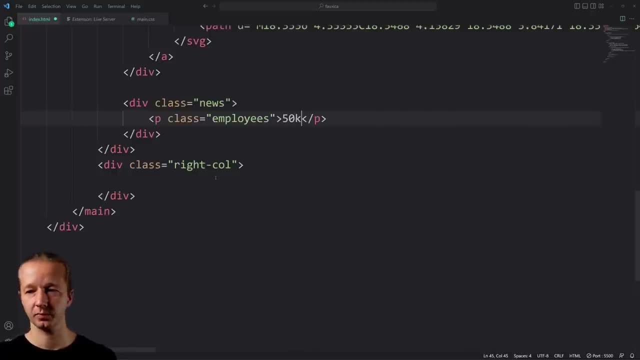 and then just put in 50k. i'm going to capitalize that k. there we go, and then right here, p period details. so these are the details about you know this little news thing. so i'm just going to go ahead and copy and paste what goes inside of here off screen, all right? so 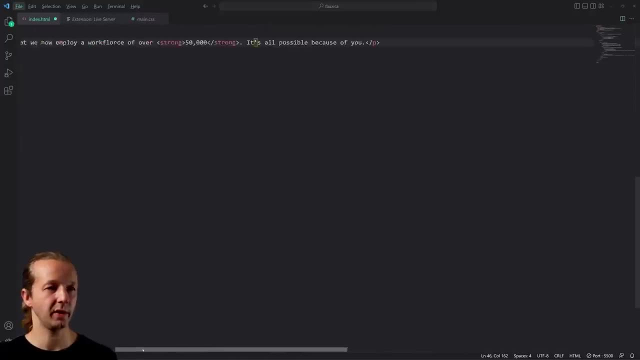 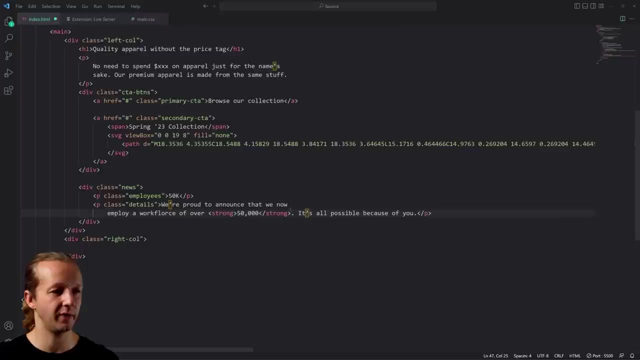 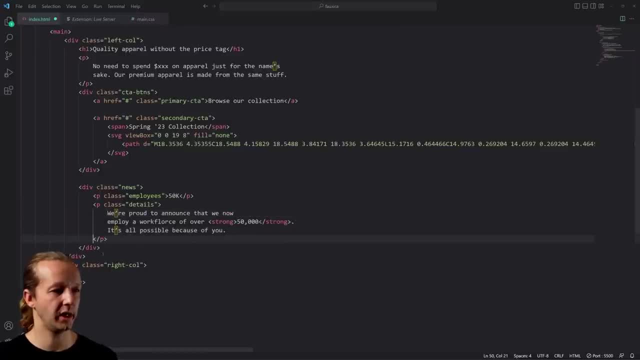 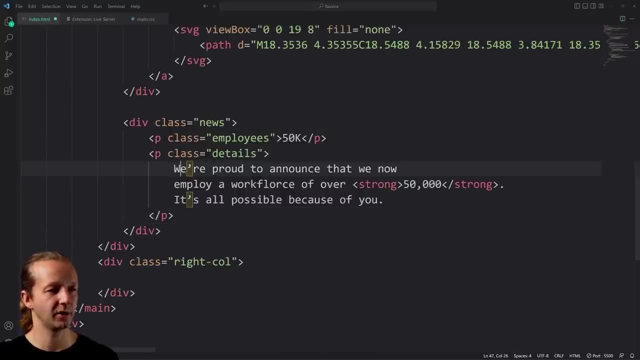 there we go. so now, if i zoom up, try to get your structured so that it looks like this- don't worry that these are outlined right here. um, where it says: we're proud to announce that we now have a a workforce force of over 50 000. notice it has these strong tags: around 50 000. that's. 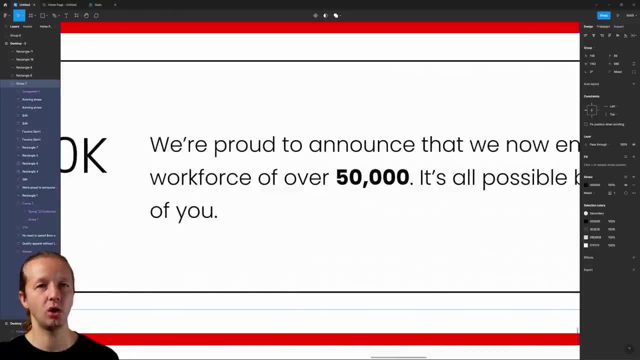 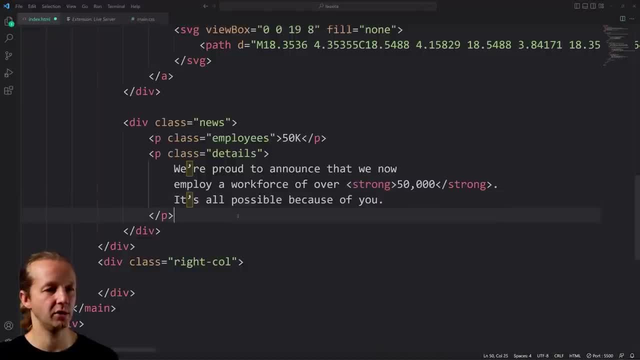 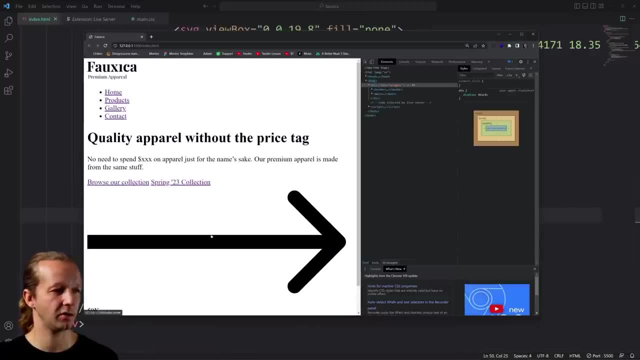 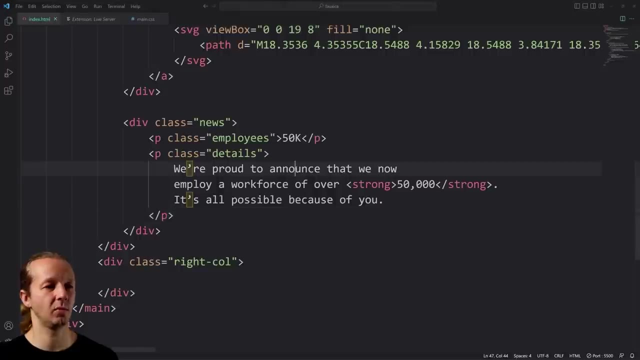 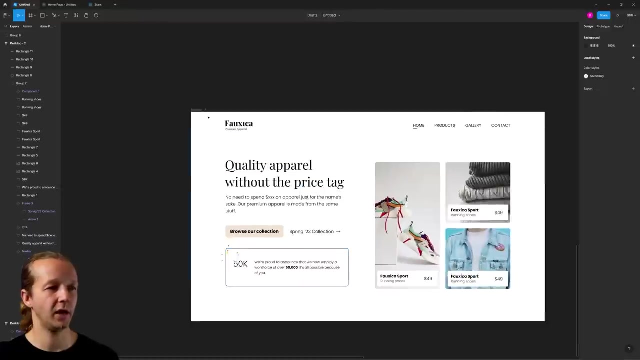 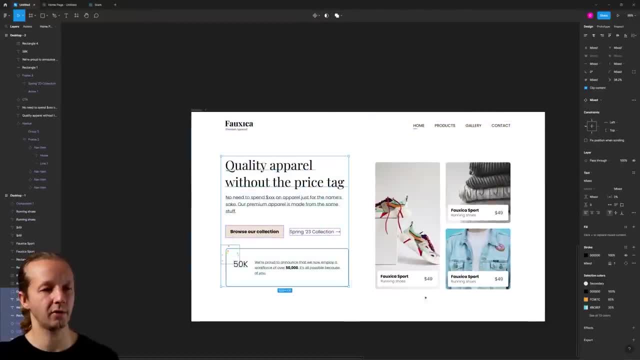 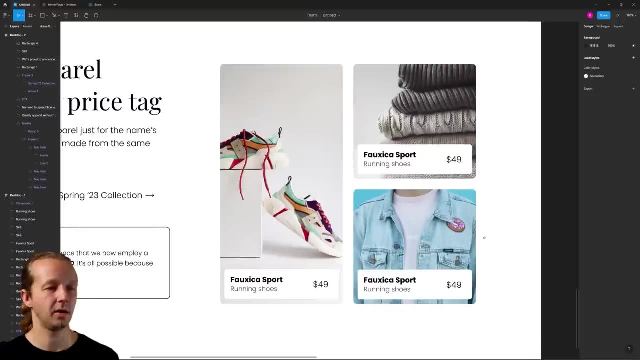 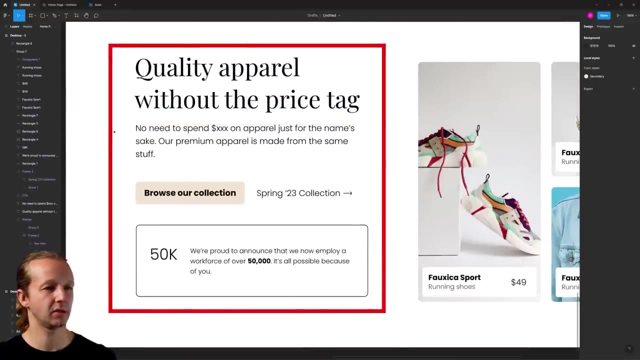 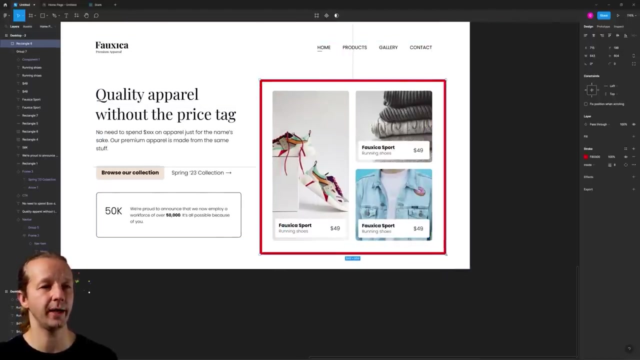 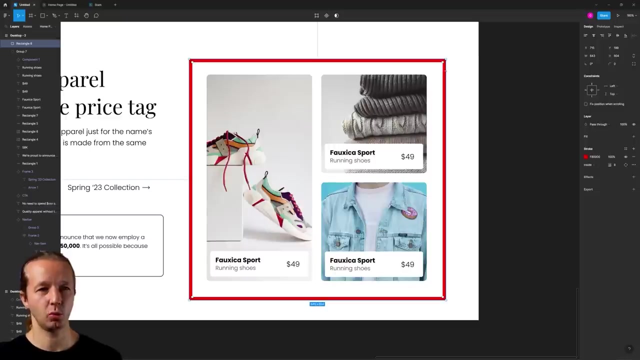 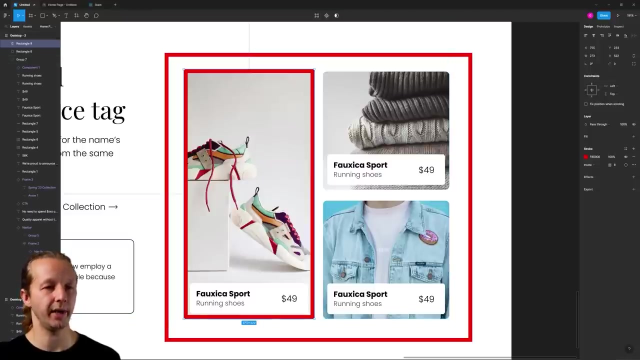 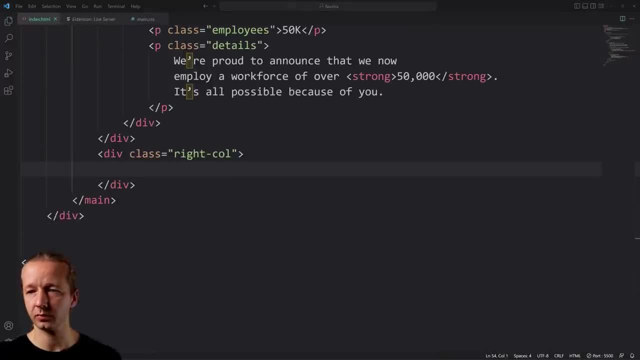 alright. so inside of right call we're gonna go ahead and specify a class called card and again we don't have to put like divcard, because inherently Emmett knows if we don't put the actual HTML element in front of or before the period, it's gonna be a div element. so we're gonna say: card imitator admin. 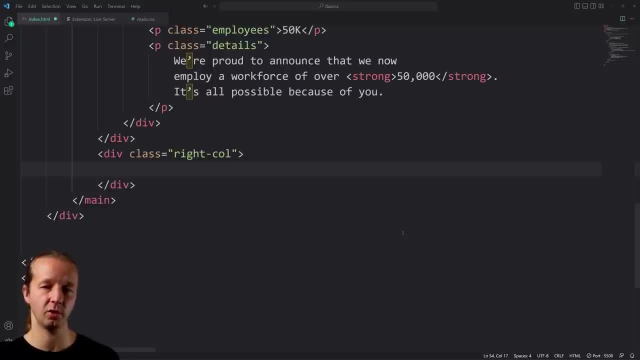 imitator. admin is the ste forskling. it's going to be a div element. So we're going to say card and we can chain multiple classes together in Emmett like this. So we put a period after that and this is going to be card one. 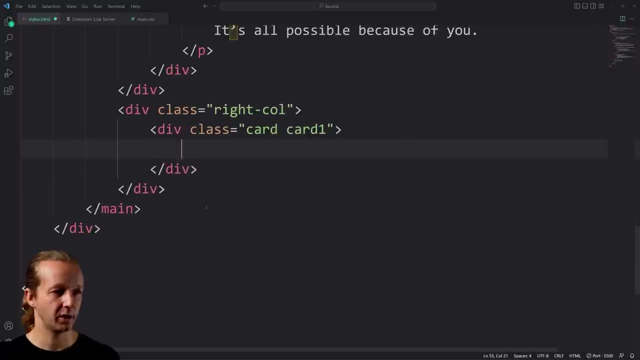 hit enter And this is what your markup should look like. So, yes, you can have multiple classes inside of the class attribute, And the reason we're going to do this is because each of those three cards will share the same class of card, but we have to have a way to create the distinction. 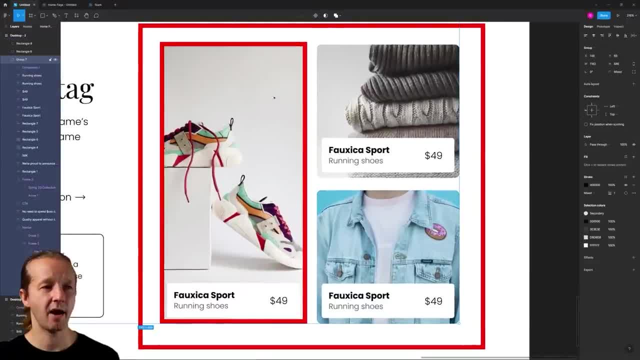 between each of the three because they have different background images. Now there is a caveat to that: using CSS, pseudo selectors nth of type. That's more intermediate stuff. We're not going to worry about that, We're just going to give them explicit class names that are: 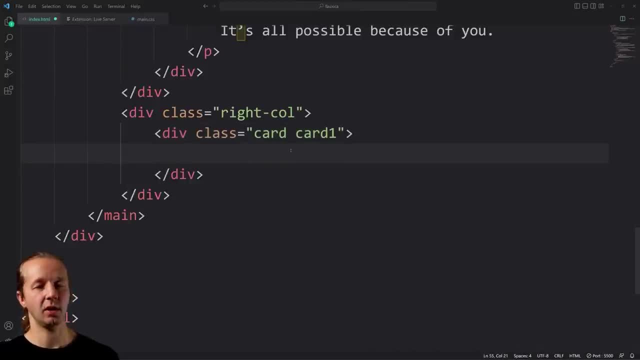 different from each other. So inside of here, our card, card one, we're going to have card two, card three, card four. card five. card six. card seven. card eight. card nine, card 10, card 11, card 12, card 13,, card 14,, card 15, card 16,, card 17,, card 18,, card 19,. card 20,. card 21,. card 22,. card 23,. card 24,. card 25,. card 26,. card 27,. card 28,. card 29,. card 30,. card 30,. card 31,. card 32,. card 32,. card 33,. card 34,. card 35,. card 36,. card 37,. 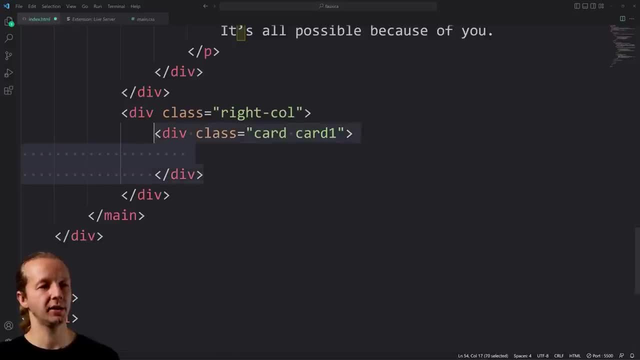 card 37, card 38, card 38, card 39, card 40, card 41, card 42, card 41, card 42, card 42,. another element Now. first I should say this right here: this div element in and of itself. 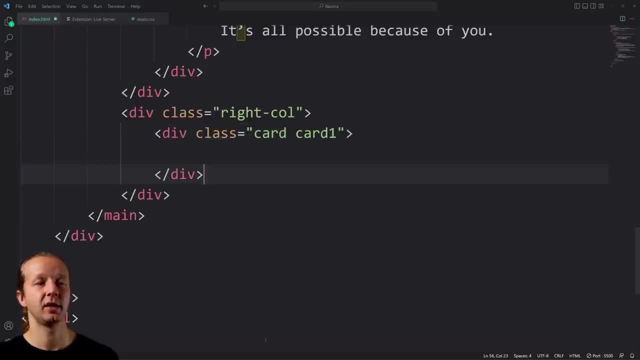 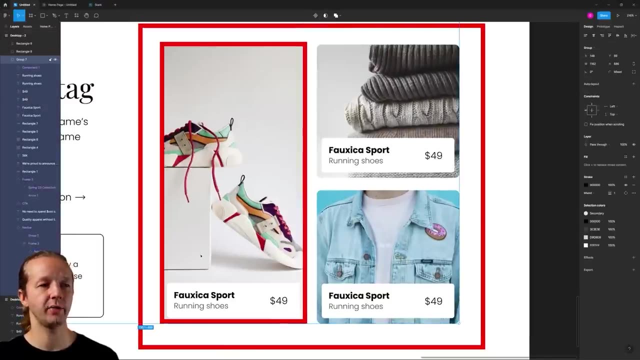 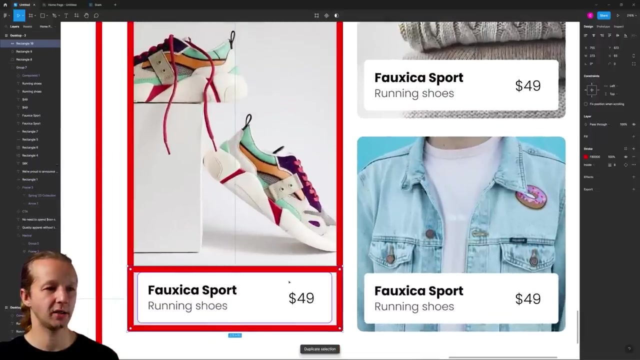 that is what is going to contain the whole picture, the photograph, rather, So we can use CSS to target that card one and give it a background image of this. So the next thing that we have to write then- let me duplicate this- is this white, these white little boxes. All right, 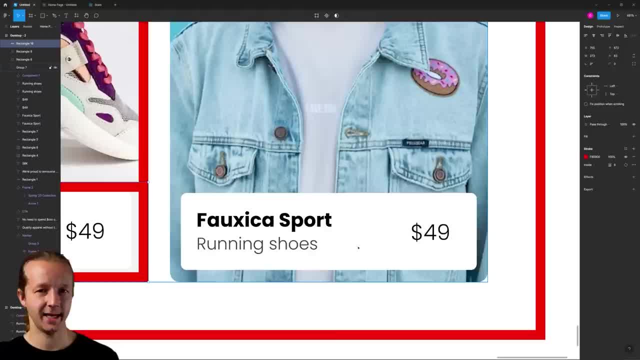 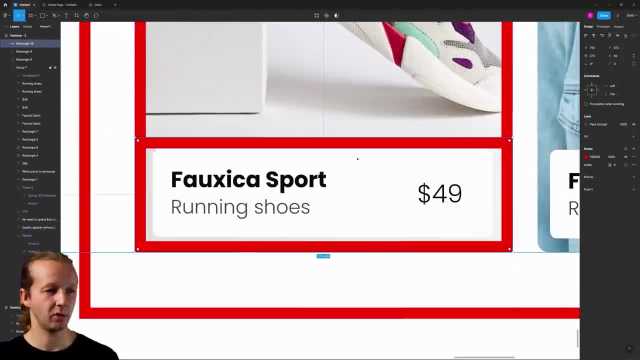 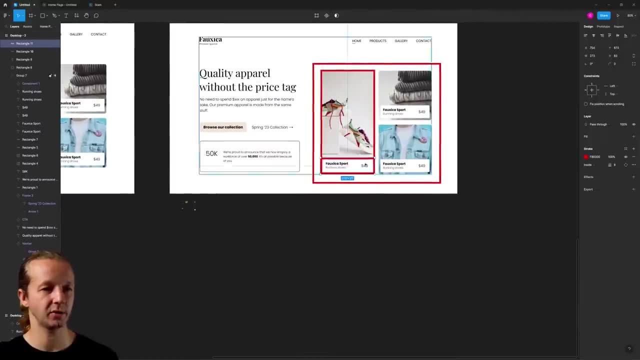 And then you have to ask yourself: all right, do we see any columns here? I do. There is a column, Let's go refer back over here. Uh-oh, I hit control D and something happened. Oh, it moved it down there for some reason. All right, So we have a column right here. 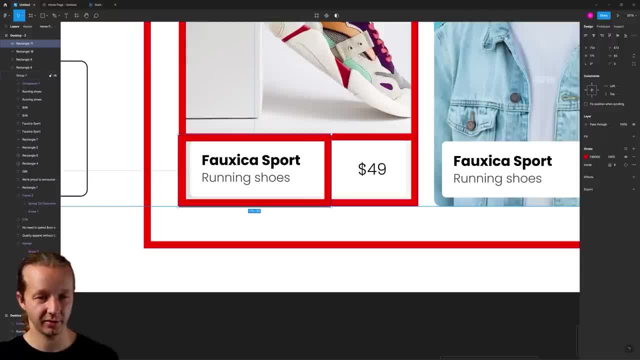 with this type and a column right here. So it's very important to remember this. the structure here: Okay. So what we're going to do is we're going to go ahead and we're going to go ahead and we're going to. we're going to go ahead and we're going to go ahead and we're going to go ahead and we're going to. 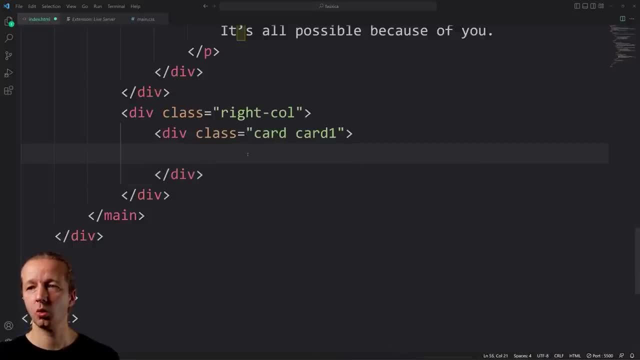 do first in our card is we're going to need to wrap everything around that white container with a div element called card details. Okay, Now, inside of card details, we need to have two elements because, remember, it's two columns. We have the two pieces of type sitting on top. 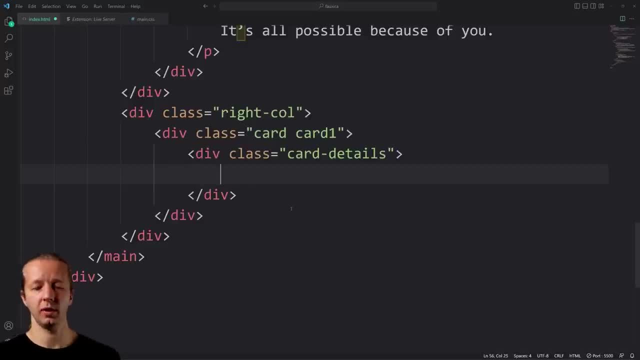 of each other, but then off to the right is a price. So I'm just going to put in- and this is something you can completely do- just a div element with no class. You don't have to put classes or IDs or any attributes in them if you don't want to. So for me I don't need to in order to. 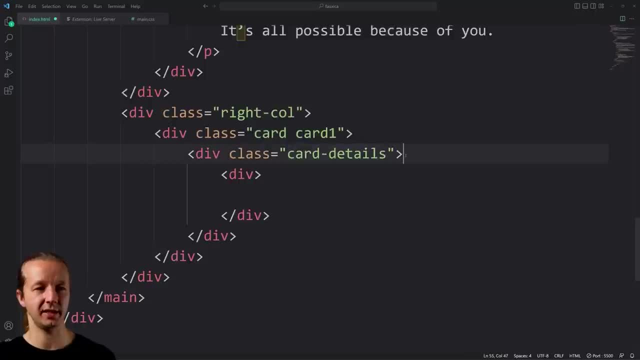 structure this stuff. we can just reference card details and then say div and CSS, So we could be like card details, div. That's completely acceptable. There's only going to be one div element in there anyway. Okay. So now we're going to have a clickable link and I'm targeting 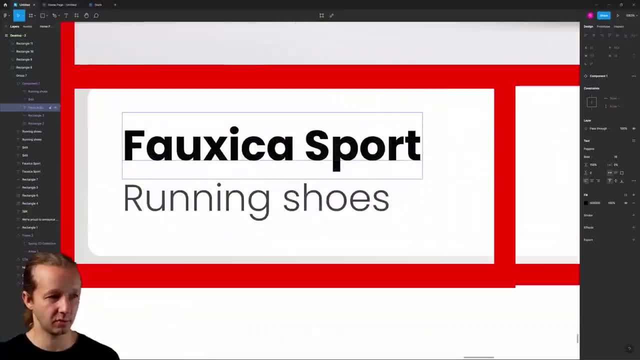 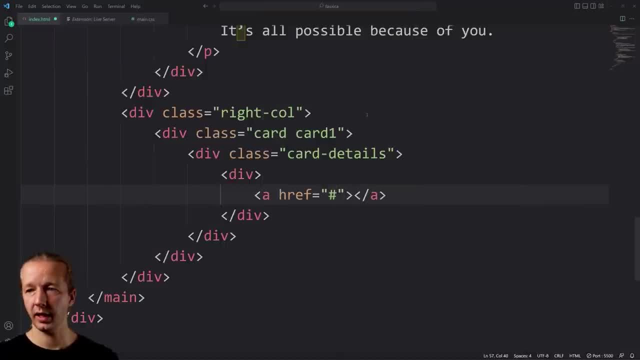 this Foxica sports thing right here, this title, So we're going to assume that's clickable. So we put in an A element hash sign here, and we can give this a class of product title. Now, thinking about this, though, if this is the only A element inside, 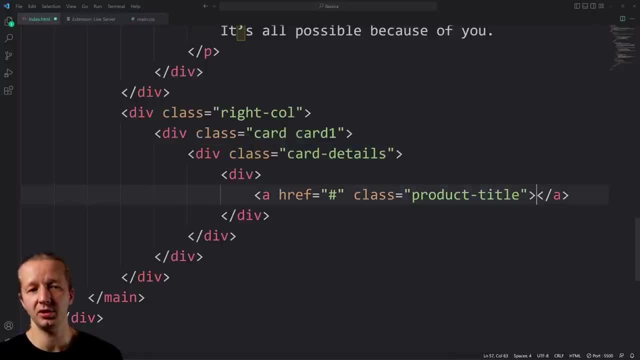 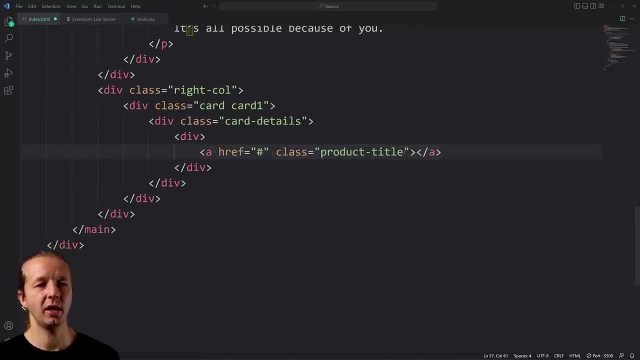 of card details. we don't even have to give it a class. I'm choosing to do it, but you don't have to. Okay, And one thing that does help, though, in the case of like text, having a class name, when. 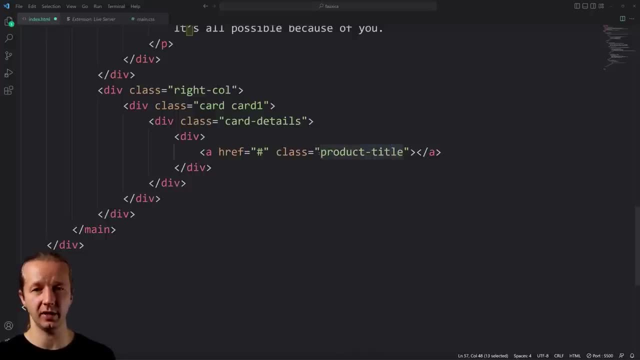 you're reading. when it comes to readability for your CSS, if another developer's working on it, or even if you're doing a class name, you're going to have to give it a class name. So if you're yourself in the future and you forget, you'll know that that particular rule set in CSS is. 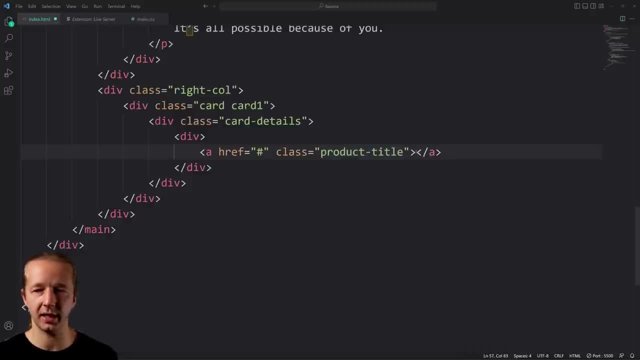 associated with the product title because that's in the name. So hopefully that makes sense. Yes, Okay, So now let's go ahead and put in Foxica, let's see sport, And then underneath it we have a little paragraph: running shoes. It's kind of like a little tag or category or 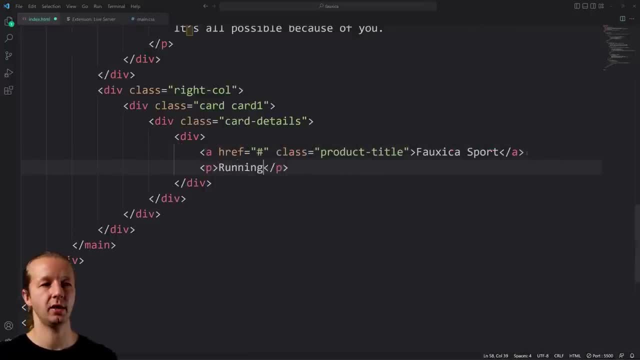 something like that. So P, and we're going to say running shoes, All right. After that we have the price, which is off to the right in the second column. So we'll use a paragraph, a class of product, hyphen, price, and we'll say 49, something like that And that. 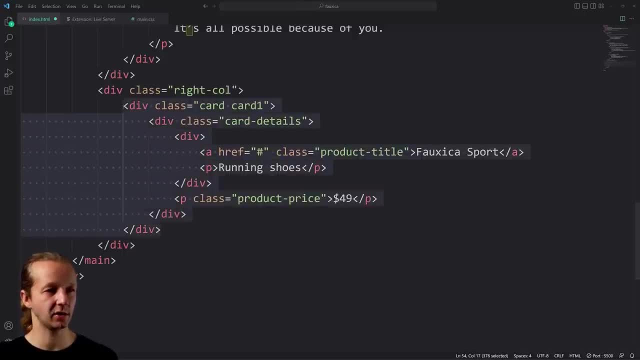 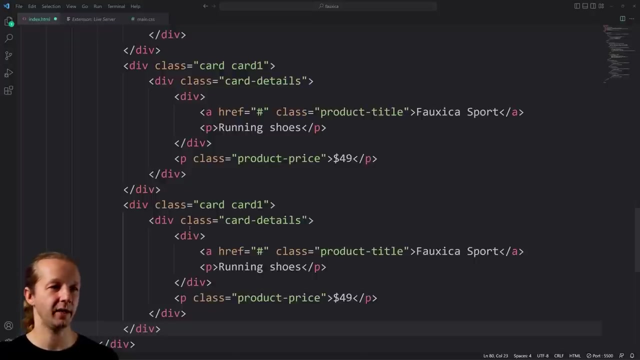 is it? So now what we do is we take left click and select that whole card card one, all the way to the closing tag associated with that card card. one element: We copy it, come outside of it, paste it, hit, enter, paste it. So now we have three. So let's see: one says card one, This one. 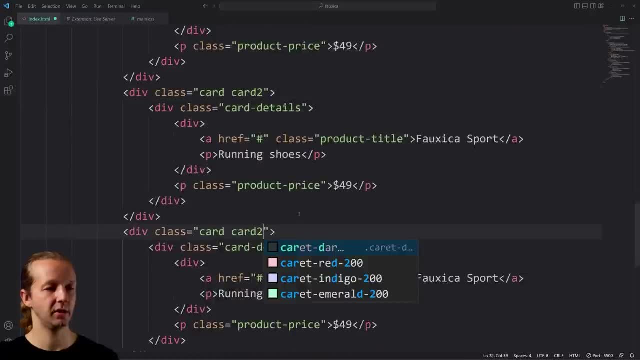 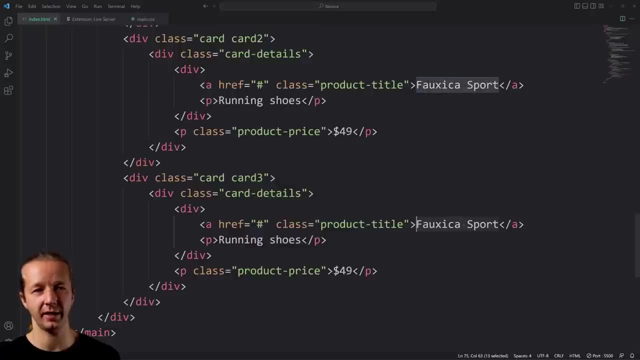 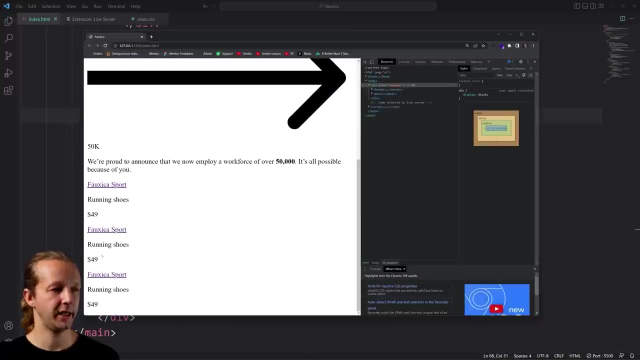 needs to change to card two. This one needs to change to card three. Hit save And that is it. Now, of course, you can give it. you know fake, other fake titles or whatever, but I'm just leaving them. So now, if we look, we can see. this is what it looks like. Foxica sport running shoes. 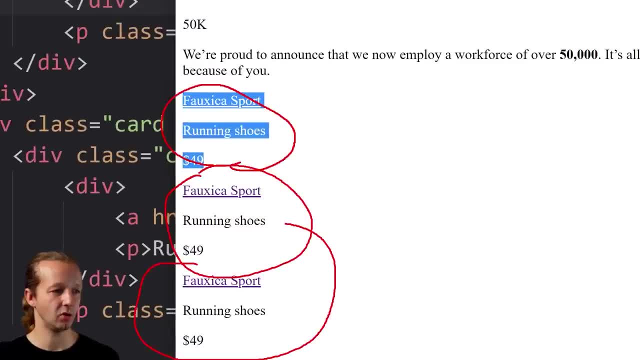 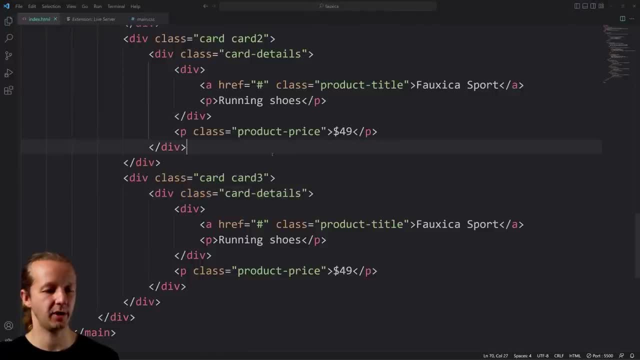 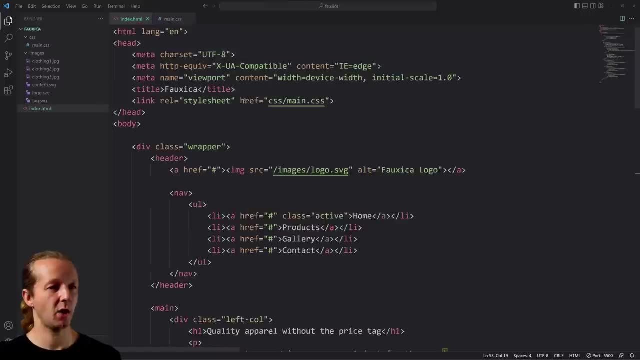 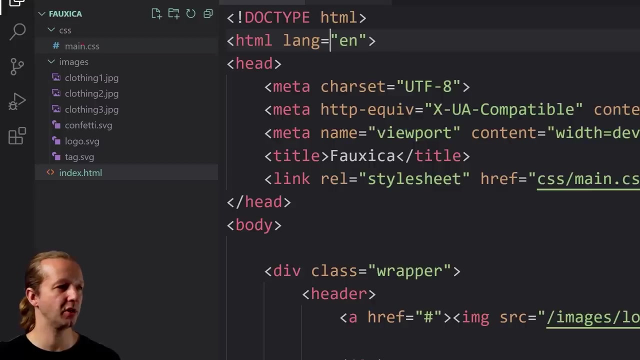 here's our first one, second and third- And guess what That is about it? for the HTML. So now I get our sidebar back up here. Let's close this out. We are now ready to proceed to the CSS section. Okay, So let's go to our CSS. So come over here. You can double click on this, It's. 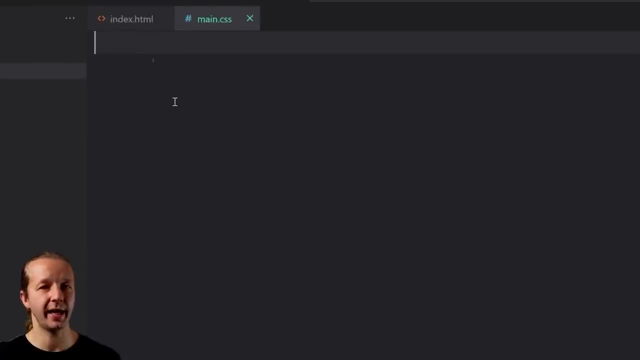 up here. So the very first element that I add. uh, typically in every project, it's a rule set rather, Um, I'm going to target the HTML element itself, which is like the element that holds everything, And I'm going to give it a font size of 62.5%. And what the heck does that even mean? 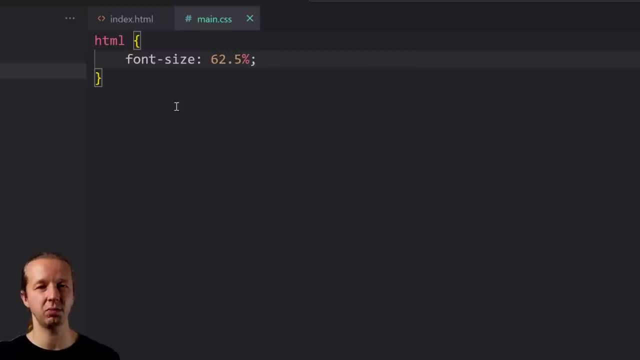 All right, This is kind of. it's a little bit difficult to explain at first, but basically its purpose is to make conversions from your proto, your Figma prototype, easier when you try to translate value certain values to CSS. All right, So let's see if I can do this easily. Um, and don't think it's too scary, It's one of. 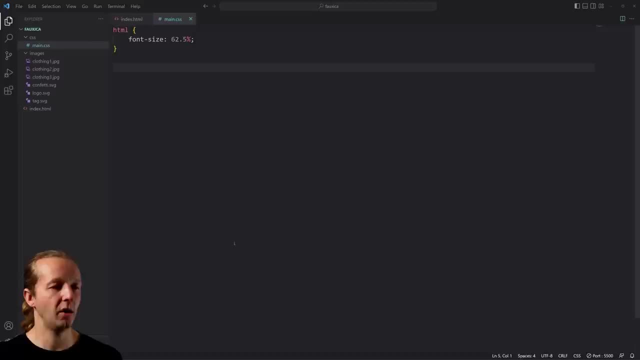 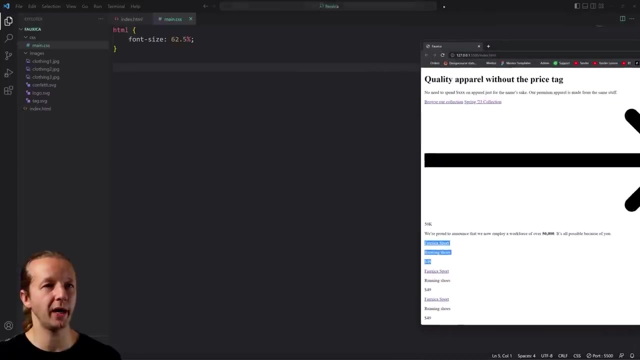 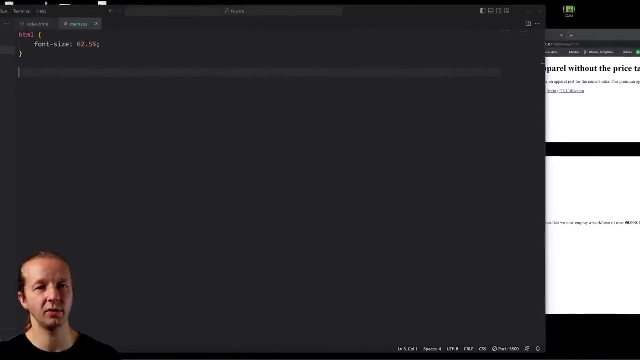 those set it and forget it things. So if I hit save, we're going to notice that And in fact let me just show you by dragging this off to the side So that we can see a little bit of this. off to the side, this uh browser, even though it's hiding. 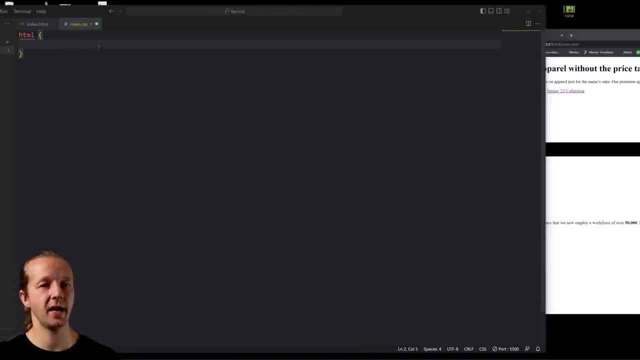 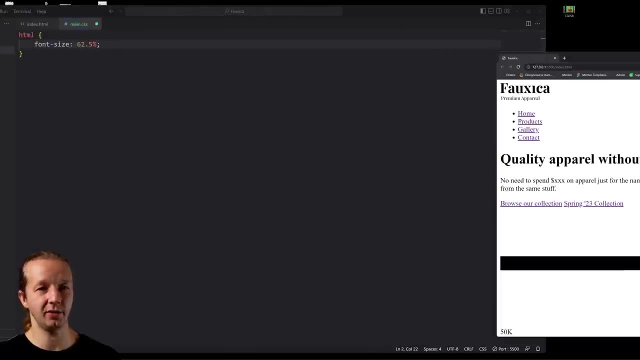 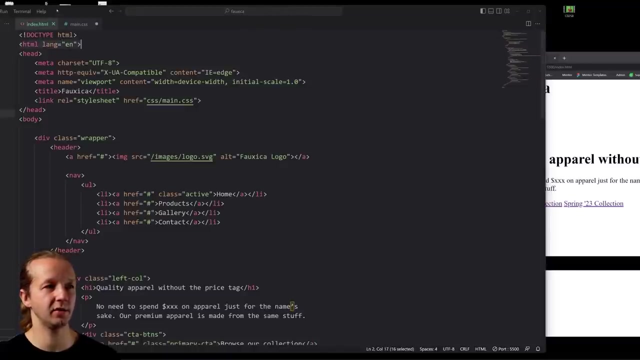 it If I take this off and just delete that and hit save. the type just got way bigger. Now I'm scaling the font size down, all the font size everywhere, because HTML, if you look over here, contains everything. So it's going to take all the type that's found in here and it's going to 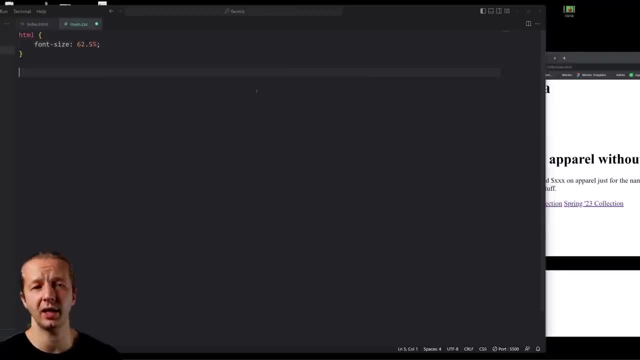 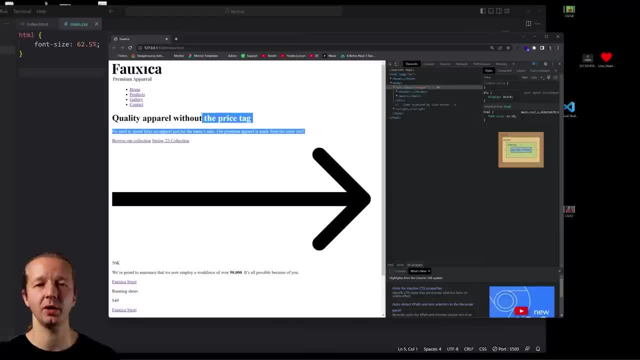 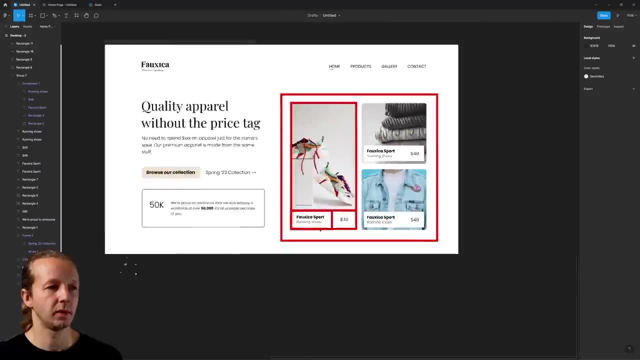 What is the purpose in doing that? Well, it's not because I want smaller type here, It's because it's going to make my conversion life. If that's a thing, it's not. I just made it a thing a lot easier. So here's what I mean. Um, if I go to Figma and I look at the font size, for instance, 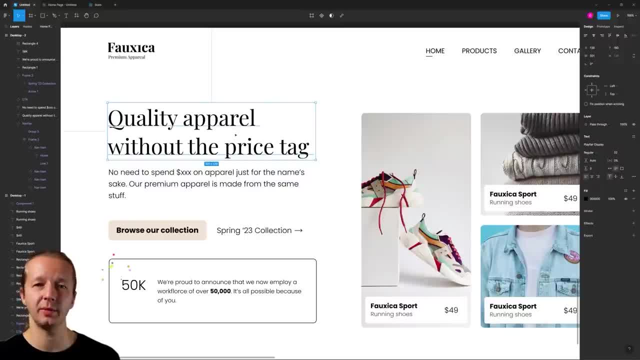 of this headline and this is in the H1 element in our HTML and the font size, if I select. this is right here. it's going to scale it down to 62.5% By default. it's going to scale it down to. 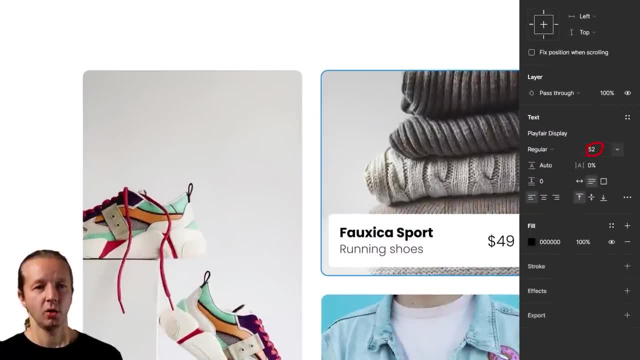 here It's 52.. All right, Well, I can't just put font size 52 pixels. Uh, when it comes to font sizing, I, along with certain things like your margins or your white space between elements, and you're trying to construct that in CSS, you don't? you pretty much never for the most part. 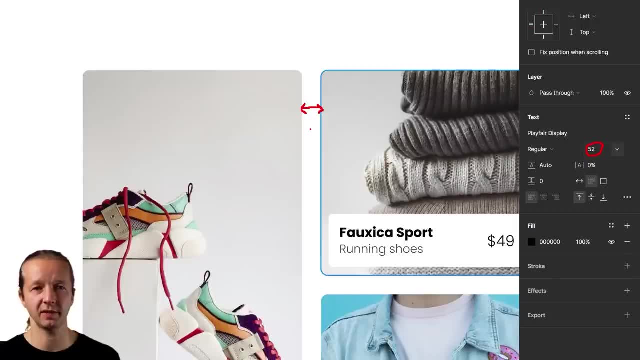 there's exceptions. I want to use pixel values or PX values. You want to translate those into units that are relative, As it's called, uh and and, and. in order to do that, you have to apply a conversion to it. 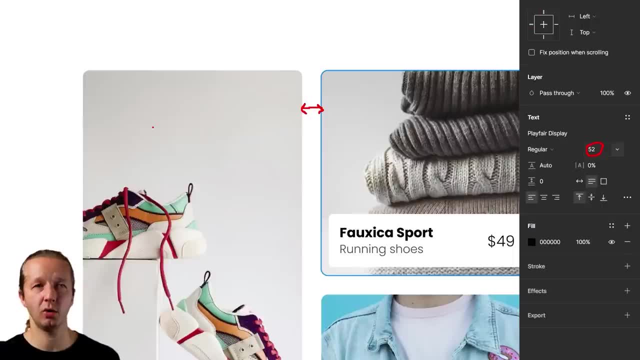 And so what that conversion does, making all font sizes 62.5%, means that we only have to rely on decimal places, our decimal point. So instead of 52 pixels we can put something like 5.2 rem units. So we just move the decimal place over one notch and that will give us 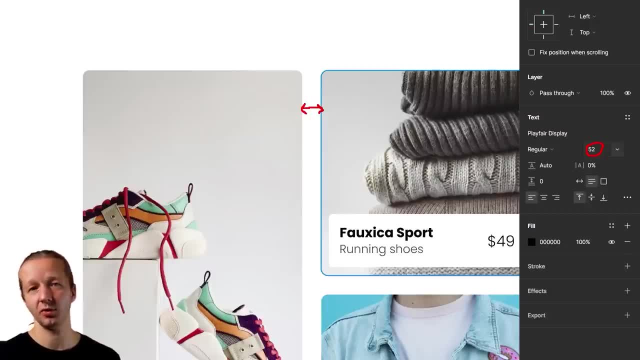 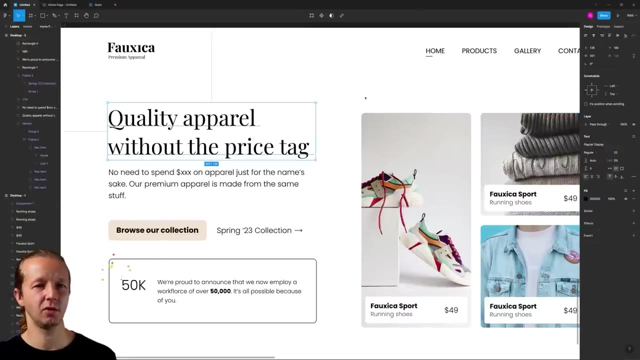 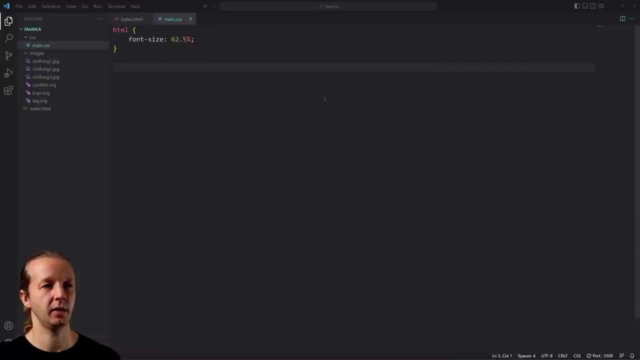 we're going to copy that by using the and the thing that we're going to start with now, after you know this very convoluted, like what the heck are you thinking? All right, So let's go back and we're going to start with the text. 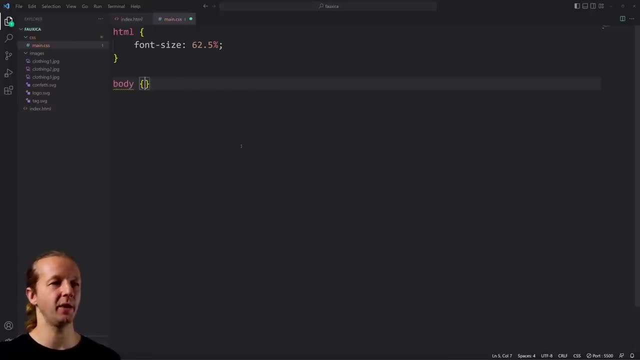 So let's go back and we're going to start with the text. And so we're going to start with the text situation. we're going to specify the body element. now, if you remember, the body element is really the element that has pretty much all of our HTML markup. 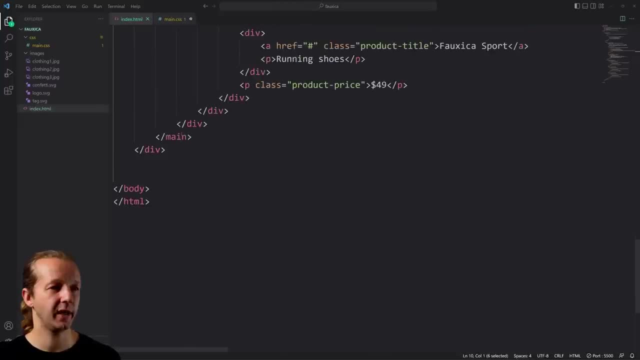 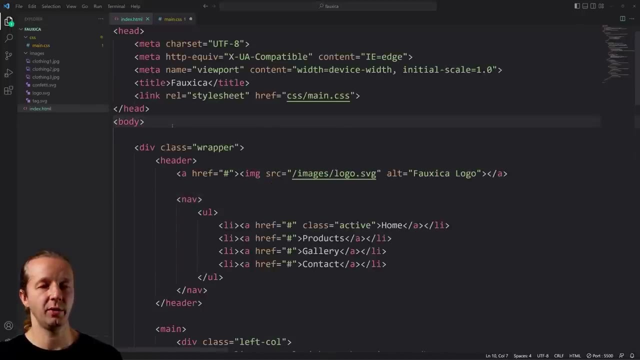 inside. so here's the opening, the closing tags, all the way down here, right there, the body element. so now, what does the body meant body element do? what is it responsible for? well, it's a responsible for a lot. like our website background color, ours is white and that's what it is by default, so we don't even have to. 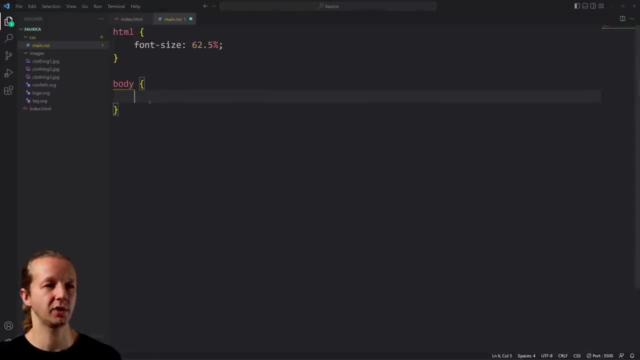 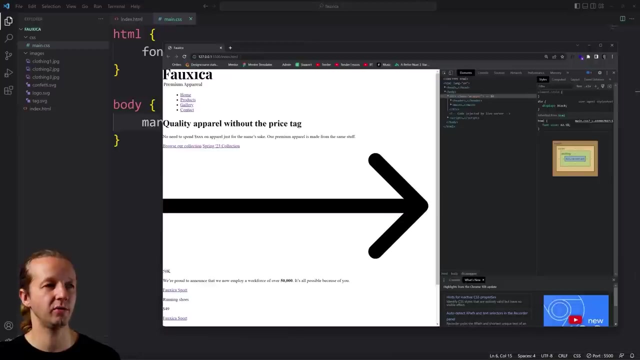 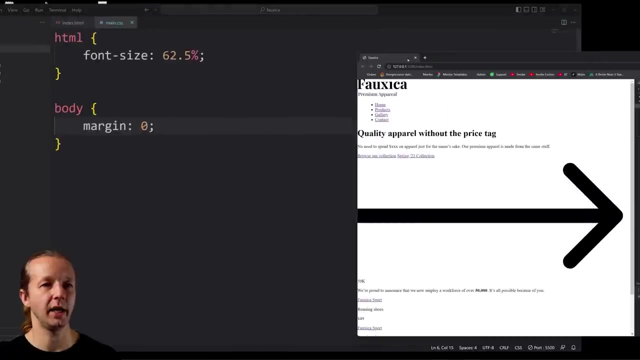 specify that, but there's still a few things that we want to do. first thing I'm going to do is change the margin to zero. all right, so by default, the browsers will give our design a little bit of margin around. so what I mean by that is, if I move this over and we take a look at the very edge, right there you. 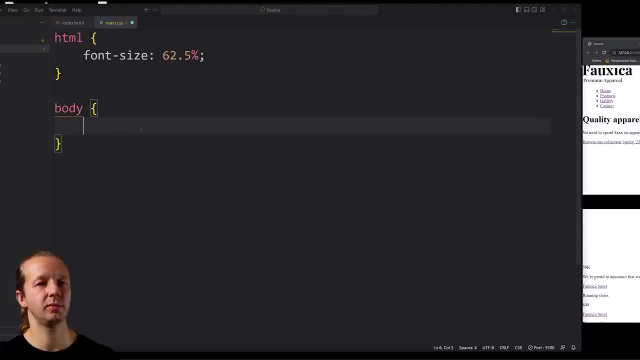 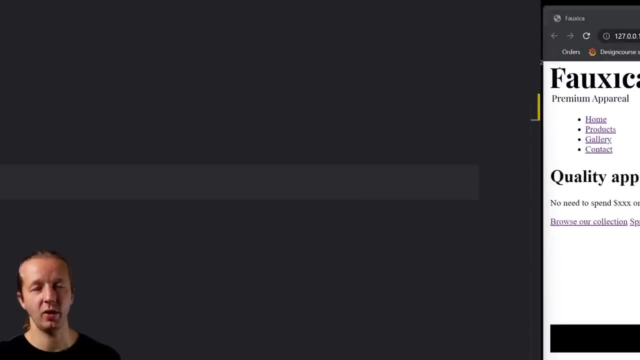 can see where it says foxy cut. if I remove margin, zero hit save- see how it moved over. so there's a little bit of margin. zero hit save see how it moved over. so there's a little bit of margin. and margin is a way for CSS in a browser to give you white space around things. 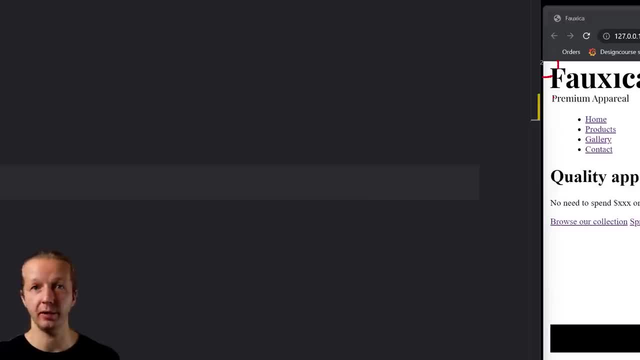 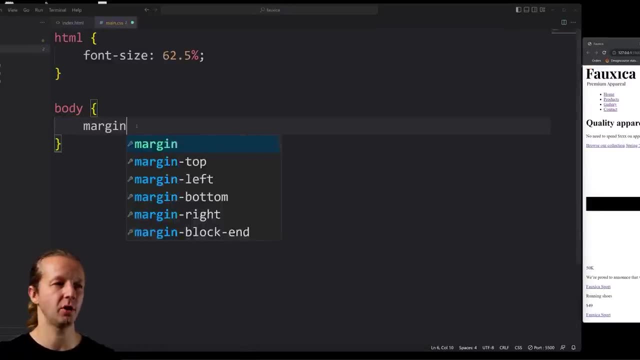 like on the top and the left and the right and bottom and all that good stuff. but I typically want to remove that, so I have control over that myself. so margin zero, all right. next up, after that, we're gonna have a font family now the font family we have actually in our design. we have two different fonts. we have this: 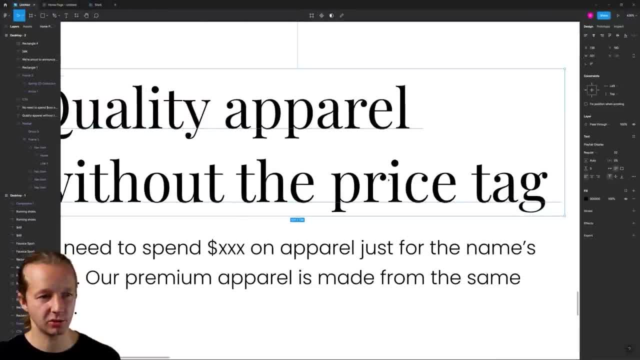 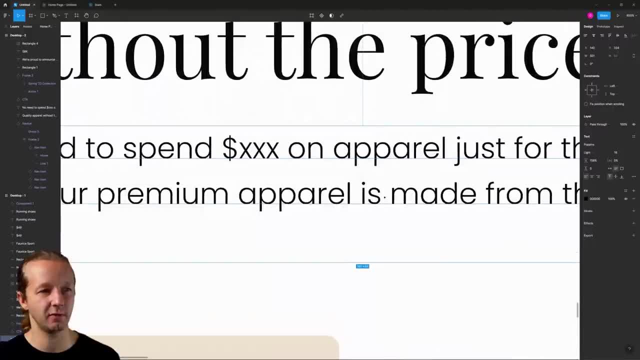 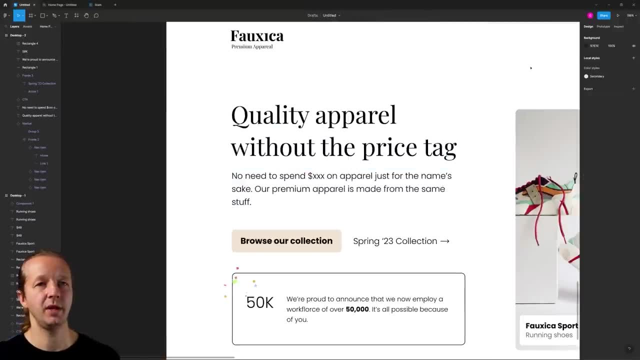 one. it's called play fair display. it's a nice elegant sort of serif font, as it's called. and then we also have like this one underneath called Poppins, and this is a sans serif font. it doesn't have those little crazy things hanging off the top of them like the letters and stuff. so this is a font pairing and we 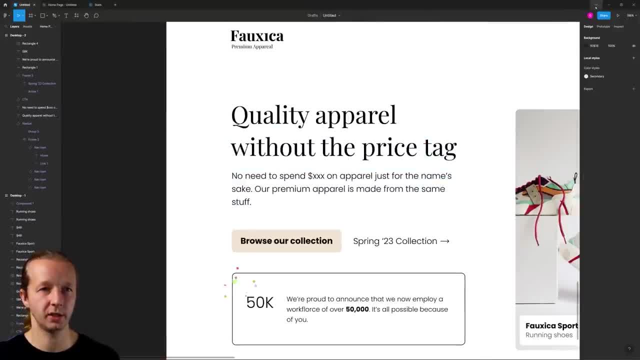 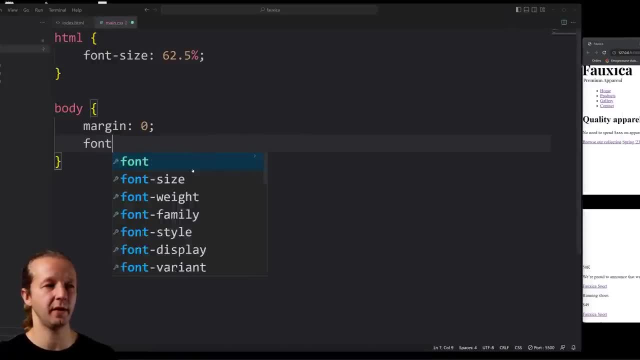 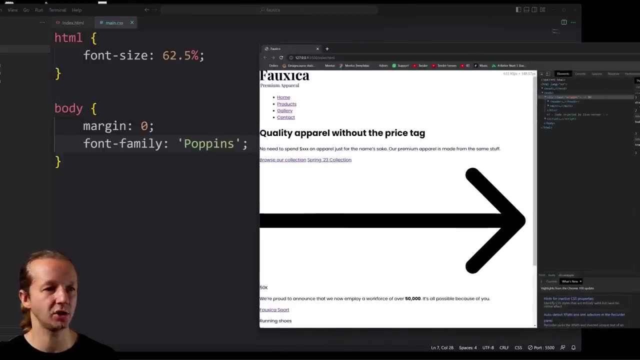 need to be able to include both of those fonts. so first let's specify the predominant font that's found throughout. most of it is the cleaner font called Poppins, so I'm just gonna do font family poppins. now, when I save that, a lot of our type is going to change to that font. 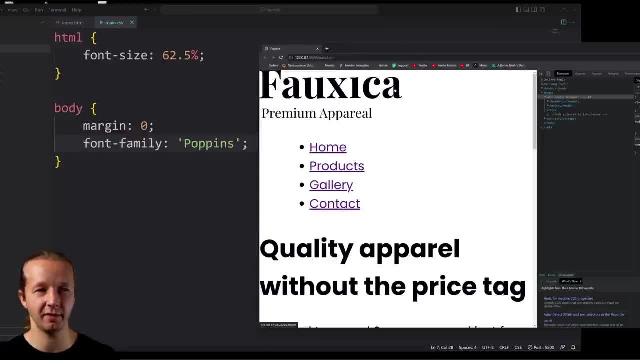 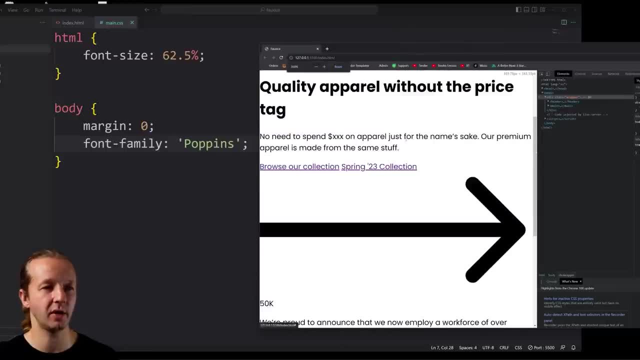 the. the logo is not because that's an SVG and that's not a font really it's. it's an. it's an actual graphic asset. but everything else here has changed to that Poppins. I font now the reason it showed up on my computers. I have it installed. 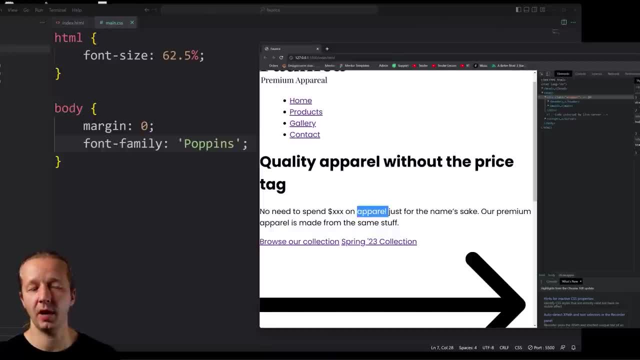 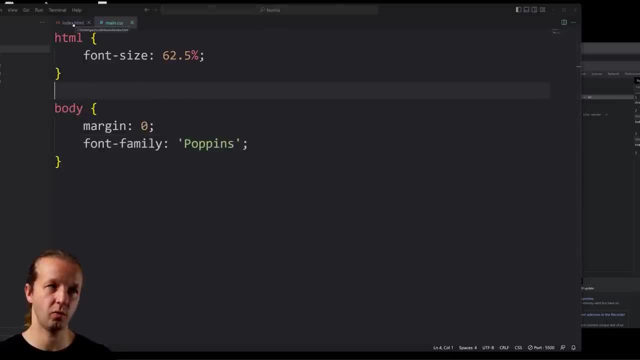 on my computer. many fonts that you use other people may not have, so you have to include the font in your project, in your design, in order for it. you know, for other people who don't have it inherently installed on their phones or their their computers, for then their browser to 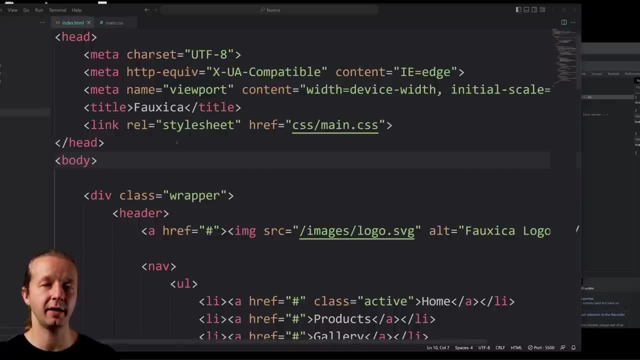 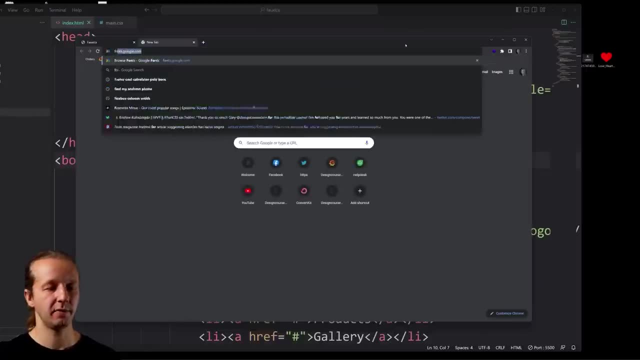 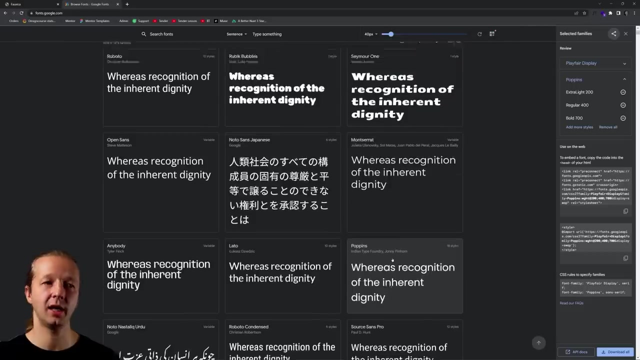 download it essentially, and so play. fair display and poppins are two fonts that are available from Google fonts, so here's how that works and create a new tab: fonts. Google comm we're gonna go to, and there's a bunch of cool fonts that you can use in your project. there's tons of them, so I'm gonna do a search here. 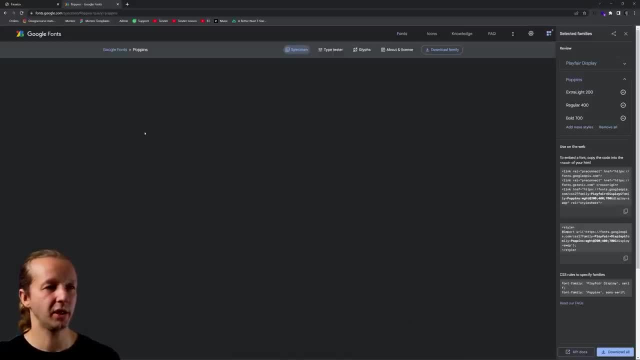 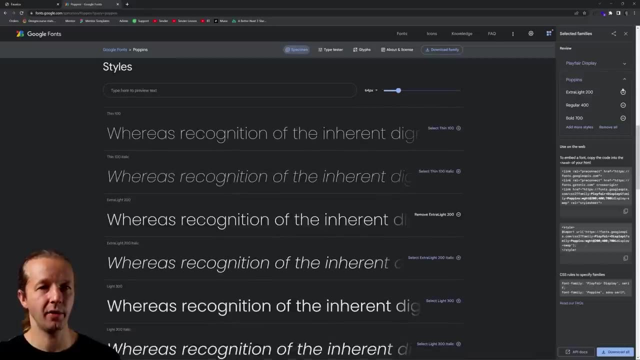 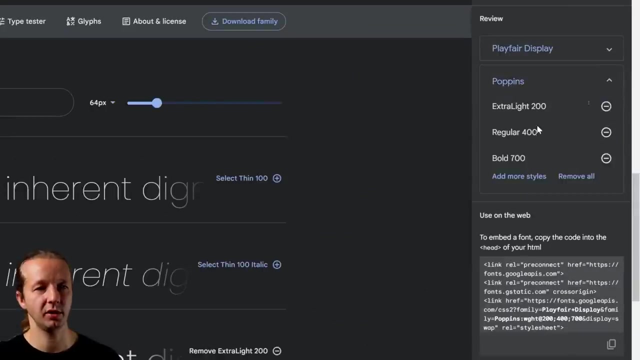 Poppins. you'll see it right there. you click it and notice I have, because I've already set this up. I already have the fonts here. notice how it says I zoom up Poppins, I have extra light, 200, 400 and 700 and I have play fair display. 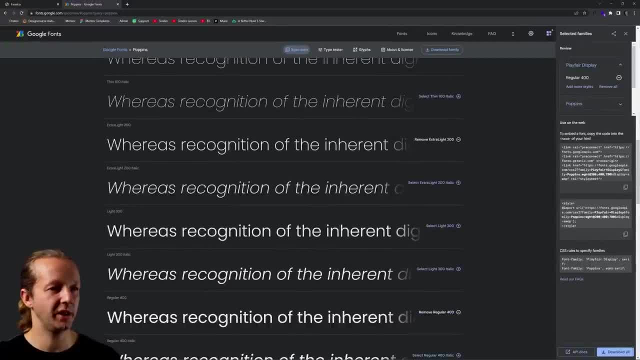 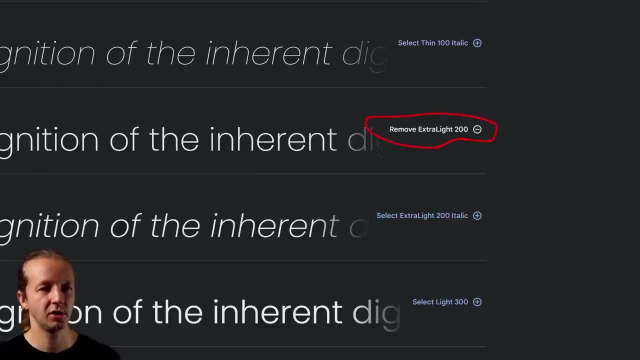 regular 400, just one style so you could see all the different font weights associate associated with Poppins. and so right here it's gonna say extra light 200. you want to click select and then it's going to change that and when you click select it'll show. 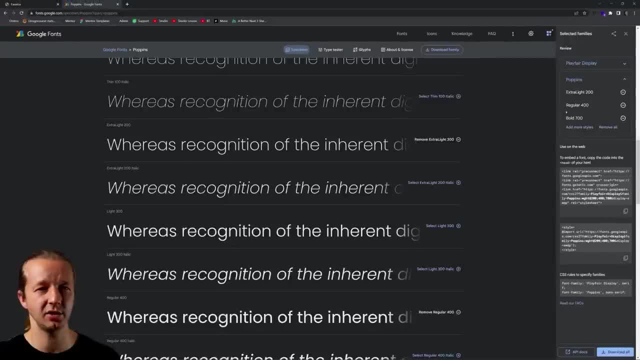 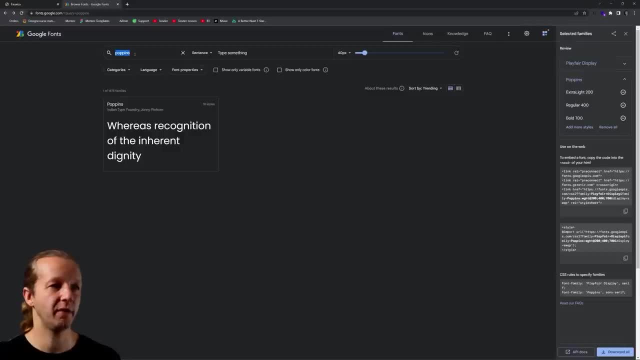 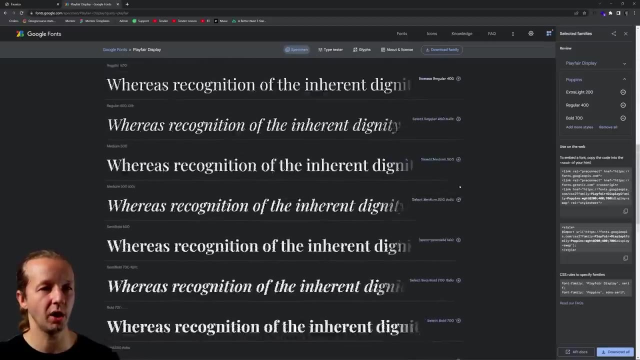 up over here in this area. hopefully that makes sense. you need to do that for 200, 400, 700 and then after you you did that for poppins. you just go back, type in playfair- you'll see playfair display right here and just do regular 400 right here. it's the top one. once you have this situation, 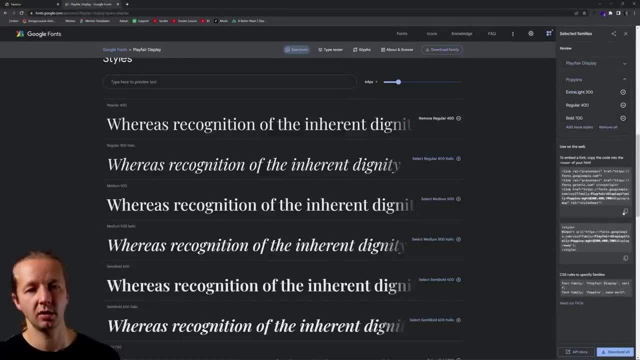 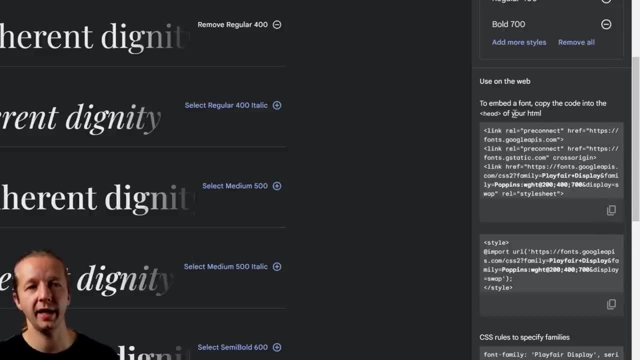 to your upper right corner. you can then let me zoom up. click this now. notice it says to embed a font. copy the code into the head of your html or, if you wanted to, you can actually import this as a style, or just take this hole right there. that's import text right there and put it at. 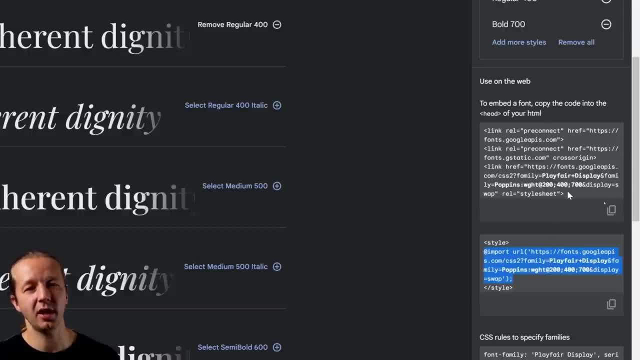 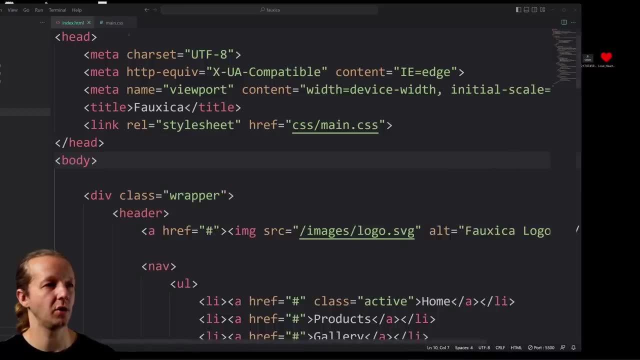 the very top of your css file. it's advisable, however, not to do that. just use this one right here: hit this little thing, that'll copy it to your clipboard, and we go to our html, we put it above our maincss file and just paste all that stuff. there's a lot. 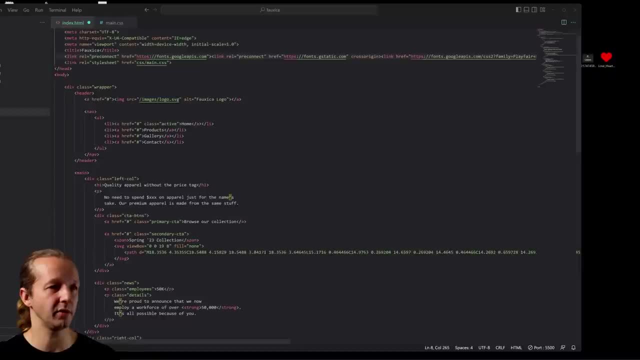 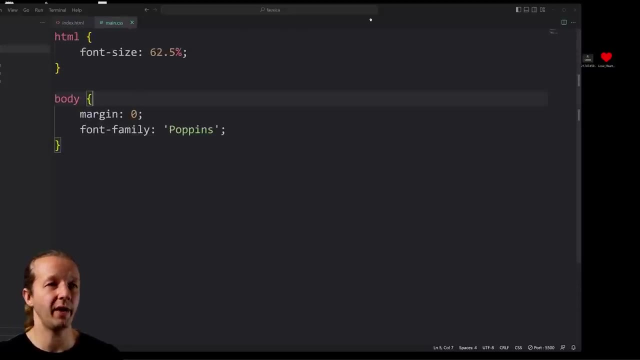 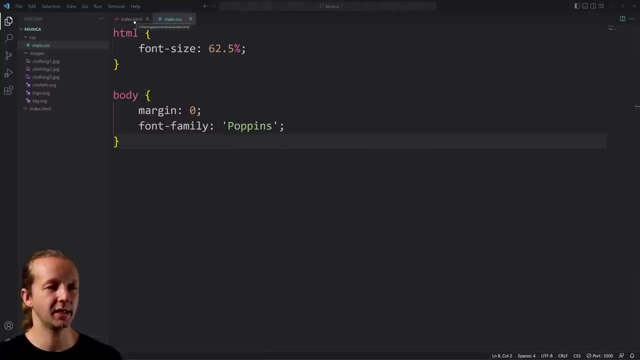 of stuff there. don't worry about trying to make it readable or whatever. it's fine as is so hit save and there we go. so now other people who don't have that font will be able to use it or see the font that we intend them to see. all right, so after that, what is the next element? it is wrapper, remember? 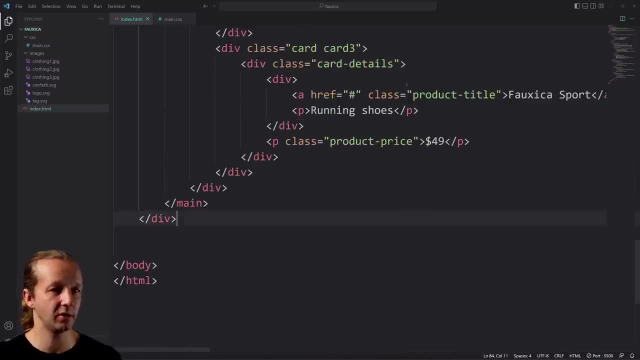 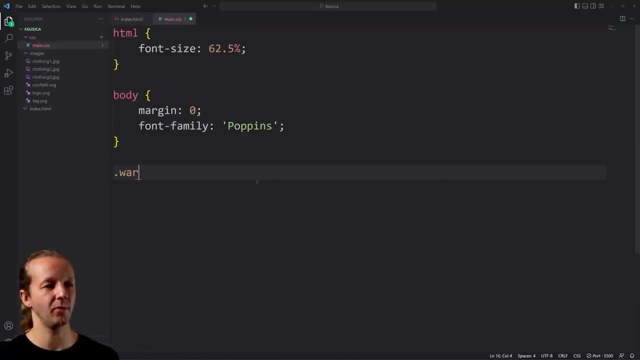 wrapper wraps around everything. see, it's highlighted all the way down here, so let's create the markup for that. so i'm going to put wrapper, not warper: wrapper. come on, gary, let's type. and the reason we need wrapper- and i tried to explain it before- is because, to a certain point, let's close that out. 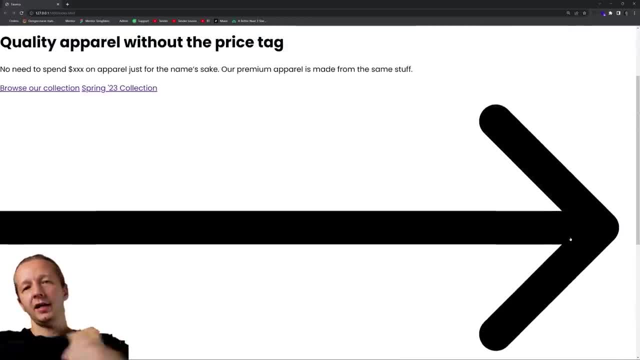 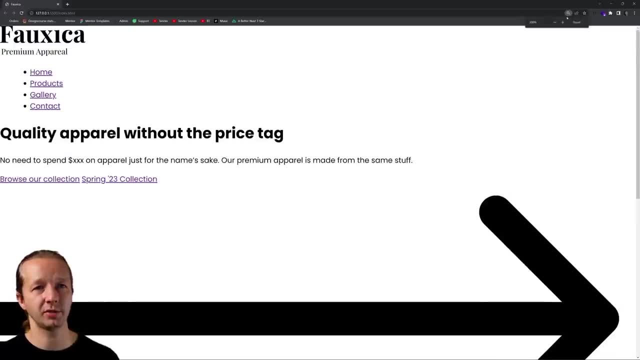 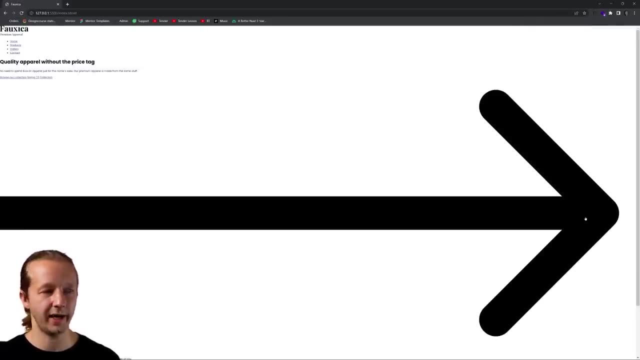 notice how everything is just like. take it's consuming the entire width of the browser and i'm on a 4k resolution monitor right now, so it's real large and i'm also zoomed up, so let me reset that. okay, there we go. and so this, this, this huge arrow is letting us know that wrapper is doing nothing what we want. 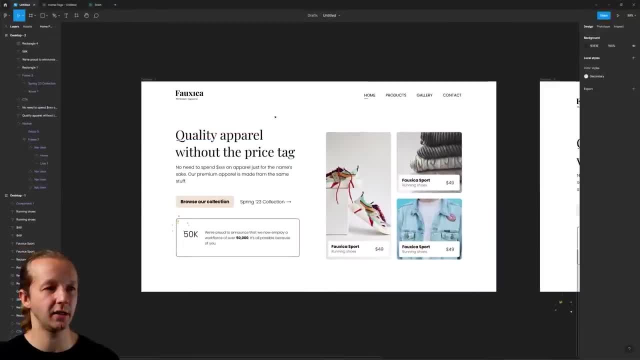 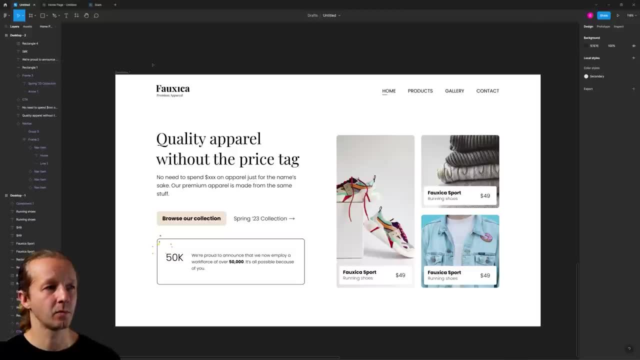 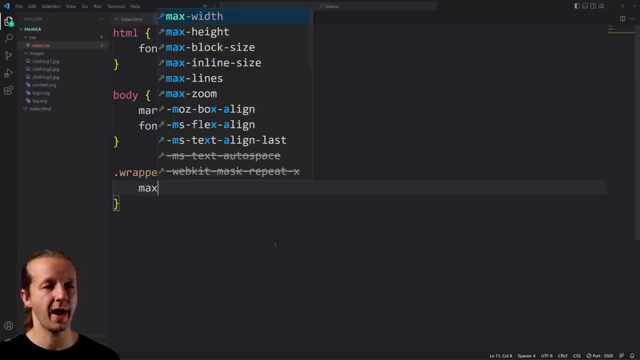 wrapper to do is what we intended to do in our design. we want white space over here to the right and the left here on desktop. so to do that, i'm going to come back here and we're going to say there's a property called max height, max hyphen width, and that's going to be 1200 pixels. 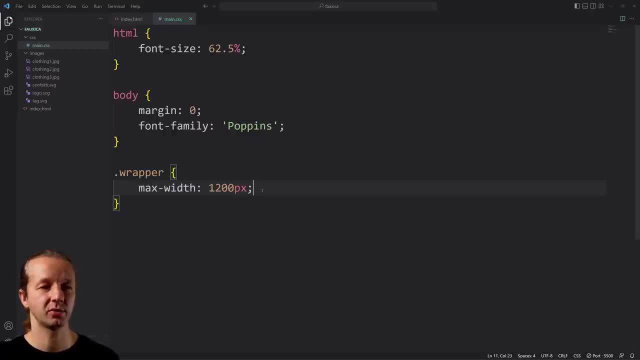 now, where did i get 1200 pixels from? i just kind of pulled it out of thin air. no, it's actually pretty close. it's probably very roughly close, i, to the value that's probably over here. so ancients get 1200 pixels from? i just kind of pulled it out of thin air. no, it's actually pretty close, it's. 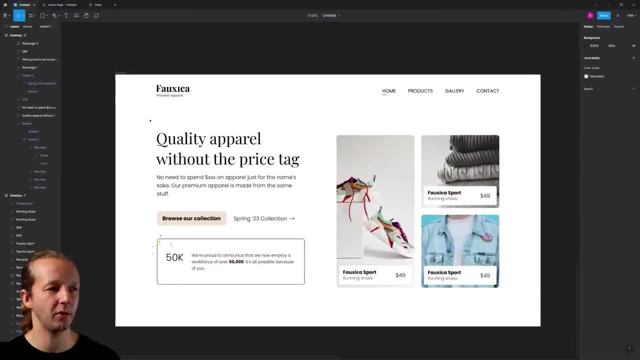 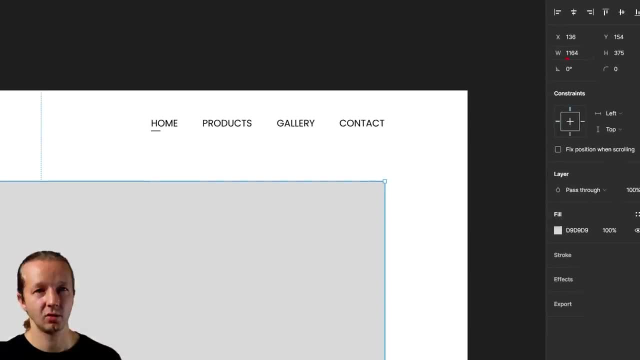 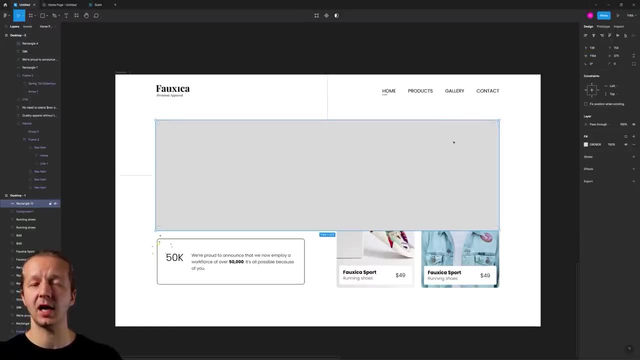 probably very roughly close, uh, to the value that's probably over here. so if i hit rectangle, i do this: it is 1164.. so 1200 pixels is golden ciudad based, meaning that yeni율 1200 pixels is a pretty standard for me when it comes to the maximum width of my design. 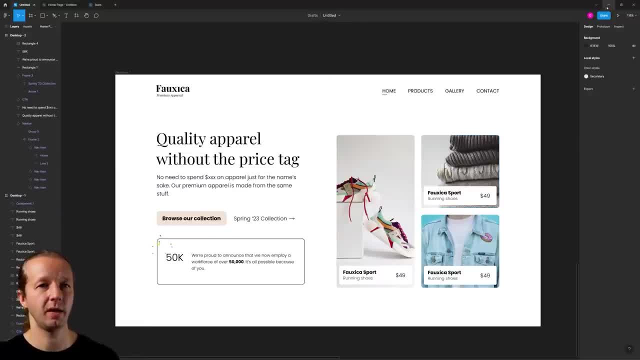 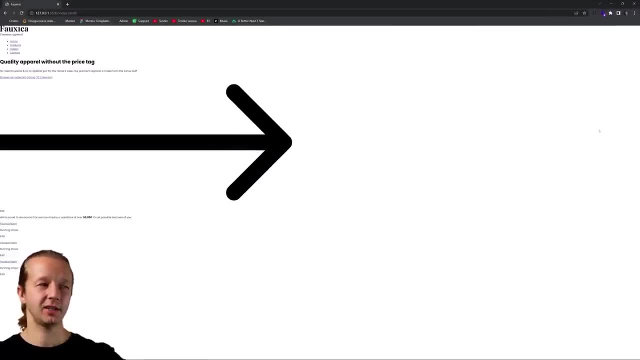 on desktop, if that makes sense. Now, if I go back and I save this right now, notice how it doesn't extend all the way over, but notice how it's not centered. it's to the left. So to center something like this and it's going to be one of those things, there's a 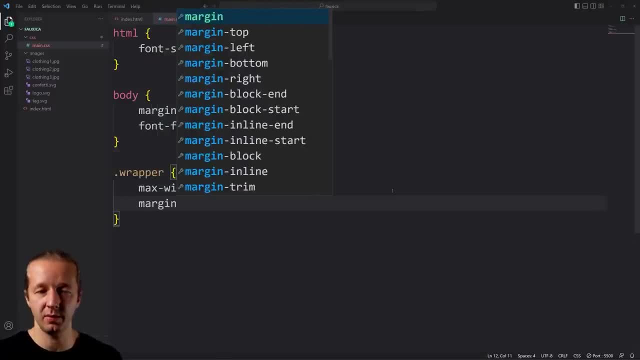 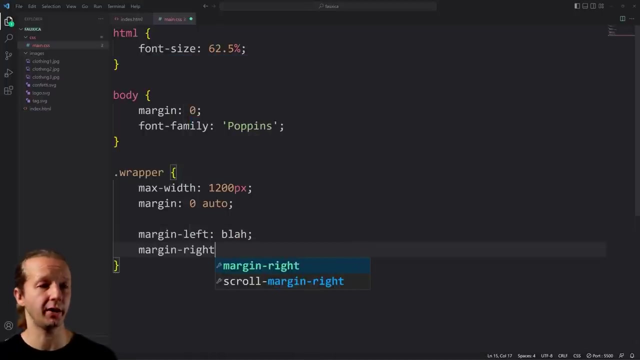 lot of properties to memorize. It's annoying, but you'll get it if you keep on doing this. through muscle memory We type in margin zero, auto. Now margin is a shorthand for margin left, blah, margin right, margin top, margin bottom. 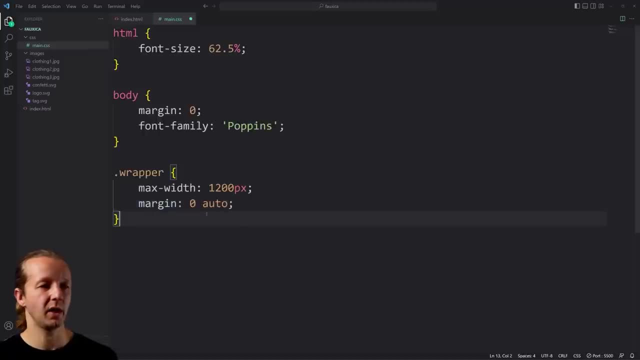 blah, blah, blah blah. and it's a shorthand property and the way you can write margin is top and bottom is zero, so no margin or white space at the top or bottom. but setting right and left to auto will center it automatically. it will center this element and that's what. 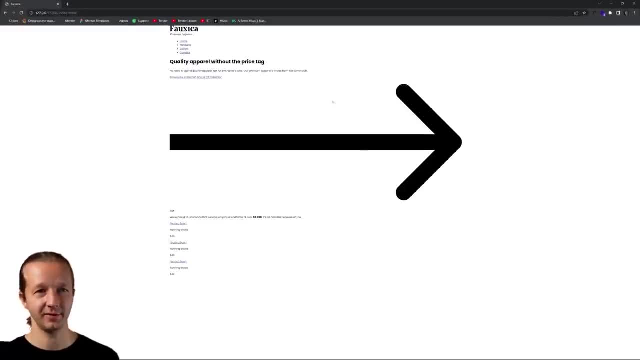 we want. So if we hit save, guess what It's all centered and that's what we want. Hopefully that makes sense. Don't get discouraged, because this is a crash course, and I'm just. It's a crash course. 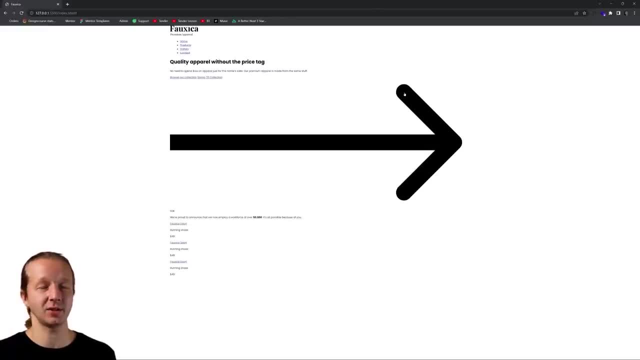 You probably feel like you've been hit by a car by now. That's why you need to take my course. I'm telling you. we start at the very basics. So, anyhow, sorry, shameless plugs. What we're going to do now is, after that is start focusing on our navigation section. 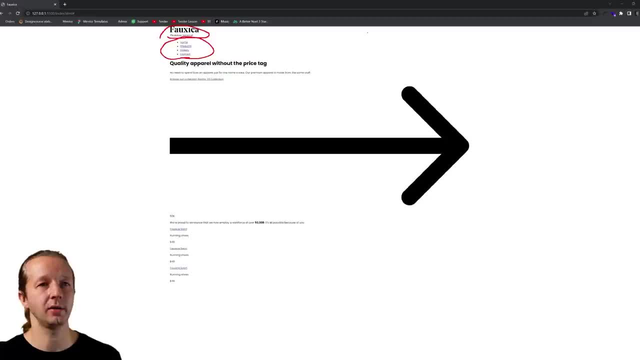 which is the logo, and this element right here. All right, so now we're getting to the fun stuff, because we're going to start piecing together this layout. It's going to start looking exactly like our Figma design. Okay, so, going back, let's look at the HTML markup for that section. 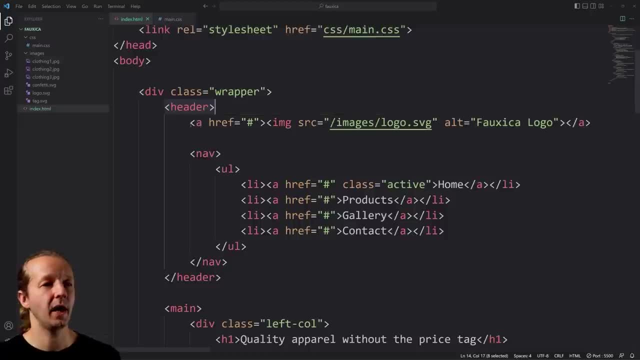 We have a header element and it has two elements inside of it: an A element, which is the logo, and then the nav element. Now, remember, I said ad nauseum, I said a bunch of times: Okay, We need to wrap these elements that show up with each other in columns next to each other. 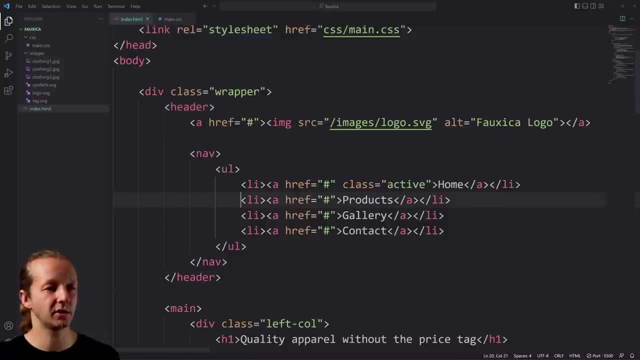 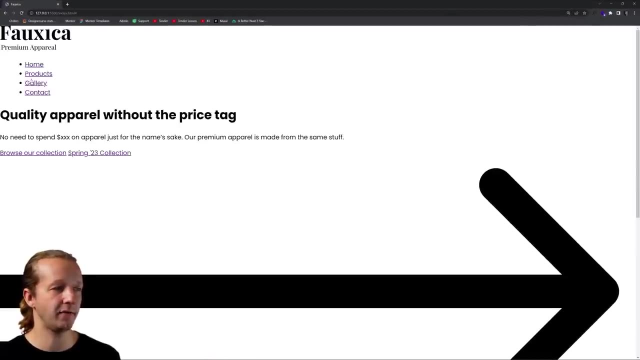 and so header is that element. And so the way we do this, because if we look back again here, these are sitting on top of each other, Foxica's on top of this nav element, but Foxica needs to be over here, and then this nav element. 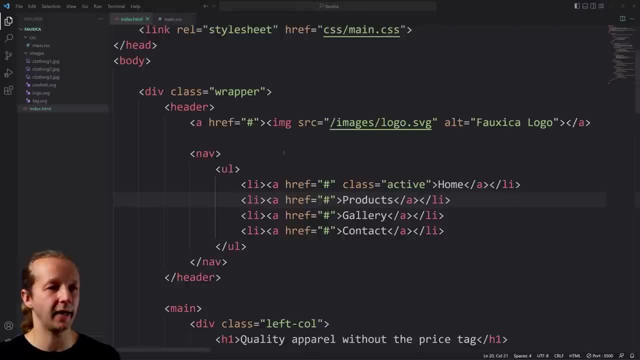 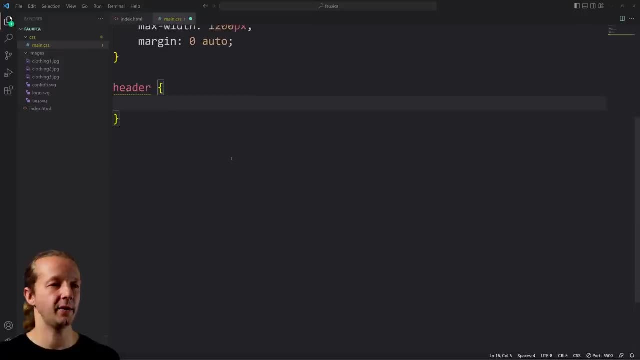 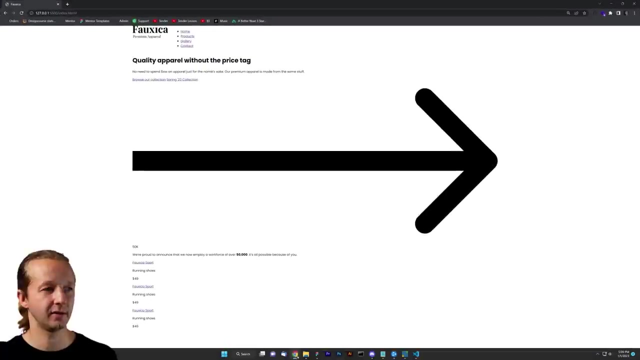 needs to be pushed over here somewhere, okay. So to do that, we take the element that's wrapping around both of them, Header- and we say display flex. Now just watch what happens when I save that. Look what's happened. We have our logo and now it is sitting right beside it. 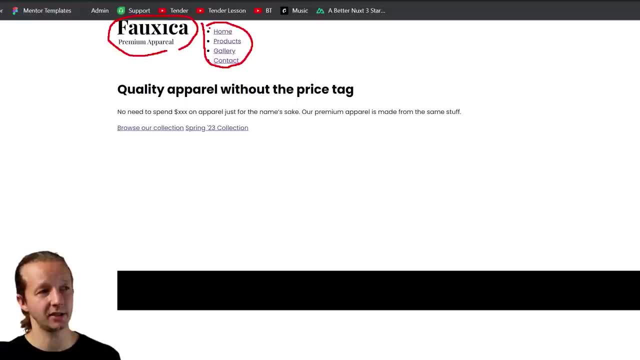 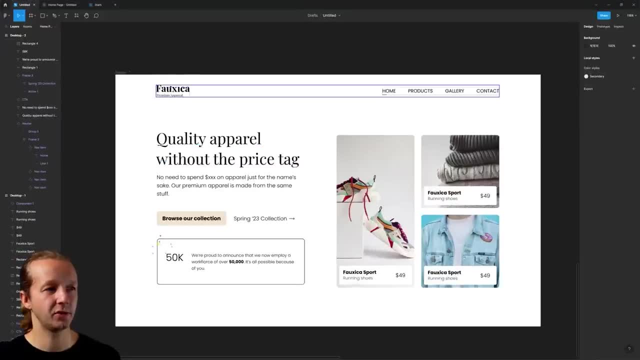 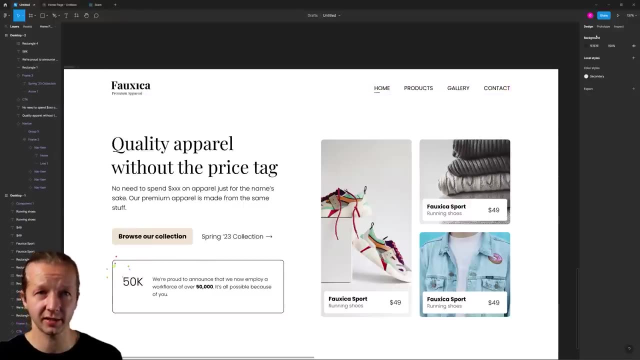 It has created two columns for us. That's awesome. It's a step in the right direction, because if you look over here, you will see that we have two columns over here and over here. Okay, So we obviously still have a ways to go for our navigation to look like this. 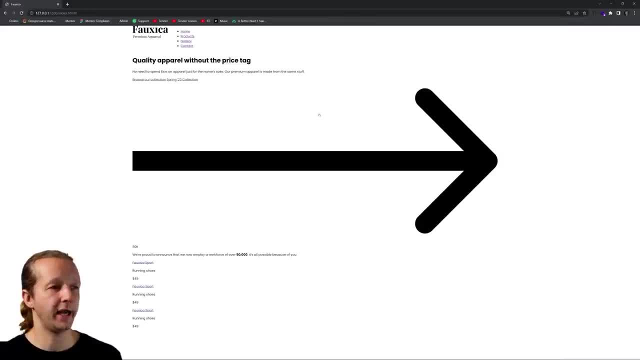 Right now it looks butt ugly. it really does, So we're going to get to that in a second, But now what we want to do is we want to use another property and, by the way, display flex is a property that allows us to structure layouts. 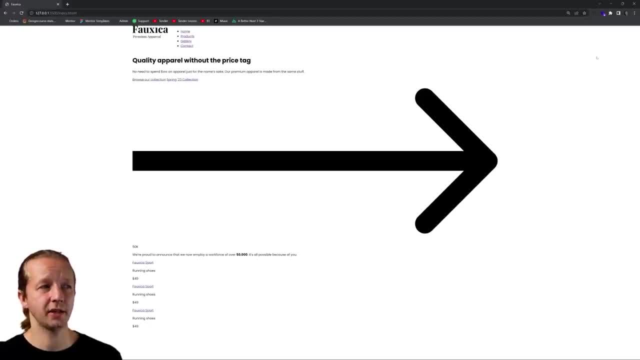 There's also display grid, which we will use, but display flex when you need to create two columns or three columns or whatever. it's a very good method of doing so. It's called flexbox, and I could create a whole course on flexbox alone, but this is 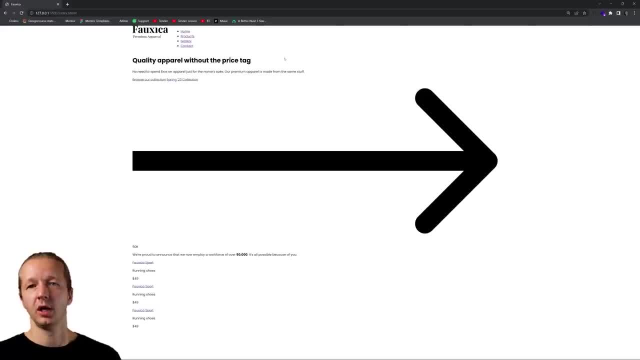 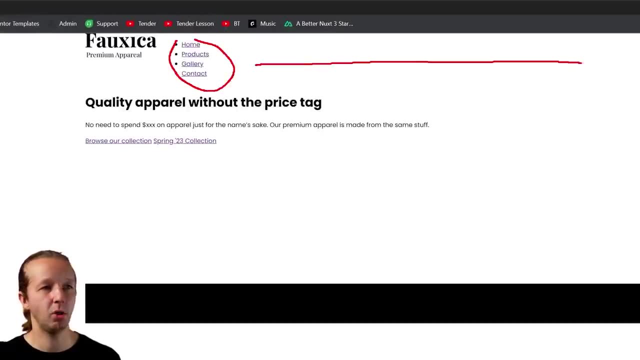 a crash course, So we're kind of working through things as we need them. Now what we want to do is we want to designate this nav element and we need to push it all the way over here, because that's how the design is. 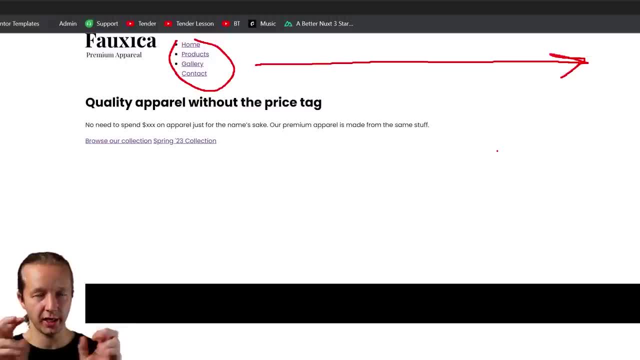 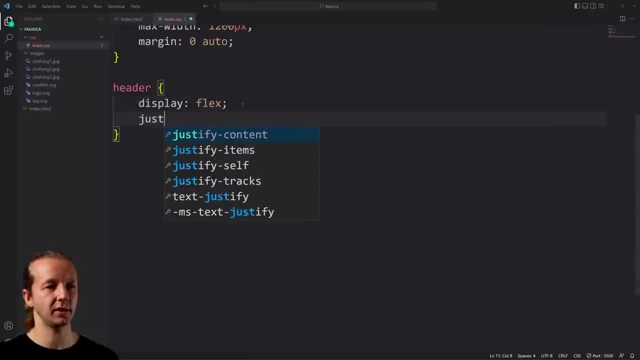 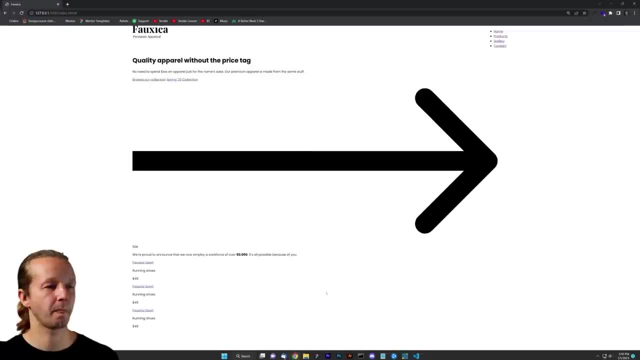 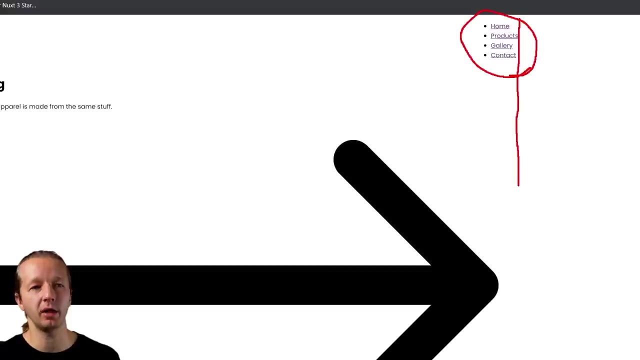 We need to use something that will create space between these elements, these flexbox items. So we'd say, justify content J content, space between Save that. And look at that, We have our element right over here. It reaches the very edge of our wrapper element, which has an invisible line that goes all. 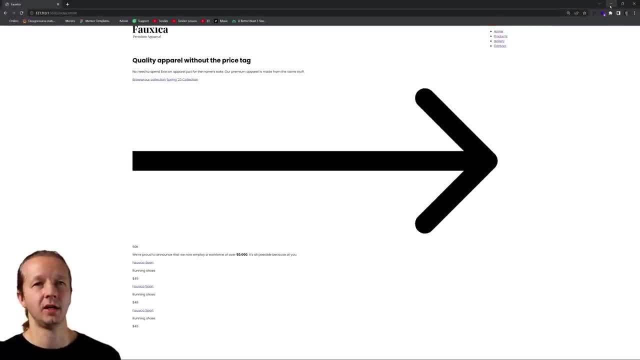 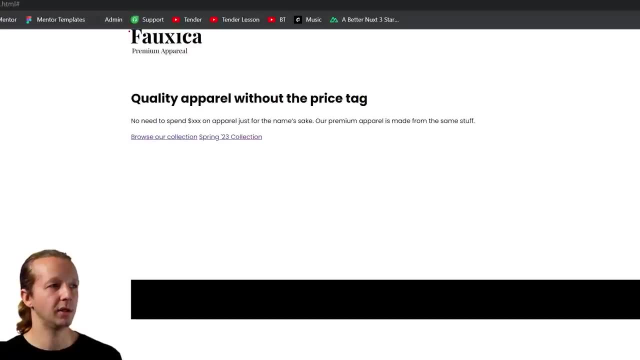 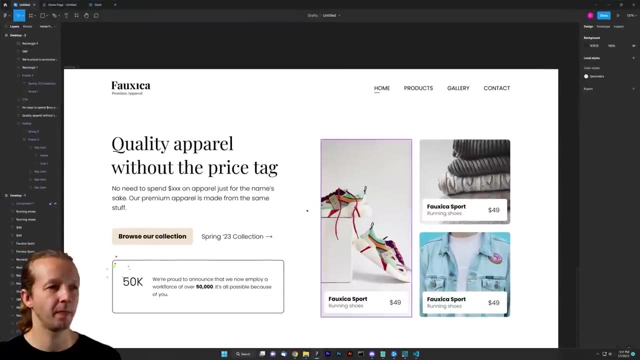 the way around here. All right, great, So next up. another thing we want to do is notice how there's no white space above our logo. If we look at the design in Figma, you will see we have a bunch of white space. 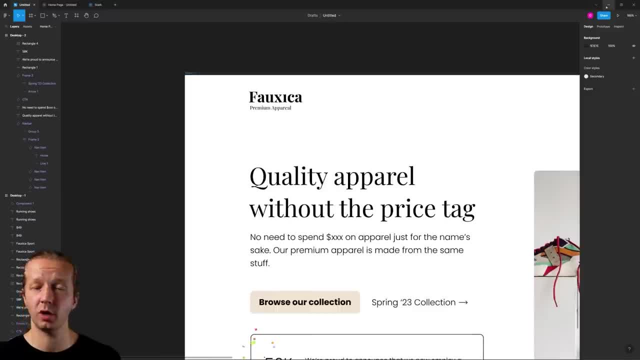 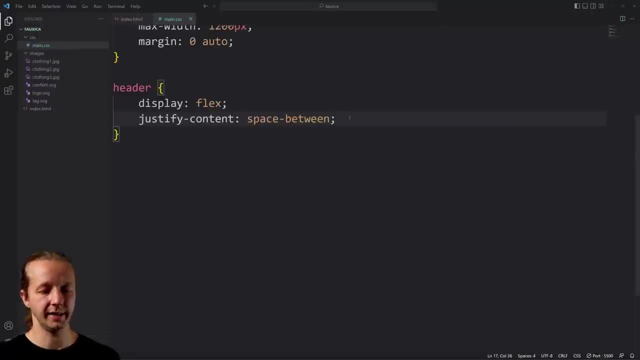 One of the ways we can ensure that white space is there is through margin padding and also, in our case- and this is another flexbox sort of property- align items center. So that means all the items that are found within header which are the A element, and 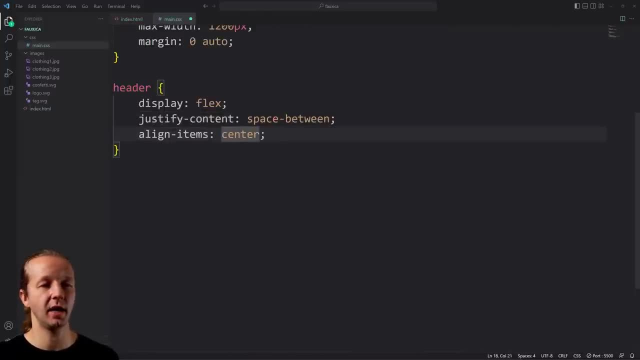 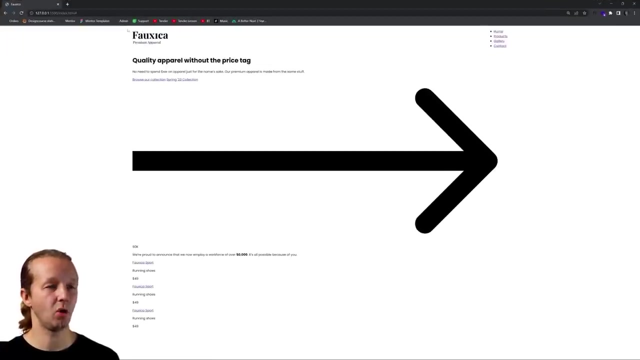 the nav element We're going to align them on. and align items is alignment on the vertical axis, So it's going to align them to the vertical center. So watch what happens. We save that and guess what? Based on the overall header element that wraps around these two elements, it's going to center. 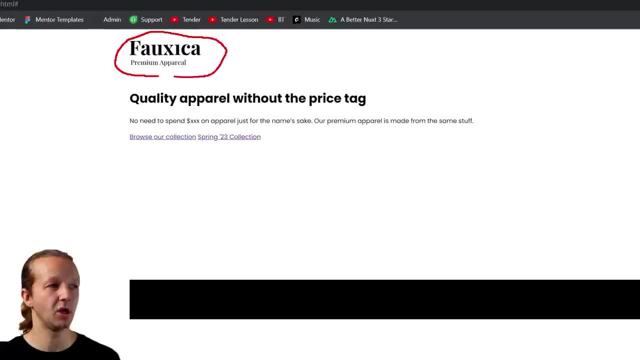 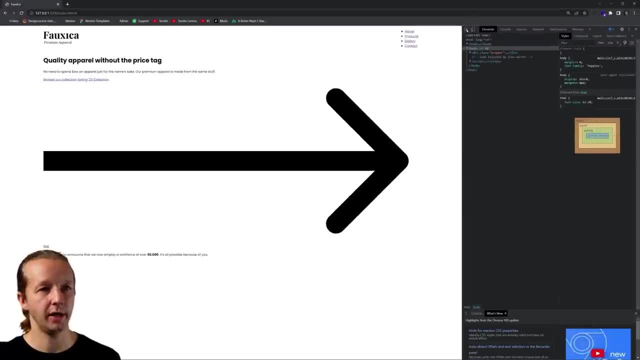 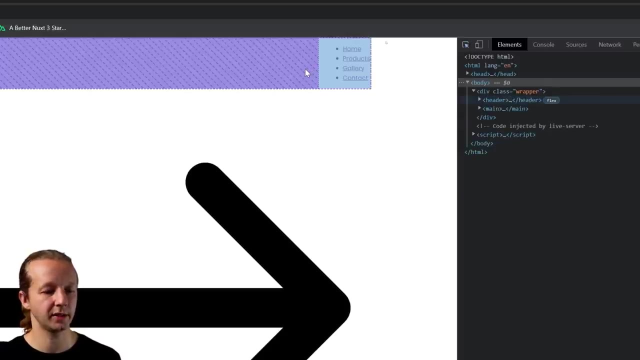 them vertically with align items. So this is now centered. We can visualize this. actually, if we hit F12 to get the developer console, Okay, We click on this little thing right here, this little selecty thing, And if we hover over this, you'll see that this is now in the center of this flexbox. 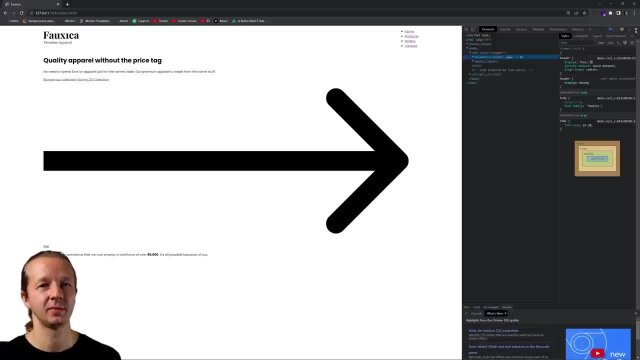 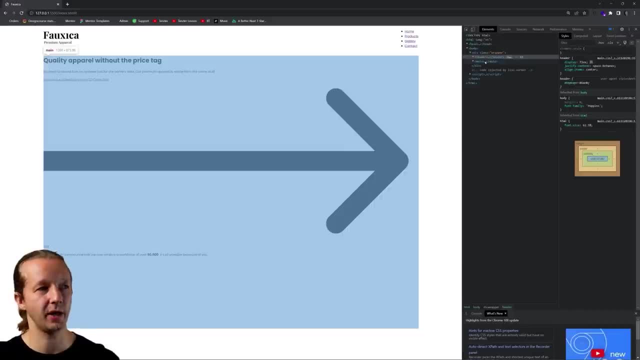 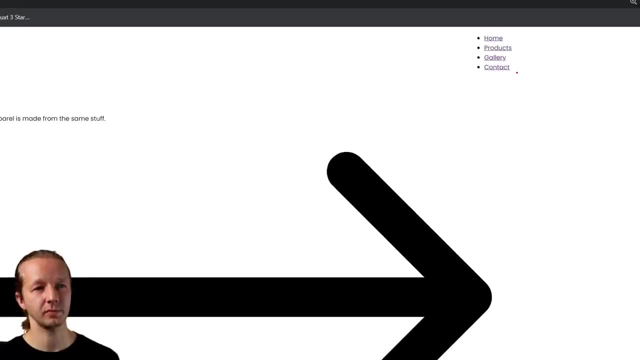 container. All right, So hopefully that makes sense. So the developer console, which you can access through F12, is very handy to help you visualize where things are, And there's a lot of things you can do with it. Okay, So now we have to work on this nav, because this is default and it looks very ugly. 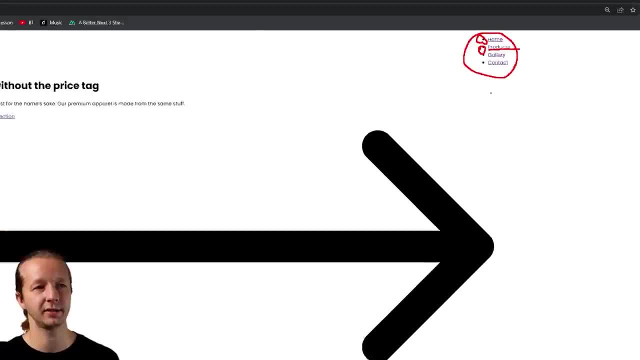 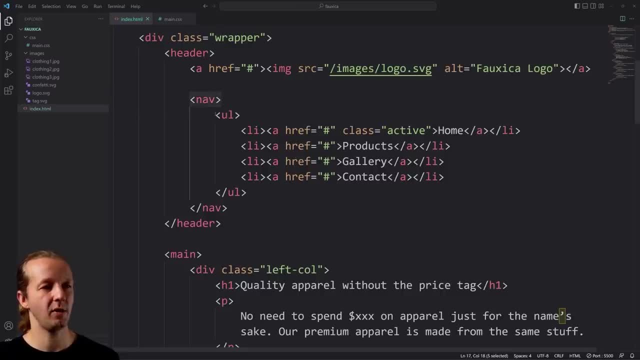 We don't need these little dots and all that crap, don't need the underlines, So let's get to that. So, referring back to the HTML, we have a nav element with a UL element- unordered list- and then we have our list items inside of it. 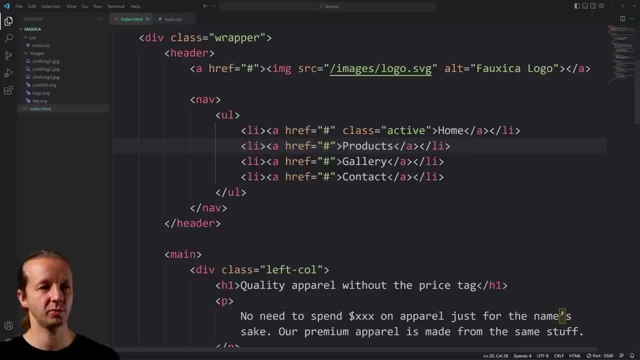 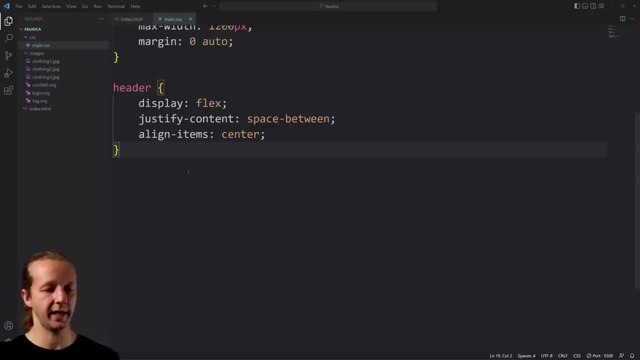 So what we'll do first is we're going to specify and create a rule set with one property for our nav element itself. Okay, And that is going to be a margin of four M units, or in other words 40 pixels. So if we save that, it's just going to give us more white space around it. 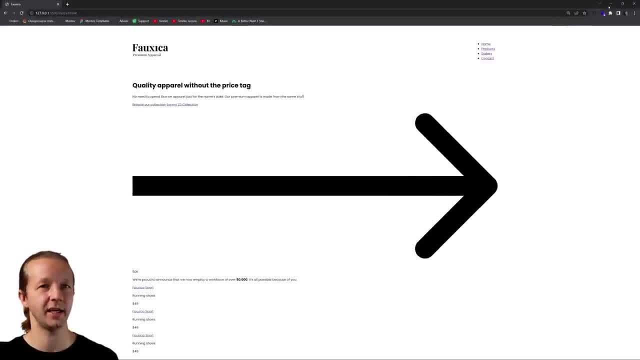 It doesn't make sense as to why I did this yet, but you'll see in a second and I'll show you a before and after. if we remove that rule set we just created Now, after that we're going to go ahead and target the UL, the nav UL element. 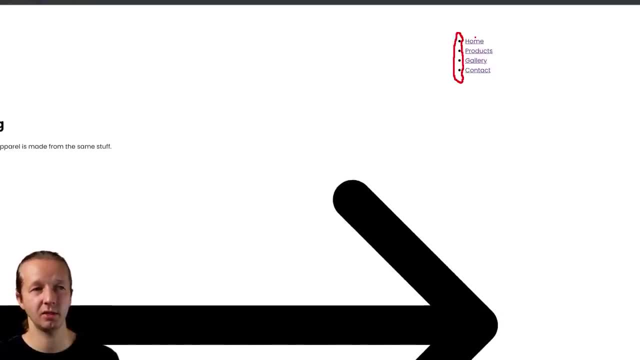 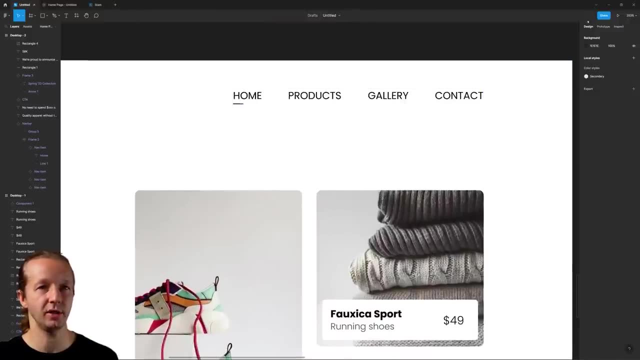 We need to get rid of these little circles. Okay, They don't exist in the original design. Again, as a refresher, our nav looks like this: There's no periods, little circles, right? So that's one of the things we'll do in this rule set, among others. 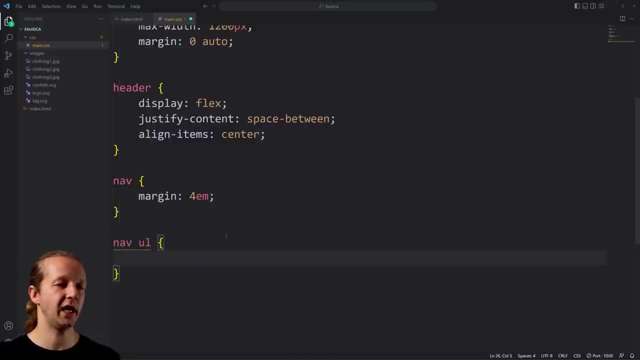 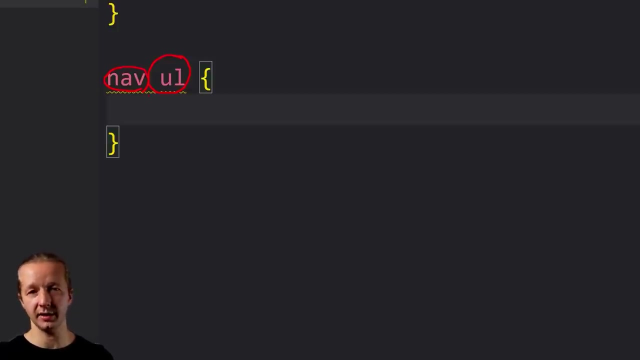 So we're going to take our nav UL, So we're chaining these together right here because we want to only target the unordered list that exists within the nav element, Because there might be other multiple unordered lists In our design. there isn't, but there could be. 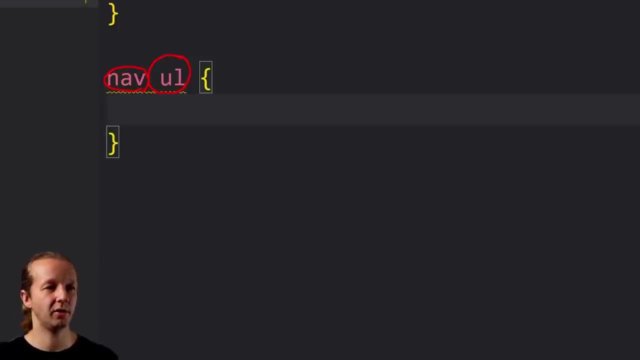 So we don't want to just put UL itself, So nav UL just is a command, a selector that says only select in style or apply this rule set and this CSS styling to unordered lists. that exists within nav. Okay So, and, by the way, we could have given this unordered list a class, like you know, main. 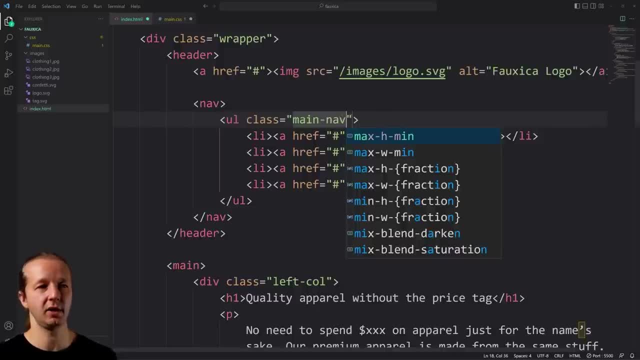 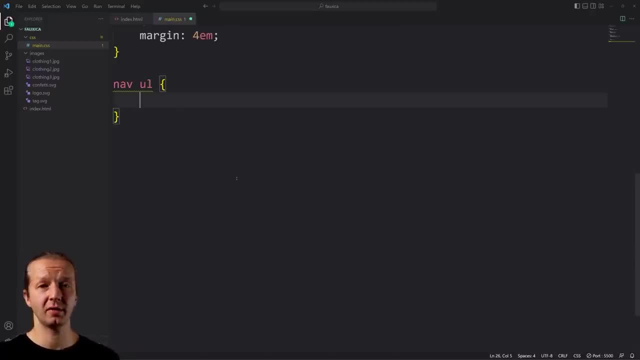 nav and then we could just reference period main nav. So you have options. That's just how I'm choosing to do it here. I wanted to show different ways, All right, And so the way we get rid of those little periods, list style type none. 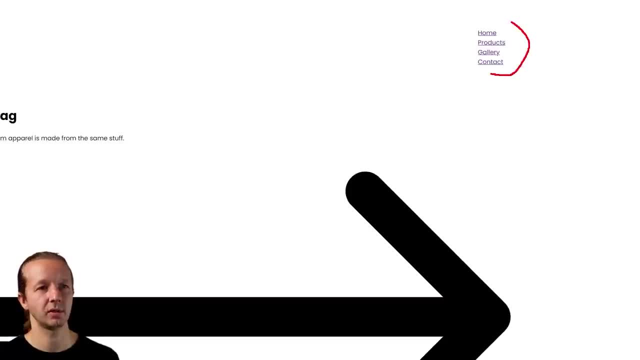 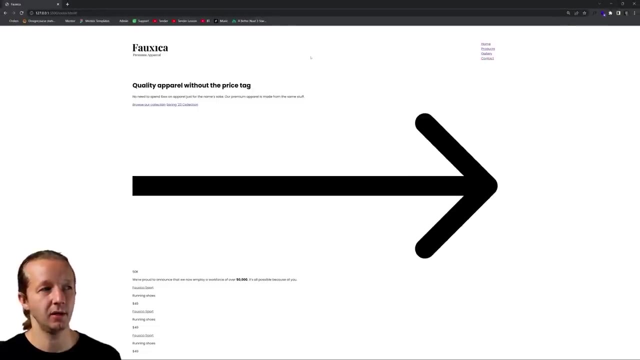 So if we save it, those things will disappear. Tada, Now we don't need four rows: one, two, three, four. We need four columns like this. And if you recall, how do we do that? Well, In these elements- the logo, in the nav- we just simply add display flex. 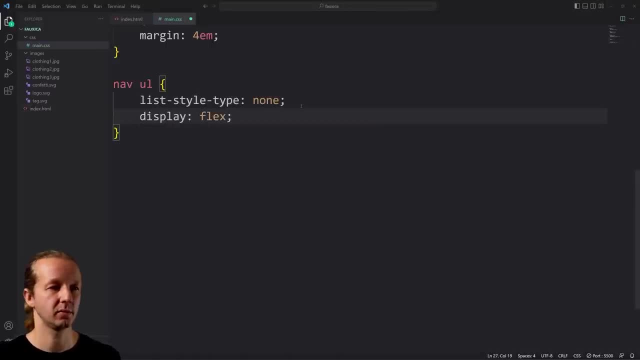 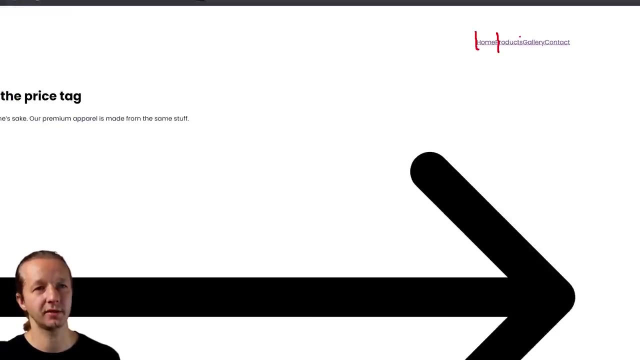 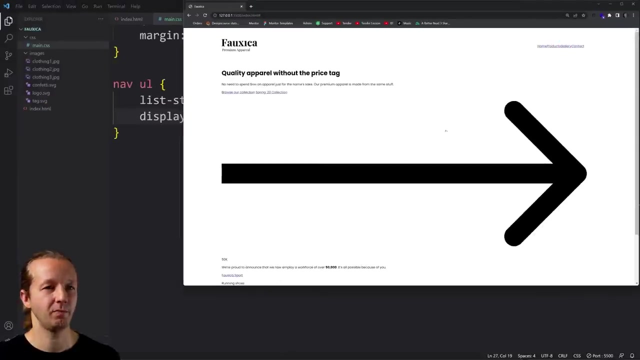 So display flex, save it and look at that. They are actually in four columns, but there's no white space between them, So that's not good. So how do we figure out the amount of white space to use? Well, we can come over here. 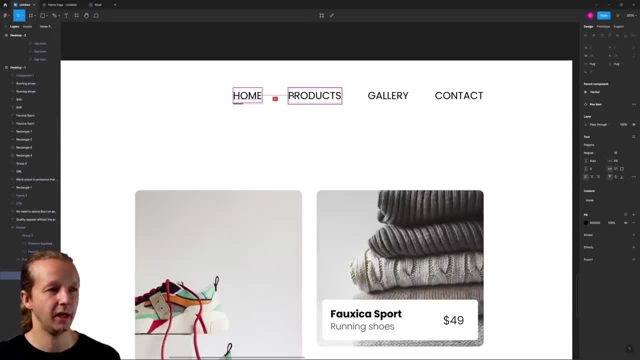 And we can just Control left click to select this one. And if we hold alt and then hover over this, this adjacent nav item, you'll see it says 41.. All right, So 4.1, that's why we use that font size: 62.5% hack. 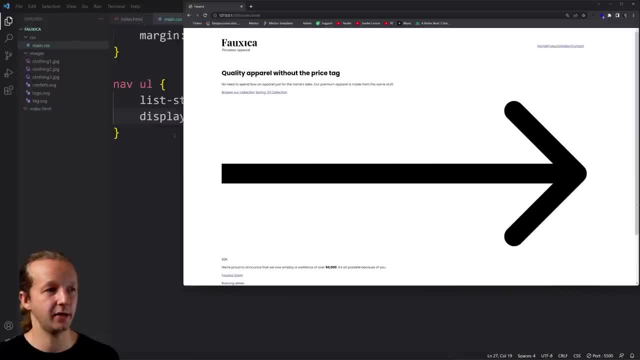 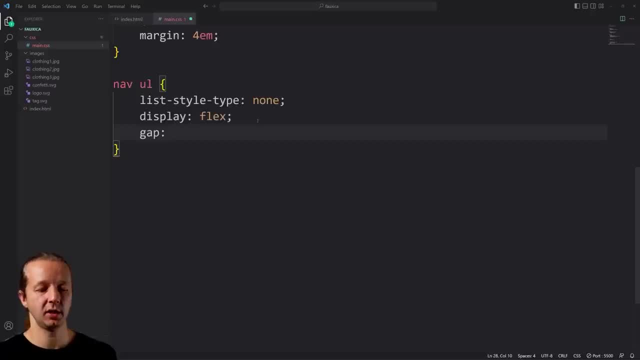 So I we're going to say gap, which is literally gap at the gap between these, these elements is going to be 4.1.. And we're going to say M units, Save it, Go back. And there we go. 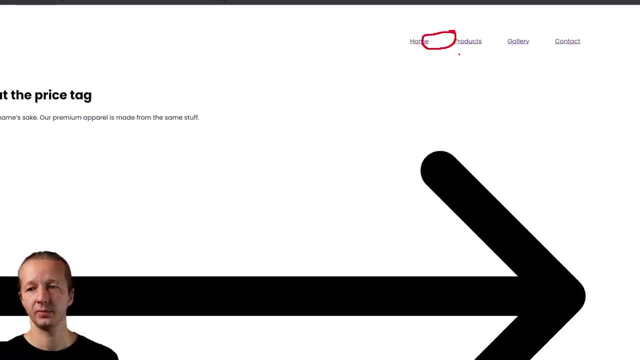 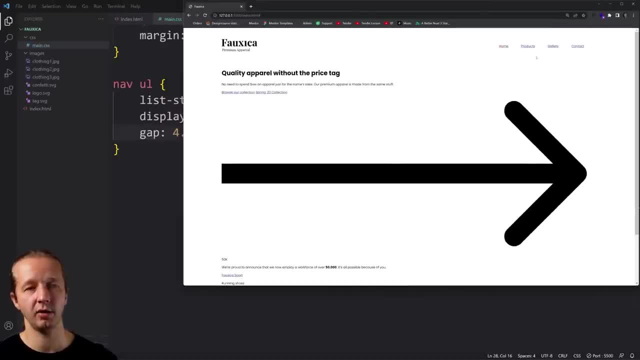 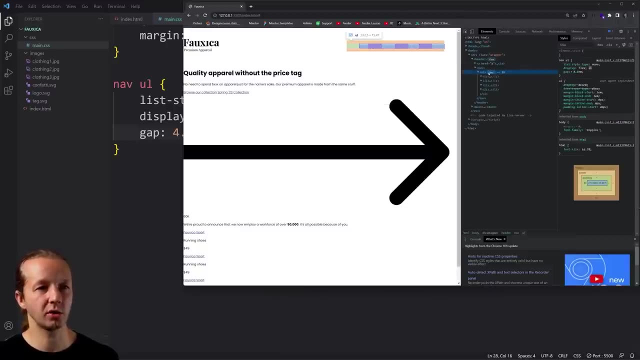 Ta-da Okay. So now another thing I want to do is: you can't really tell, and we can tell if we get out our dev console F12 and we select it And if we hover over our unordered list. so let me zoom up here. 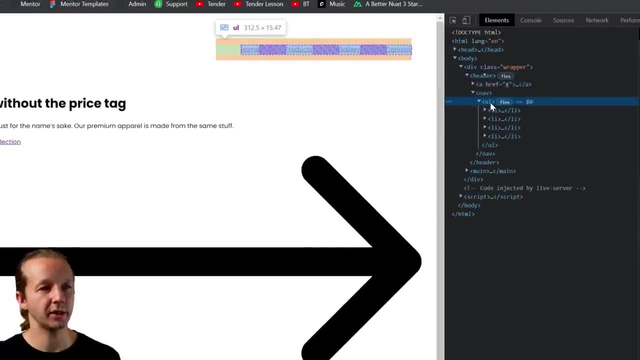 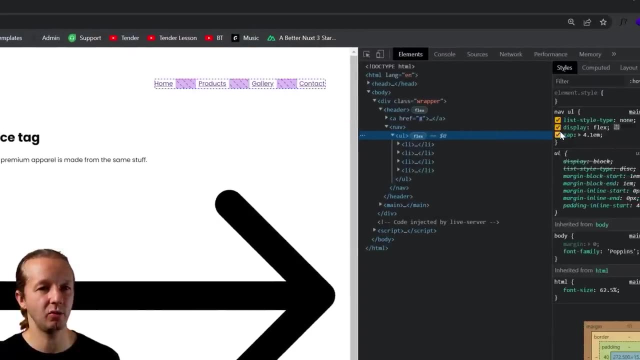 Notice that orange stuff around there. You see that orange stuff, Yeah, Yeah, Yeah. Well, that orange stuff simply means that the browser is adding by default some styling around this. And if I move over here and we could see where it says margin block start margin, it says: 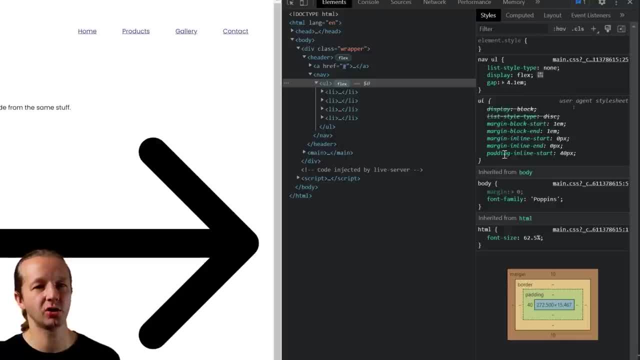 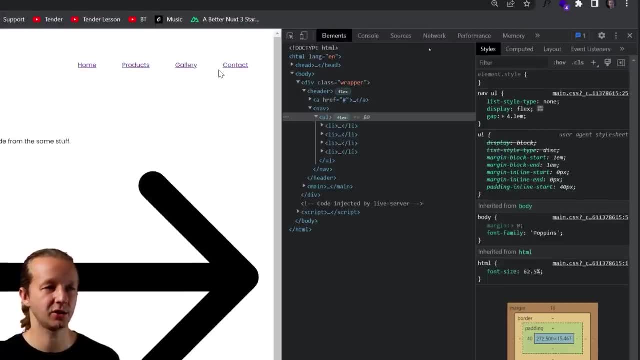 one M unit, and that's essentially what's created. also, padding inline start And it's creating white space around there by default that we don't really want. All right, So what we're going to do is reset the margins, as it's called. 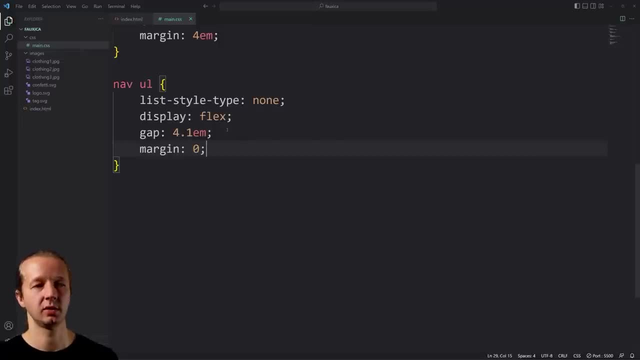 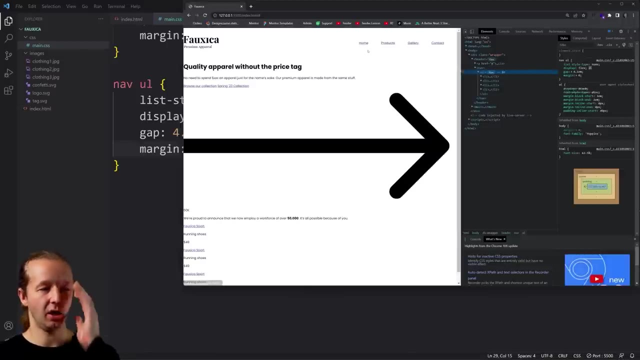 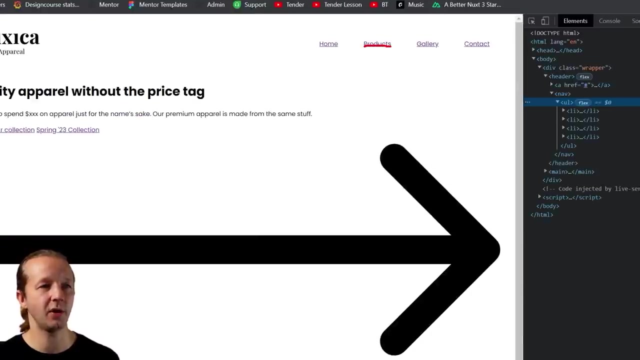 So margin zero. We'll save that. You're not going to notice like a huge difference, but it actually got rid of some white space around here, All right. Next up, we have to start actually styling these links, because we don't want these type. 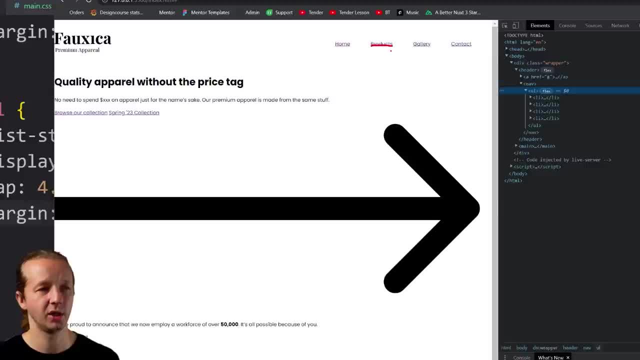 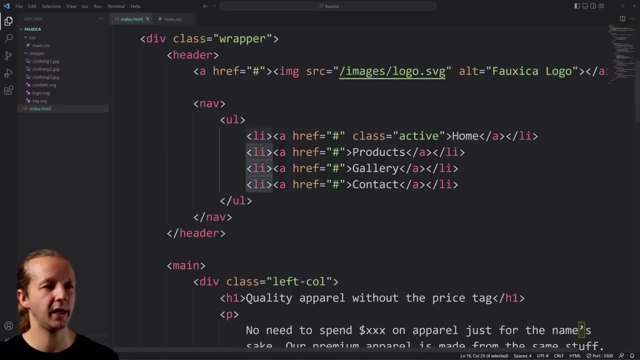 of underlines. We don't want this color, this kind of purple color, And so what we want to do is now, if we look at the HTML, We have Nav U L L I A. This is where we start to change the actual appearance of these elements. this: 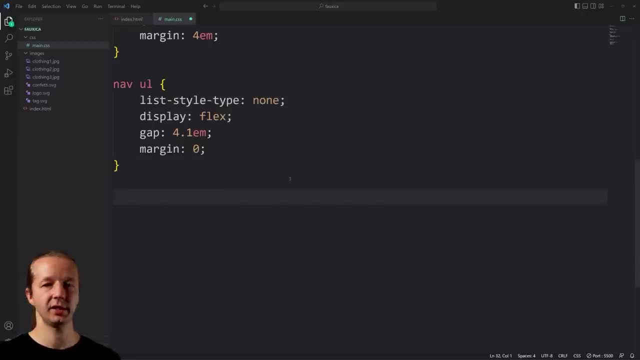 A element, So we could say nav A. So this will target any links that are in the nav element. That would work just fine. If you want to be real specific, U L L I A. Same thing. Well, it's not going to change. 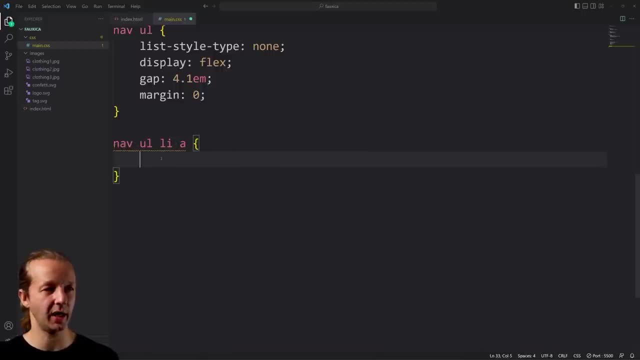 Okay, So it's almost the same thing, except we're being specific. Specificity is a thing. So now what we'll do is we're going to say text decoration. none That will get rid of, if I save it, the underlines. 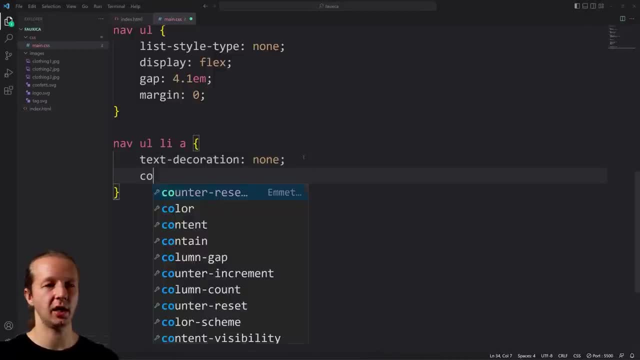 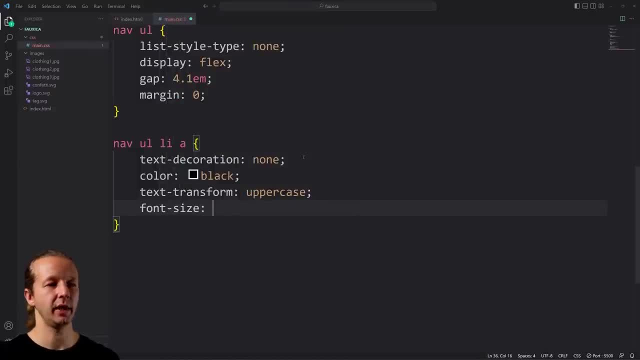 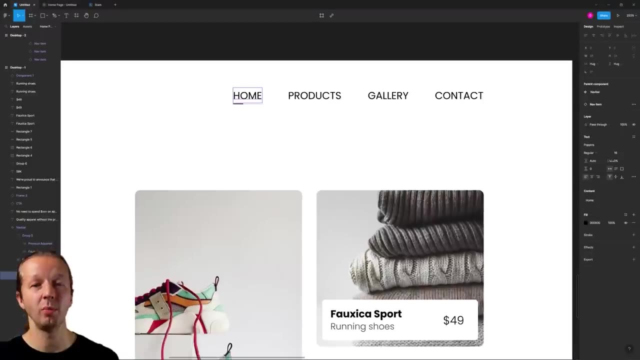 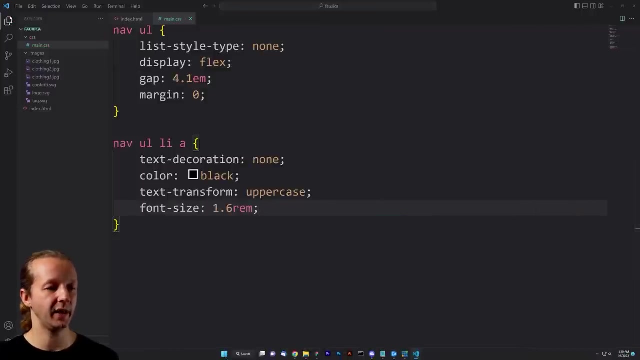 We're going to go. We're going to go ahead and say font size. Now, what's the font size? Well, control click 16, 1.6 REM units. All right, So 1.6 REM units. If I save this, there we go. 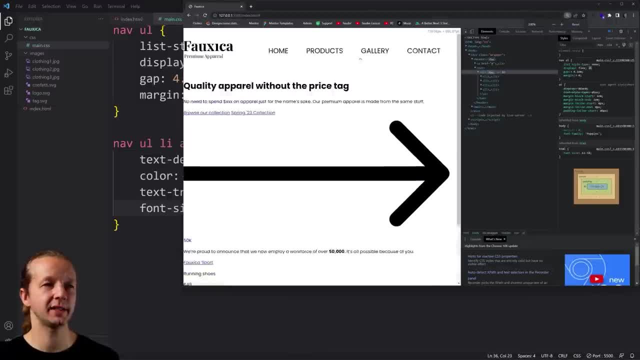 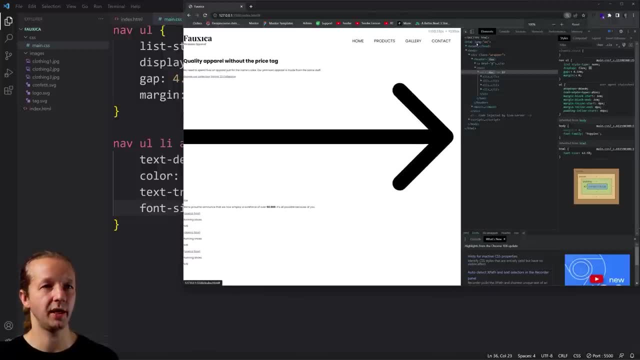 Now we're a lot closer. I'm going to reset my browser zoom. By the way, you can browse in and out, or zoom in and out with your control key plus your mouse scroll wheel. All right, So this is a hundred percent right here. 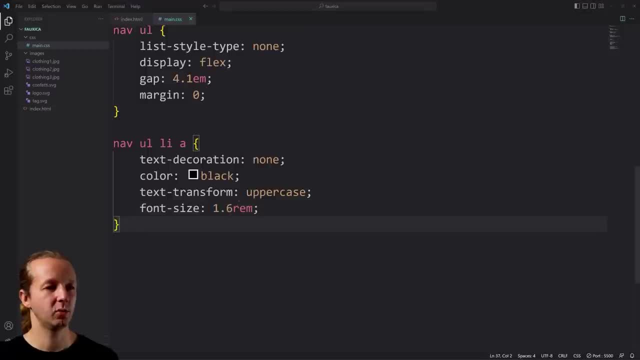 Now you might be wondering something is: what is the difference between REM and M Like? why did I use M on our gap property but on font size? have you used REM Well? in short, typically most of the time you're going to use REM units for your font. 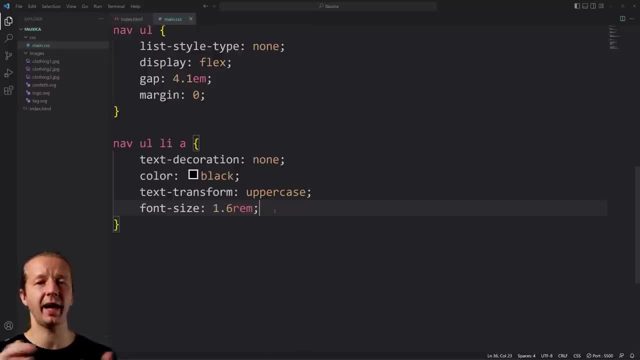 sizes And when it comes to stuff like scaling, like your distance, like margin and padding and stuff like that, Or border radius, You can use M, And sometimes it's difficult for me to off the top of my head while coding. explain the. 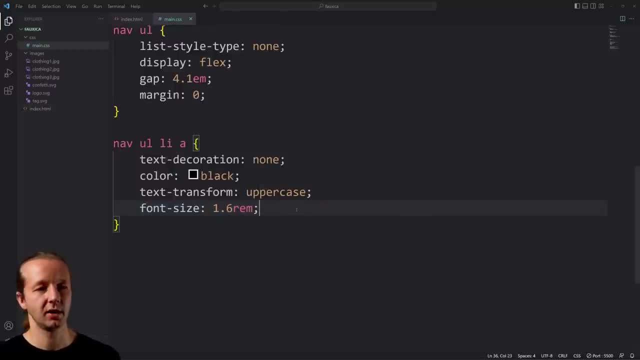 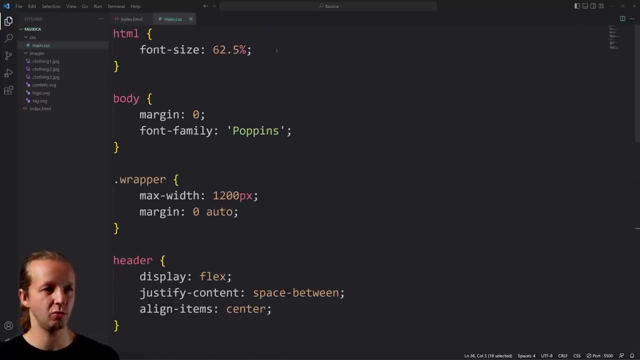 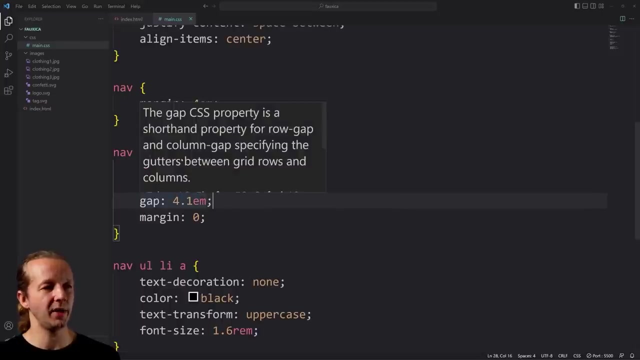 difference. REM simply means root M unit. All right, This is tied to the font size that has been established by our font size: 62.5%. The M unit This is. this gets tricky Because, say, for instance, this: this is attached to the font size. 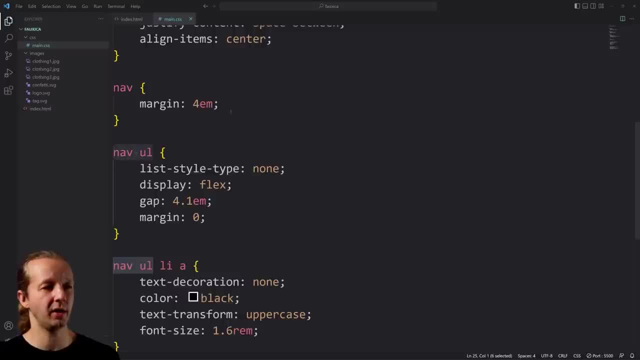 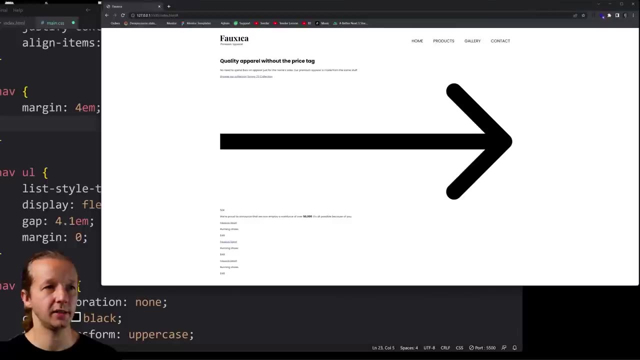 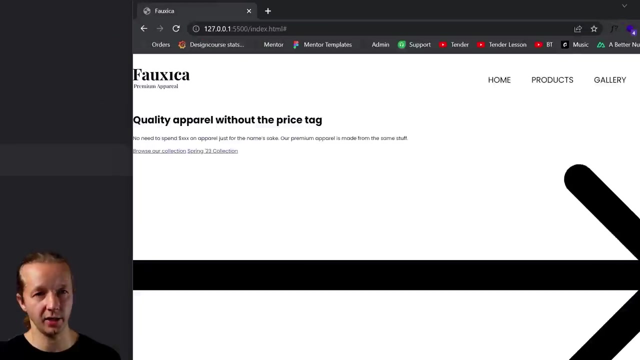 This is attached to the font size. Let's say, for instance, this: this is attached to the nav UL element. Let's say, for instance: I'm going to move this over and we're going to look at the, the current distance between these elements, these right here. 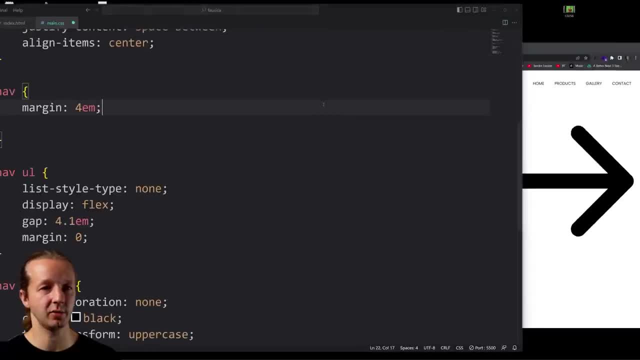 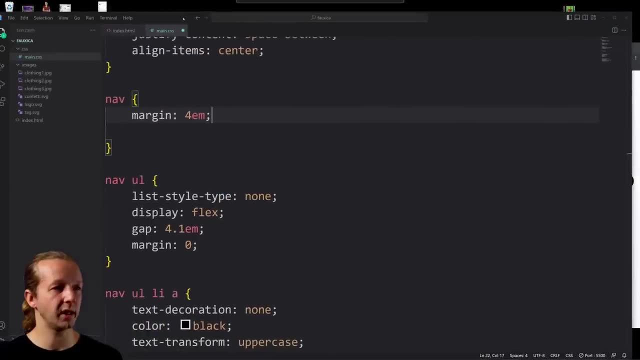 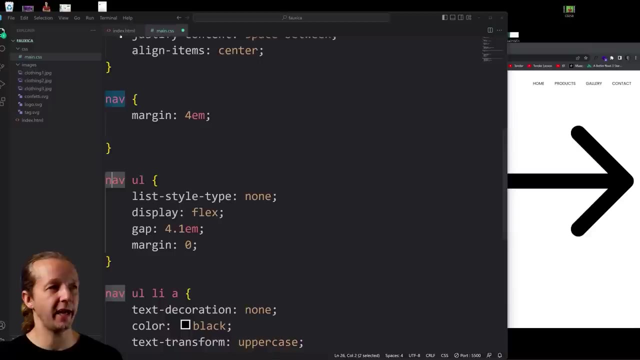 Notice we have this amount of white space, All right, So keep keep an eye out on that section. If I change over here, let's, let's get this structured a little bit Better. So UL is nested inside of nav. 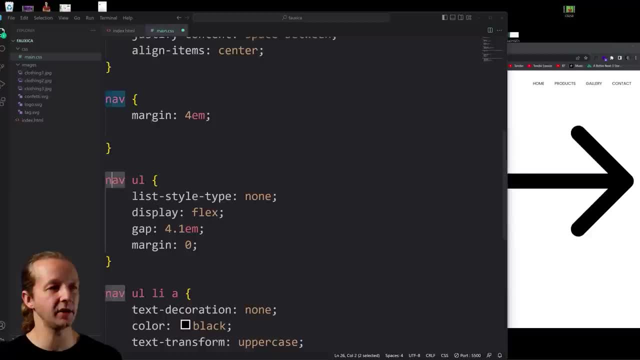 And we know that through our HTML we have nav here and then UL is inside of it. I if I change the font size property to like three M units or something and save it. look what happened to that amount of white space between these elements. 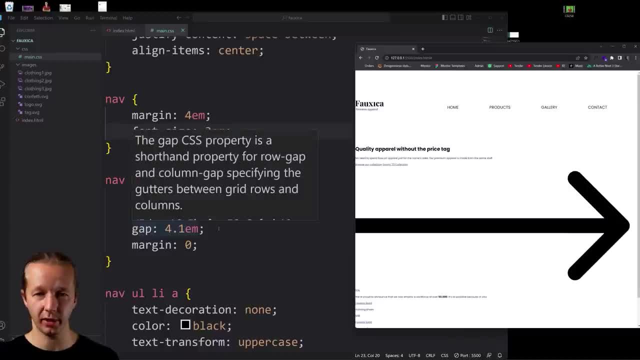 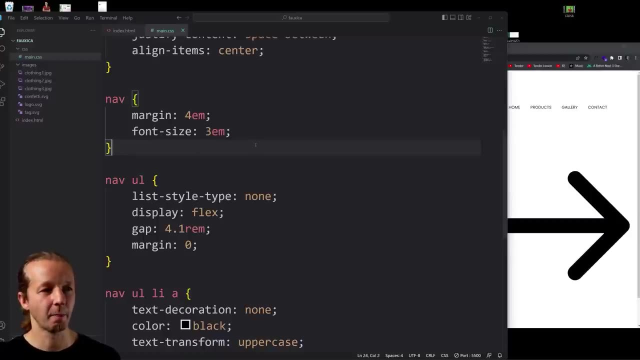 It just like: multiplied this 4.1 to some value, right? So if this was a REM unit, Okay, Guess what? And I save it. It doesn't get affected by the font size that exists in the other elements that it's nested. 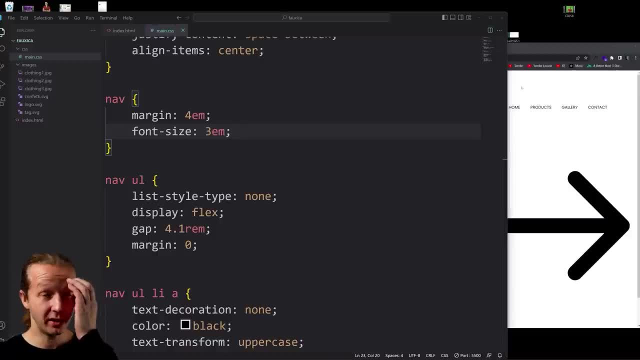 within, if that makes sense, And I'm not going to go into exactly why or why exactly we want to use M versus REM in certain use cases. There's some great videos specifically about this topic that you can find on YouTube, and also articles. 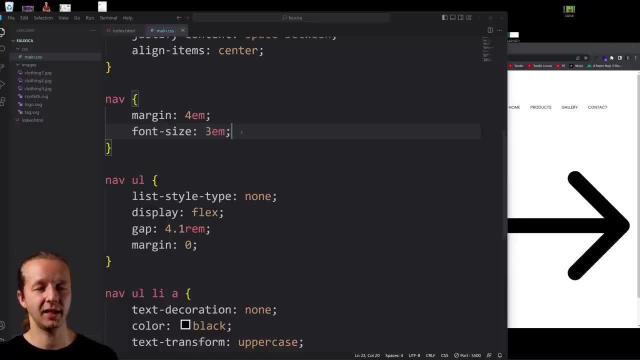 But as a general rule of thumb, us CSSers- you're a CSSer now- I typically use, for the font sizes your REM unit, and then for other stuff you typically use M unit. Okay, Oh boy, Enough of that explanation, right. 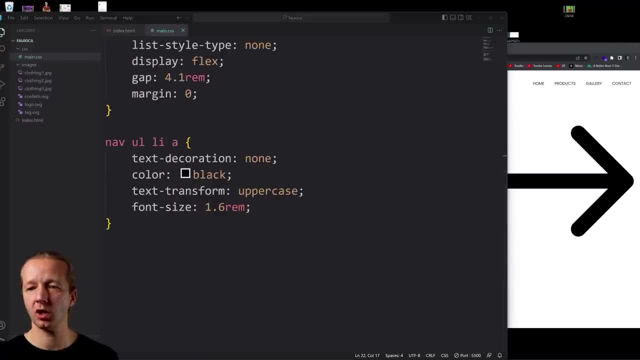 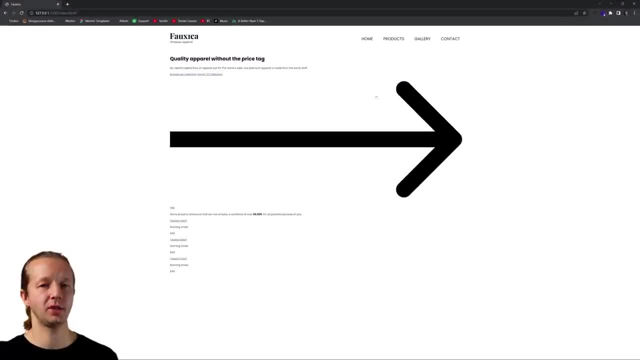 Okay, So now that we have our list item set up, that's looking pretty good, All right. So now we have an issue, and this is getting more into intermediate CSS. but this is a crash course And I wanted to show it to you. 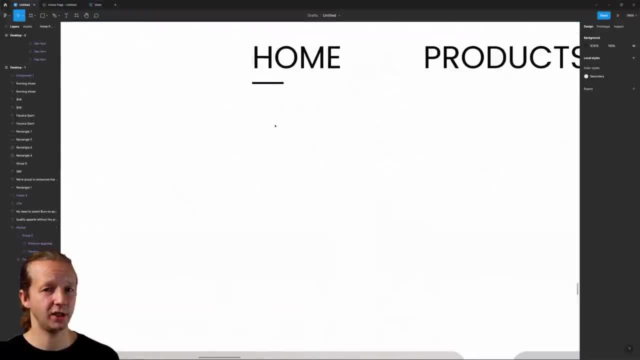 This right here, this underline. So remember, we did text decoration none to get rid of those underlines. Well, it's not like we can restyle those into a version that looks like this. We have to kind of create our own custom little element, this custom little asset underline. 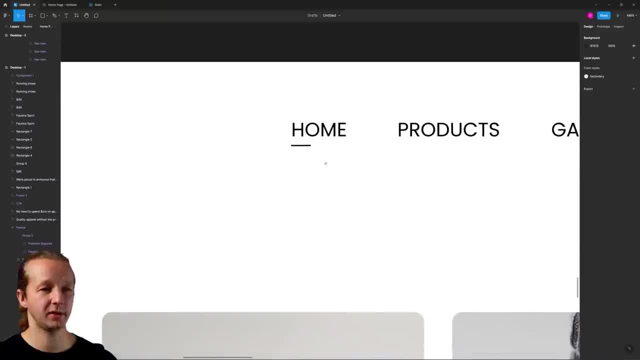 that we've created, And so we can do that purely with CSS. Here's how we do it. Every HTML element has what's called. It has what's called a before and after pseudo selector. Think of it as just a placeholder value where you can style extra things, like adding an. 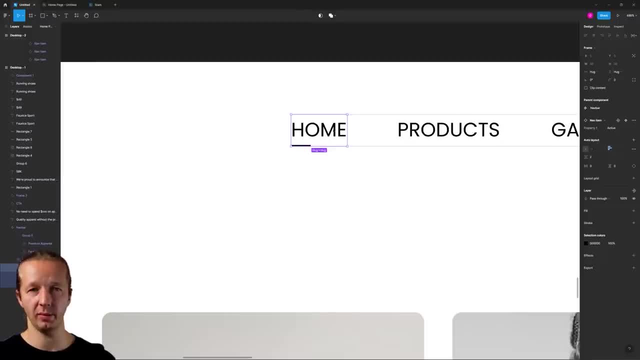 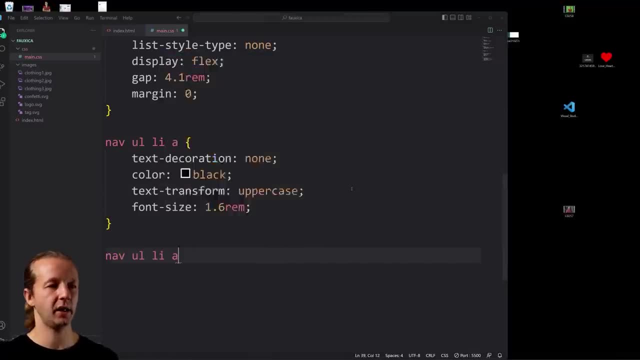 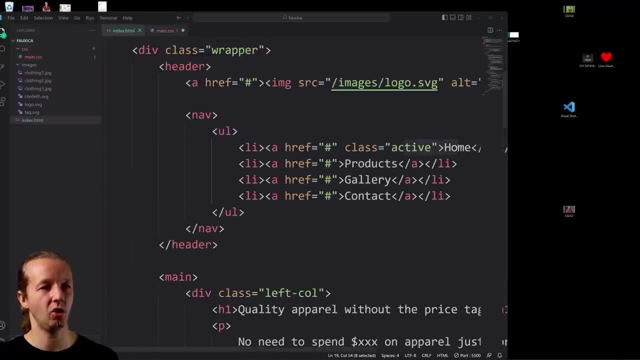 underline adjacent to this home element, this little nav element. So the way we do that is we're going to say nav U-L-I-A, just like above dot active, Because, remember, active is the one right here Home that we want to add that little underline to. 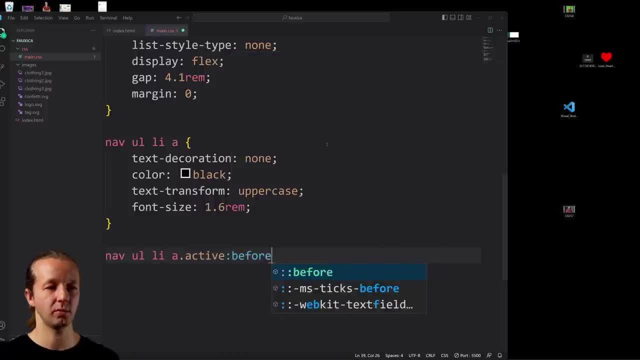 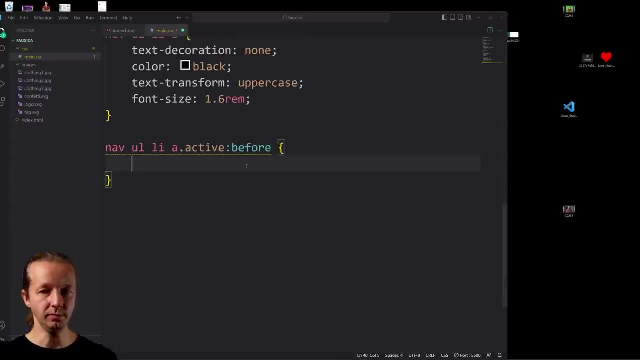 And then what we say is: the pseudo element is before, So you put a colon before. okay, Now, when you do this sort of thing, like you're adding extra design accents, we're going to do this as well with the confetti graphic that showed up. 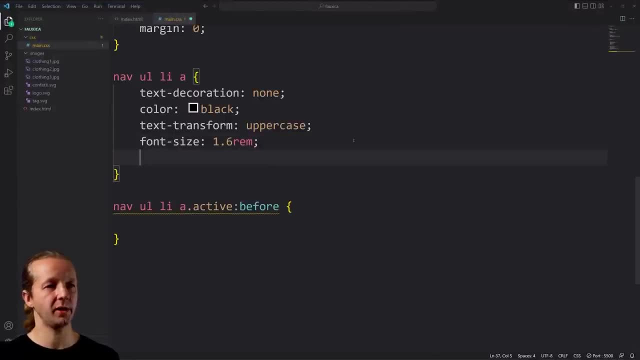 When you do this, the parent element up here, we say position relative. Okay, Position relative. And I'm not going to describe what that does right now. I'm going to show you what it does in a second. So we put position relative on the parent and then the pseudo element which is attached. 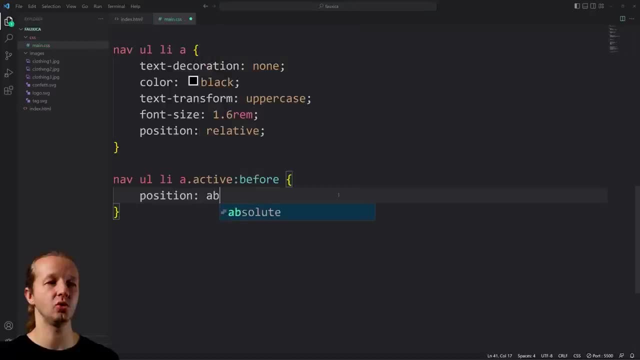 to it we're going to say: position absolute. All right, Now, just remember, I'm going to explain this in a second. I'd rather show you, though, And then what we do is put content empty. It's one of those things that these three elements, you're putting together pretty much. 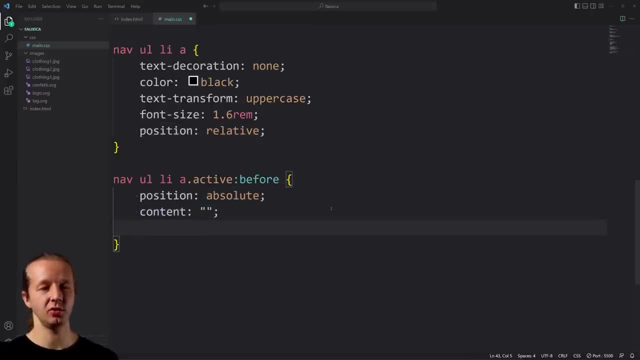 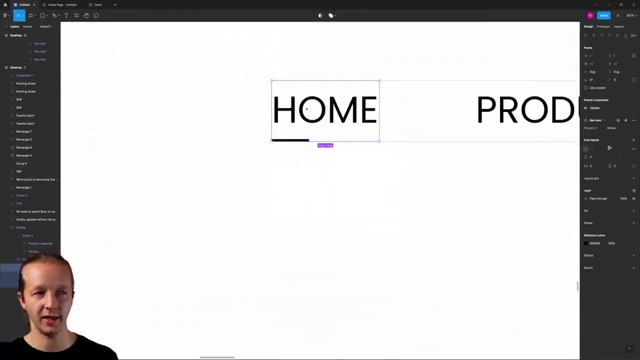 no matter what, All right, Then what we're going to do is give it a width of like 35%, because if you look at the design, the length of this thing is like 35% of the width of home. essentially, All right. 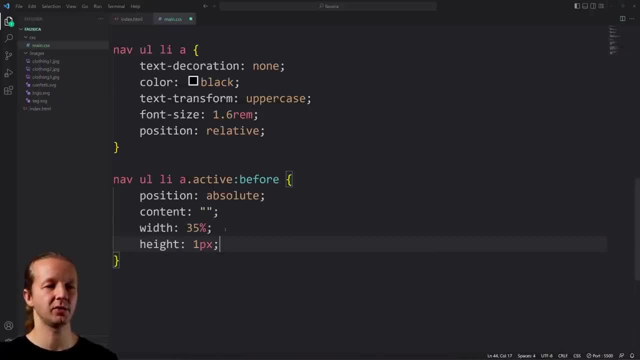 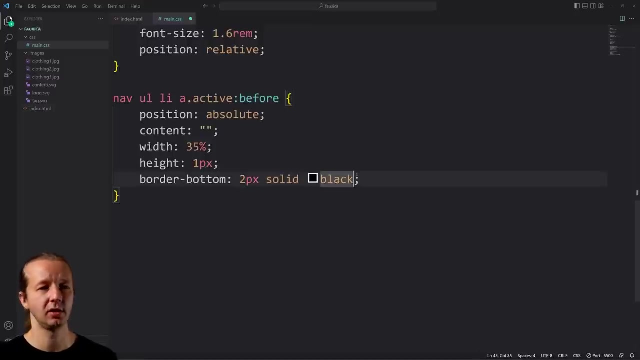 We also have to put: we're just going to do a height of like one pixels and then a border bottom of two pixels, solid black, All right. So that's how: we add a border to the bottom of two pixels. We make it a solid because you can do dashed on the lines and stuff like that. 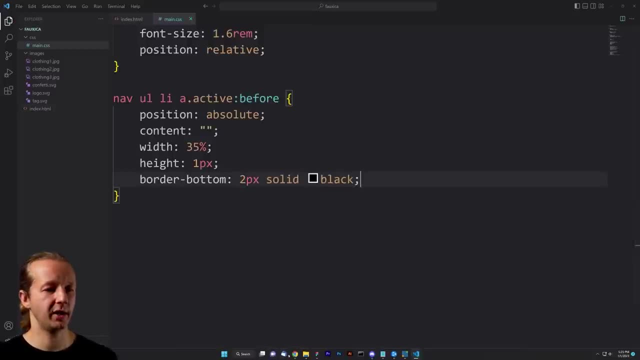 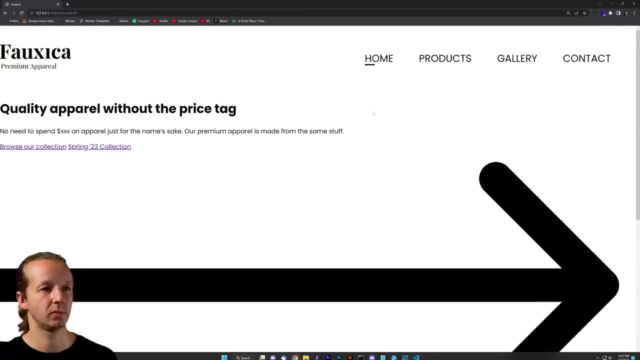 We'll save that And then let's go ahead and see if we see anything yet. Yes, we actually do. Right there, It's above it, We want it to be beneath it, So we say bottom, we can say zero. 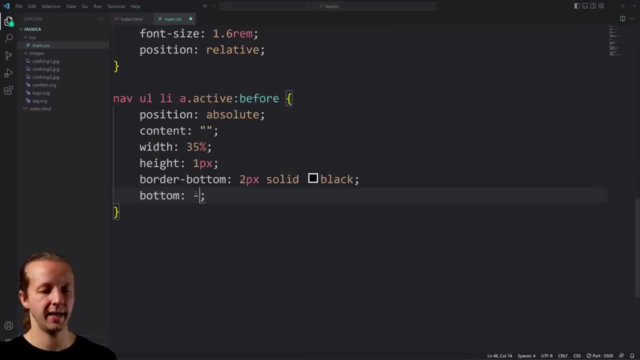 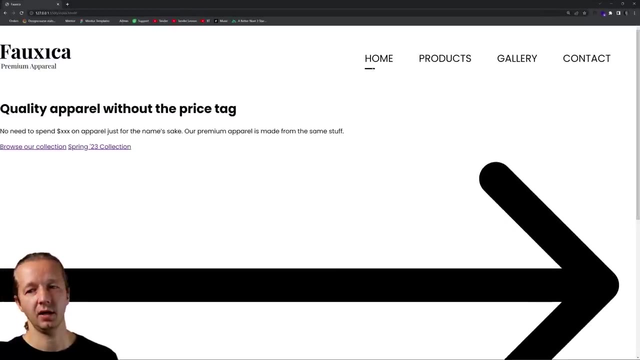 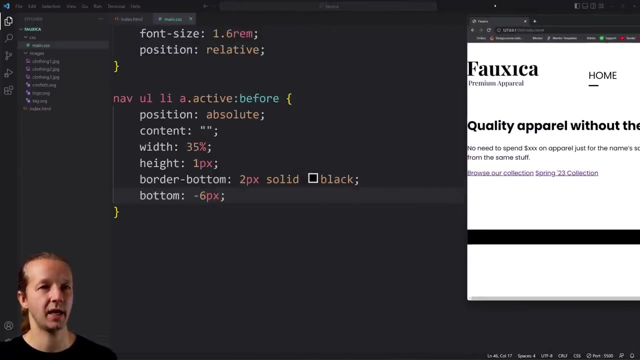 That looks pretty good, but we want it to be a little bit further. So negative six pixels, All right, Just like that, All right. So that was confusing. What happens if I remove position relative? Let's put this off to the side. 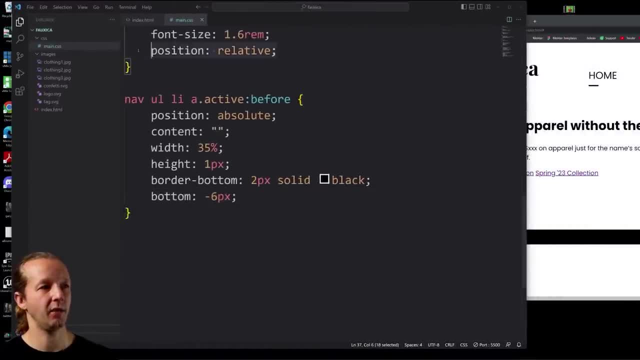 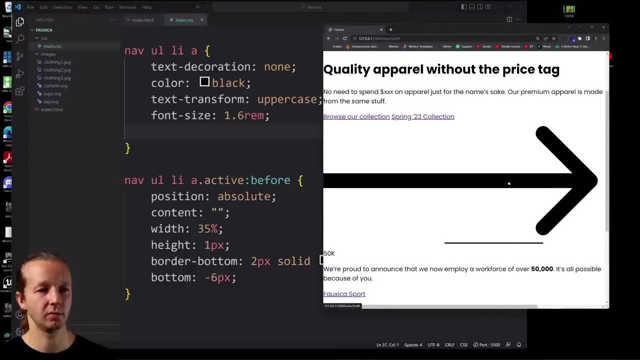 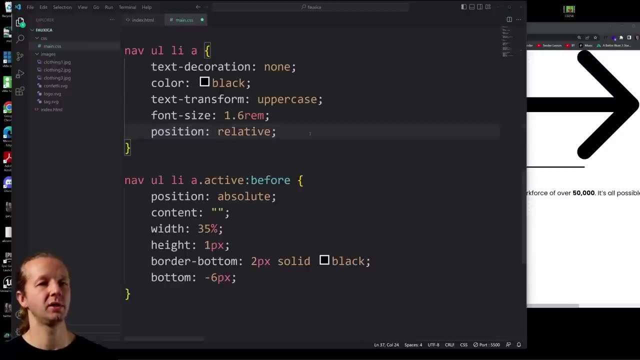 We'll drag this right here and I remove this position relative. Well, it disappears. Where did it go? It's right there, actually right here. So position relative simply: Oops, Don't do that, Gary, There we go. Position relative simply means that this position absolute is zero. 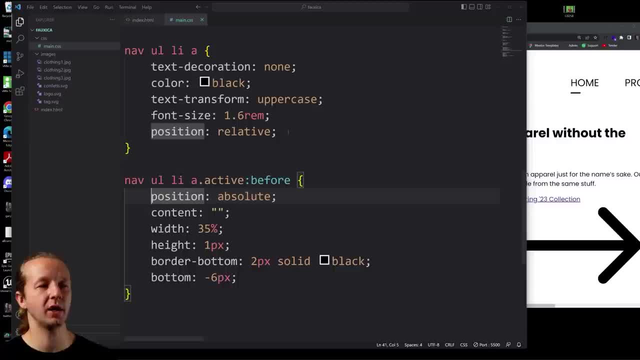 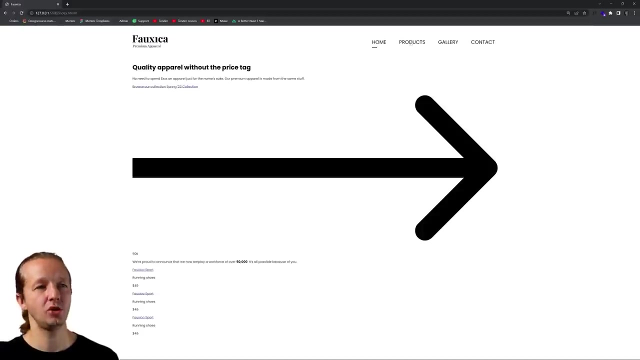 All right, So this position, absolute element- will be in relative. Its position is relative, based on this element, its parent element, container, if that makes sense. Hopefully that does. All right, So that's how we do that. Okay, Now continuing on. that is all the HTML markup that we need, almost, except we do want to. 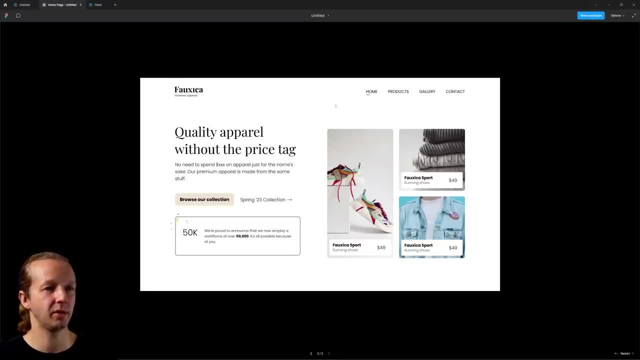 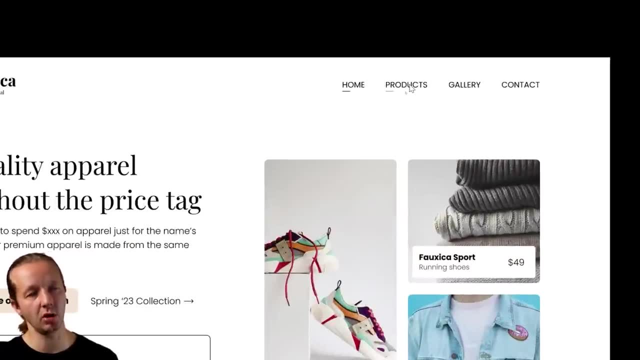 have. And let me go back to this and play the Figma prototype. Okay, So if we zoom up when we hover over, you can see how the little- I'm not sure if you'll be able to see it well in the video. 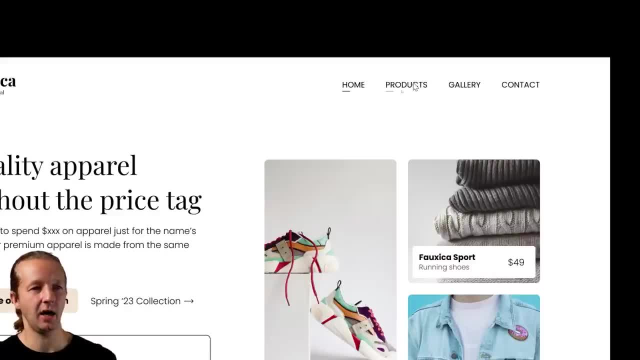 It's so small. There's little borders underneath it. They're gray. They animate in. We're going to tackle that at the end, when we get to the micro interaction section. So for now, we're good with this section, All right. 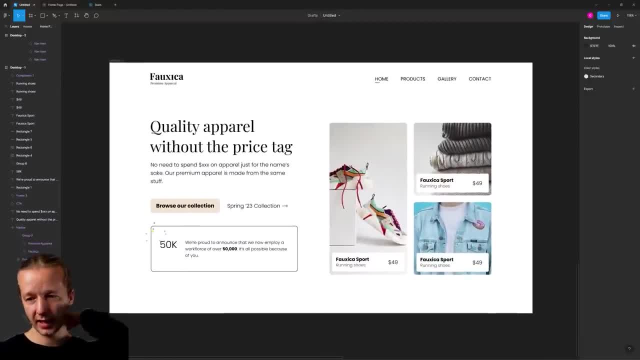 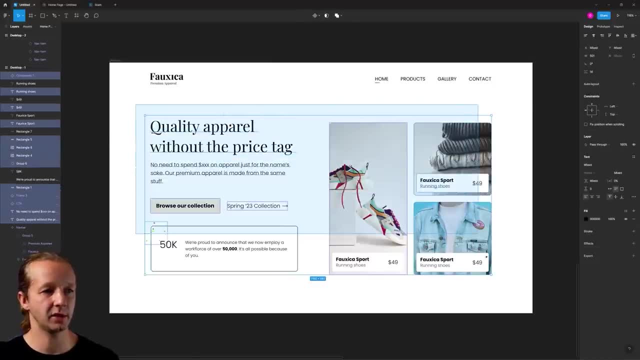 So let's go back. What is now the next element we're going to start designing? for It is our hero section. Remember, our hero section has this element. We're going to go back and see what it is. It's this element, called main, that wraps around those two columns. 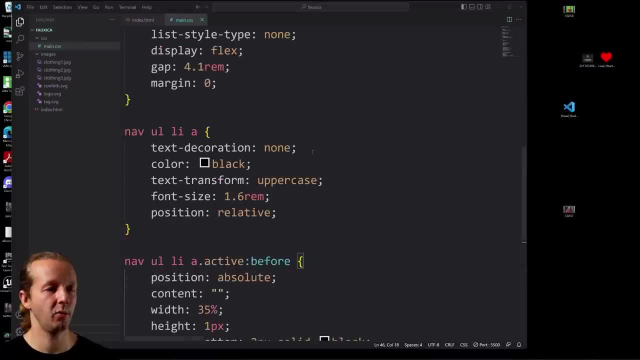 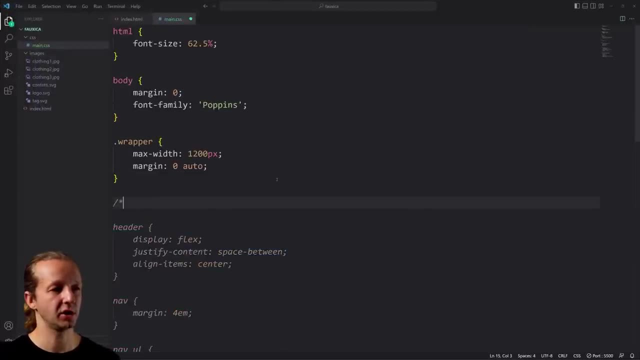 So we're going to target those And, by the way, it would be a good idea to get in the habit of adding comments in your CSS. So, forward, slash, asterisk, We can call this the nav bar, And then we uncomment by just reversing. 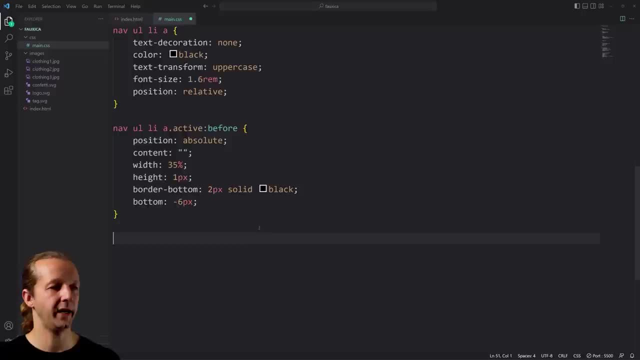 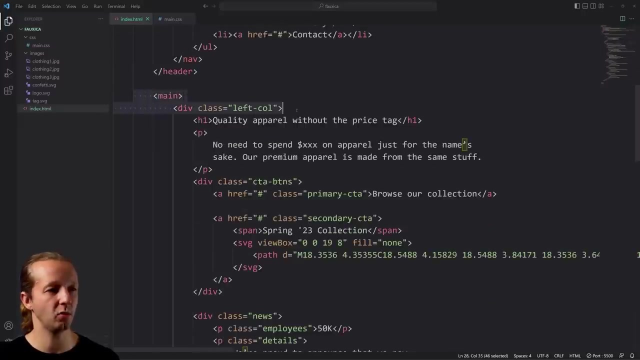 So asterisk first, then forward slash, So then after here we can do the hero section. Okay, All right, That's looking good. Save that. And now we have. if we refer back to our HTML, we have main right here with two elements. 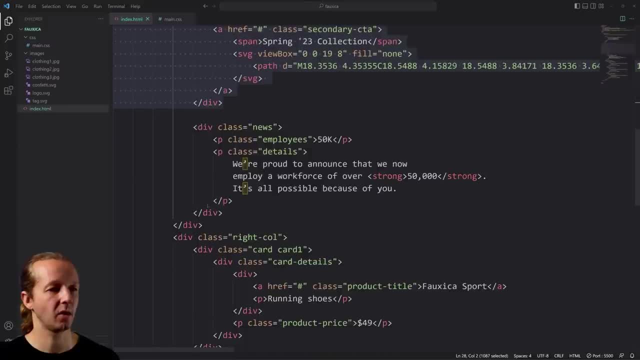 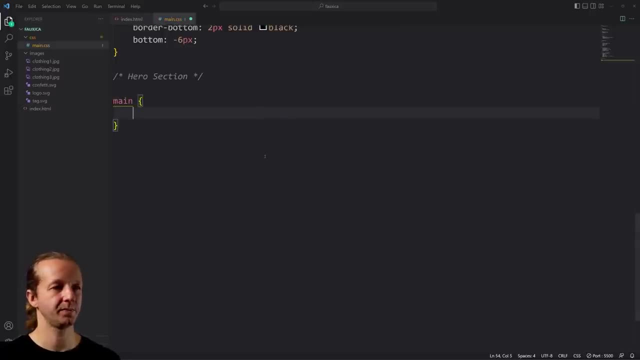 inside of it A left call. Oops, The left call is all the way from here to there And then the right call. All right, So main, We're going to specify. Remember we have two. We have a left call and right column that need to be in column format. 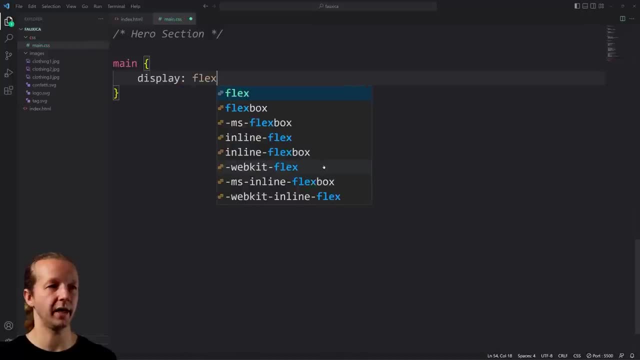 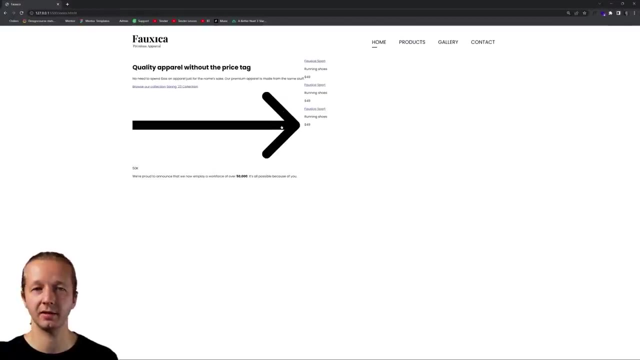 What do we do? Display flex? So display flex, That should alter our layout quite a bit And it did Notice how the lines, the arrow's, smaller and we have our right call stuff right here in the right column. See how things are starting to come together. 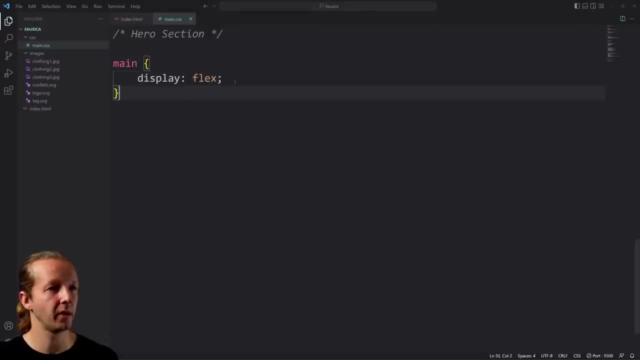 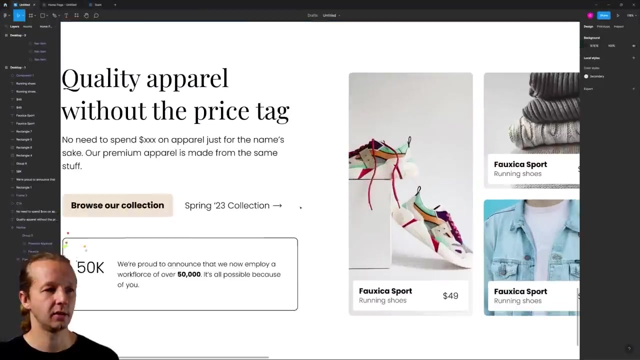 It's very exciting. You can make money doing this. It's unbelievable. So we're also going to put a gap, or white space between them. If we look at here, We can see that. Okay, So you can see this. There's a pretty sizable gap between these elements. 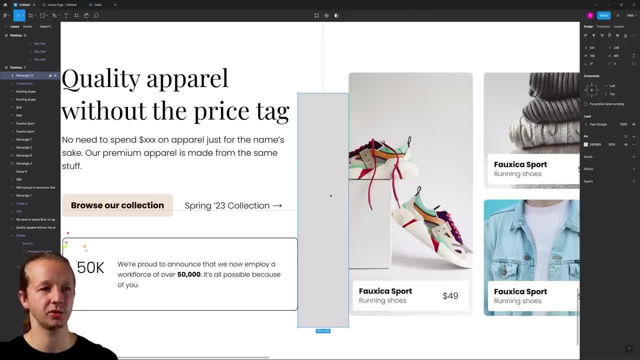 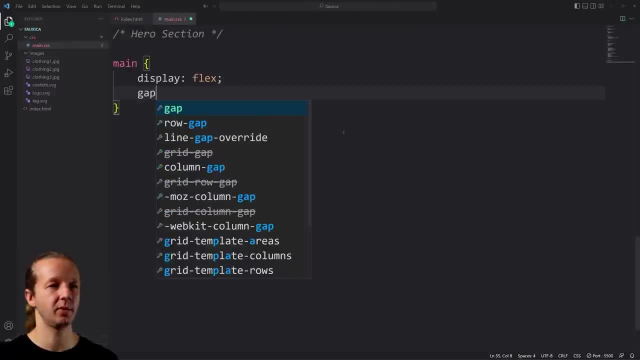 It's like the width says 108 pixels or so, So that would be 10.8 REM units or something like that, or M units. So what we can do is say gap. We'll just put eight M units and you'll notice it creates white space between them, right? 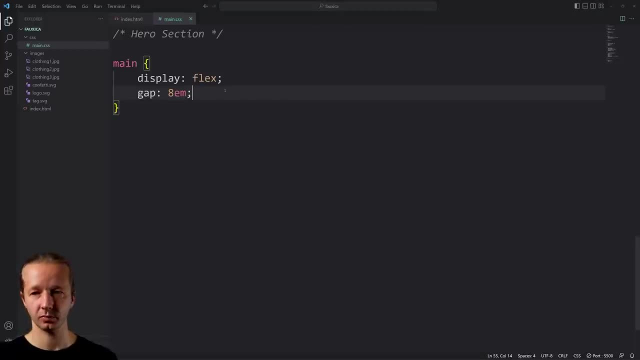 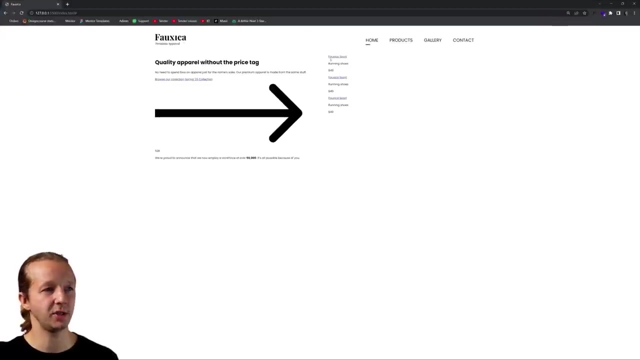 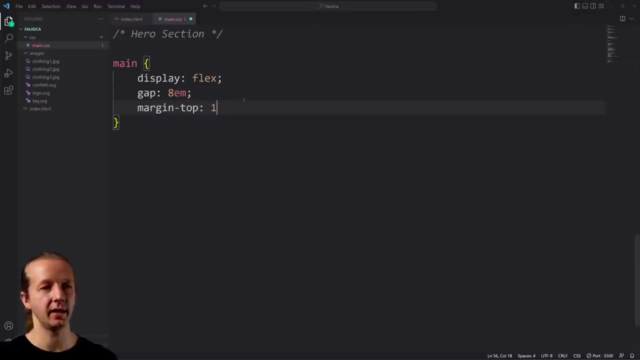 there. All right, Now we're going to also move it away from this nav bar. We need more white space between this elements with margin top, margin hyphen top, And we're going to give that a 11 M units. 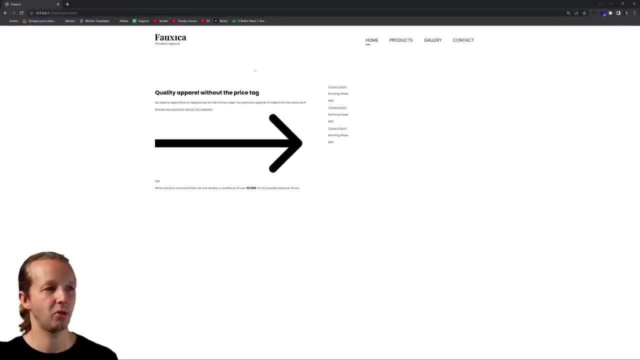 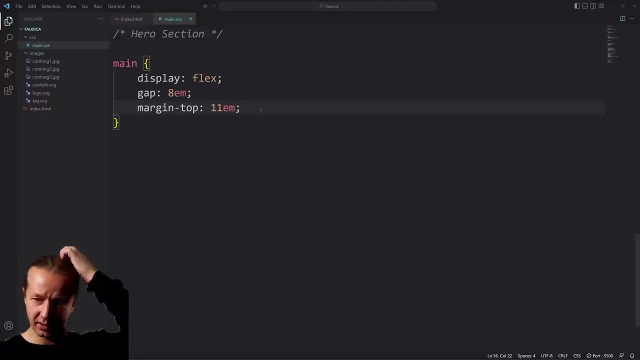 So 110 pixels essentially. Now it's been pushed down quite a bit. After that, we're also going to go ahead and specify our left call and we're going to give this a width of 45%. I'm going to save it. 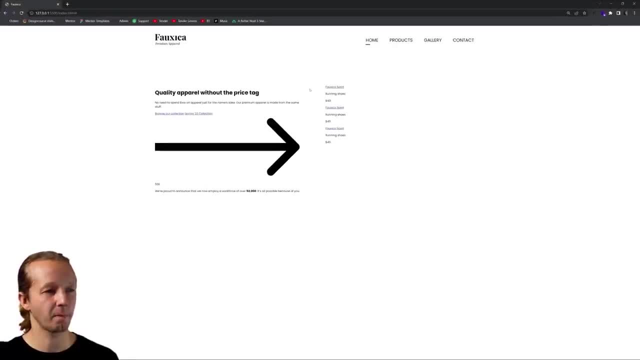 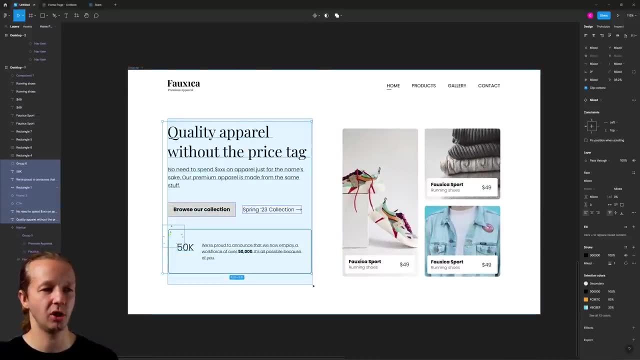 Okay, All right. So if we look at our design here, this is basically 45% or so of this available space within that main parent container. All right, So that's why I gave that 45%. And another thing to pay attention to is we want this stuff to consume. right column like: 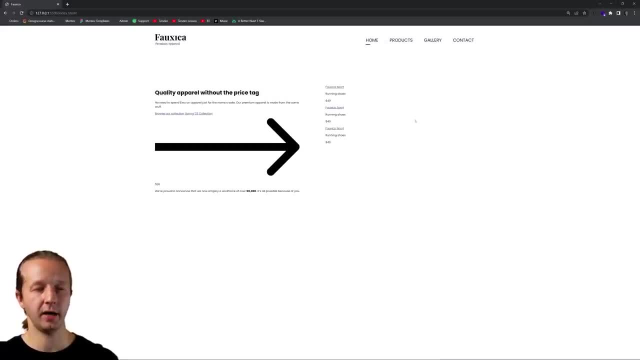 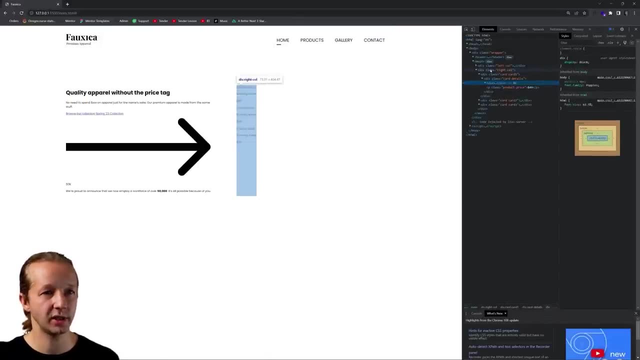 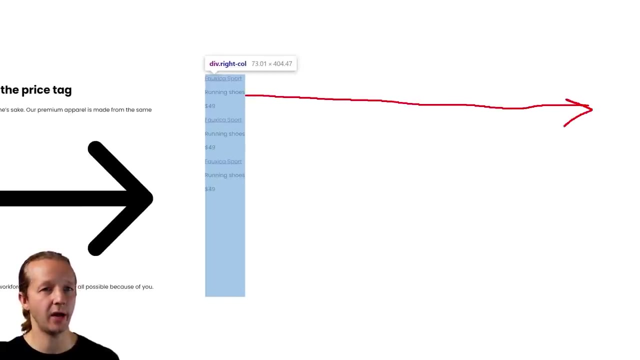 these three pictures. And right now, if we get out our Our F12 dev console area and we choose this section where it says right call, Look how small that is over there- It doesn't extend all the way out. We want that to extend all the way out to this section, right here. 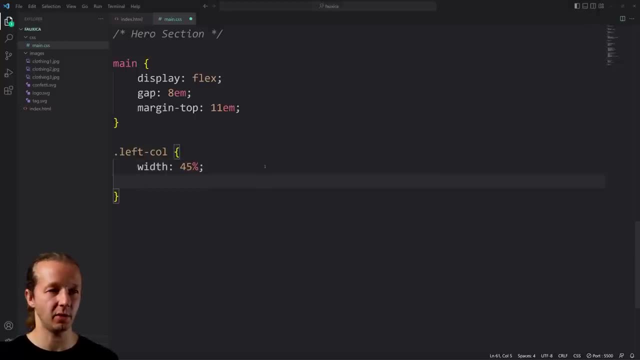 And we do that with a property and it's based on flex box. This is a flex item because it's parent is a flex box container. We say flex. Oops, sorry, I put it in the wrong rule set. We're going to do right call because that's the one we're working with now. 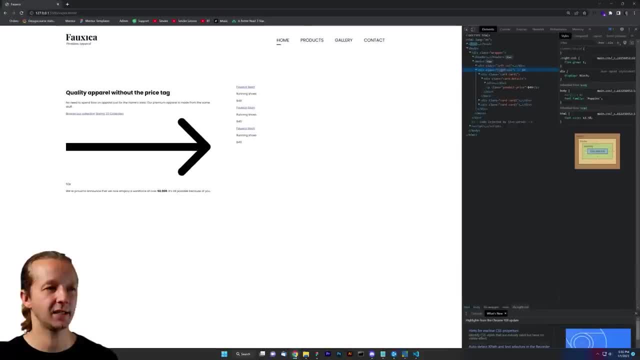 Flex grow one. If we save that, the design itself isn't going to change. However, if we hover back over, look how it opened that up. So the default behavior for flex box items is it's only going to consume the amount of. 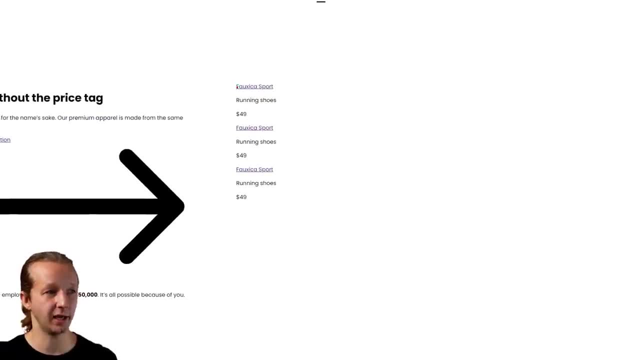 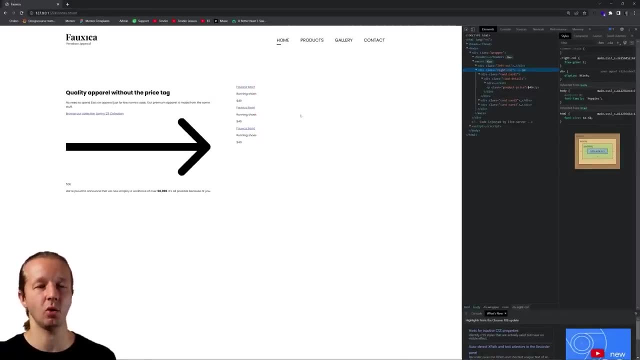 width it needs, based on the content that's inside of it. So that's why initially it was only this big, But we need it to be to fill out the whole available space. So you use flex grow one. Hopefully that makes sense, All right. 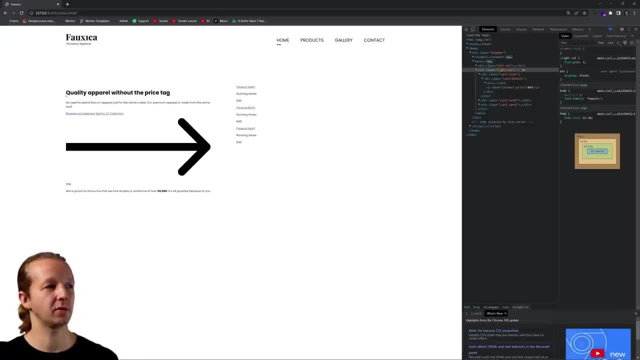 So now we're going to focus on our H1 element, because that does not look anything like our design. So we're going to take our H1 font size. Again, how do we do font sizes? Well, we come over here, we select it. 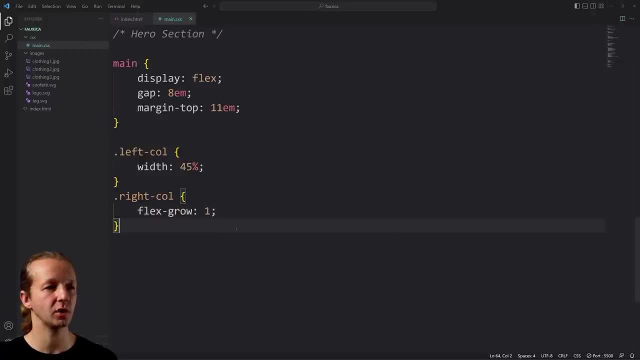 We say, ah, it's 52,, 5.2 REM, That's what we want. So 5.2 REM units, And again, this is going to make it a little bit more complex, So we're going to do this. 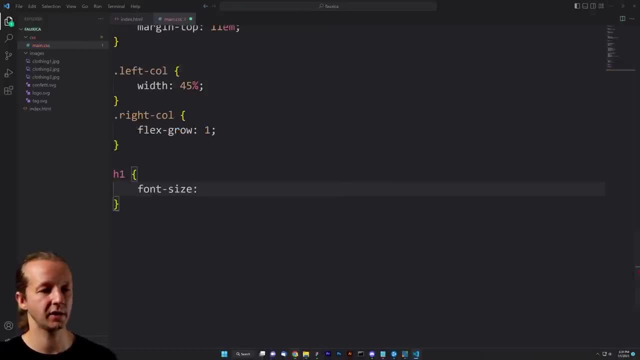 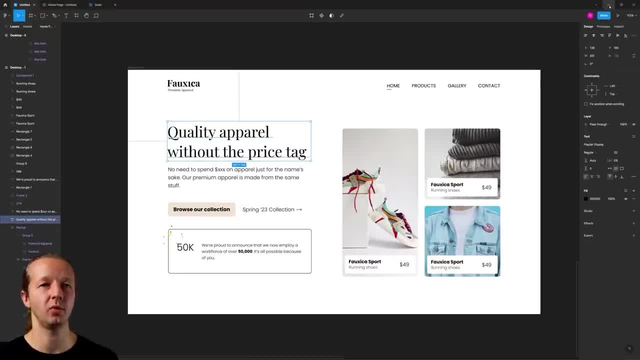 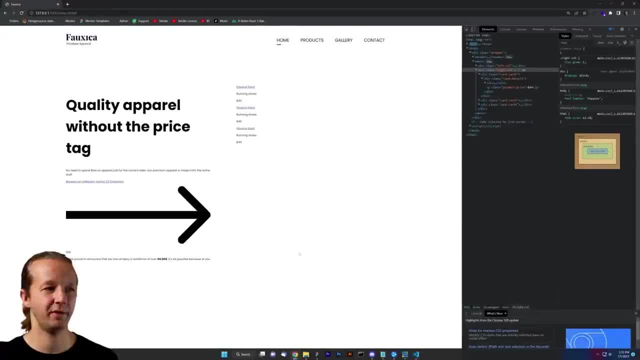 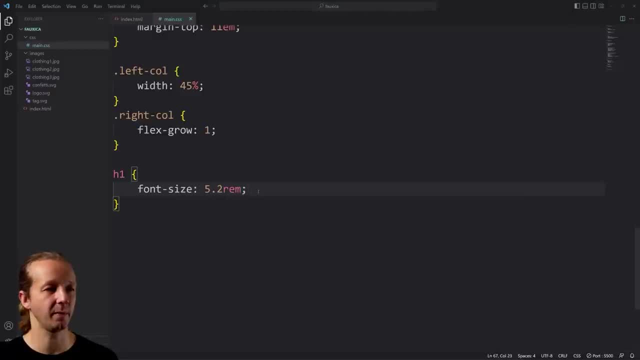 We're going to do this And again, this is going to make it big and beefy. There you go, Quite a bit bigger, but it's also the wrong font. We're going to use Playfair display for the first time. 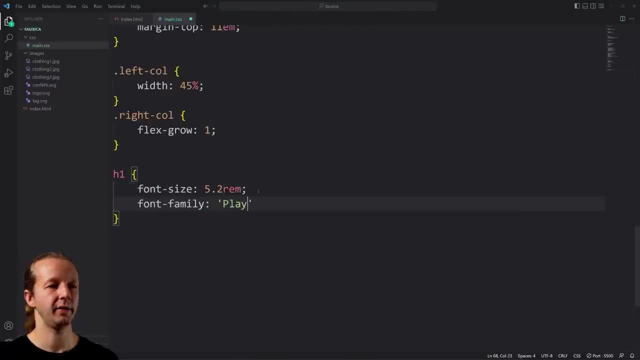 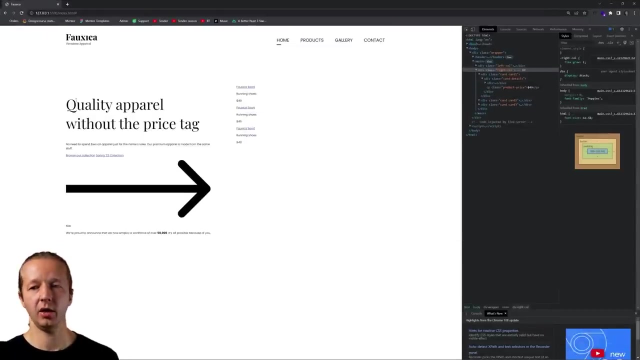 So we say font family Playfair display And then we also say font weight normal because it's going to make it bolder by default. Okay, And let's look at this. There we go Looking much better And also notice if we click on this. 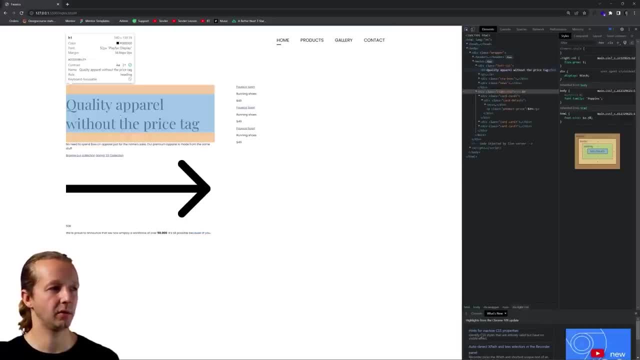 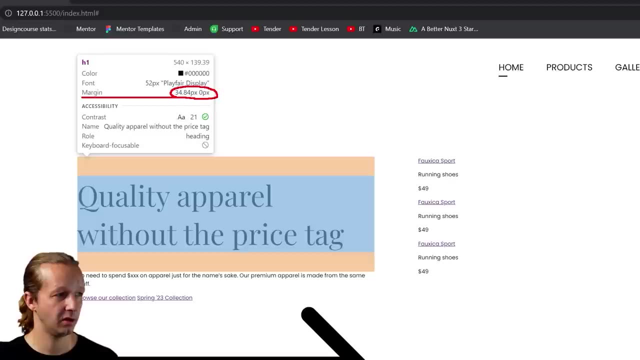 notice that orange stuff. Now if I zoom up, it's telling us the margin by default is right. here It says 34.84 pixels, And so the margin will be adjusted programmatically by the browser based on the font size. So it's adding a lot of margin around it And I don't want that margin there. So 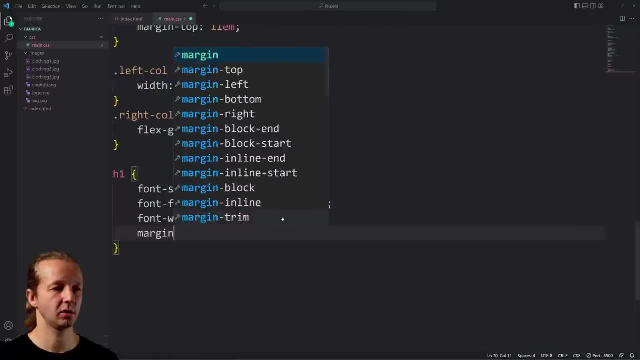 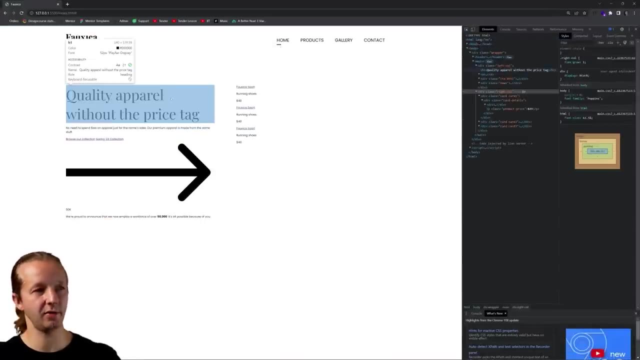 we reset it to zero. So we say: margin zero, Save- All right. And now, obviously those orange little indicators went away, because there's no margin now, All right. So now let's go ahead and focus on the subheading, which is right here. this tiny text Again, what is the font size? We click it. 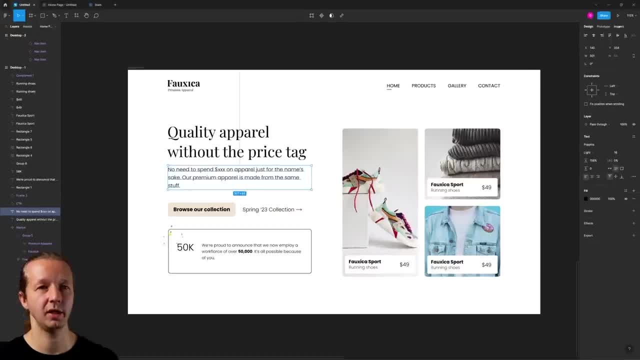 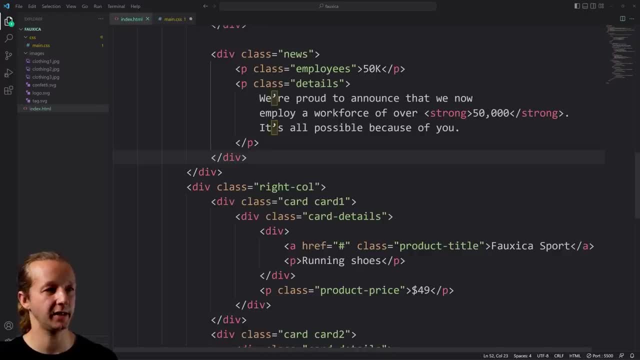 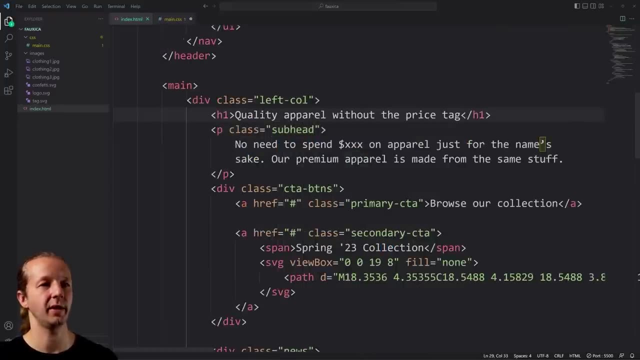 It's going to be 1.8 rem units, So we gave that a class, I believe, of subhead. If we didn't opt at it, it is: Oh no, I didn't add it. So we have to add class subhead for subheading. 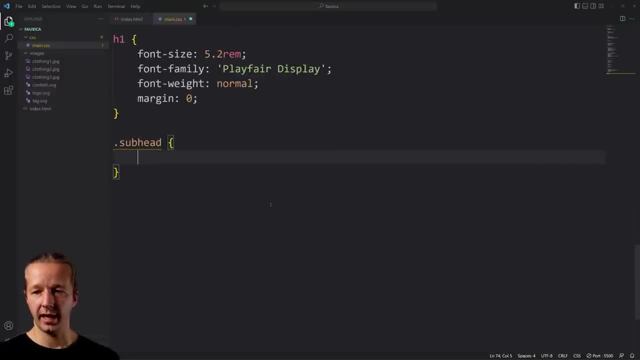 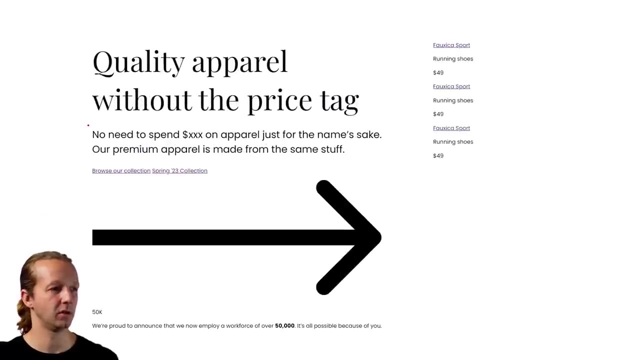 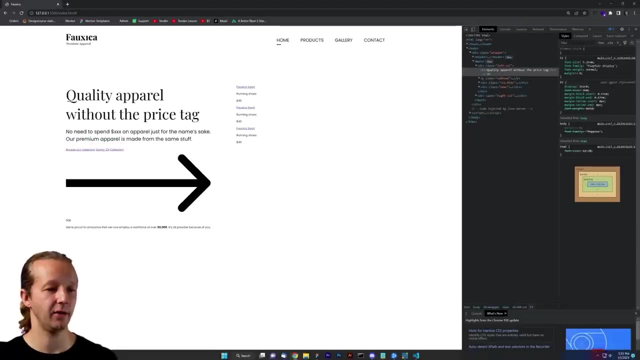 And then we're going to specify a font size of 1.8 rem units. Now it's going to make it quite a bit bigger. There we go Looking a lot better now. Now we have to worry about this section. This looks nothing like our design over here, Oops. 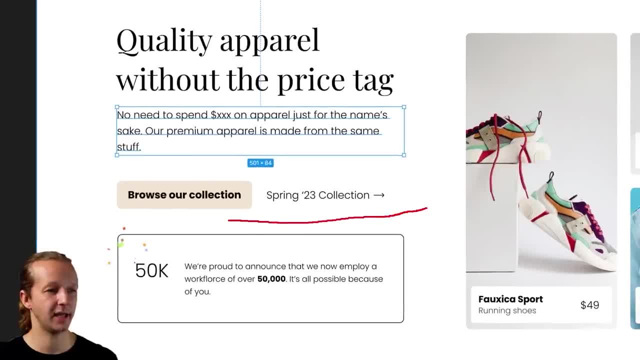 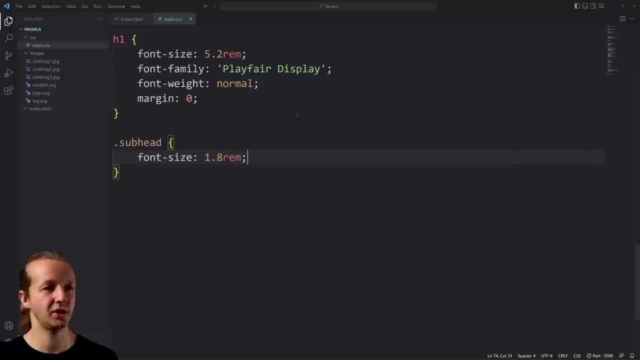 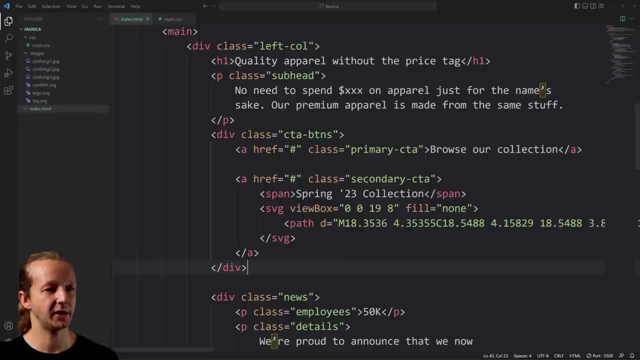 I'm clicking on the wrong thing. Yeah, So we need to translate that into looking exactly like this: essentially Got our work cut out for us, Okay. So if we refer back to the HTML, we'll see that we have our call to action BTNS, which has two elements inside of it. 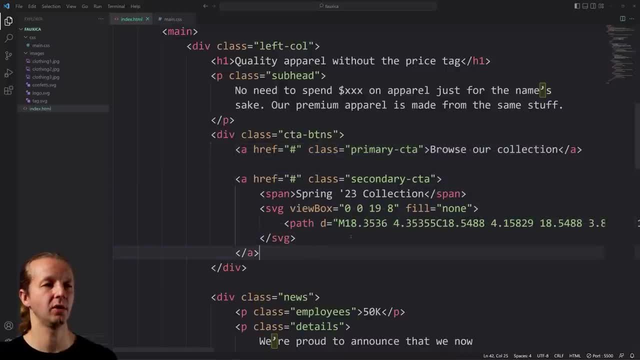 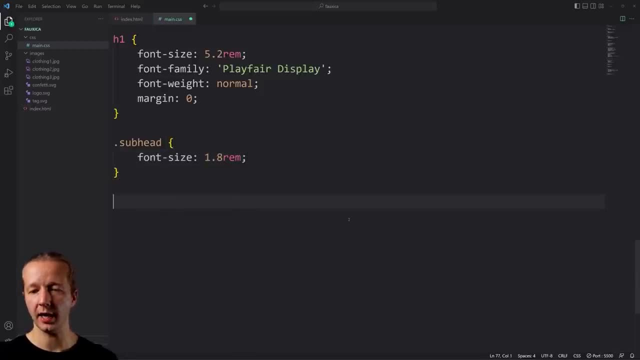 the browser collection button and the second secondary button right here, So you remember, two columns- means display flex. So we're going to say our CTA hyphen, BTNS, is going to be a display flex, with a gap of about 20 pixels. So two M units. 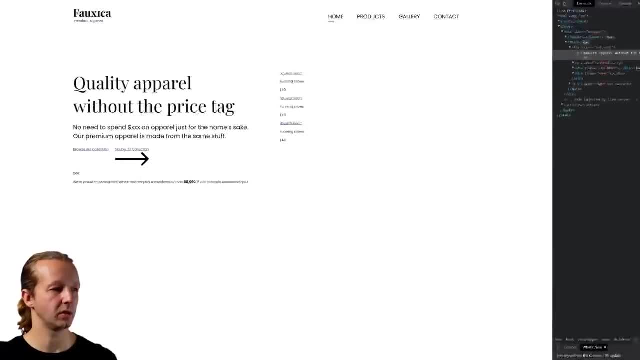 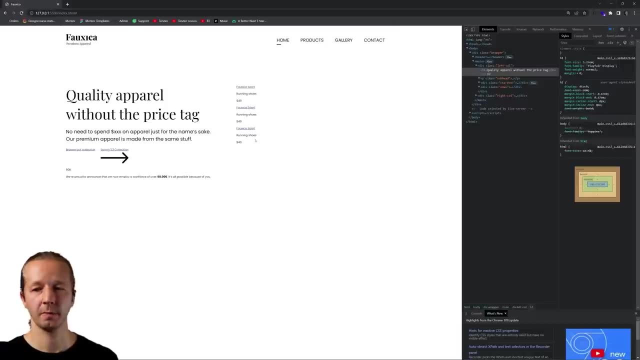 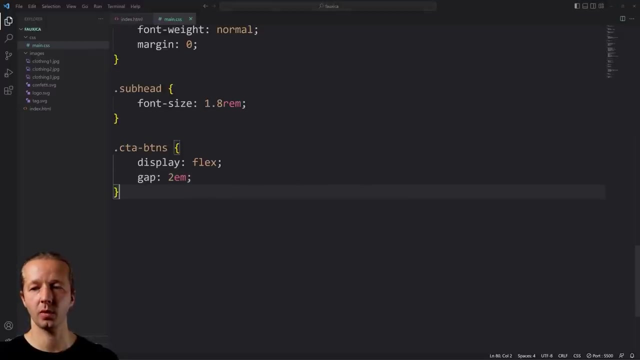 All right, Let's save that. All right. There it is. Browser collections right here, And then the secondary is right there, Additionally. now, let's, let's, let's focus specifically on browser collection and getting that one working. So now we're going to specify our primary CTA and that's the class we gave. 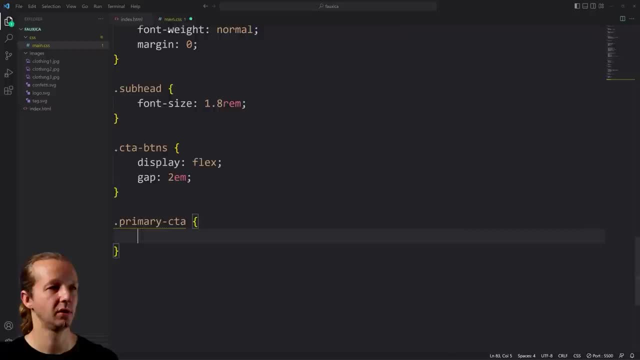 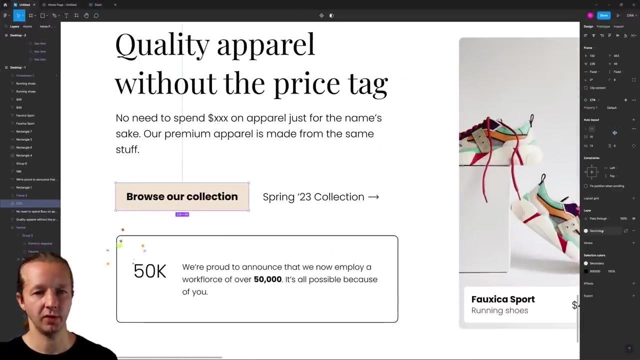 our primary CTA button right here, browser collection. So for primary CTA, we're going to give it that background color. So we're going to say background color, We'll go ahead and grab that color, So we select it and then we'll see over here we have this thing called secondary. 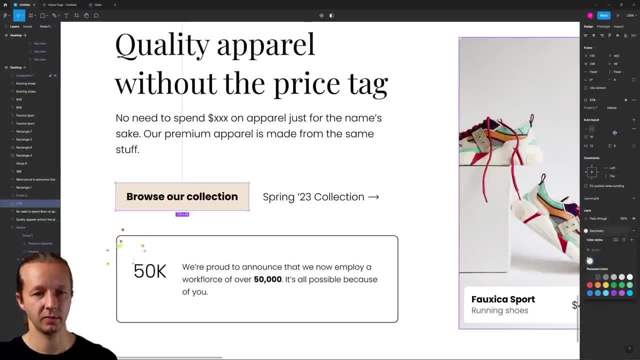 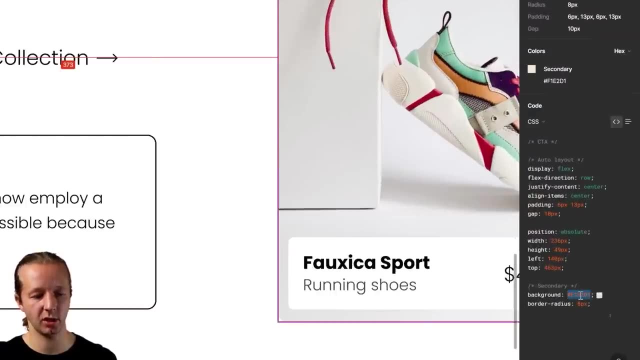 right there. So if we click on that and choose edit style, or instead we can actually go up to inspect tab on the upper right And it's going to tell you or show you the CSS property right there, This is the hex code that we want. So we just copy that and select it and copy, and then we just 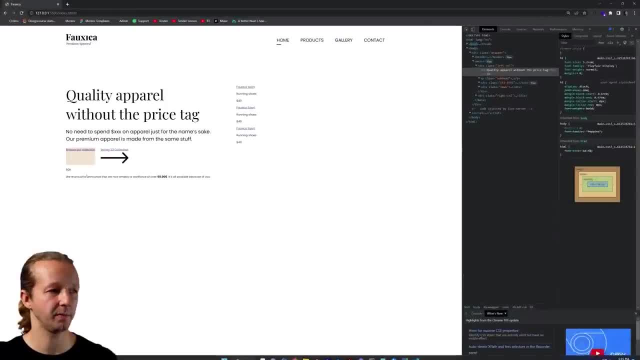 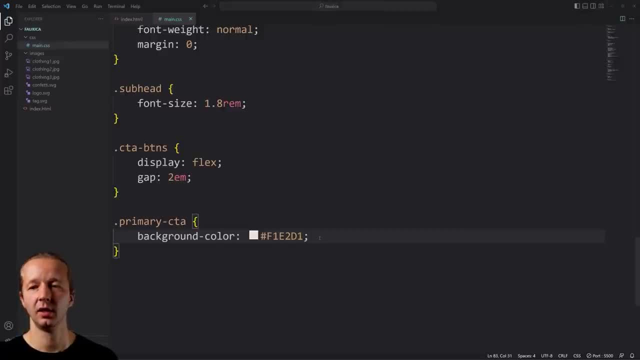 paste, So we save it and we're going to see that background Color right here. but boy, does that look ugly, right? So we still have some CSS properties to get it looking correct. So we're going to give it a font size, because it's 18 pixels. 1.8 rem units. 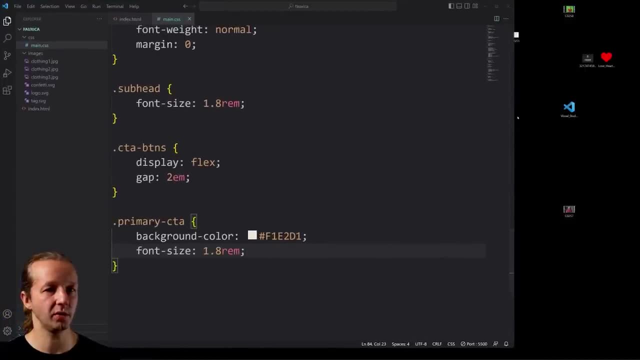 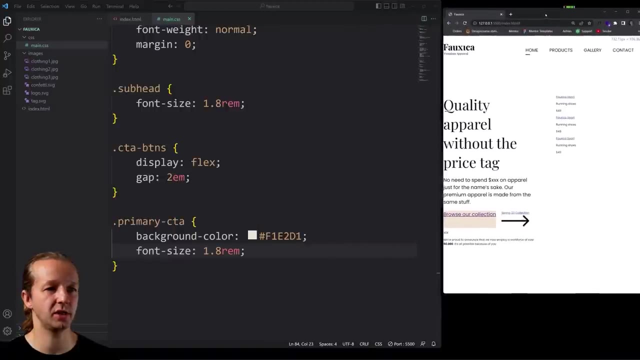 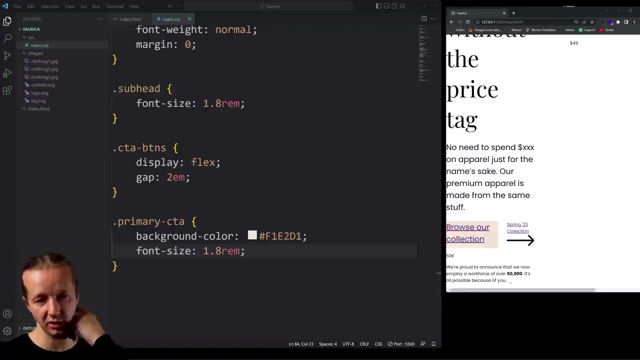 And you know what. It might make sense to move this over here, All right, And then we're also going to get this up, just so that you can see. see this start to shake, Take place and shape as we start designing or adding properties. Font weight's going to be bold. 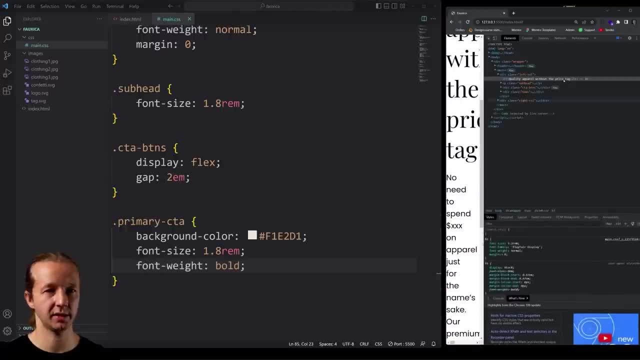 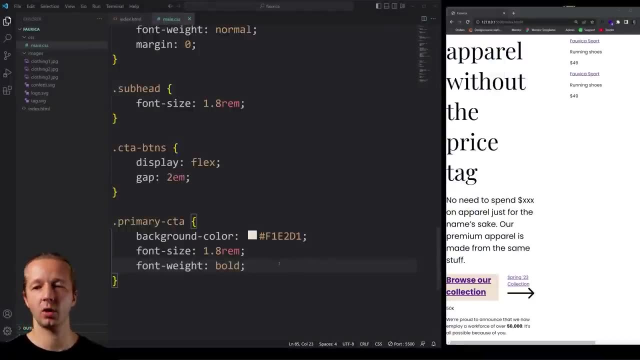 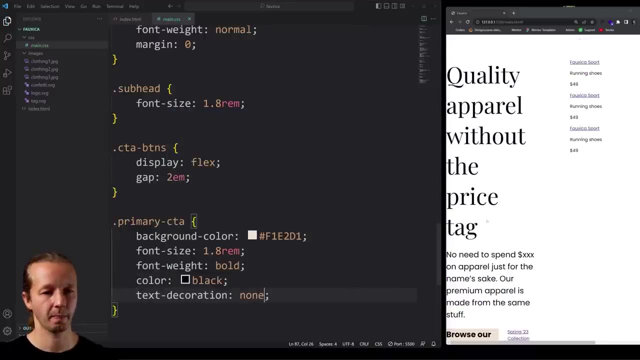 All right, Here let's increase this. Get rid of that F12.. Sorry, I'm hitting wrong keys over here. There we go, And then we're going to also say: color black text decoration: none Okay. And then we're going to give ourselves some border. 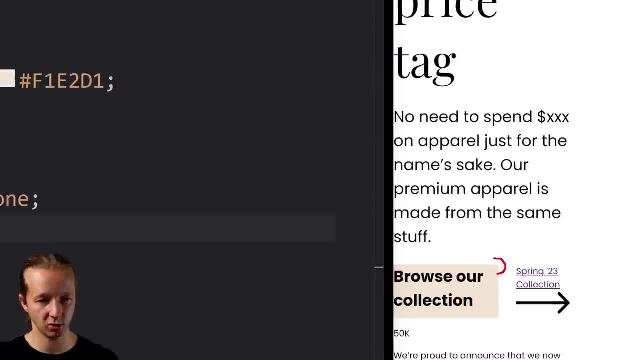 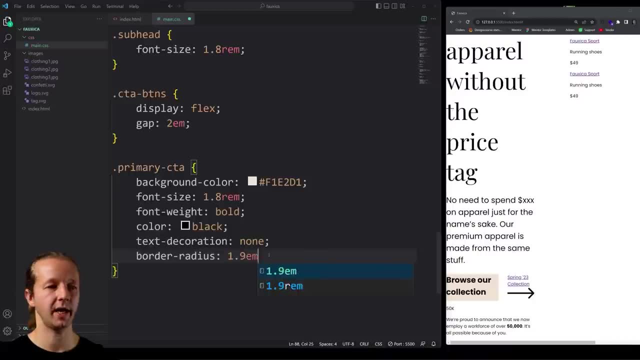 border radius on the edges. Notice right here they're just right angles. So we do a border radius of 1.9 M units, because it's 19 for the value of the corner radius in Figma. You can see right there. And then we're going to give it a padding of 1 EM on the top. 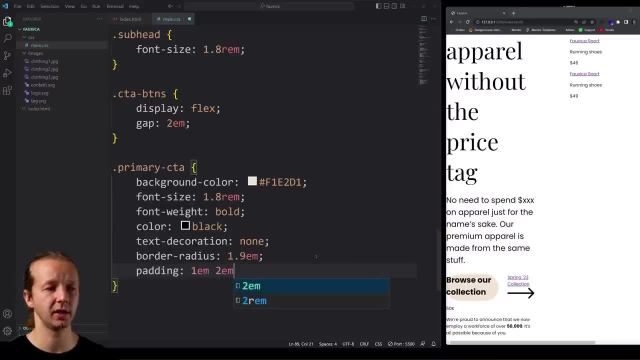 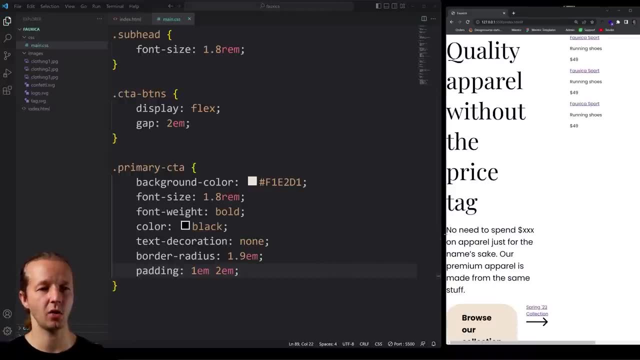 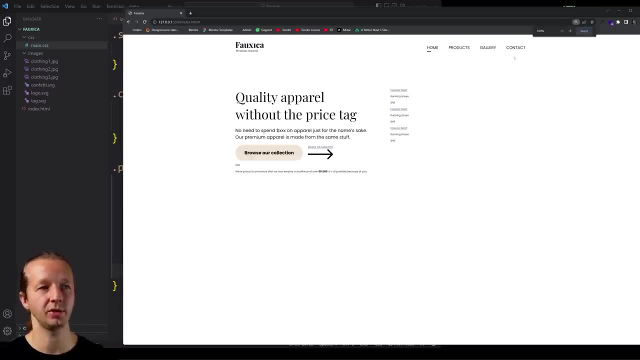 and bottom and 2 EM or 20 pixels on the right and left. Padding is white space working on the inside of a container. So this button, we want to add more padding around. So if I bring this out, we reset this browser zoom to 100%. This is what yours should look like right now. 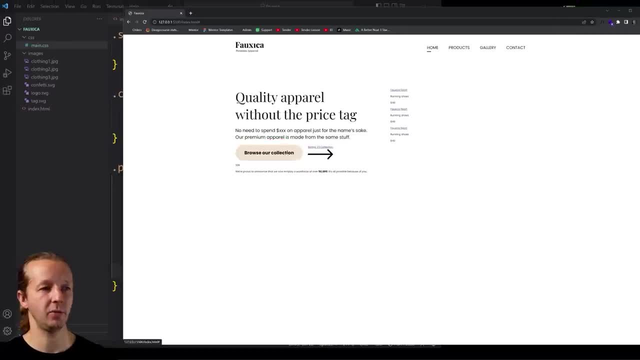 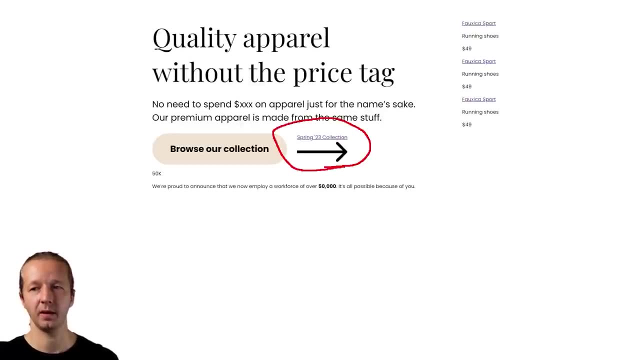 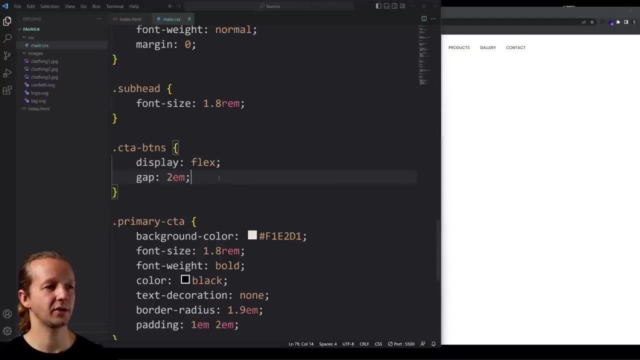 Notice how it's centered, looking good and pretty much exactly like our Figma prototype. Now this obviously needs work right here. All right, So what we're going to do now is we're going to refactor a couple things. We're going to not necessarily refactor. 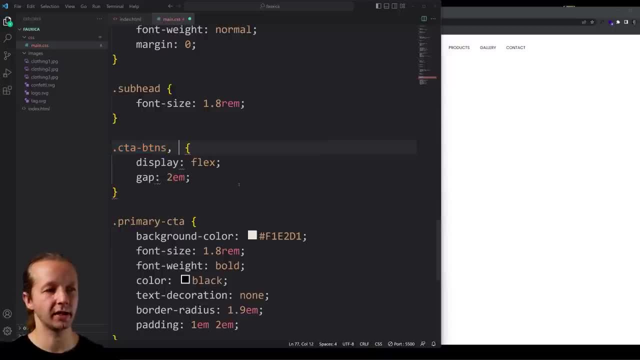 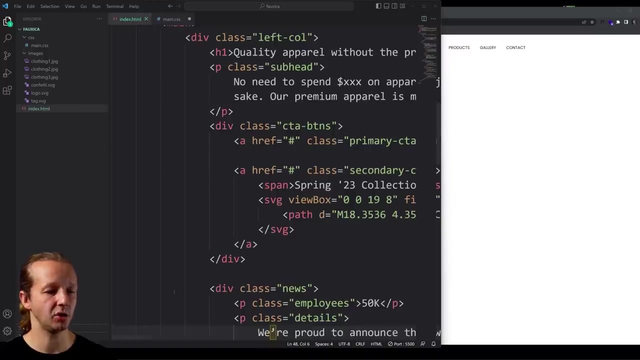 but we're going to add another selector onto this rule set called secondary CTA, because it needs these exact same two properties: a gap of two M units and display flex. And the reason we're doing display flex for secondary CTA is because, if I show you the code, secondary CTA has two. 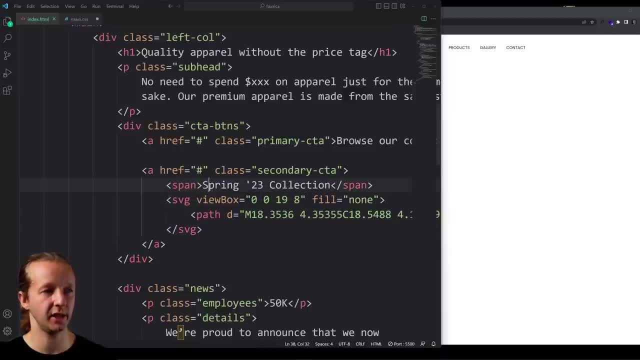 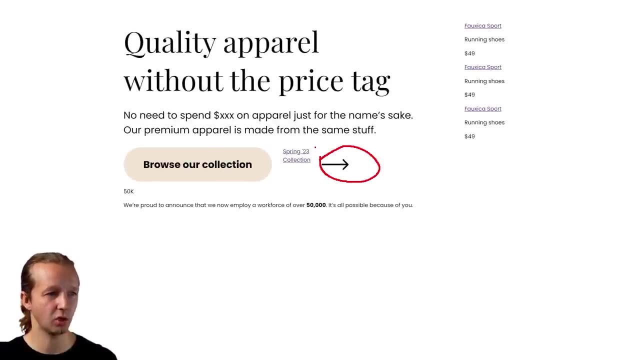 elements that need to be in two columns: the span and this SVG. So, going back here, we save that and look at that, They are now into two columns, but we still have work to do because it still doesn't look good at all. So now we're going to do target, our secondary CTA. 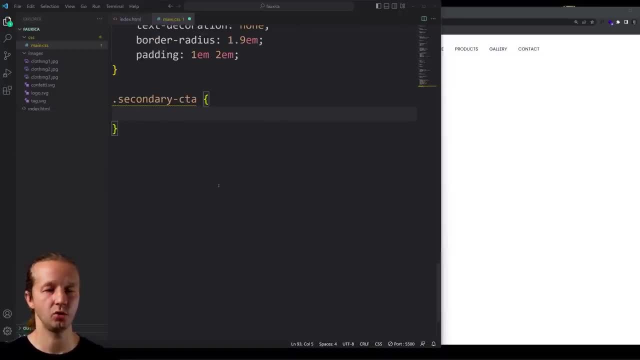 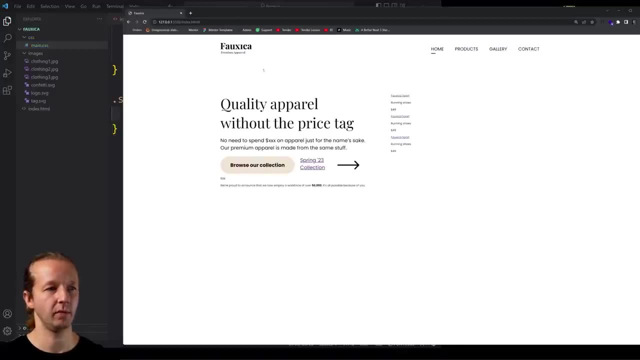 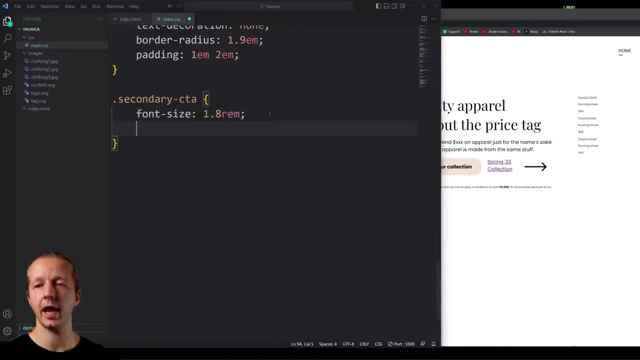 All right, And for that we're going to specify a font size again of 1.8 rem units. Might as well just move this over so you can see it while we code. All right, And then also a text decoration of none. 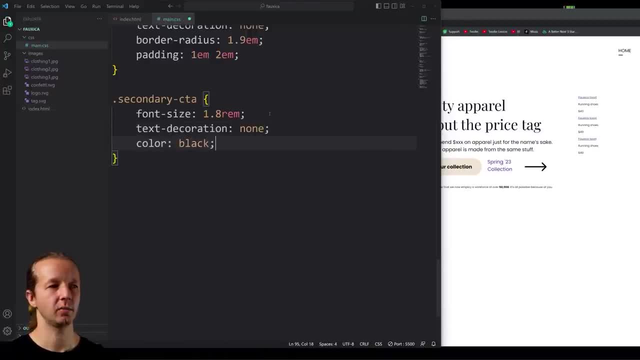 color black And this right here we're going to put display block, because right now it's on two lines and we don't want that. Putting display block will ensure that the words don't wrap in a sense, And then we're going to put display block. And then we're going to put display block. 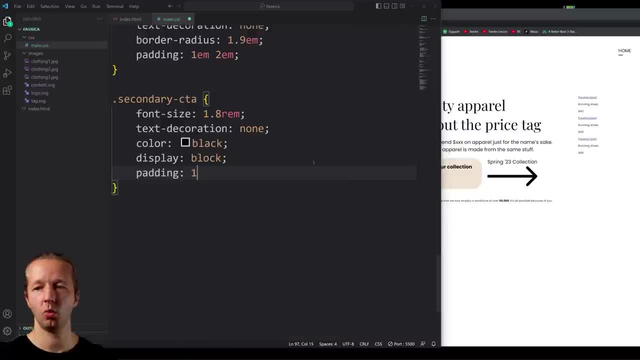 And then we're also going to specify a padding of 1M on the top and bottom and zero on the right and left. Now our SVG element. this is too big, We need to fix that. So we say secondary CTA SVG, because the element in HTML is called SVG, right here. That's how we select it. We could have given. 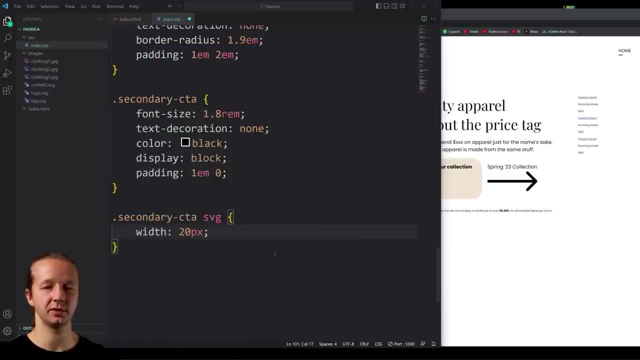 a class too, by the way. So with, let's say, 20 pixels. Now, remember, I said you very rarely want to use pixels. Well, you can use pixels if you don't care if certain elements have to scale up based on the 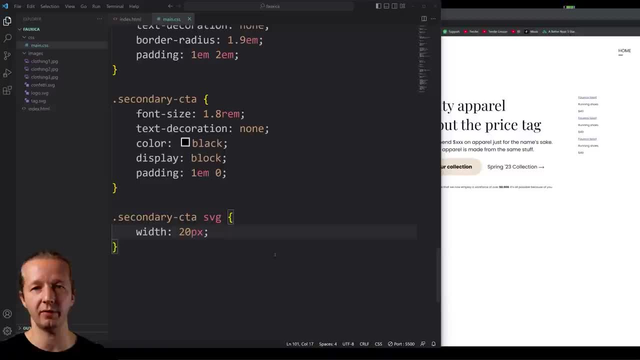 browser's or a user's zoom preferences for their browser. Some people choose to make their zoom preferences for their browser, like real large, but for an icon like this, I'm fine with it. staying at a static 20 pixels, No big deal. 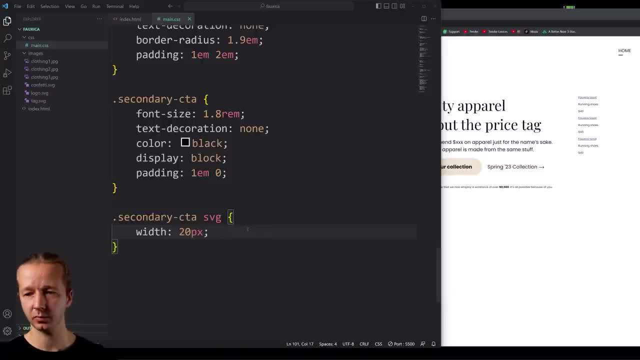 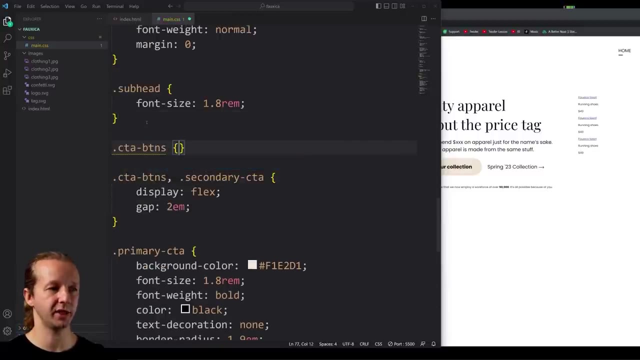 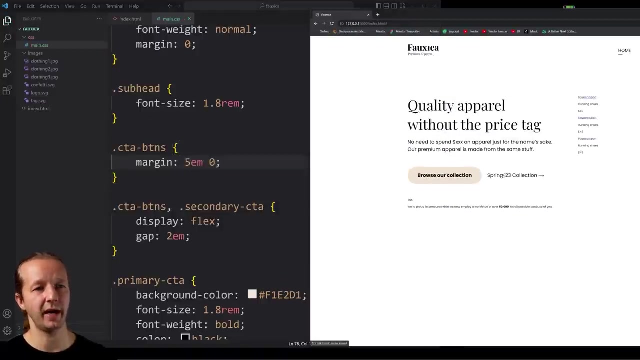 So for our width, or SVG, that's looking pretty good right there. One other thing I wanted to change or add, though, is we want to target CTA buttons just by itself in a rule set and say margin 5M on the top and bottom and zero on the left and right. That way it pushes itself out a. 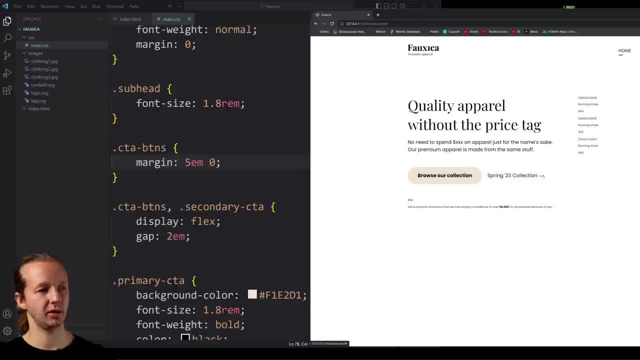 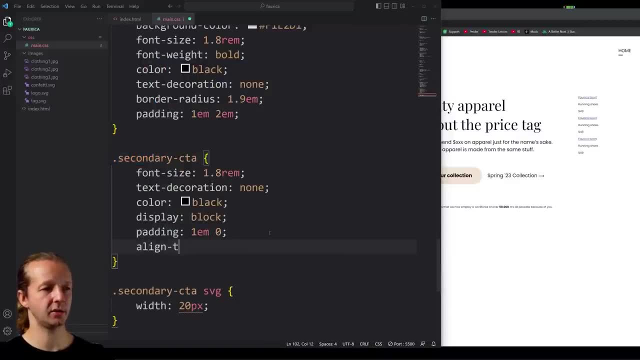 little bit more. Okay, Now that's looking real solid right there. Let's see Secondary CTA. Let's do align items center. I'm not sure if that changed anything because of this look like it wasn't perfectly vertically aligned. I just want to make sure I. 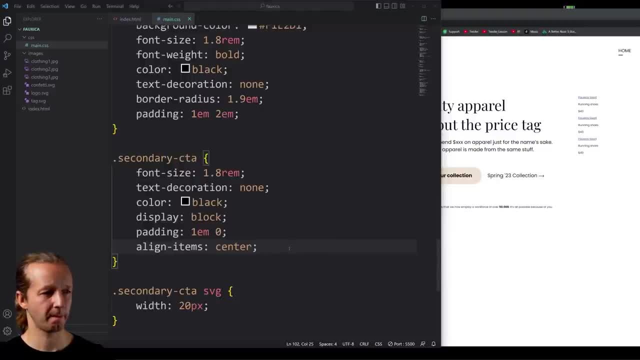 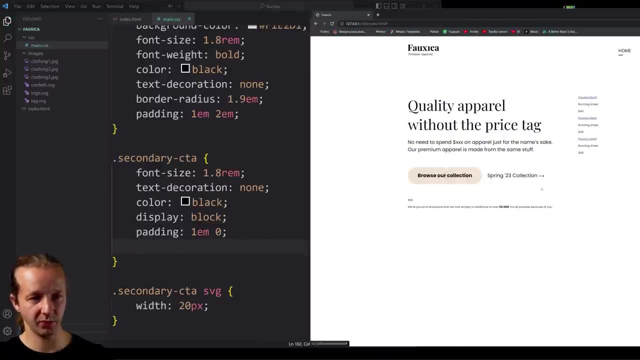 didn't screw anything up. Let's see if we remove this. If anything changes and it doesn't, we can get out our. let's see if we can get out our. let's see if we can get out our. let's see if we can get out our. 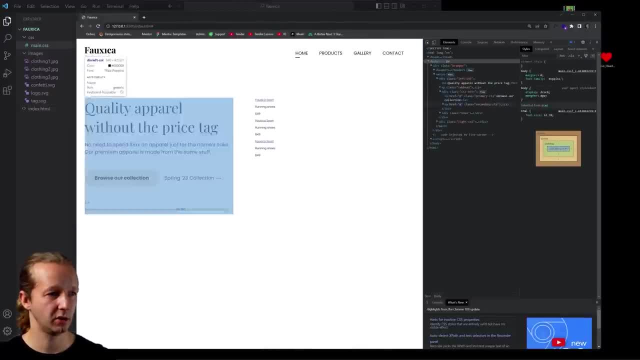 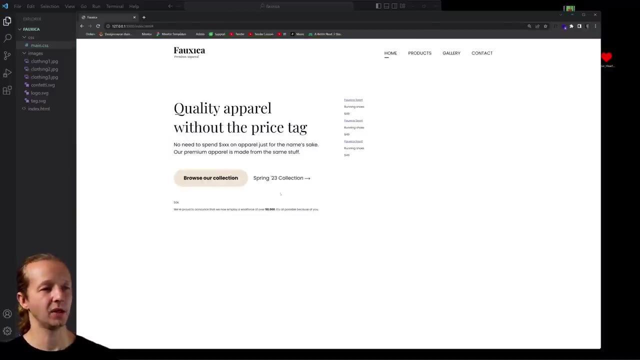 F12, our developer console. And is that being centered? It looks like it is. It just looks like it's off centered to me for some reason. Anyways, nevermind me. Okay, So we are going to make this so that when we hover over this, this will move over, This will animate. But again, we're going. 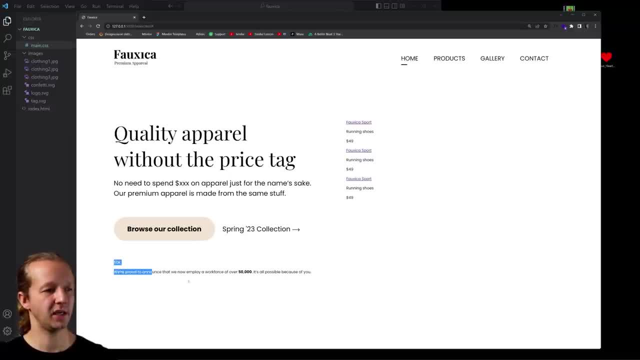 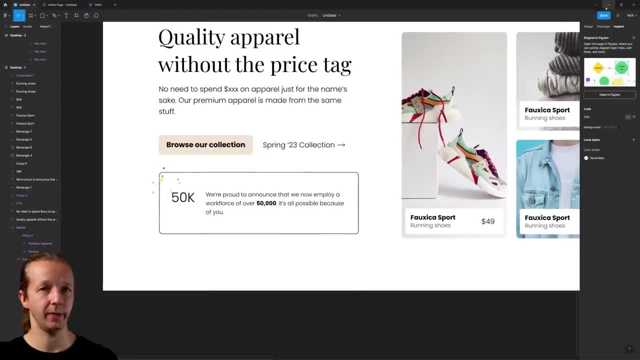 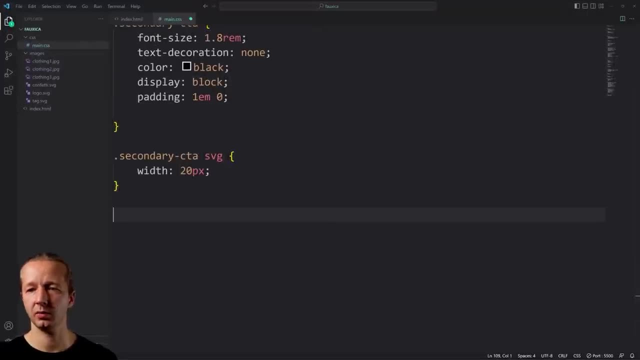 to wait until after we get everything else done here. Now we have this 50K section to do, which is not going to do too bad, And we need to make it look like this. All right, So let's extend this out. Underneath there, if you recall the markup, it has news and then a paragraph of 50K and a. 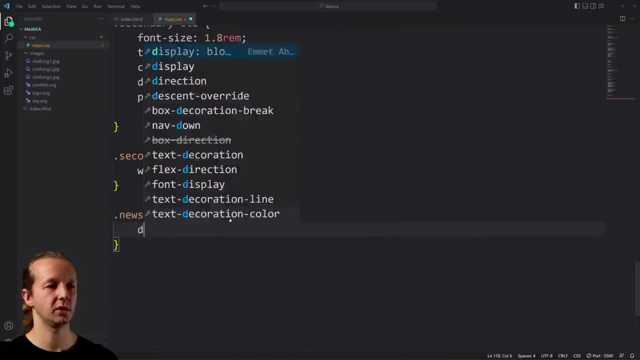 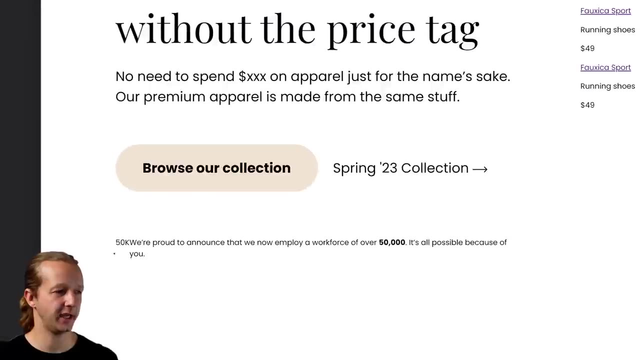 paragraph of details. So we're going to say news display flex, because remember, we have two columns, So now we have 50K. It's hard to see. It's right there, right up against the paragraph. There's no white space between it. All right, So we're going to come back. 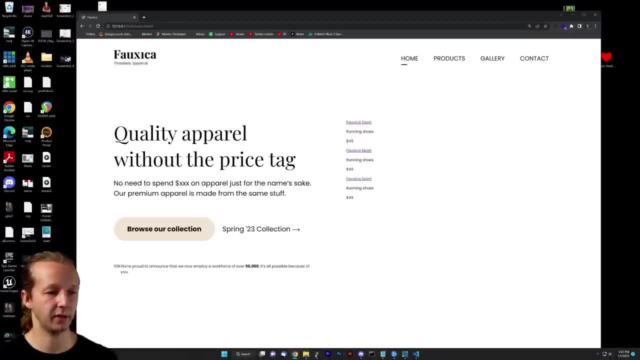 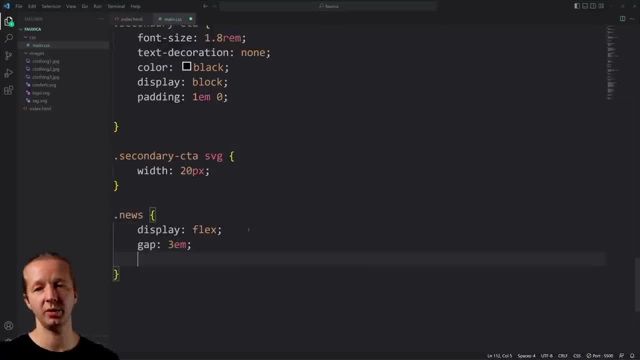 Oops, Let's get back up our code editor. Gary, you're screwing things up. Okay, There we go, And we're going to say: a gap of 3M units, or 30 pixels between them, a padding of 5M units or 50. 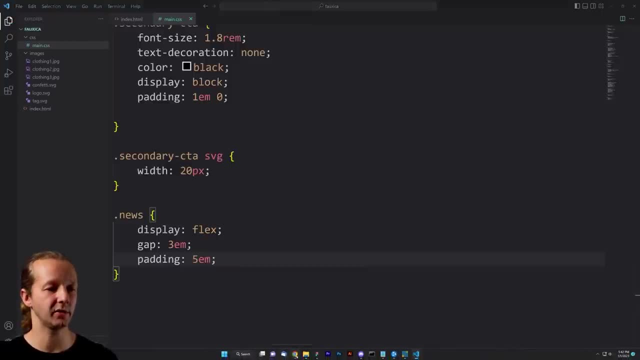 pixels inside of the news element. So let's see what this looks like. All right, So we're getting border around everything. So we're going to say border one pixel solid black. So if we save it, it's going to be just a rectangular border, but we do have a. 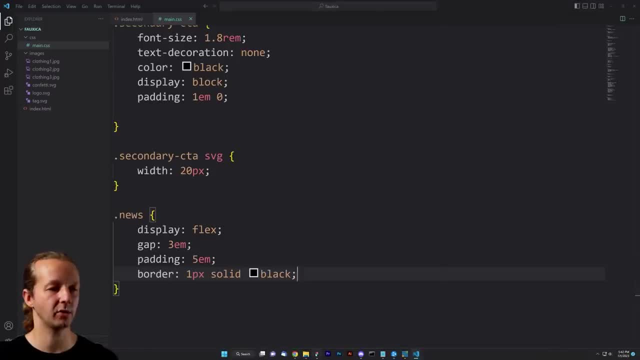 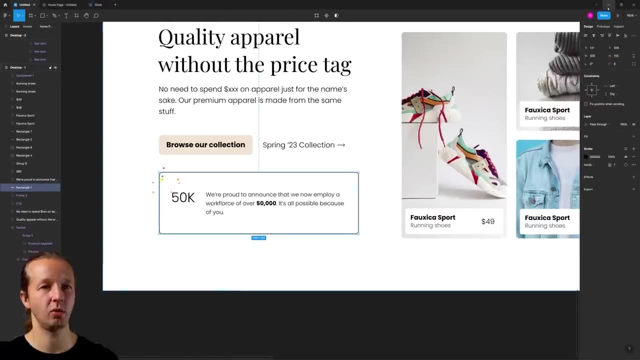 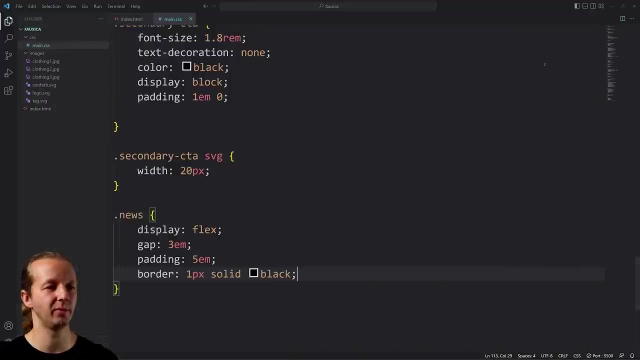 corner radius on that. So, going back to our design, we select it. It's going to be eight, All right, So 0.8 will be the actual border radius. Oh yeah, Okay, Sorry, My reference code was incorrect. All right, So border radius is 0.8 M units, And then we're going to do that. 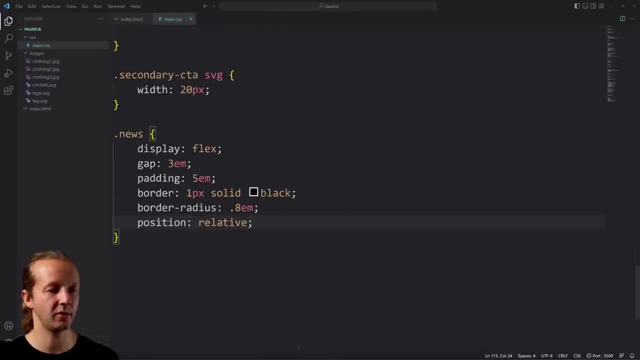 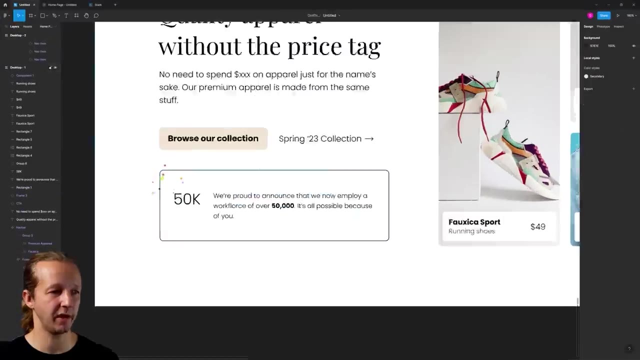 trick position relative- because that confetti, that confetti graphic that we have to add, All right. So, based on our Figma prototype, we have this confetti. So what we want to do is right click copy as SVG after you select it. 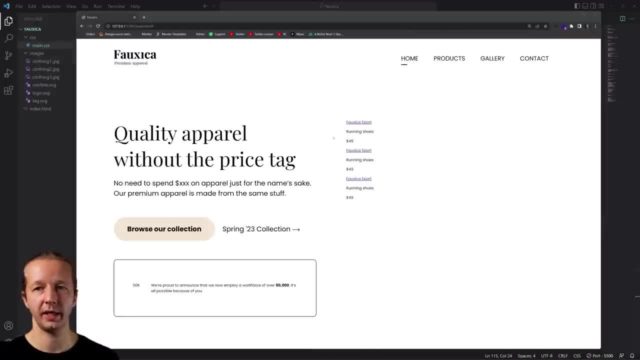 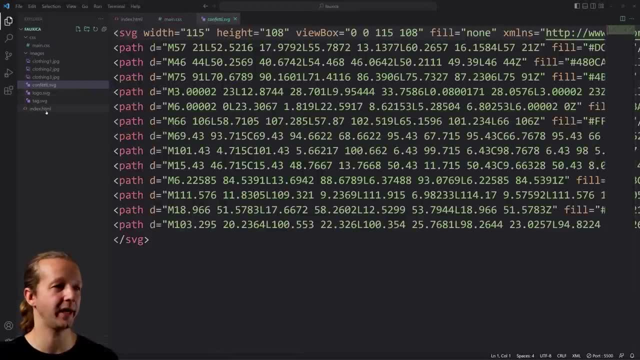 After you have that selected, what we're going to do is we're going: oh, by the way, it's already in here, So we don't need to do that. We've already saved it as a SVG file, So don't worry about that. Ignore that last step of copying it. 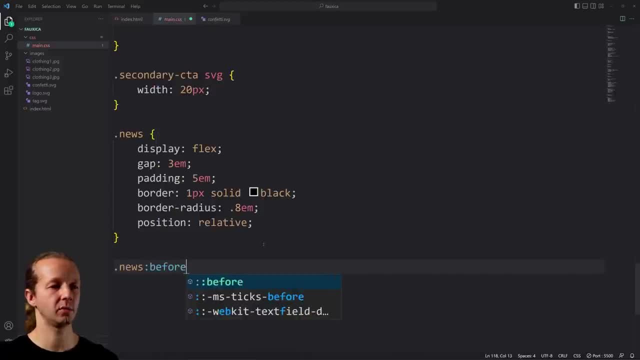 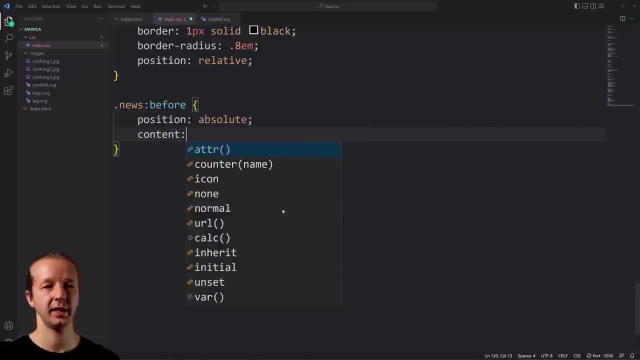 So now what we're going to do is we're going to say news- pseudo selector before, and we're going to say position absolute content- empty. Remember those three elements that go hand in hand. Background is going to be the URL to that image, So we would get out of the CSS. 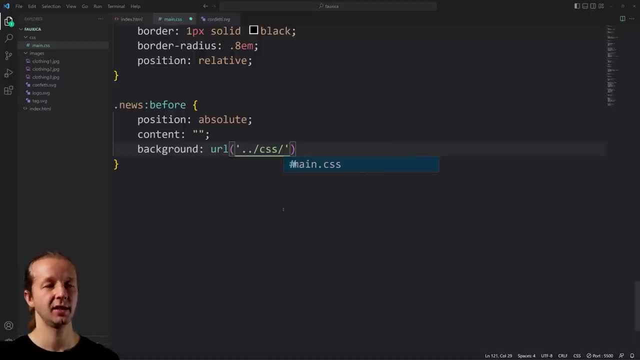 folder with the two periods for slash Into CSS, and then we select or into images, rather sorry. And then we choose confettisvg. All right, We still have to give this an explicit width and height, Otherwise we won't be able to. 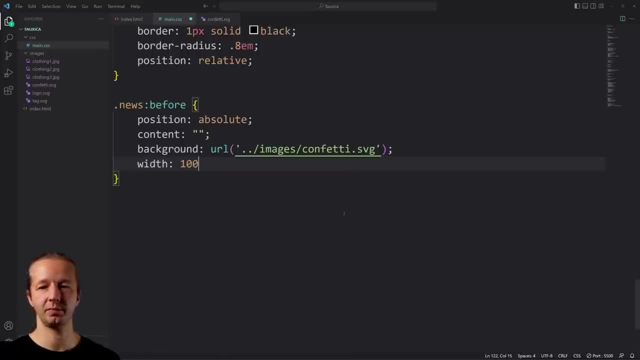 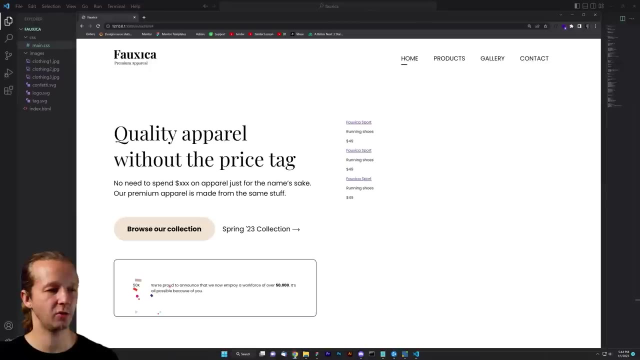 see it. So we're going to say width: 100 pixels or so, height 100 pixels or so, And let's just save it to see if we see anything at this point. Yeah, we do actually, but it's not in the correct. 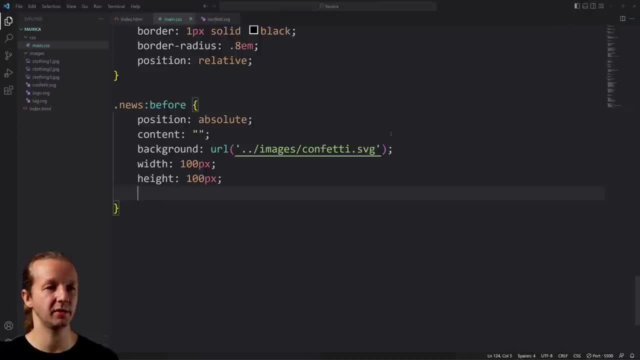 area that we want it. So what we have to do is specify a top value. We're going to make it negative, So you can do negative values. It'll be actually above where the news element starts and you'll see the black line. So, for instance, if I save this and show you now, I might as well. 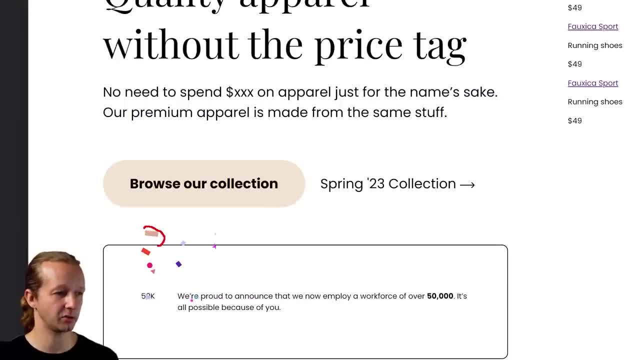 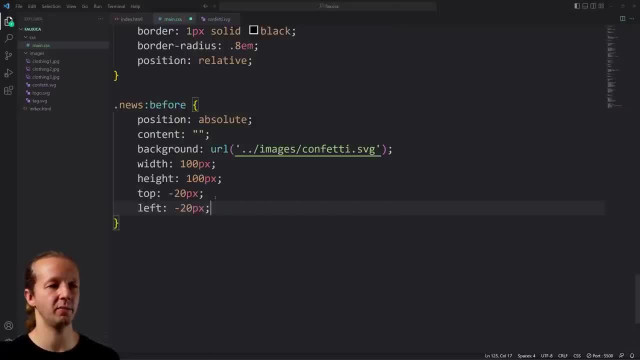 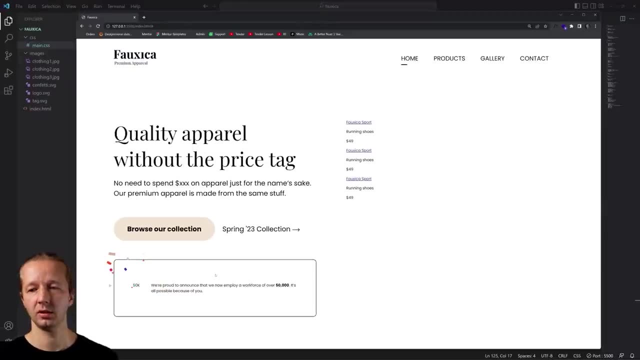 just show you and not try to describe it. It is starting 20 pixels above it. We also want it to be off to the side by about 20 pixels or what as well. So left will be negative 20 pixels right here. So we save that and there we go. Very cool, All right. Now just to make sure. 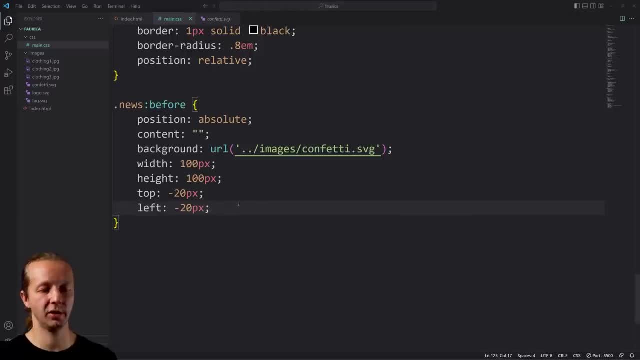 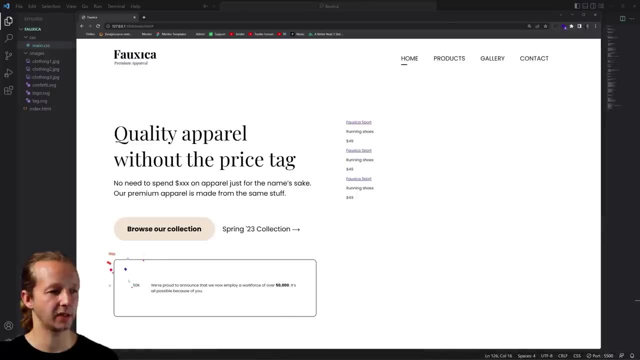 things are on top of each other. when you use position absolute on an element, you can use what's called z-index and we can make this like two. By default it's at a value where everything's kind of equal with each other. I don't think it really changed anything, but if you need something, 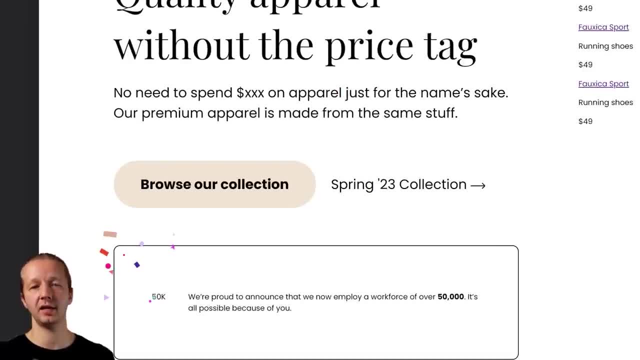 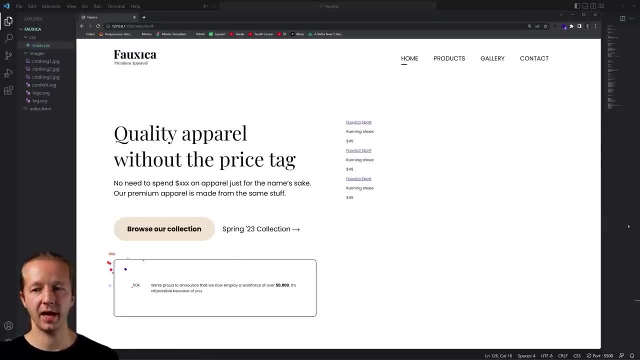 to show up like on top of something or behind something. you can use negative z-index values and so on and so forth. We'll use it again here At the end as well, and you'll see. Now we have to specify the type, because this is not big. 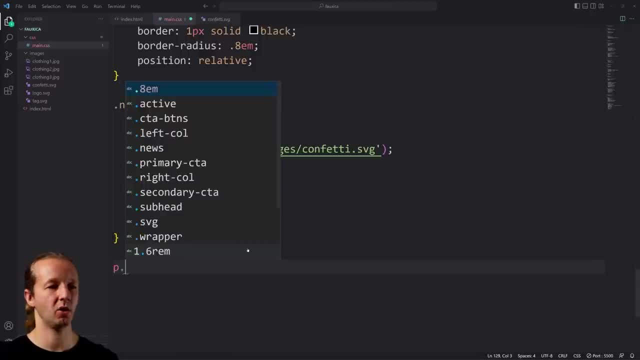 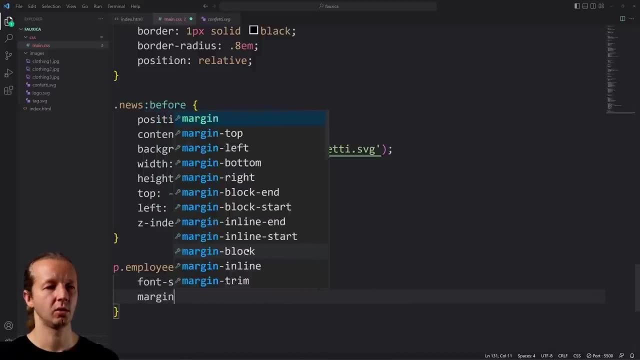 enough the 50K. So that is paragraph employees. Font size is actually 33 in Figma, so 3.3 rem units, Margin zero to get rid of any default margin. And then we're also going to use a lighter font weight of 200.. And there's going to be another element here that I specify. 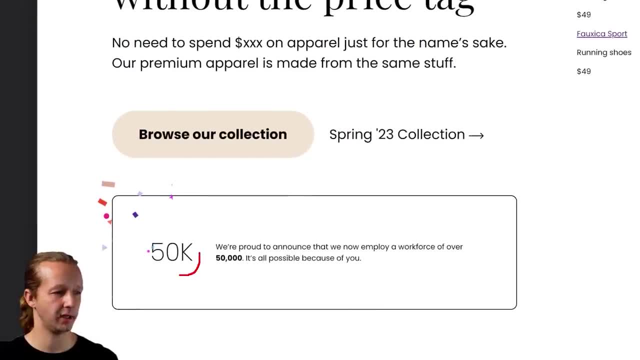 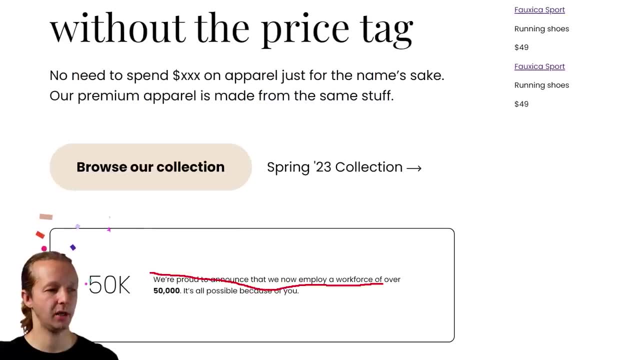 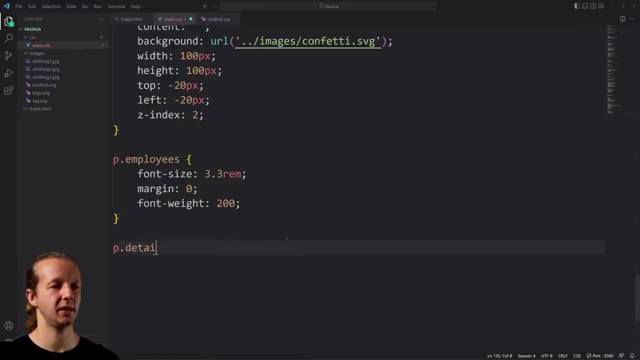 but I see here we are looking pretty solid right there. Yeah, it actually looks good as is, And then we're going to take our type right here and do something with it. So let's come over here. We're going to say paragraph details. Font size is 1.4 rem and get rid of any margin. 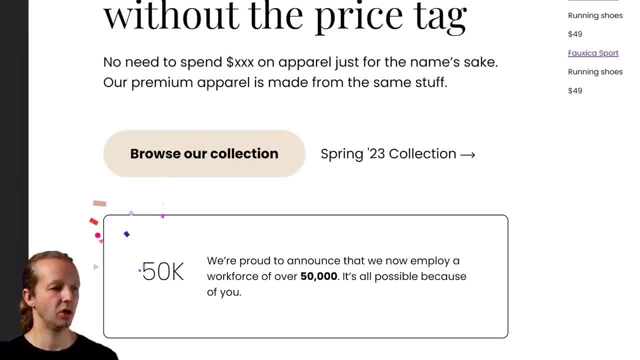 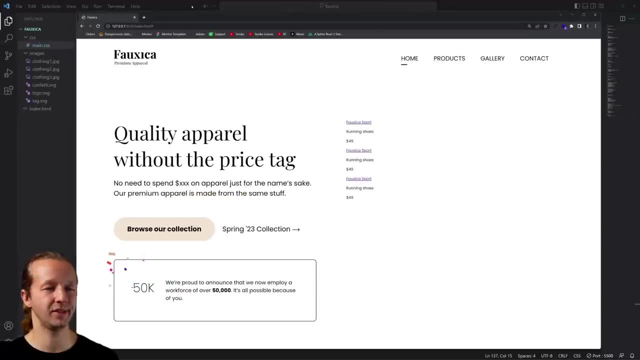 So we'll save that All right. So notice something right here. There's a column established right here, but the 50K is not matching it right. So this is one of those weird things, And you just kind of understand these things through trial and error. We need to. 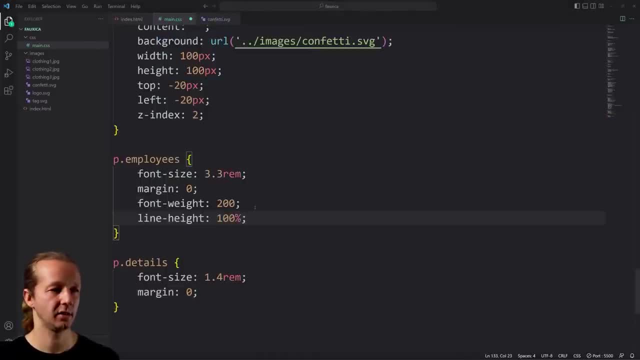 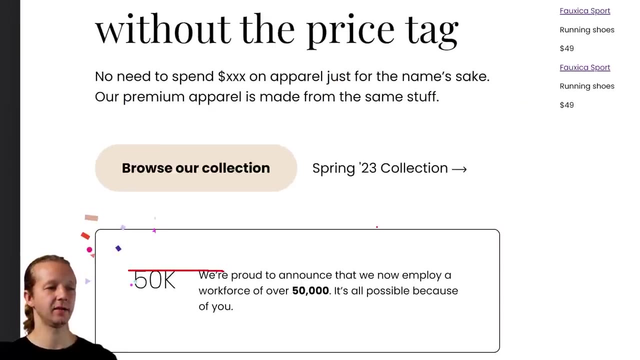 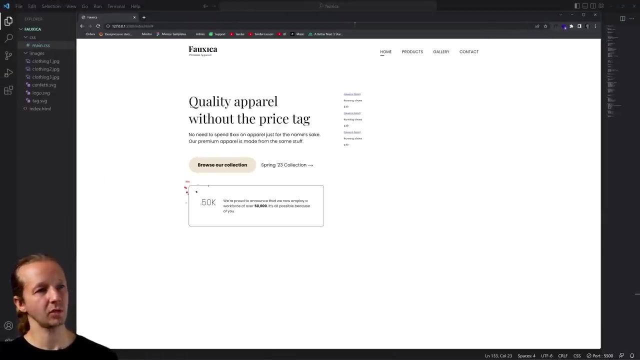 add line height 100% to employees And now it makes them even along that line. All right, So the bigger your type in is, The more the line height might affect certain things that you don't want to happen. Okay, So now we have this whole left column done, Let me go back to 100%. Looking pretty solid here Now. 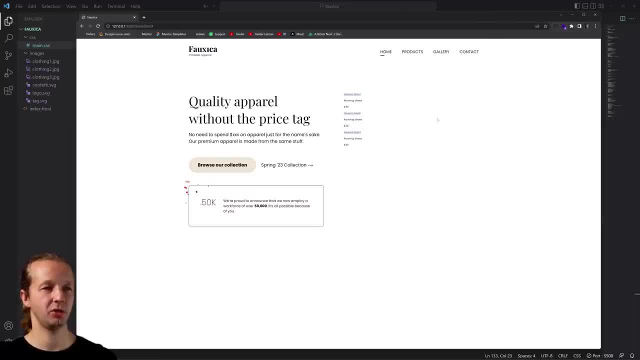 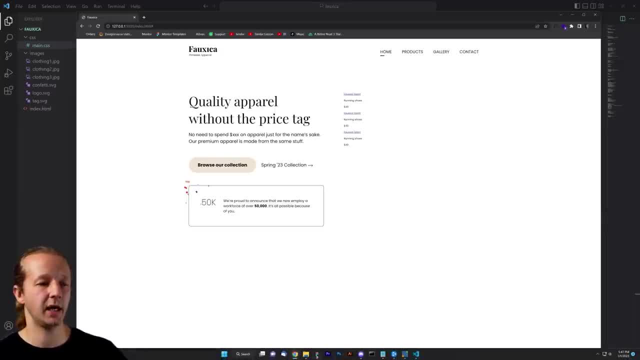 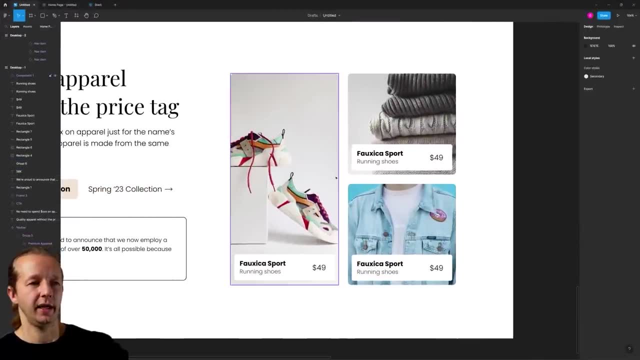 We've used nothing but flex. But if we look at our design you'll see we have kind of like a. it's not complex but it's. it's a design where, if you, if you think about things logically, we have, if you think about like in a grid sense, we have a. let me get rid of this. 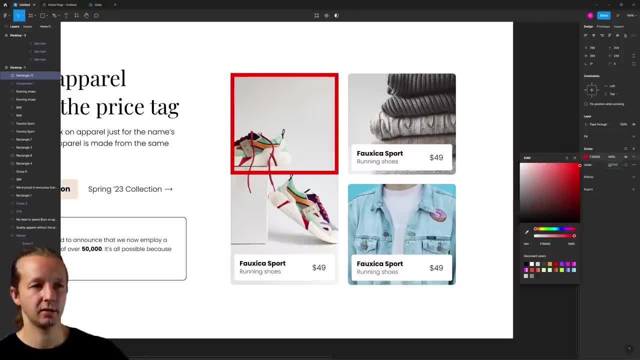 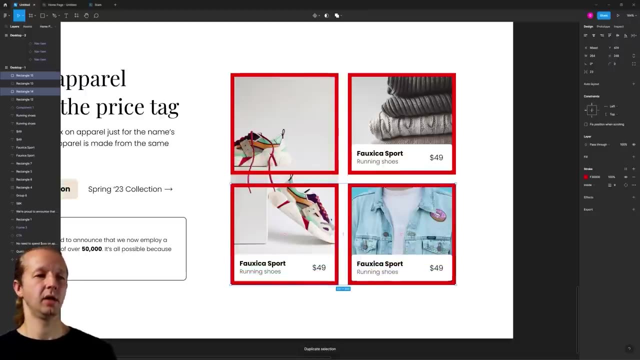 add a little stroke, make it red. All right, Think of this as columns and rows. Here's two columns with one row And here is another two columns with one row. So we have two columns in two rows. Whenever you need to organize things in this fashion, both on the 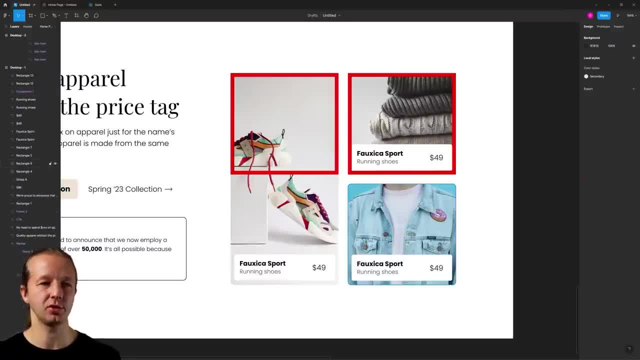 horizontal and vertical axis. the grid is a great way to do so So it can handle more complex sort of arrangements of layouts. So we have this overall element that wraps around all three of us. So we have this overall element that wraps around all three of us. So we have this overall element. 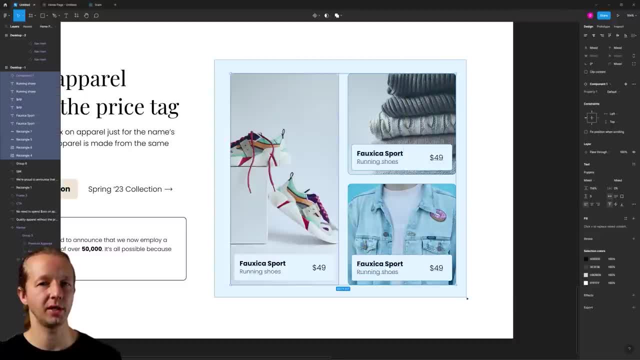 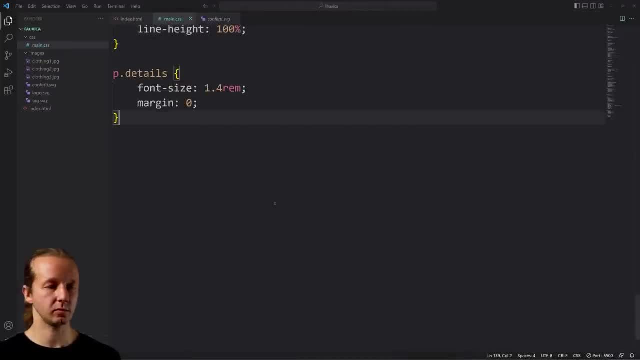 called right call. That's going to be our grid container, All right. So let's go ahead and start focusing on that, So we can put in a comment: right column, gallery, and we're going to say: right call, display, grid. Now we can also give it a gap, The physical distance or white space between 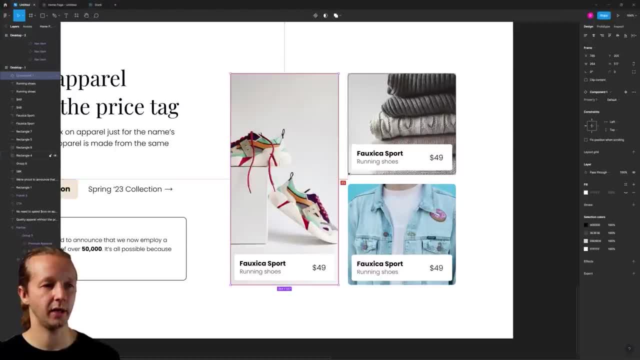 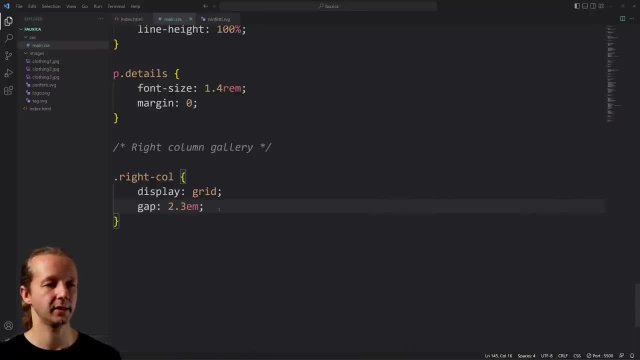 these elements is two, 2.3 or 23.. So it's going to be 2.3 and M units. All right, Now, if we go back and look, nothing's really changed, by the way. So now, just so we can visualize what's happening. 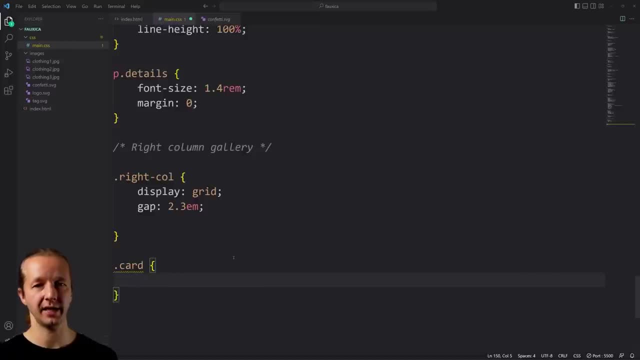 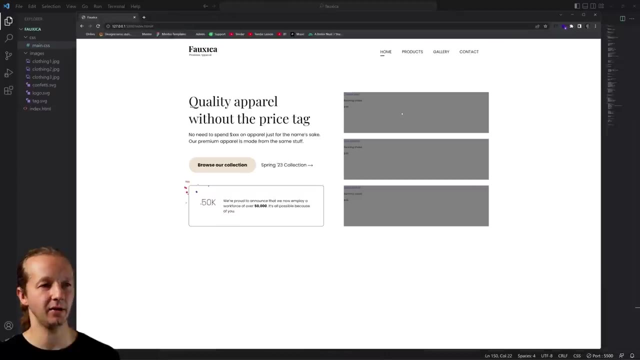 by the way, let's take our card- Each one of those card elements has a card class- and just give it a background of gray, just temporarily, So we can see what the heck's happening here. This is what it looks like right now. 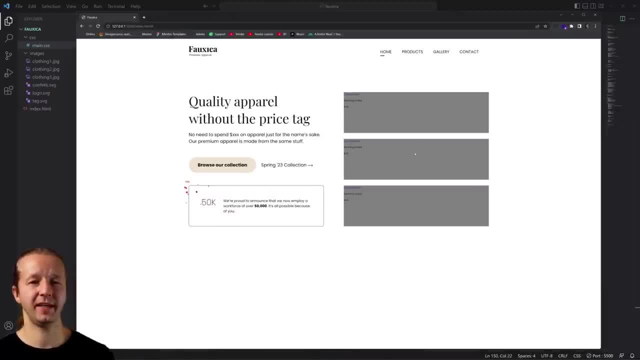 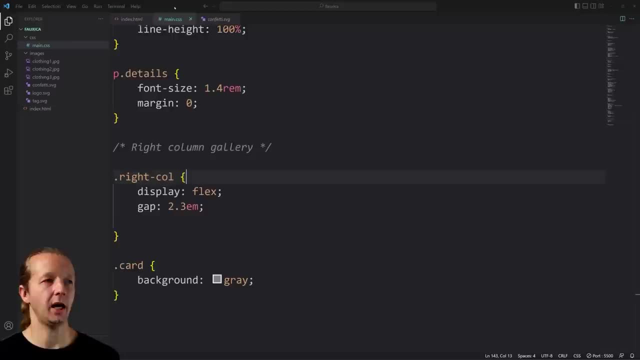 Unlike Flexbox, when you specify display grid, it doesn't automatically put things in the columns. It leaves them as rows, like this. That's an important distinction, because if we change this to flex and saved it, look it's in columns. So we don't want that, though We want it grid. 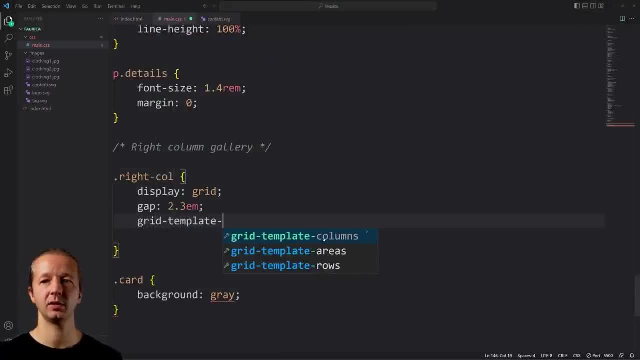 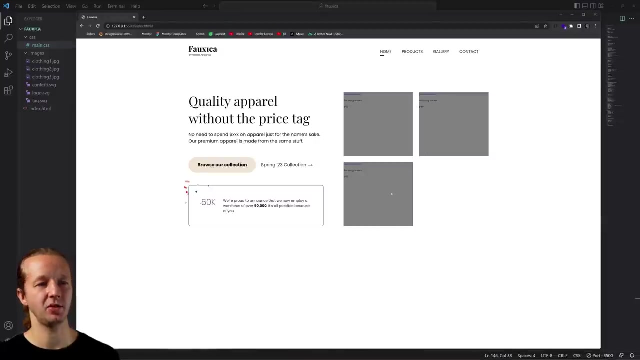 And then what we want to do is specify grid, template columns, repeat to auto. So that's the same thing as saying auto, auto, which means they're going to be the same width. If I say this, we see we have this situation, but to save yourself some time, repeat to auto. same thing. 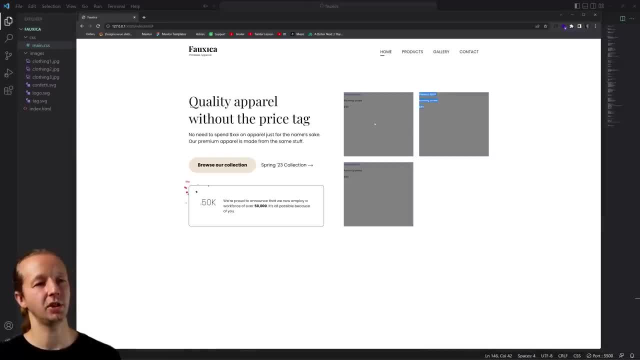 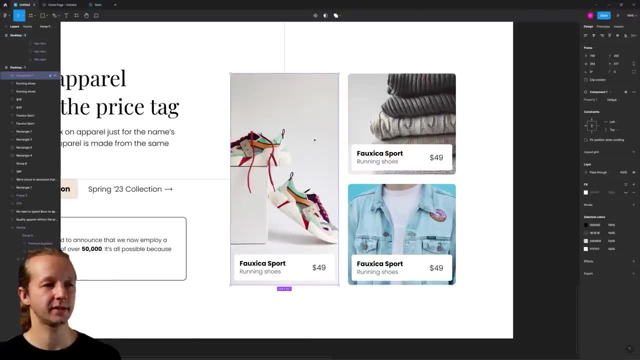 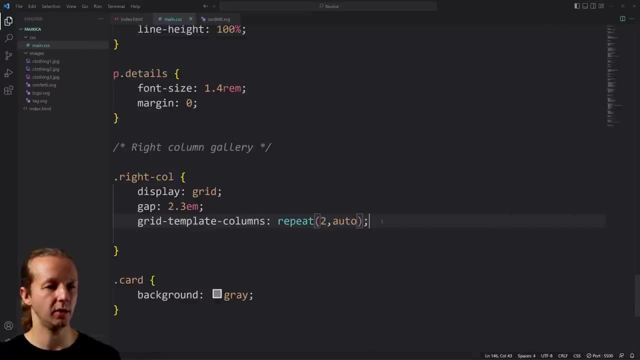 We're going to get the same exact result. It's a function. So, yes, you have functions in CSS. Now, this isn't consistent with the structure of this, because we want the first card to consume both rows, All right. So how do we do that? Well, we use something called grid template areas. 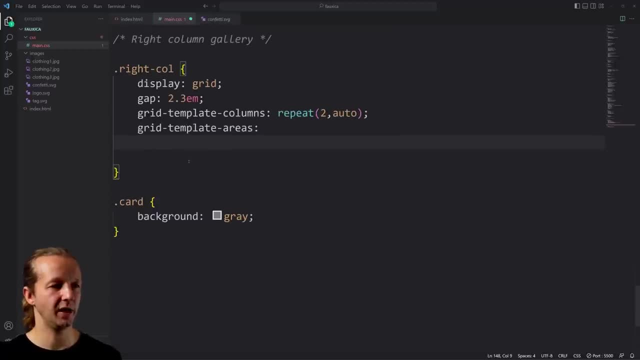 All right, And here's how I do it: Underneath I'll tab in and I'll put quotes and we give these names and you can name them whatever you want. So I want you to visualize this in the context of two rows and two columns. So left right, That's the top two, I guess. 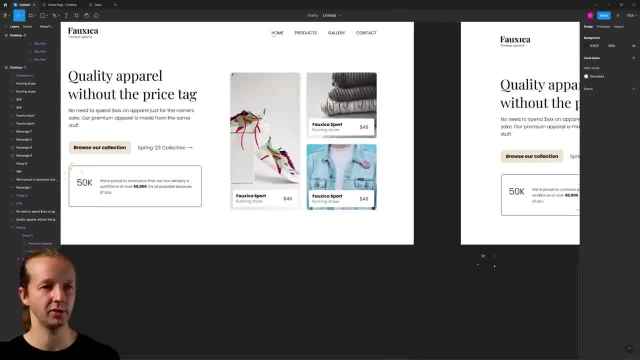 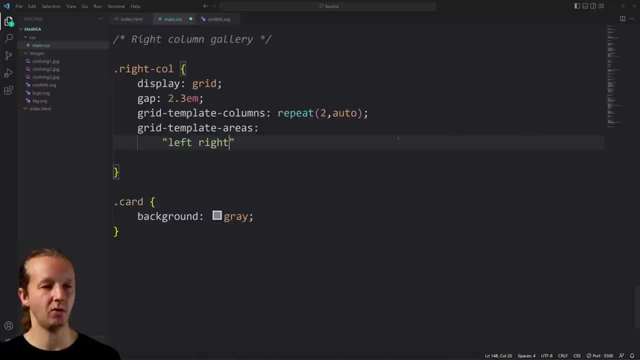 you could say grid cells right here. Remember, we created those red lines. So you have one right here and one right here called left and right. Now shift alt down. We're going to keep left there. We're going to keep this the same name because we want that first card element, which 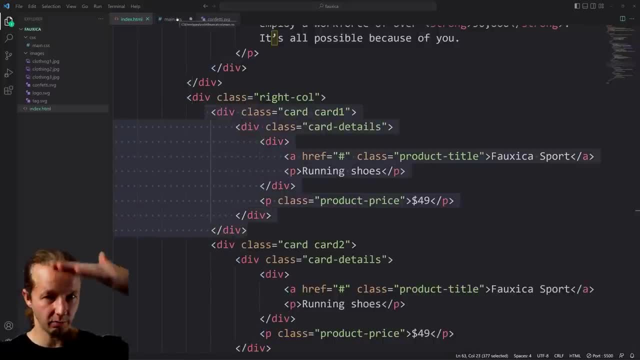 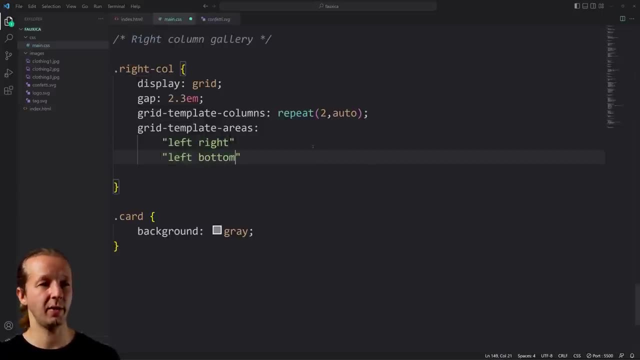 has shown up right here to span both of those rows, So we keep it the same name, This one we can just say bottom. So if we look at the amount of the words that we have, we have one, two, three, three different words and that we 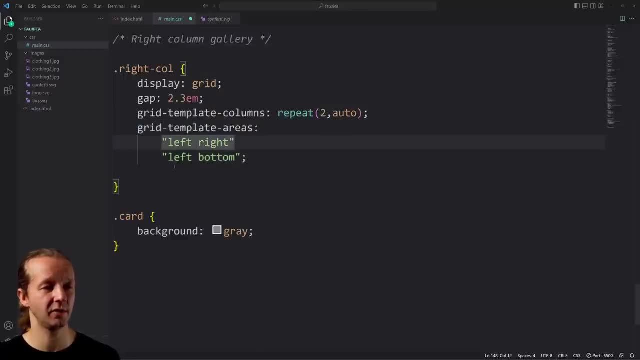 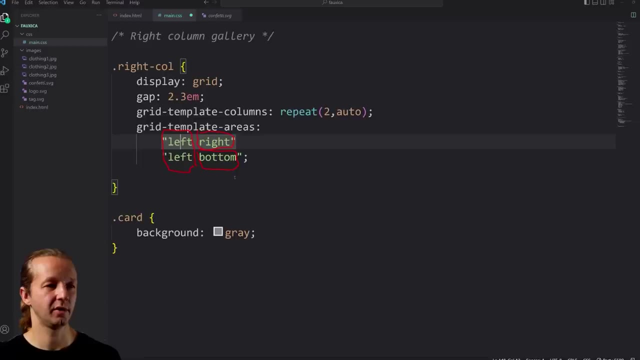 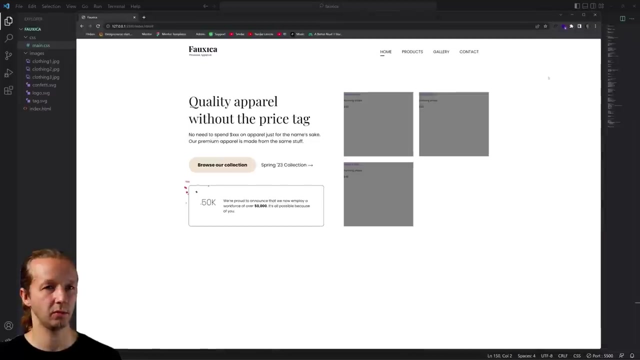 have three different cards and we've structured it so that we give a visual representation that this is the left column, Then we have a right and a bottom. Okay, So we're done with that, And now nothing's going to change really from where it was before. Now we have 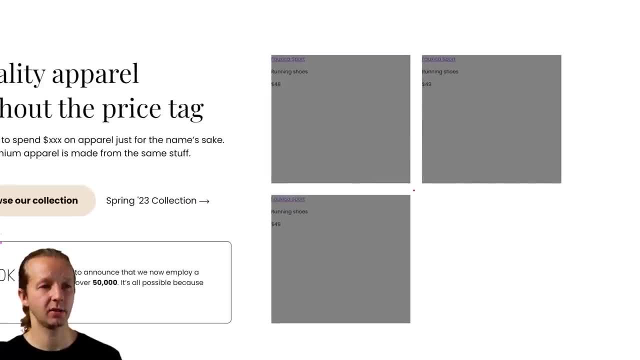 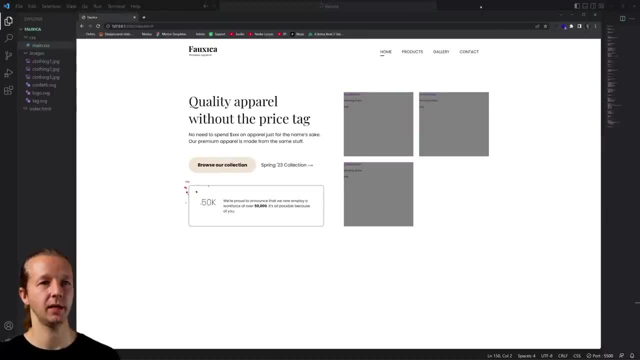 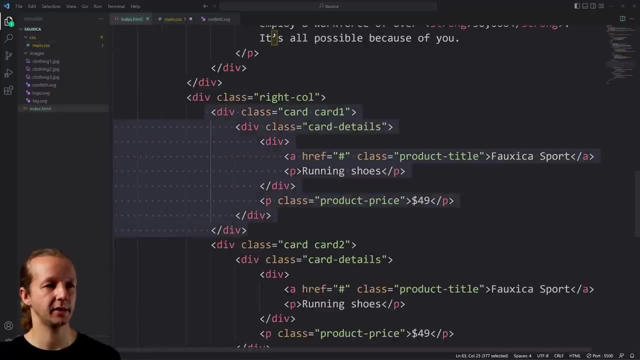 to assign grid area names to each one of these, So it knows, you know, which one is going to be called left. All right. So to do that, we simply say card one And again. that's a class that exists right here on the card. 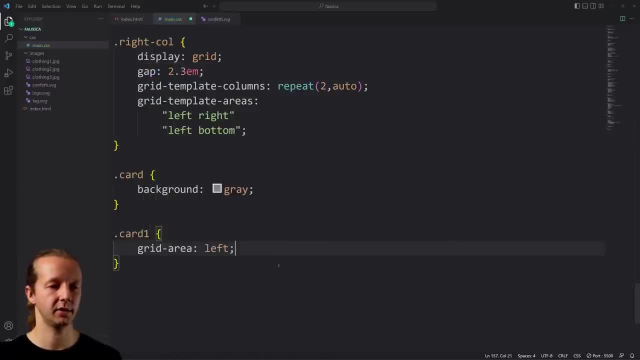 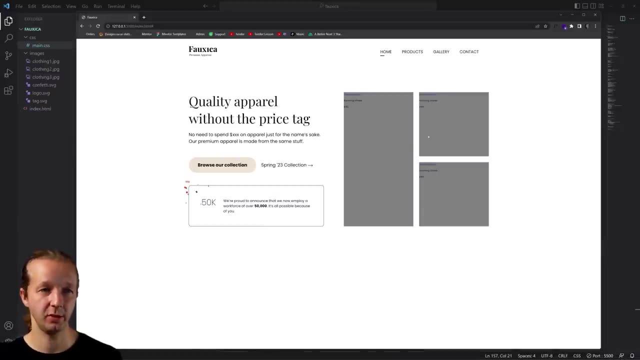 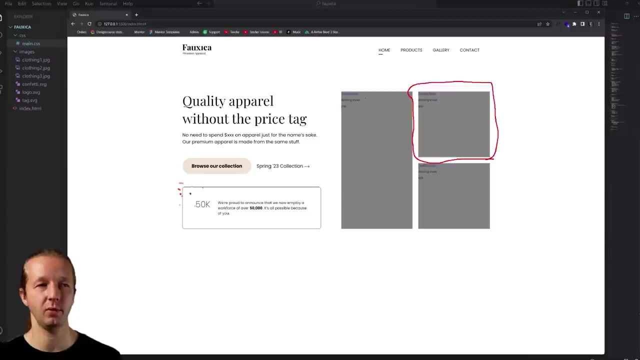 one And we say: grid area left: save it. Look at that. All right, So we don't even have to explicitly name these two over here, Because it already has the structure that we want And in that case you don't even. 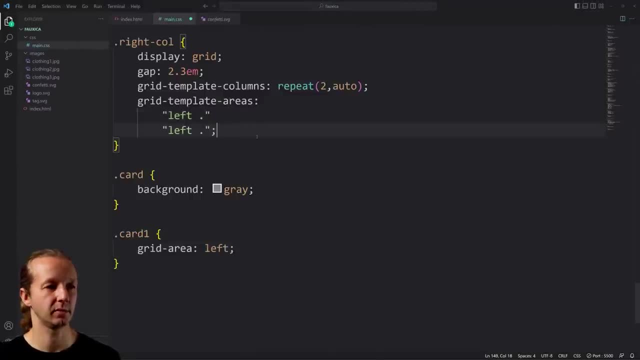 have to put right and bottom. You could just put periods. Look at that Awesome. So now I let's go ahead and start working on our card rule set. because our card rule set. there's a lot to be desired about what this looks like. This looks nothing like this. All right. 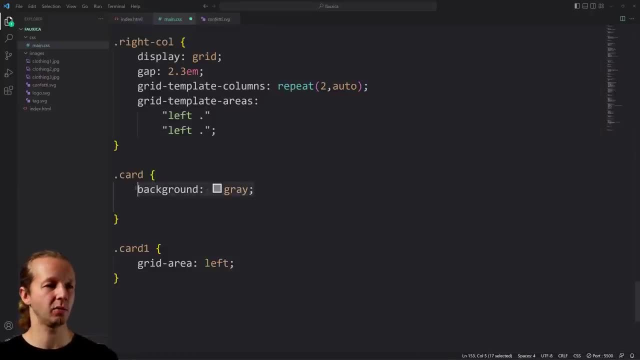 So card does not need a background. Uh, because we're going to have image based backgrounds in a bit. What we want to give it is a border radius. Each one of these has a border radius of what? Eight, just like everything else says. our buttons have eight, So it's going to be 0.8 M units. We also want: 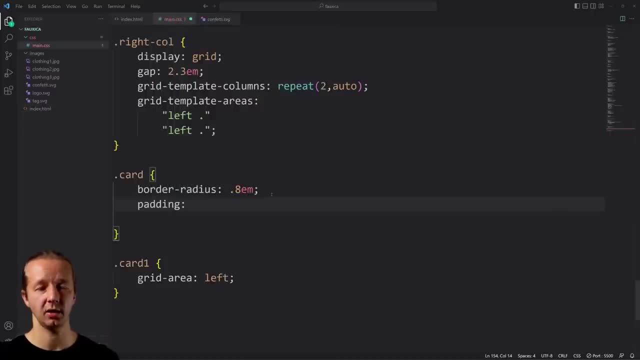 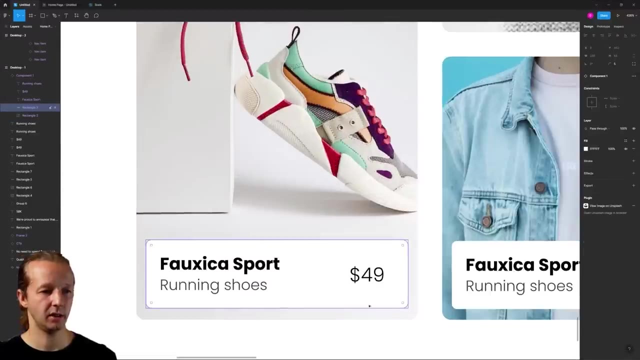 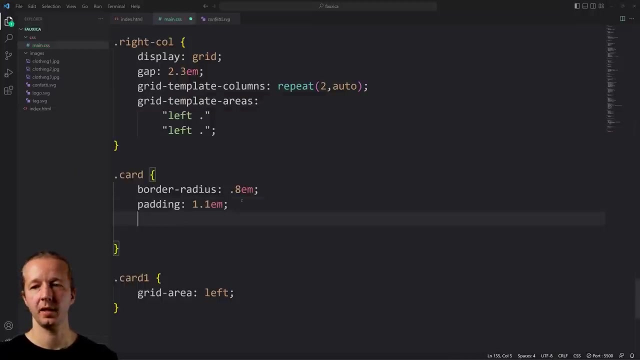 to give padding of about 16 pixels on the inside around, uh, the white little container. I'll just show you real quickly right here. So take this element alt actually Okay. So this very variation is actually a little bit different. I have 11 here, so let's just do 1.1 M units there. All right, We're also 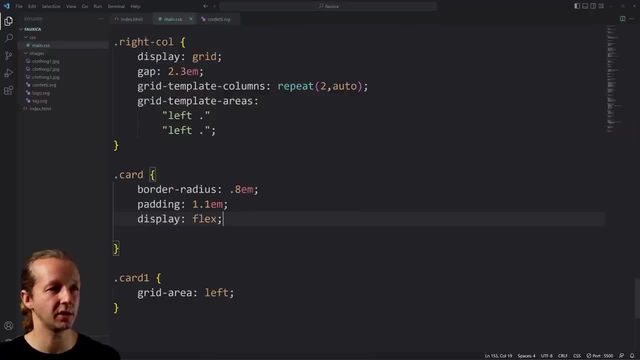 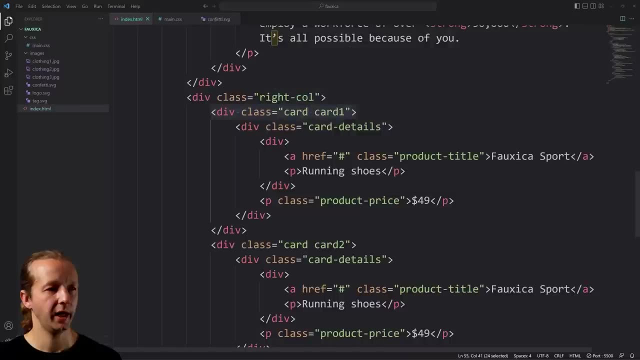 going to do a display flex on the card itself. Now, this is a little bit different What you're used to. We have the div class card element and we have only a single element inside of it. We're going to called it. We're going to call it, And you know the requirement for. 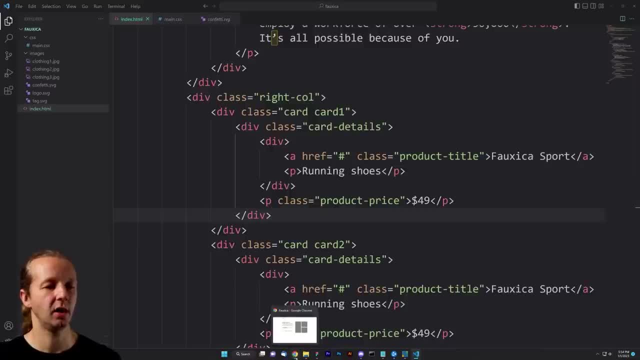 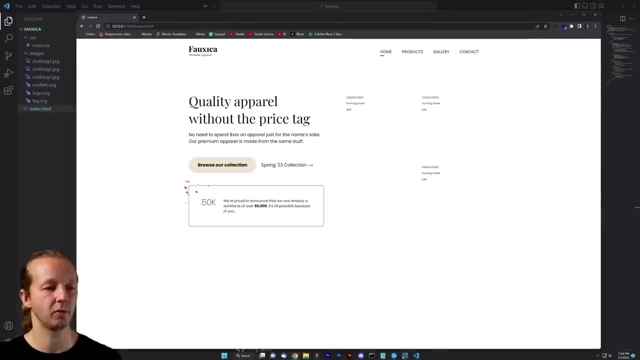 that is, that we want to make sure that the top element is always at the bottom, So the table does not have to be at the top. But we want to make sure that that content right up here is not at the top but instead at the bottom. because if you refer back to the 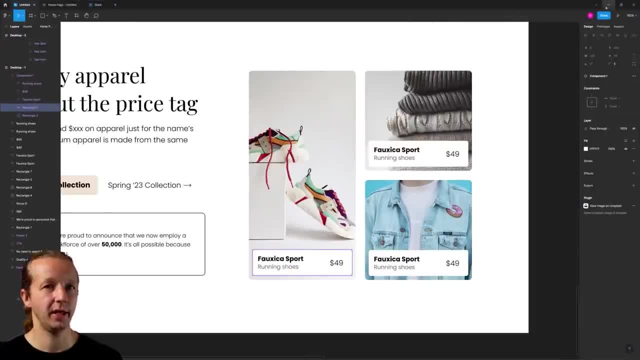 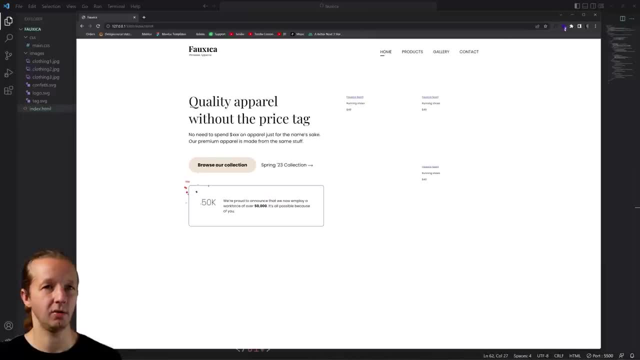 design we'll see that these are at the bottom. So a way to push things around is to make the parent flex or the parent element of flex box container. So we say, go back to our CSS display flex and we're going to go ahead and say align items. 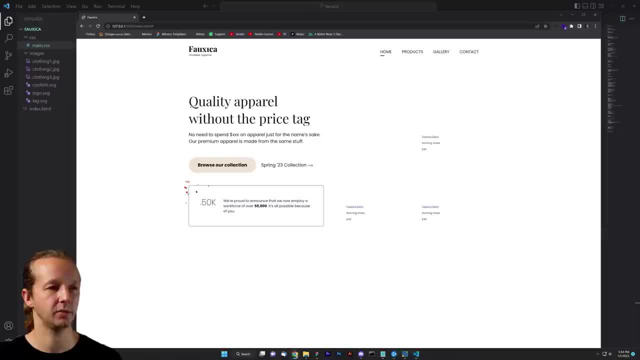 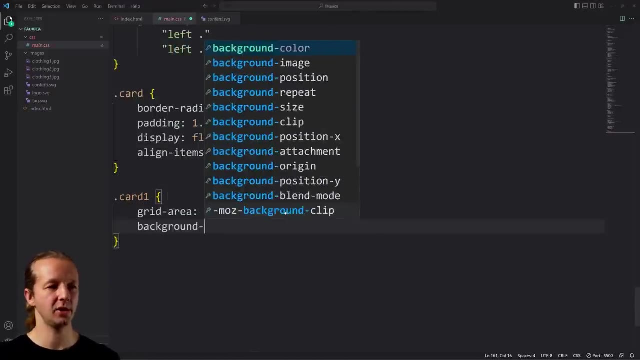 end. all right, we'll save that, and now they're at the bottom. so these little tips and tricks you'll pick up along the way, all right, now I actually want to see our images, our photographs, so let's do that real quickly. we're gonna say: background image URL out of CSS folder into images and we're gonna say: 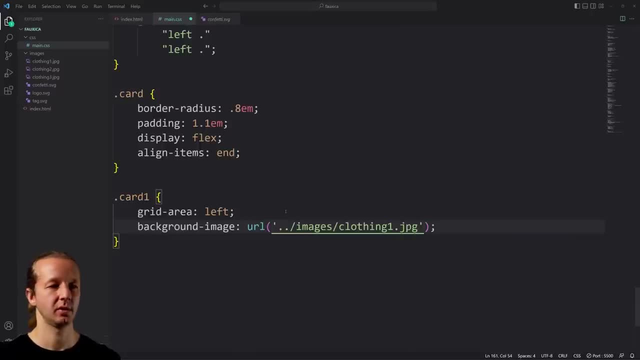 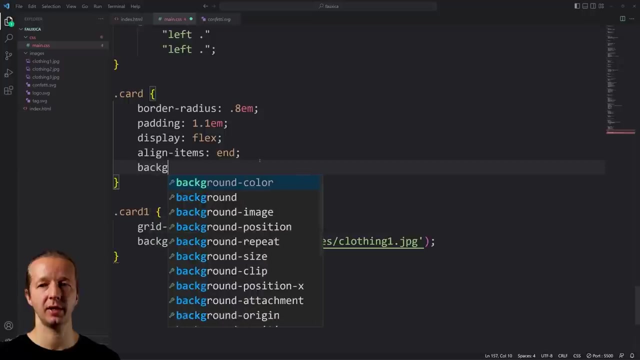 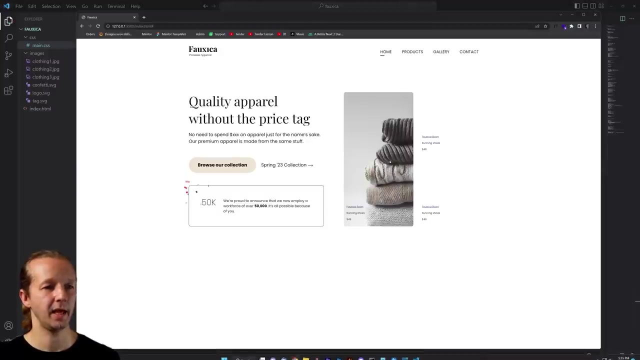 clothing 1.jpg. all right, we're gonna save it. there it is. now I'm gonna take the background size, we're gonna make it, and again, card and card one are applying to the same element here. so we're gonna say: background size 150%, save it. and now, 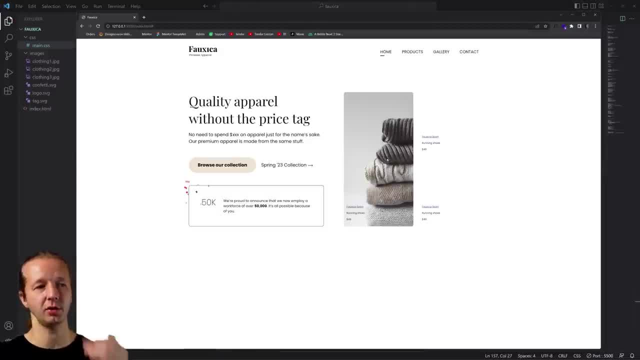 that changes the size of it. it was before. it was a lot larger and we're gonna actually, on hover, scale that down to a different size or scale it up, rather based on hover, but we're gonna get to that at the end. so now we need to make this section. 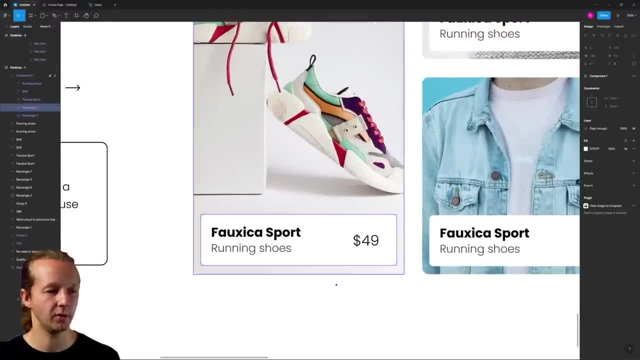 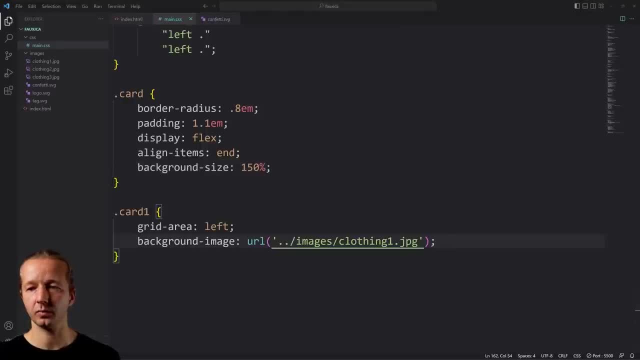 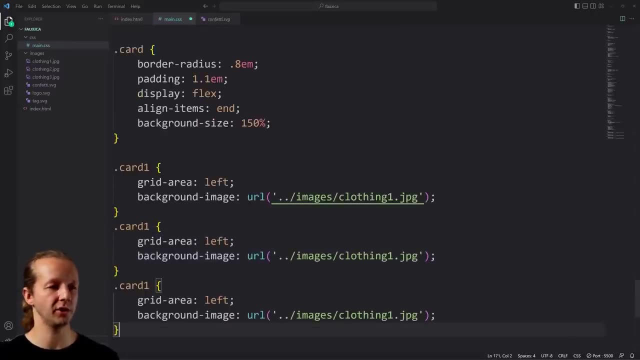 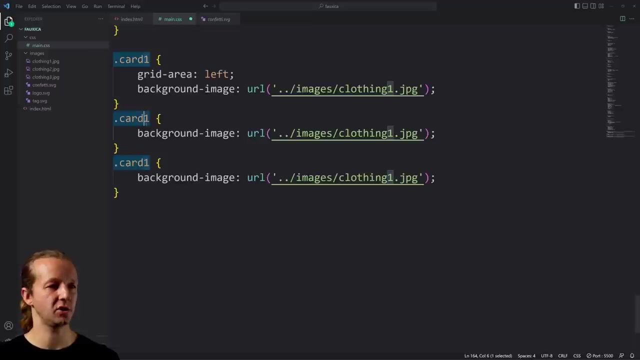 look like this over here. so let's do that. oh, and, by the way, we might as well real quickly go ahead and specify our card 2 and card 1. yeah, card 2 and 3 as well. so we'll say: we can get rid of the grid area here, change this to 2, this to 3. 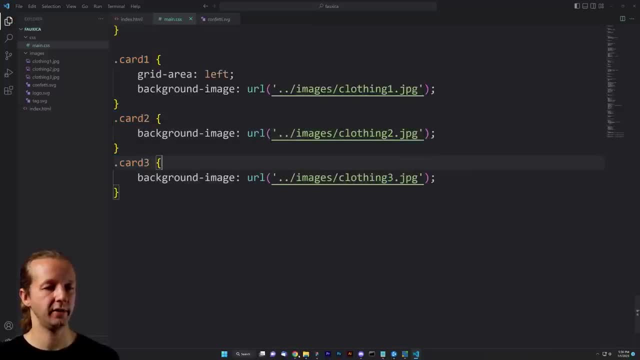 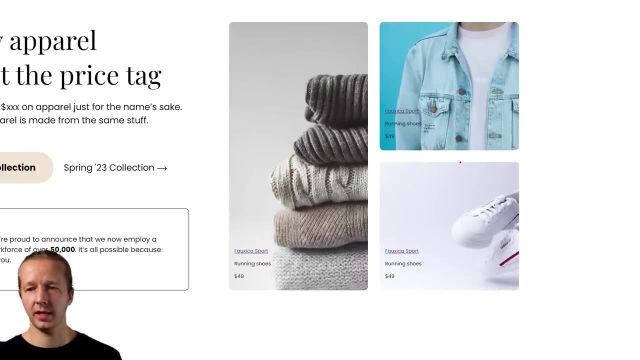 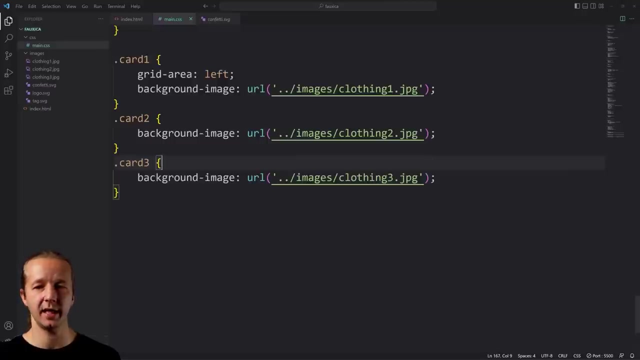 this to 2 and this to 3, save it. and there we go, getting very close, all right. so now what we want to do is let's go ahead and, yeah, like I said, work on those little white containers inside of them. all right, so that's called card details. 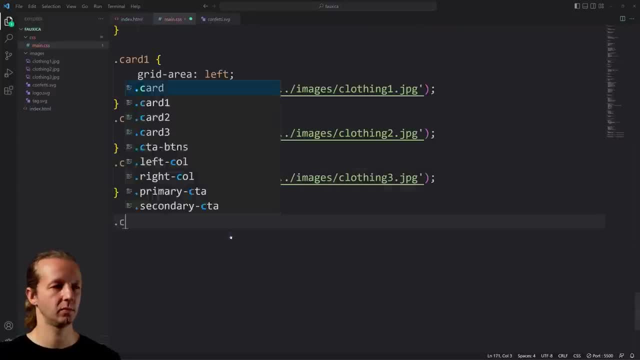 right here, all right. so card details: background: white border radius is 1m unit. actually it's gonna be a little more like 0.6. I mean sorry about that. and then padding on the inside of that white container with the text there's three pieces of. 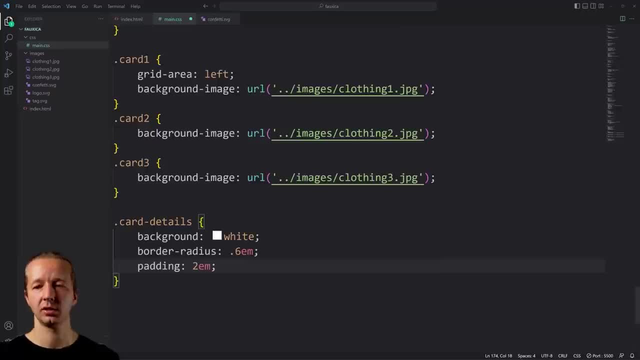 text. there's a title, a little category and then the price. so that's going to be padding of 2m units. the width will be a hundred percent. we're gonna say display flex, align items Center, so vertically centered inside that white box. we're gonna justify the content space between, because we have two columns of text, the 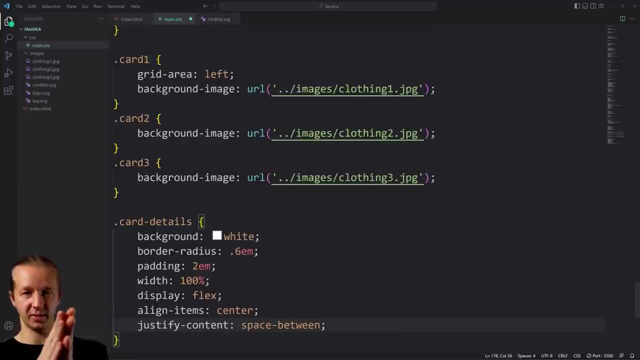 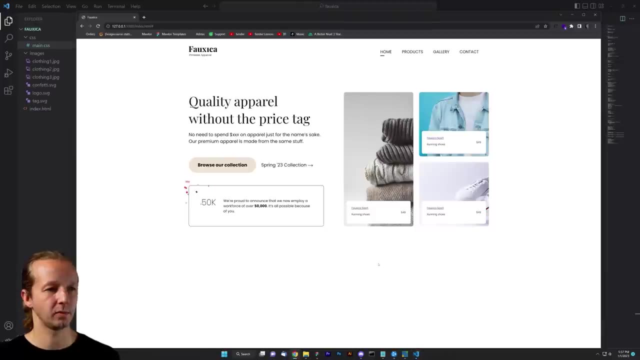 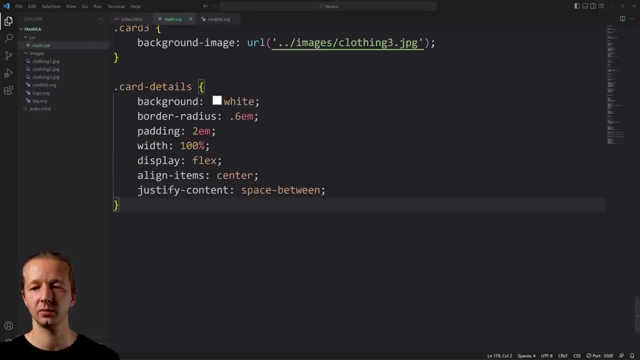 two bits of text on top of each other and then the price. so it needs to be spaced between, just like on our nav section with the logo and the navigation, and we're save that all right. so that's looking pretty kind of close. now we have to work and target the actual text to get proper sizes so we have a link inside. 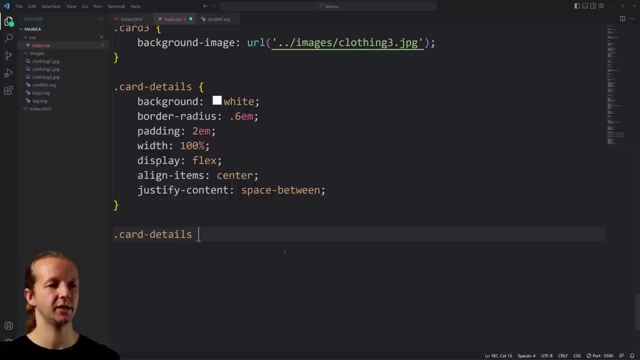 there for the title. so card details: a. we're going to say font size 1.4 for REM units, margin zero. oh, I'm sorry, I'm looking at the wrong rule set on my. yeah, sorry about that. this is actually gonna be color black text decoration: none font. 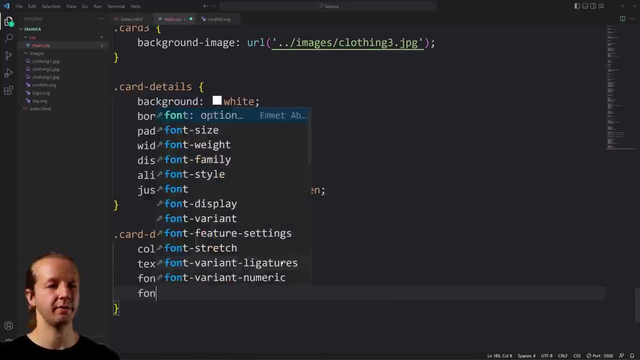 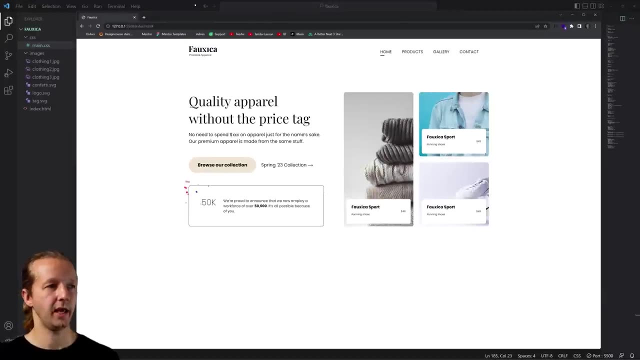 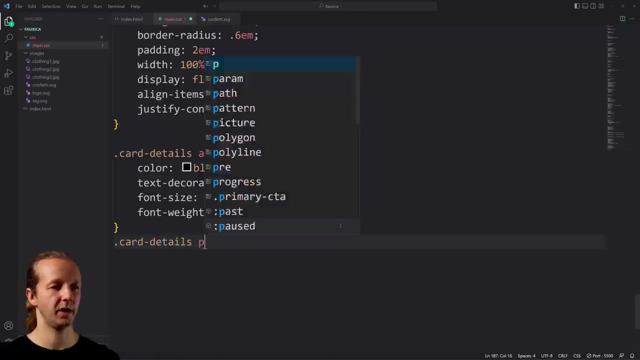 size for this is actually sixteen, so one point six REM and font weight will be bold. so this is what that should look like after saving. and then we have the one underneath it which is just card details paragraph. this is going to be a font size of 1.4. 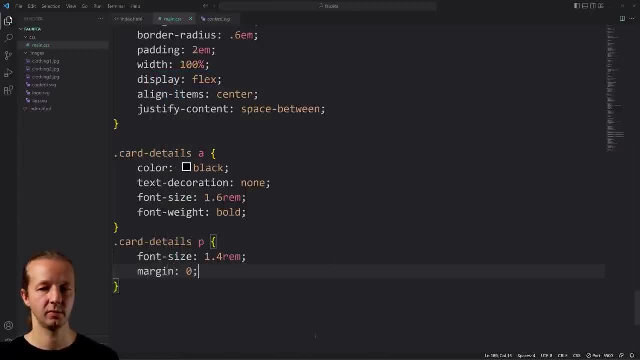 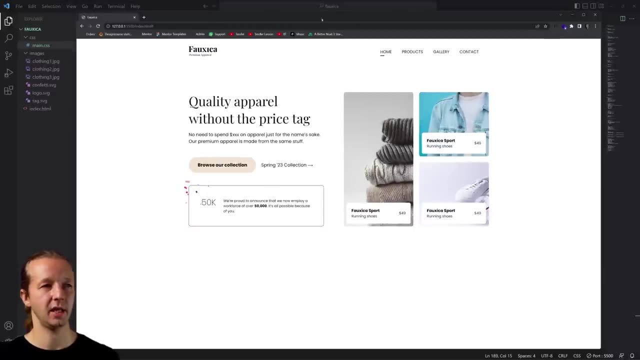 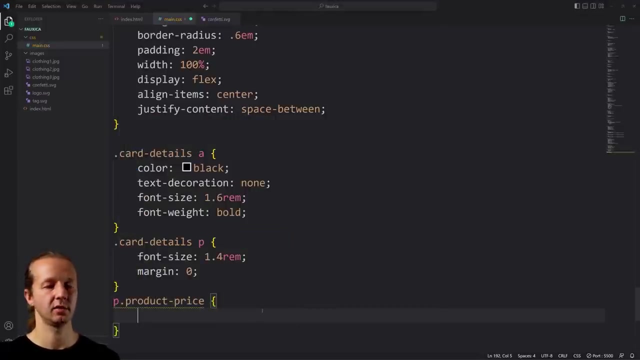 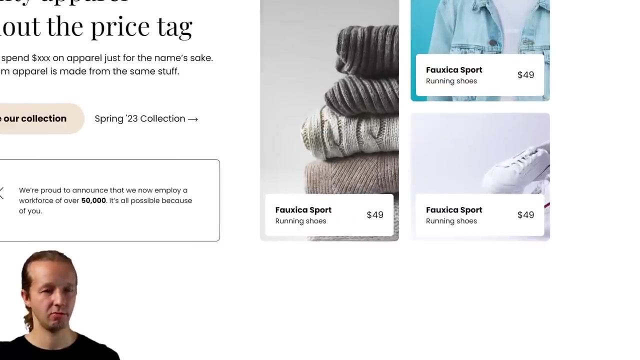 slightly smaller in a margin of 0. there we go, looking solid, very close. and then also the font size has to be increased. so p product price is font size, 1.8 rem units. save that, there we go, alright. now, if we refer back to the document, 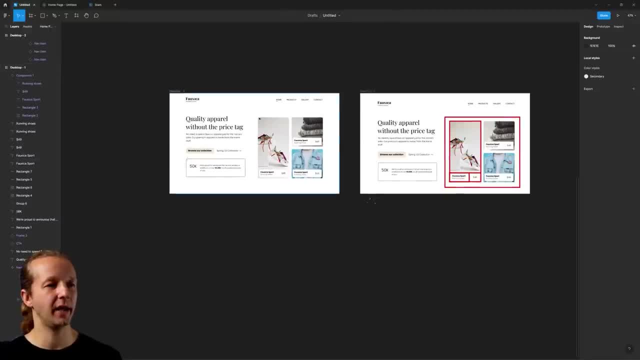 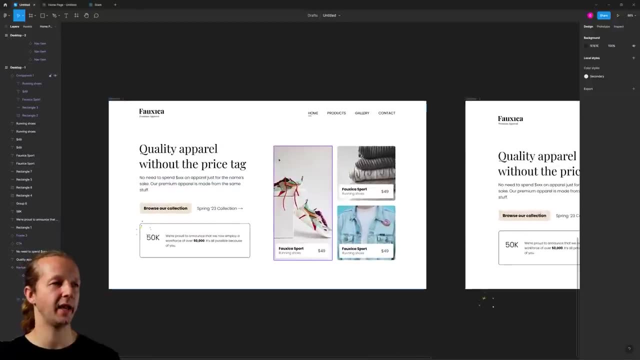 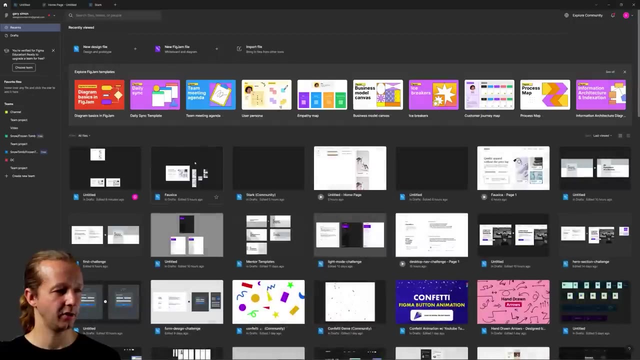 there's actually one thing that I 100% forgot to include, which I kind of wanted to include it, which is ok that I didn't do it. if I go back here to my in Figma, to my designs I had in our initial design and it was supposed to look like this: 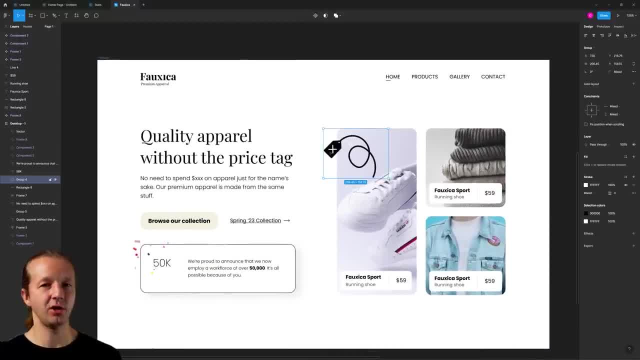 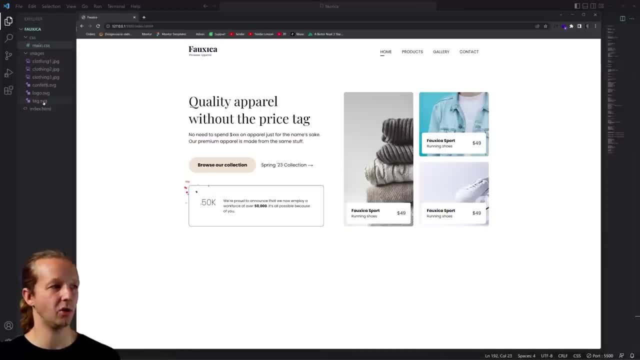 there was supposed to be this graphic right here. I want to show you how to do that actually. so this file is already an SVG file that's available right here, called tag, so I want to get that in here. so the way we do that is we go back to our main. 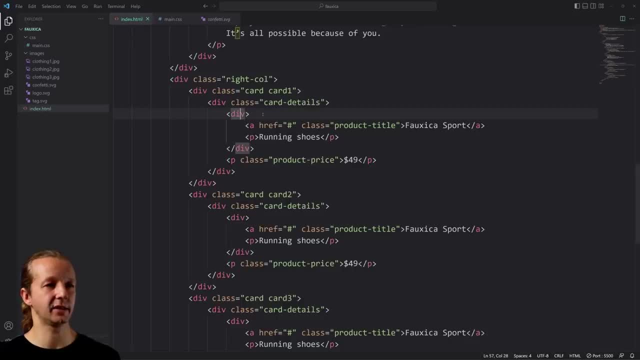 and that exists. it's going to be that technique where we're going to go back to our main, where we used a pseudo element of before, and it's going to exist on top of card one because that's where it's physically located in the design. so what we do is under card one. 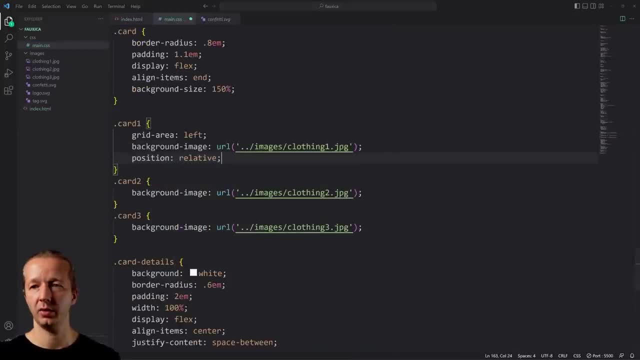 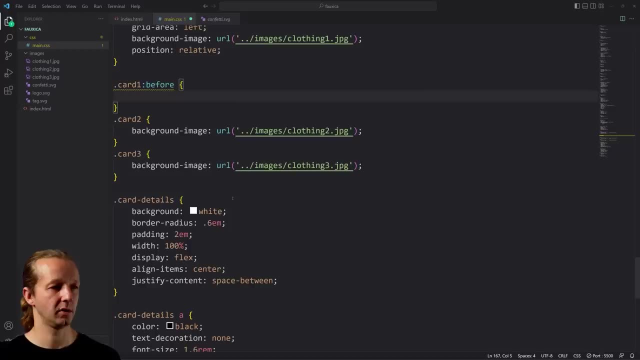 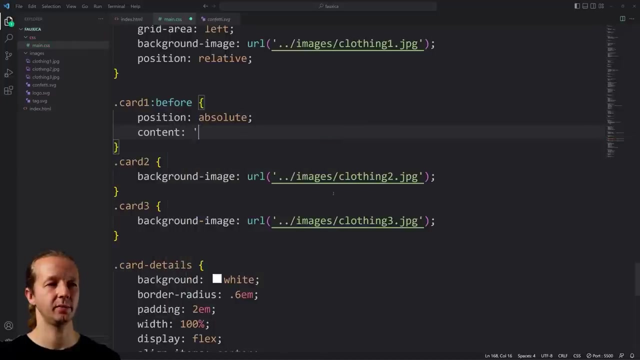 we say position relative, and then we use card one, pseudo element of before, card one before. alright. so remember: position absolute content is empty. we go back to our main and we're going to go back to our main and we're going to go back to our main. 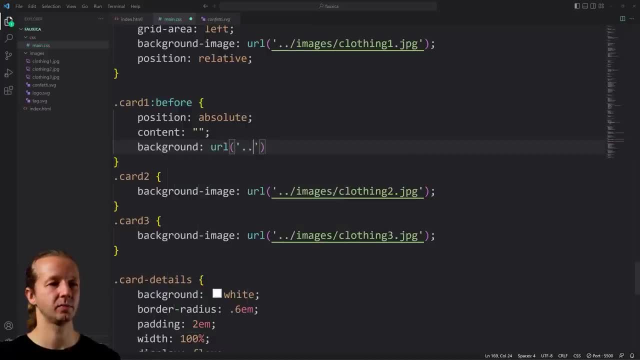 and we're going to go back to our main. we have a background of url, we have a background of url, images, tagsvg, and we're also going to put in here no repeat. after doing this rule set, you can experiment with what happens after we remove no repeat. 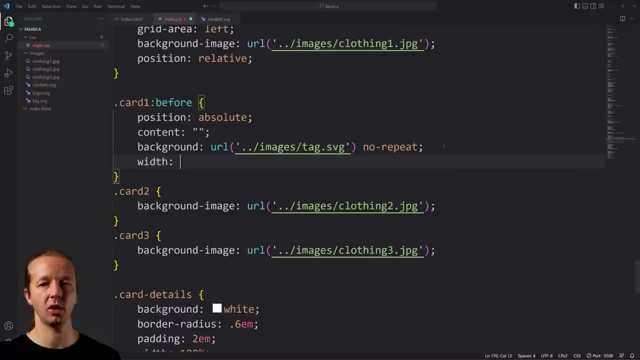 it'll just repeat. it'll look really weird. so we're going to put width: 100%. height 100%. top is going to be 20 pixels. left and right, 100% will be negative 30 pixels because it hangs off to the side of the card. 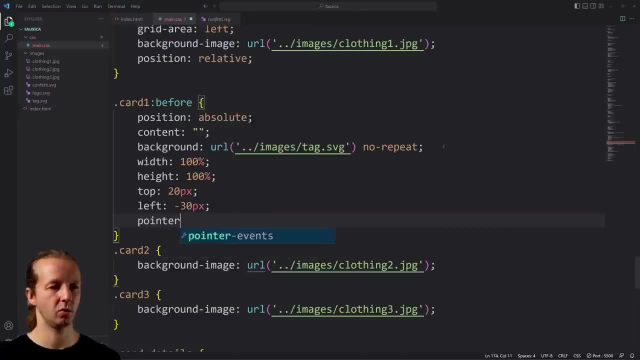 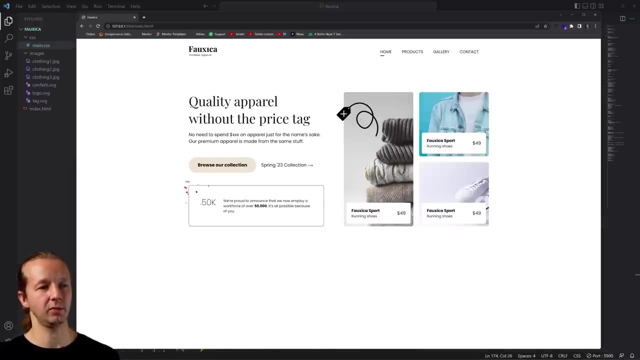 and then we're also going to put pointer events- oops, pointer events, none. alright. so let me show you what that does here. it is alright. so if we didn't add pointer events of none, notice how, right now, I can click on this link, which is what we want to be able to do. 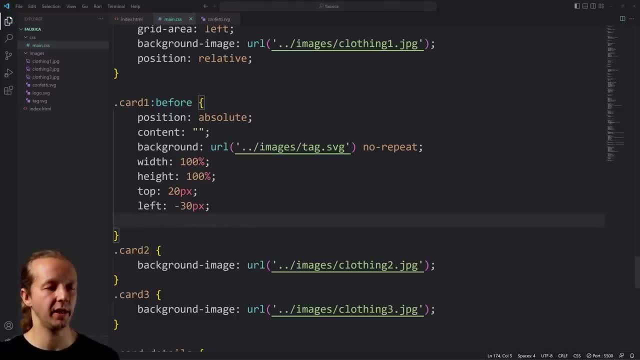 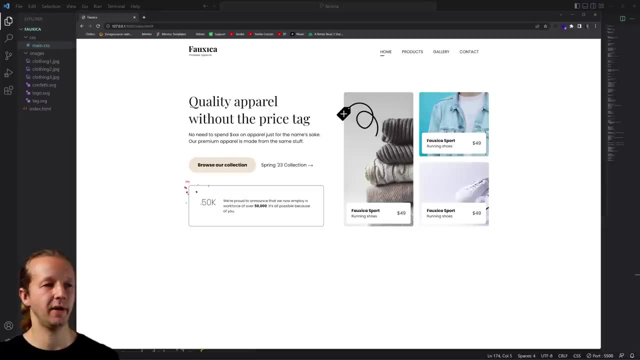 if we don't put that there, because we specified a width and height of 100%, because we specified a width and height of 100%, we won't be able to click this. we won't be able to click this. it will become unusable. so pointer events means. 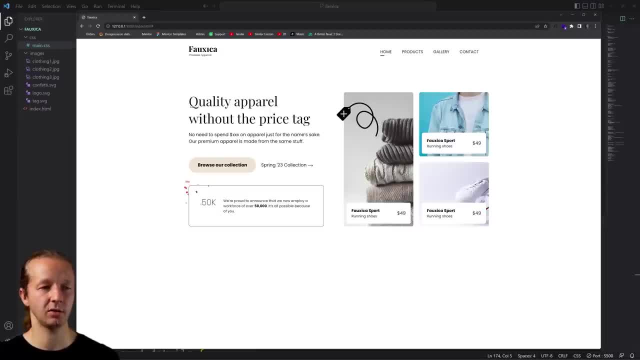 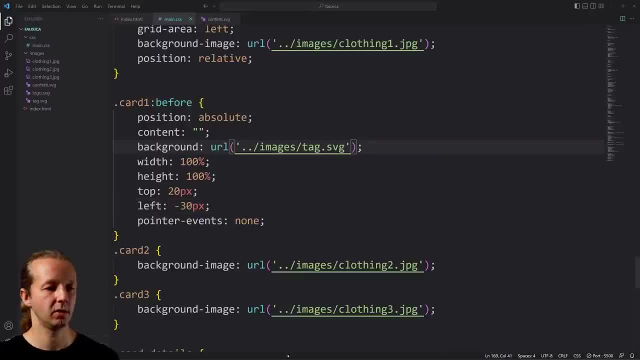 they should have no effect on the cursor at all because it's sitting on top of this stuff. so just for your understanding. now, if we remove no repeat, watch what happens. it's all over the place. so we only want it to repeat once. so you put no repeat. 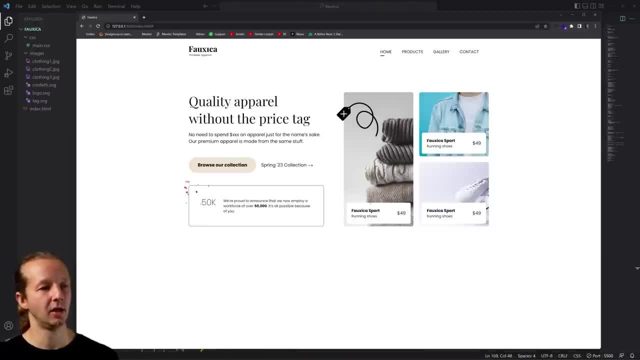 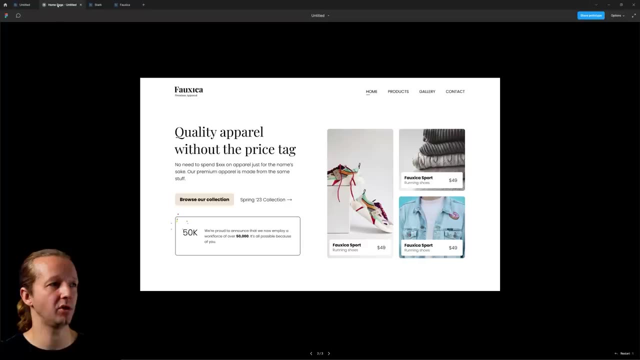 or not. we don't want it to repeat at all, we just want it to be displayed once. alright, that was intense. my face hurts from talking. anyhow, we're not done yet. we need to do those micro interactions. so if I refer back to Figma and we go to the prototype, 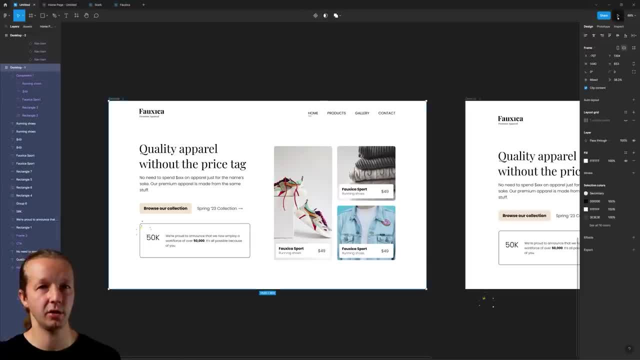 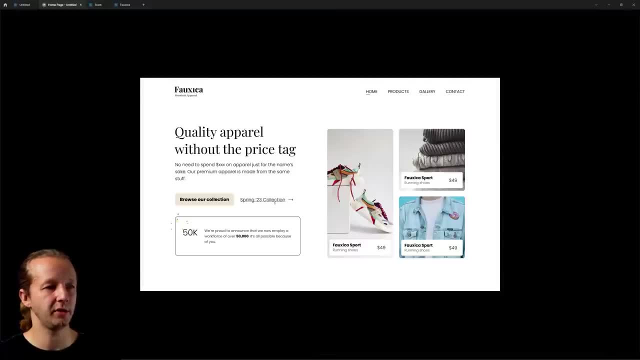 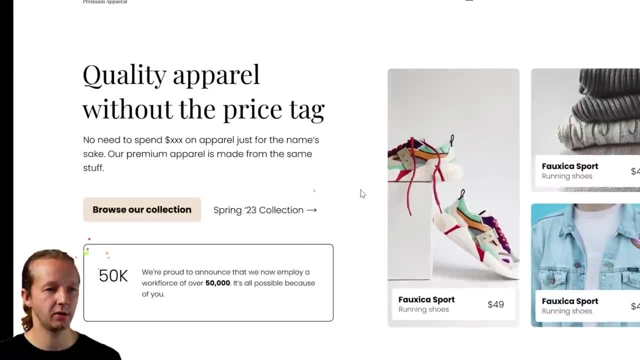 and, by the way, you just click, you select this frame and you click play and I show you. this is what it looks like. we need to do these little hover animations. we need to do this animation right here, where that happens, this little subtle animation, and then this animation as well. 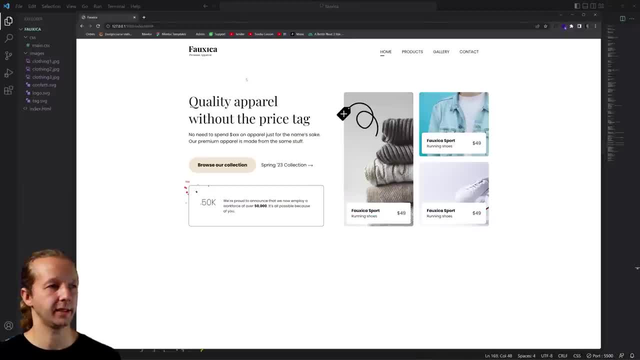 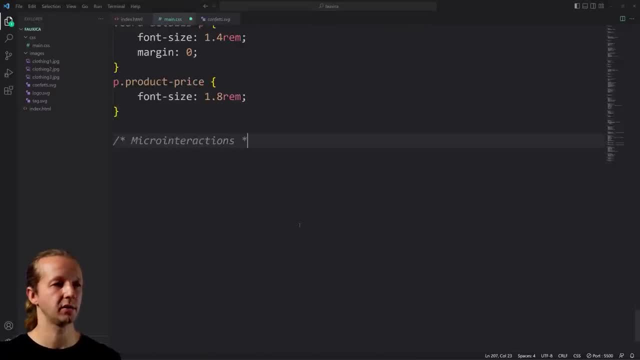 we can all do that in CSS. so let's get started, let's come down here. we'll just do a comment- micro interactions, alright, and the first one that we're going to tackle is going to be the nav hover ones, where the little line grows. so what we say is nav ul lia. 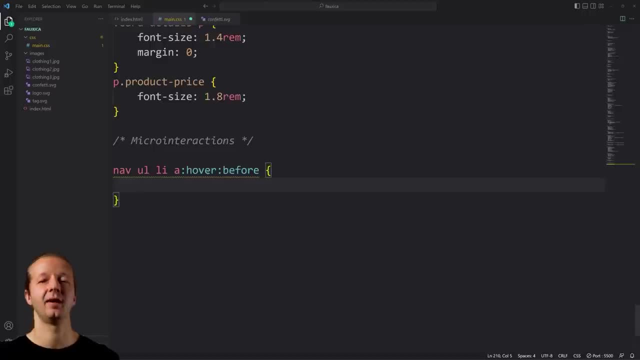 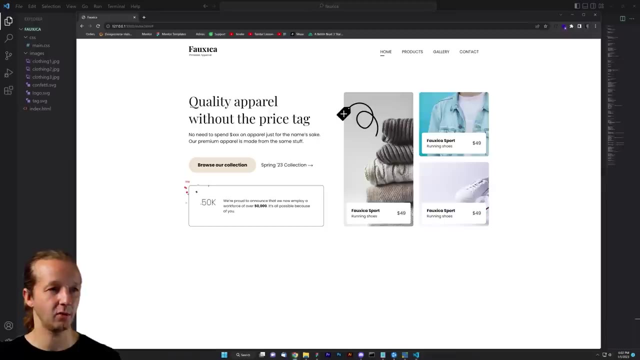 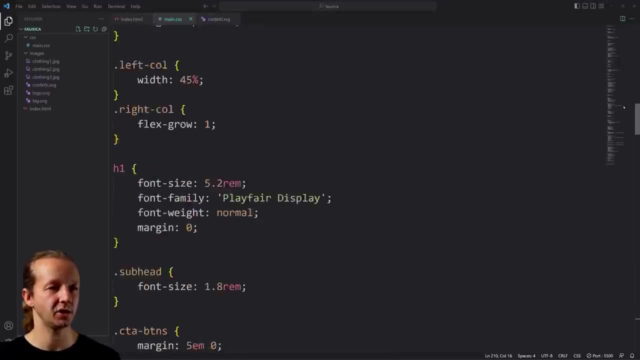 hover before. ok, so we're going to say width 35%. now what's that going to do? I don't think it's going to work. nothing happens right now. if I hover over these, that's because we have to go back up to our nav section. 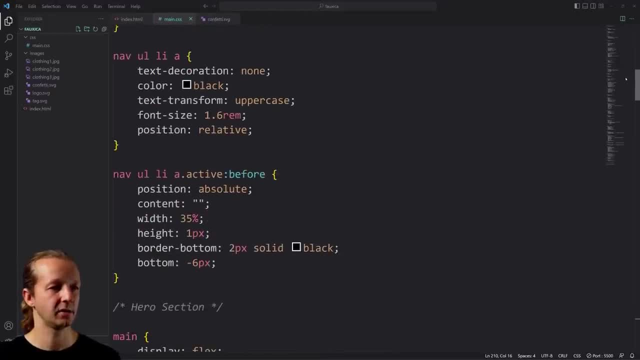 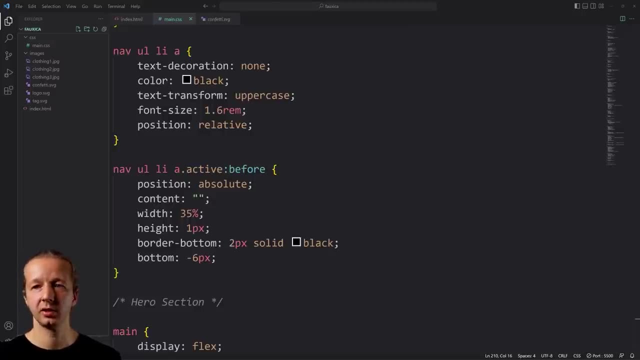 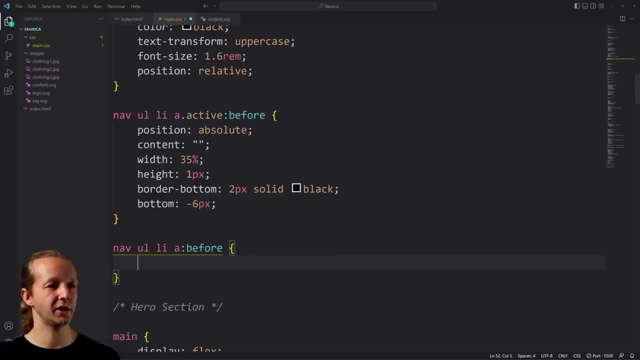 where all that stuff is at, alright, and we have to add a couple things. so essentially, what we want to do is have a transition element that's going to be added to our ul lia before a new rule set. so nav ul lia before now. notice how, before we have our underline, 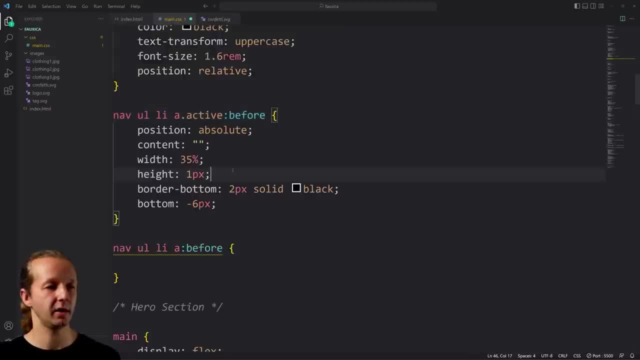 but it's only for the active class, so it only applies to the home link. but these other ones are the ones that we want to hover, are the default ones, not the ones that have the active class. so we basically all this stuff right here. I'm just going to copy and paste it back in. 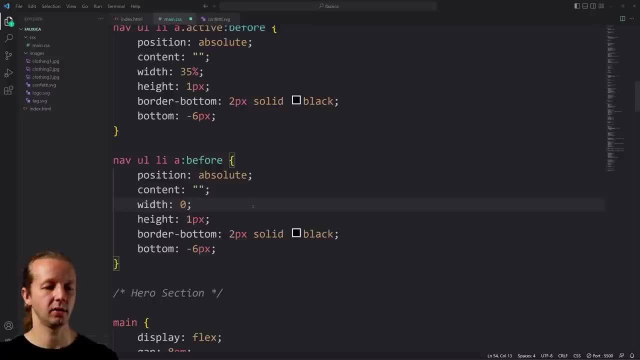 but we're going to set the width here to 0. let's put 0%, because by default we don't want to see it only when we hover. alright, hopefully that makes sense. now we're also going to make this a grey color. we could grab the color code, but I'm being lazy. 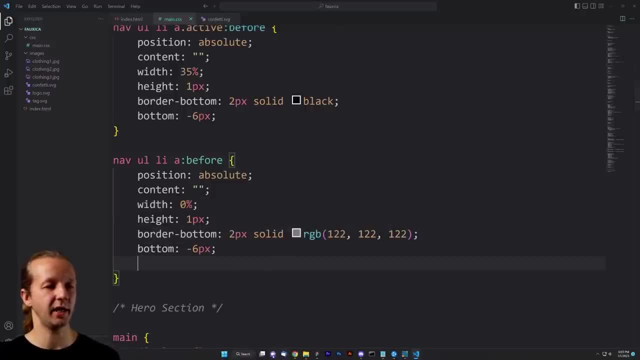 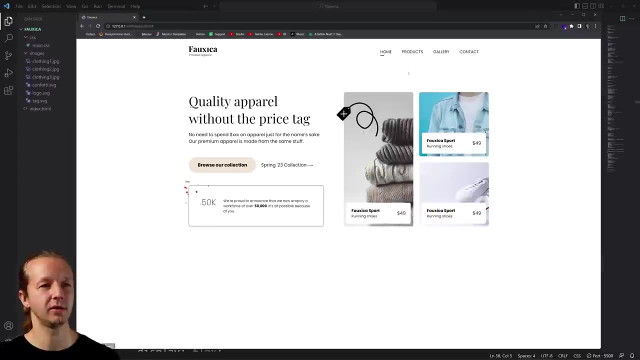 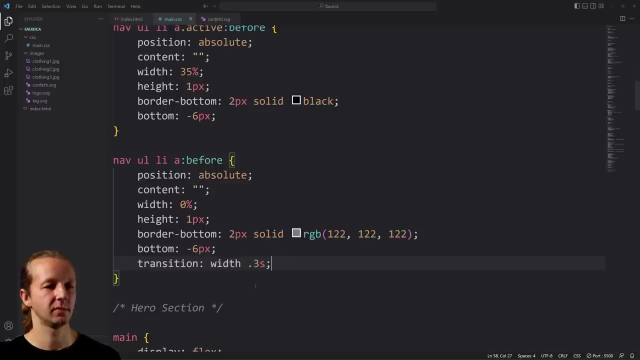 from Figma, and then we say: well, for now we'll hit save. if we hit save and I zoom up, look it just shows up. so how do we make it animate? well, we say: transition width: 0.3 seconds. alright, so it's telling us this is going to transition the width property. 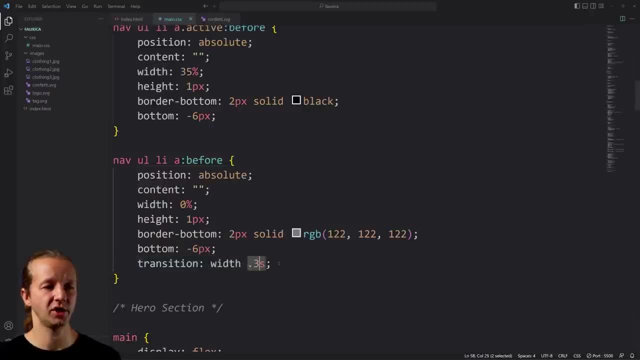 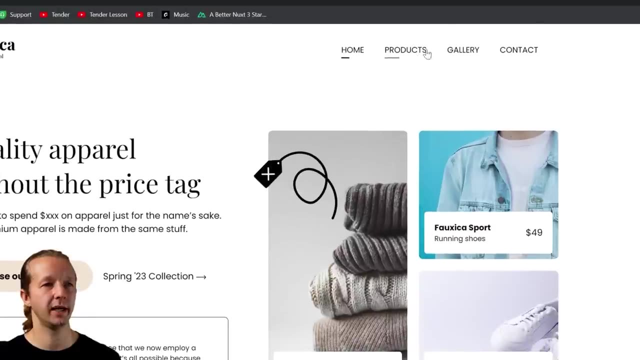 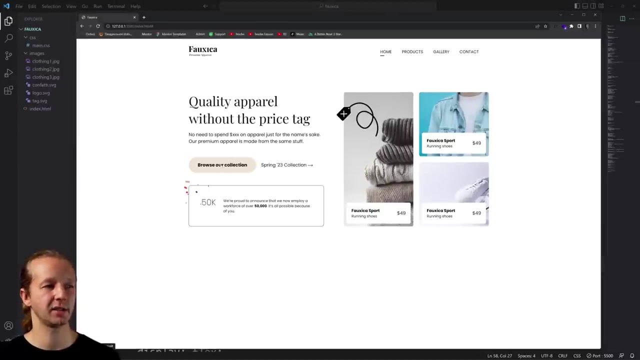 should it change? based on something like a hover and for a duration of 3 seconds, 0.3 seconds, rather 300 milliseconds. so now zoom up. ta da they grow. look how cool that is ok. next one is going to be browser collection. this is a very simple one. 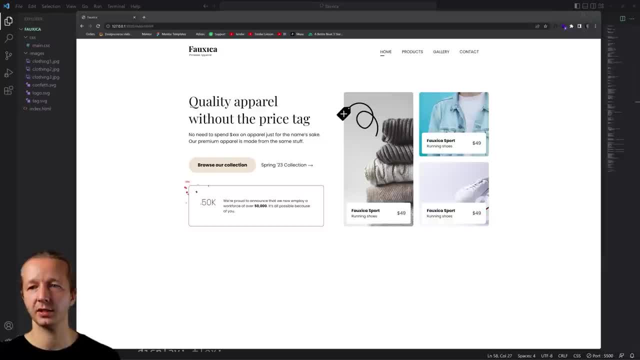 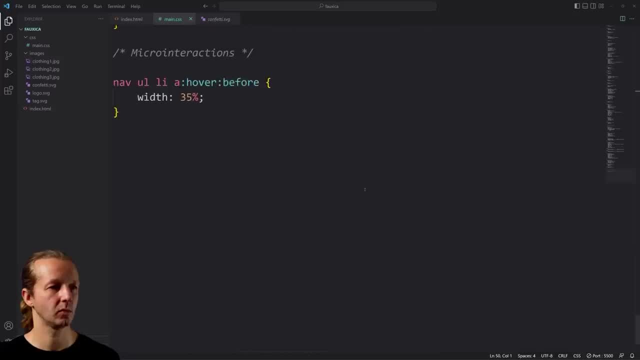 it's just a simple hover on a button, and so to do that, all we do is come down and we say primary CTA hover background, and I happen to know the color code off hand, so I'm just going to put that in. actually it might not be. 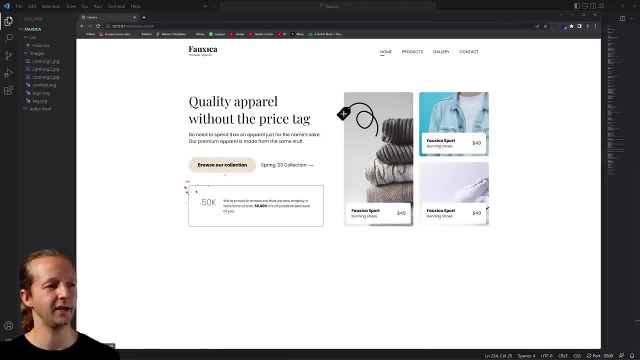 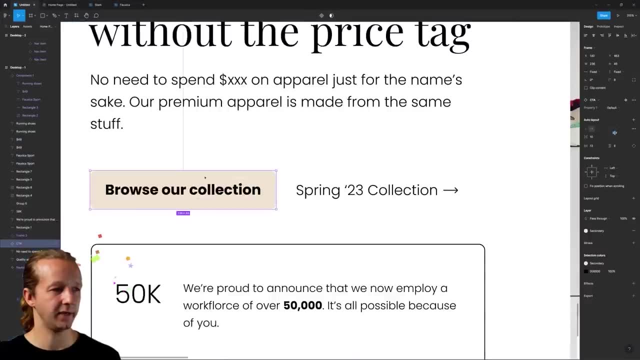 because it was for my previous project, but we'll see what it does- but kind of like a different color that doesn't look good at all. so because I'm a perfectionist, I'm going to go back and if I select this and I detach that, I'm going to make it. 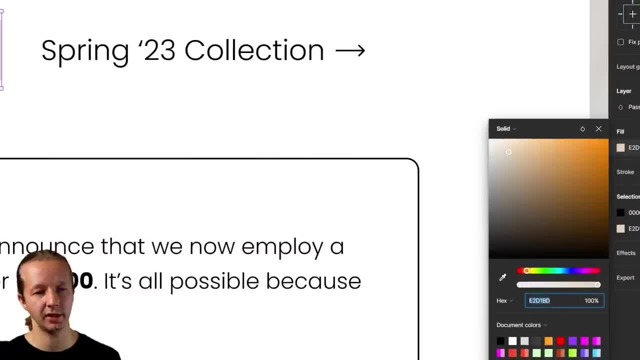 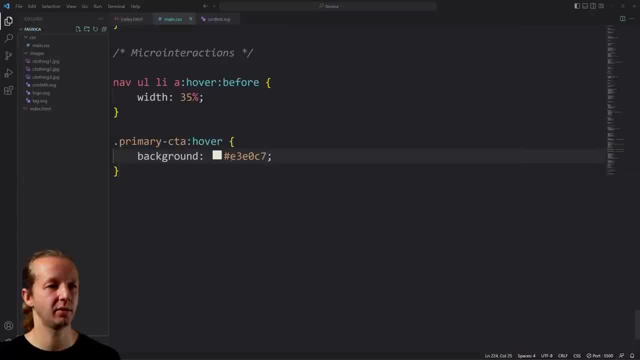 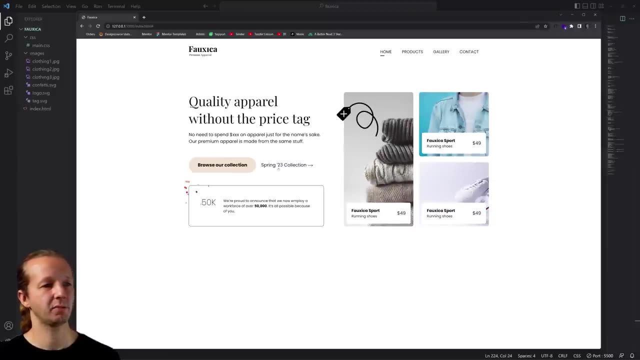 just a little bit darker, like that, and grab that color code so that color code is E2D1BD alright, so I'll back that change up. paste that in. there we go, and it looks much better now. the spring 23 collection: we want that to. 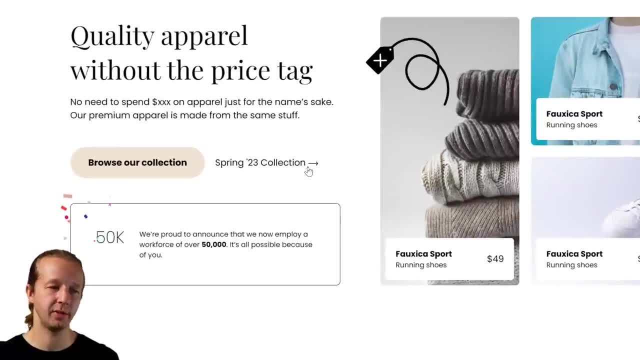 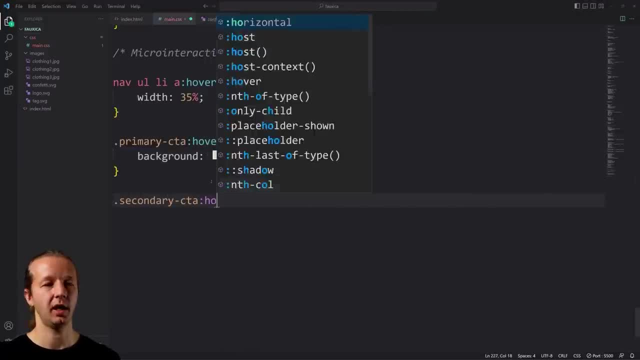 we want this arrow to kind of push over, and that will be a transition as well. so to do that, we're going to say secondary CTA, hover. but we want to focus. once it's hovered, we want to change the SVG element- SVG, alright. and then what we say is transform. 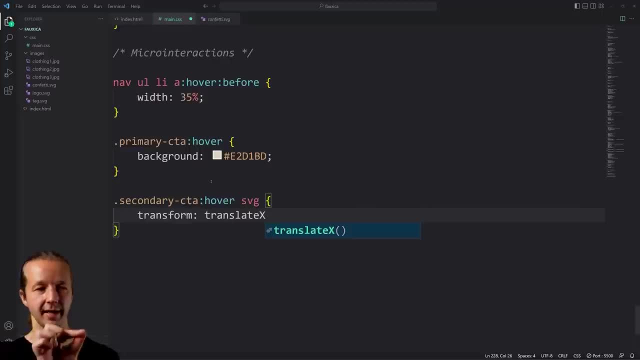 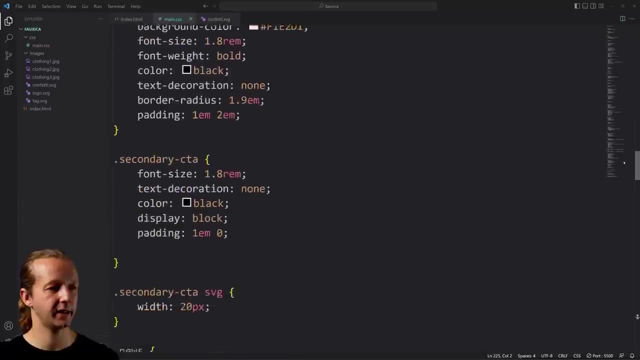 translate X. that means on the horizontal axis. we're going to push it over by 10 pixels. hit save now. zoom up now. that doesn't transition smoothly because we haven't defined a transition property. so if we go all the way back up and we find secondary CTA, 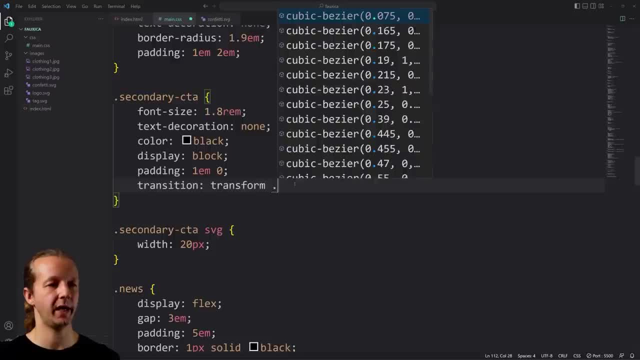 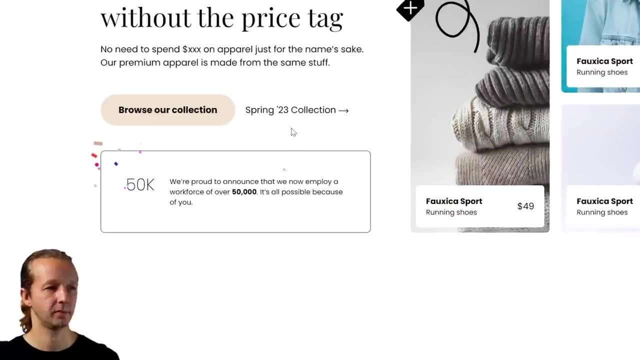 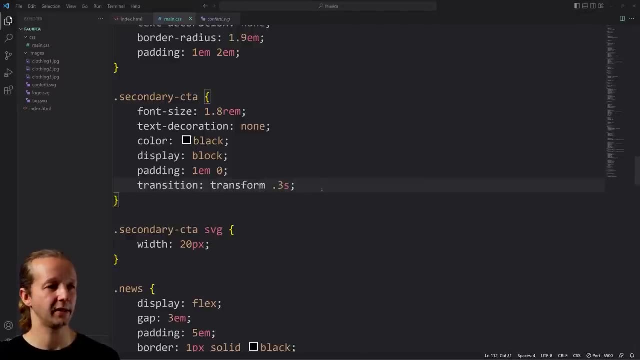 we're going to transition the transform property by .3 seconds, so we zoom up. oh no, there's something I did wrong, which you know what. I'm going to leave this in the video, because that is going to happen from time to time, so I'm going to simply look over here. 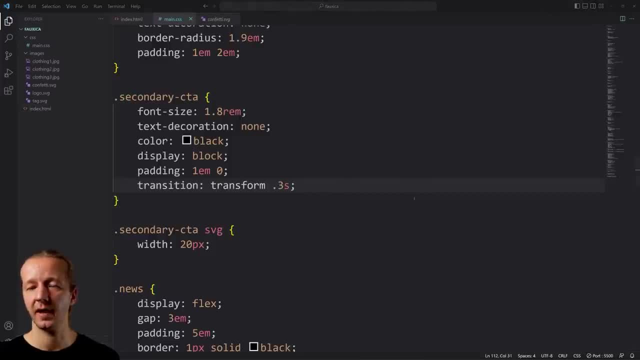 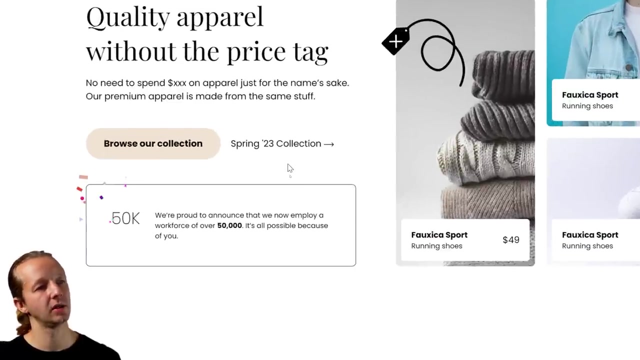 on my. oh. that's why I know why I didn't put it on the right element. it should go right here, because we're applying this on the SVG element, so if we save it and I zoom up, it's going to work. now notice we did have a text decoration. 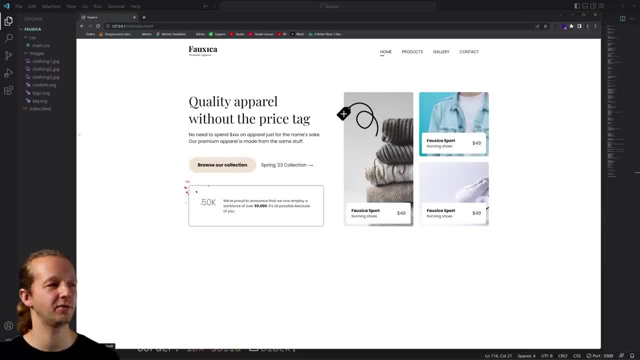 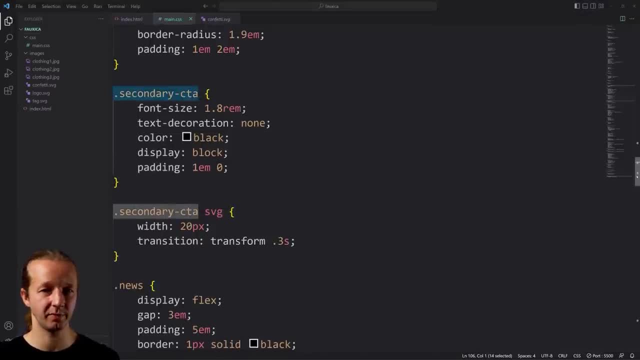 of underline on the hover. I'll let you try that yourself again. you'll put all you have to. actually, I'll show you how to do it because you're new, you're not going to probably figure it out. you might not pause. try to figure out yourself, if you want. 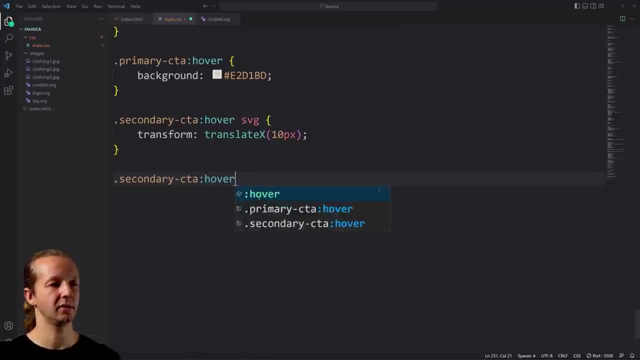 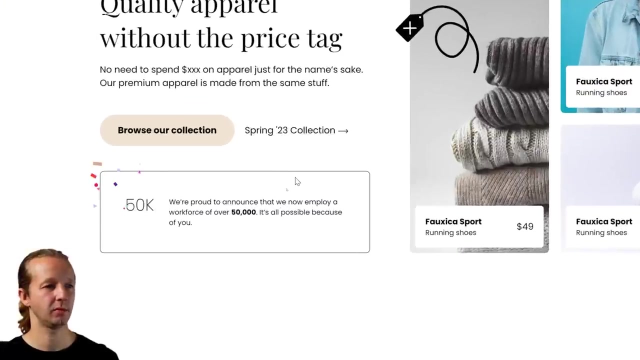 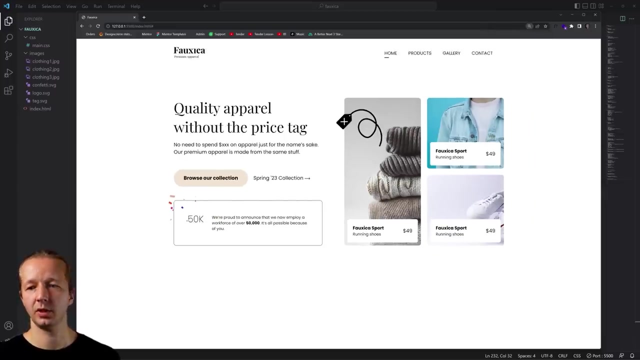 here's how you do it: secondary CTA: hover, background or not background? what am I doing? text decoration, underline, save it. there we go, awesome. and then, finally, we have the hover interaction on our cards that we need to do as well. so this time we're going to use 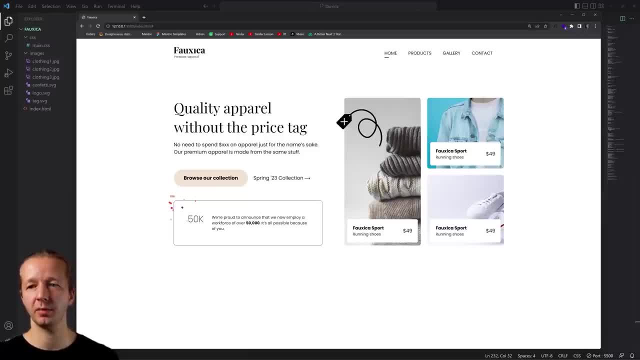 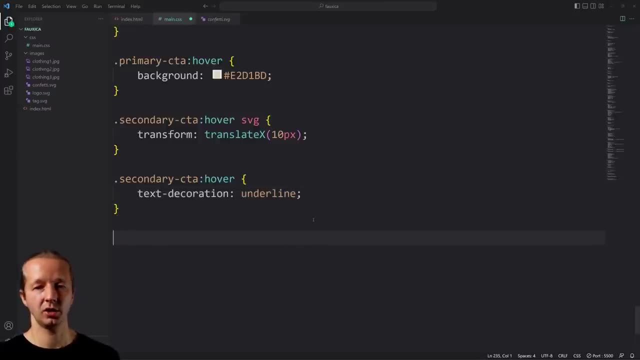 a little bit more robust animation system called the animation property, with keyframes. alright, so here's how we essentially do that. oh, actually we're not going to do keyframes. I'm jumping ahead because there's another thing that we need to do. what we're going to do is: 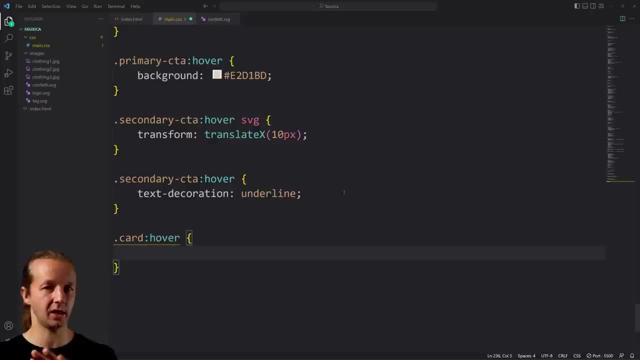 say card hover, so when somebody hovers over, the entire card could be anywhere, like the whole background image. we're going to set the background size to 160%. remember we set it at 150% for those photographs. now, if we come back to card, we need to find card. 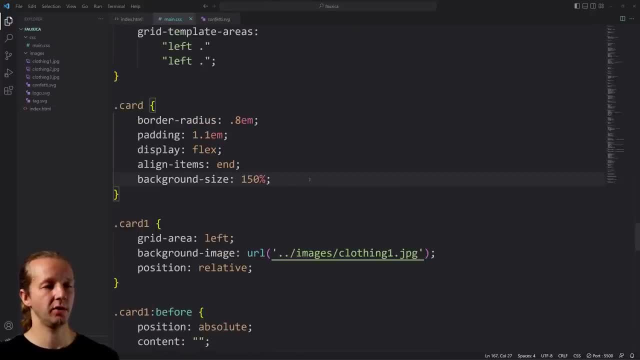 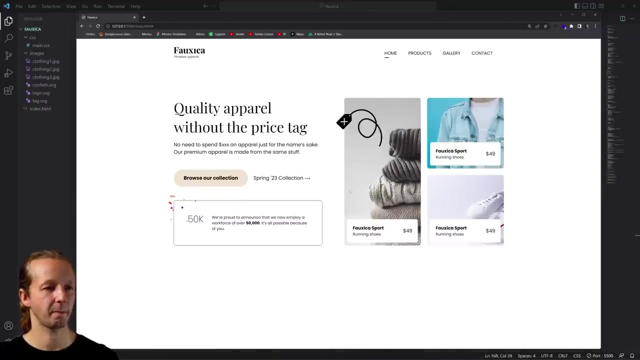 it's right here. right there, we're going to say transition background size. let's do like 800 ms milliseconds. we'll see if this works. alright, I did not spell that right. that's why it wasn't working. now, look at that. very nice. and then we also want this to move up. 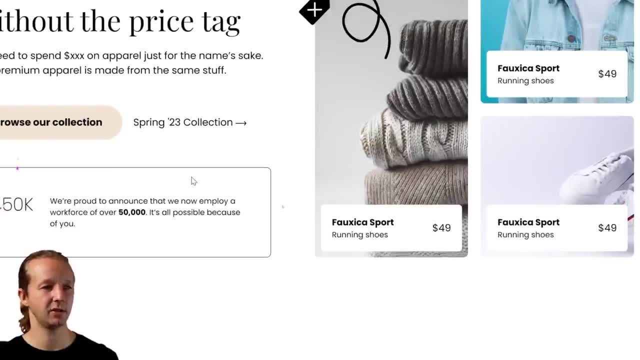 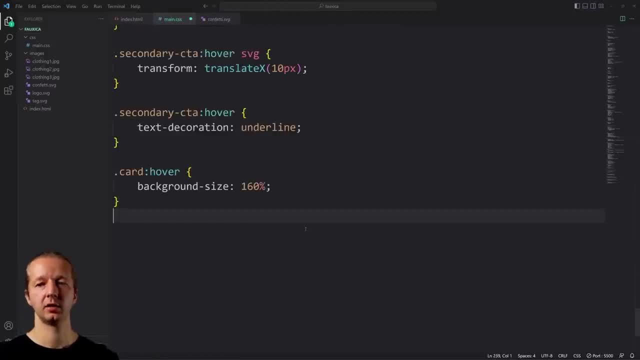 this element needs to move up slightly to be consistent with our prototype. so to do that, to come back down, we're going to say card. when the card is hovered over, we want to change card details, which is the white container that contains the three pieces of type. 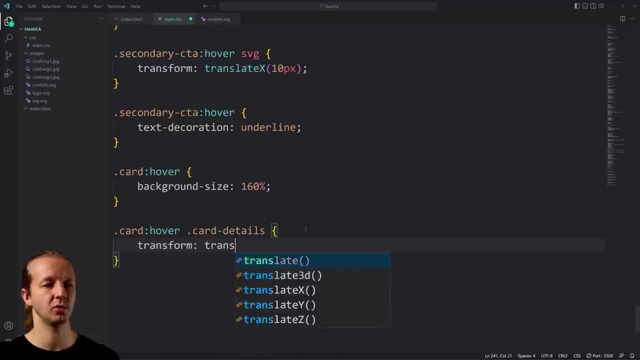 transform. so whenever you want to move something, you can just transform: translate y on the y axis and we're going to move it: a negative 20 pixels which will move it upwards. so if we save it, it's not going to have a smooth transition. to give it that smooth transition, 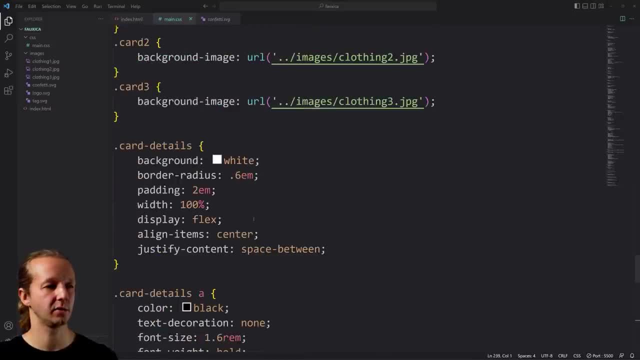 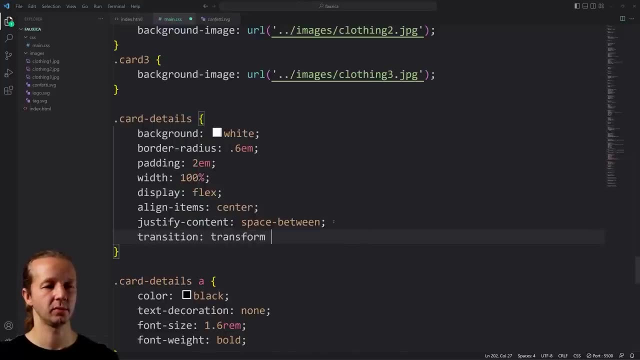 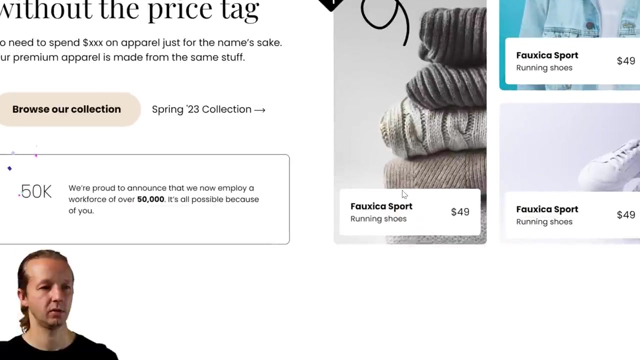 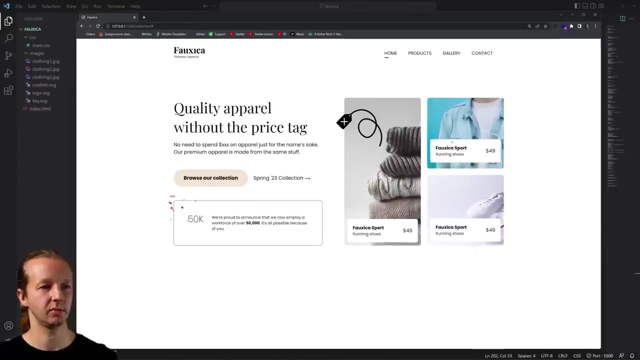 we come back to card details and we're going to say transition, transform, and again, this could be 800 ms as well. so now they all work, as one would expect, awesome. so now one final thing: what if we wanted to have a cool animation when somebody first 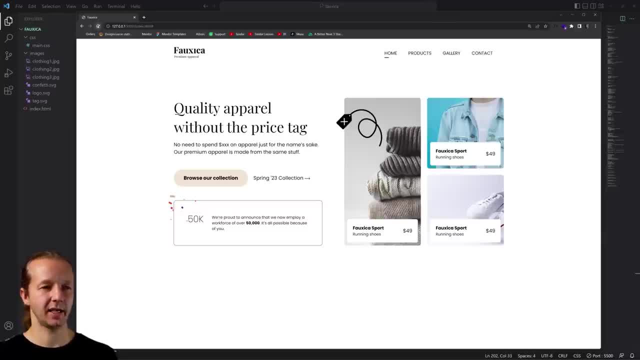 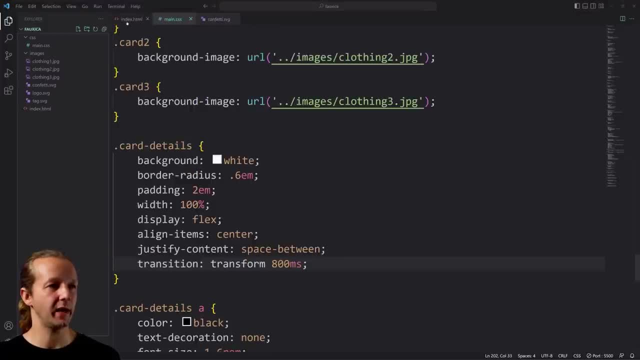 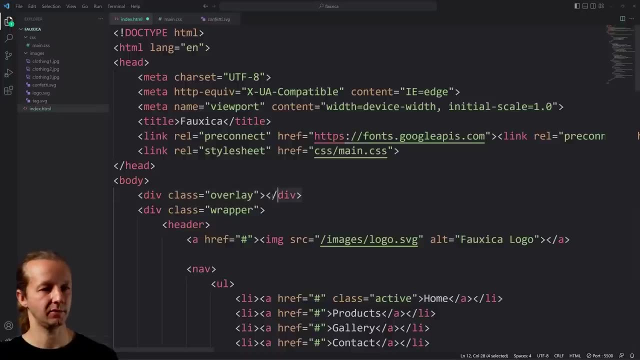 visits the website and things kind of just grow in or animate. sometimes you call them page transition animations. let's do that real quick. coming back to your html, let's add a div class of overlay and there's not going to be anything inside of it, it's just a div element. 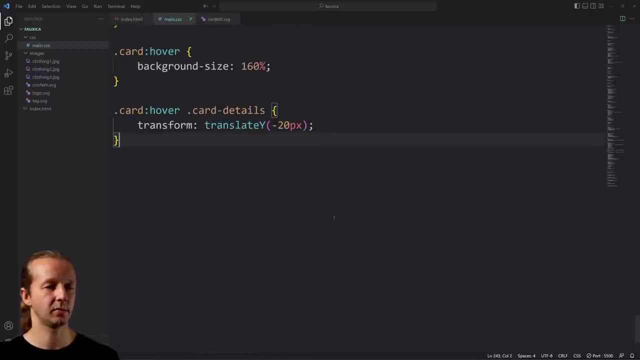 we're going to come back to our main css and we're going to specify that overlay element we just created. and let's add a comment here real quick: intro animation. so for overlay we're going to say position absolute, because this is going to consume, and just kind of 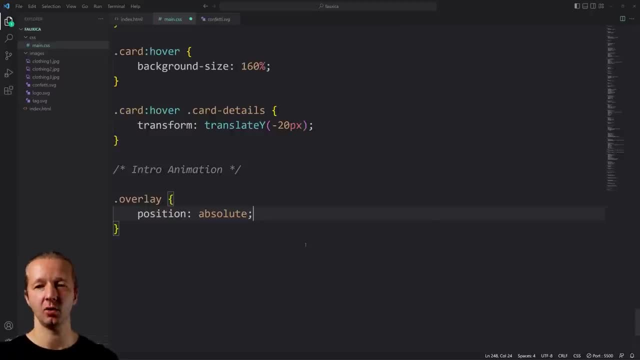 lay over on top of everything initially. so what we'll do is z index 999. it's going to be on the top of no matter what, pretty much anything, unless there's another z index element that we specify. that's larger. background is going to be white. 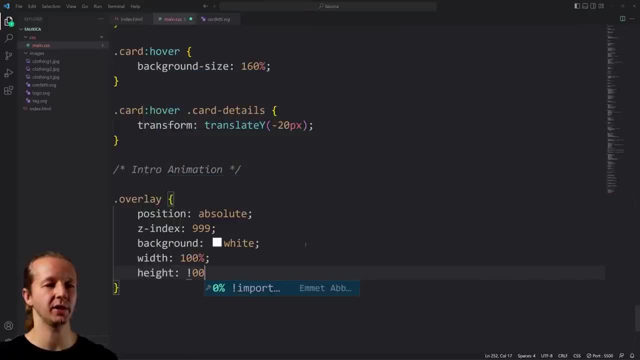 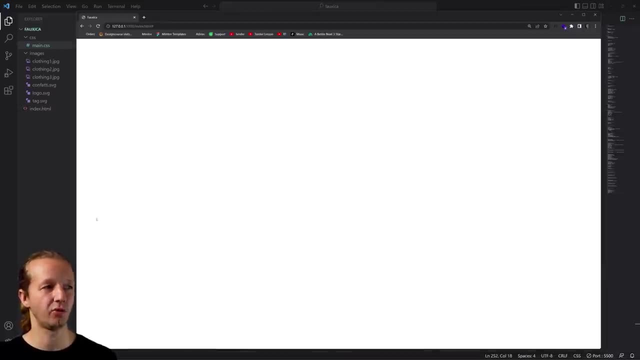 and the width is going to be 100% and the height is going to be 100%. so, if i save this, we're not going to see our design anymore because we have this huge overlay element: 100% width and height. background's white. it's on top of everything. 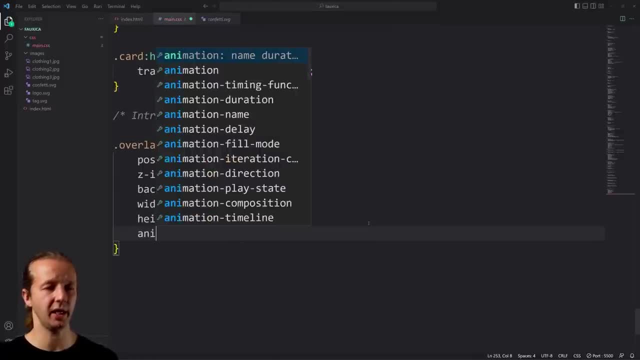 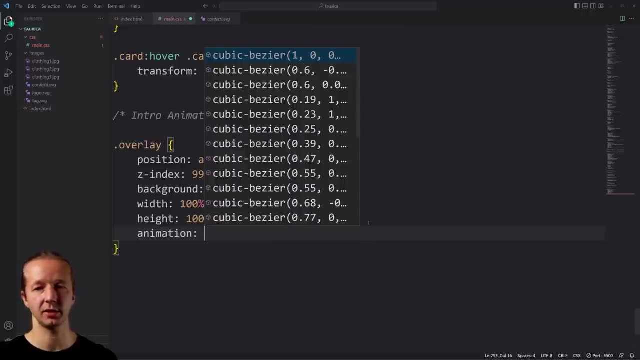 we're going to apply a property we haven't used yet called animation, and the animation property accepts a few different parameters or properties. reveal is one, so reveal is the name, so we can name this whatever we want: the name of your animation. we're later going to define the animation. 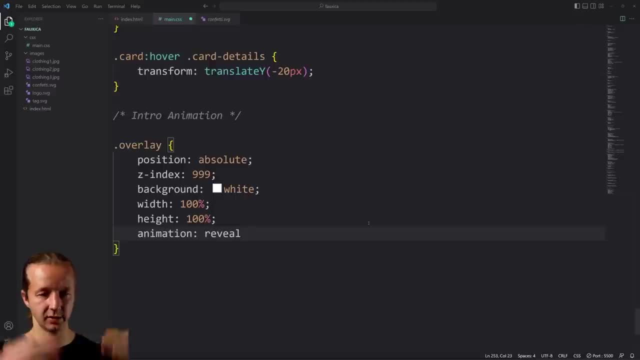 keyframes, so reveal, because we're going to reveal it, essentially the duration of one second or one s the type of easing: ease in is fine. there's entire videos on this property alone, like ease in and out, cubic bezier, all this crazy stuff. it's just timing functions for how the animation 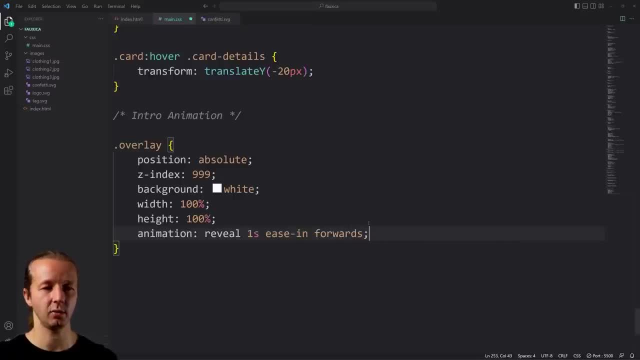 takes place and then we're going to say forwards, because we don't want it to reset itself. it's going to go from this state to the one state, and that's it. then we're going to go ahead and specify the keyframe animations for reveal. so keyframes. 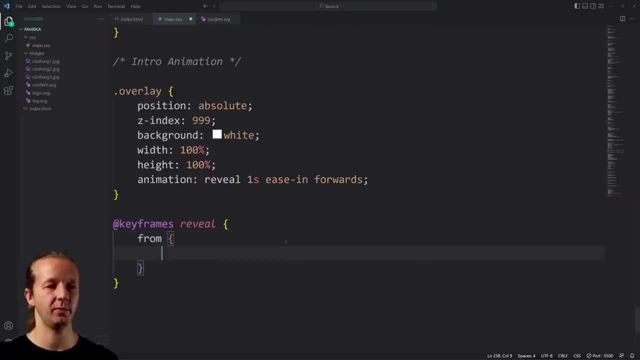 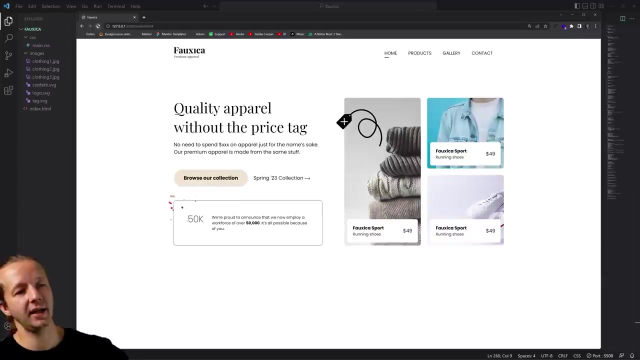 reveal all we say is from transform scale y one. let's copy and paste this change from two: transform scale y zero. now, if i save this, we're not going to see it initially. we have to refresh now. notice how it's like it's animating in. i don't want that. 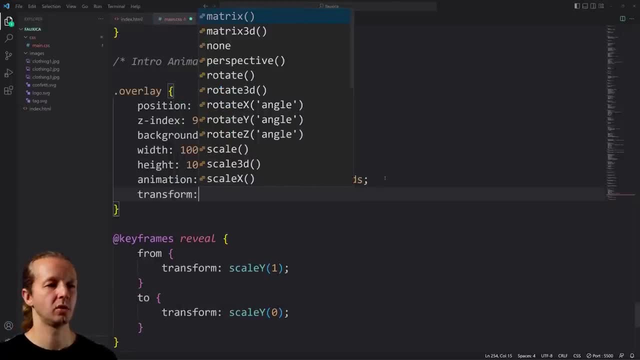 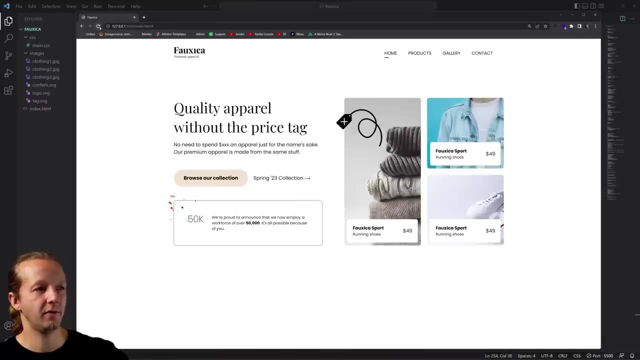 we need to change the transform origin to bottom. so if we do that, refresh, there we go. now let's make another thing where this whole section in the middle, our left and right column, kind of grows in. so to do that we're going to take and remember what consumes. 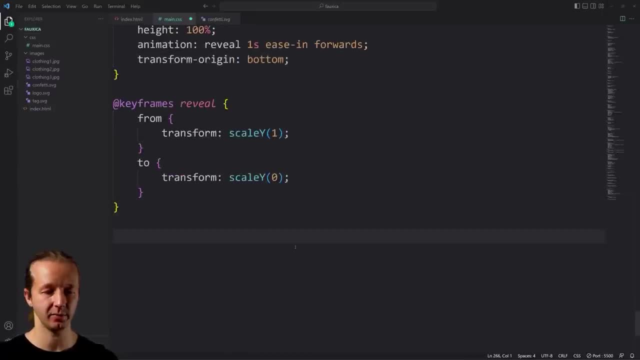 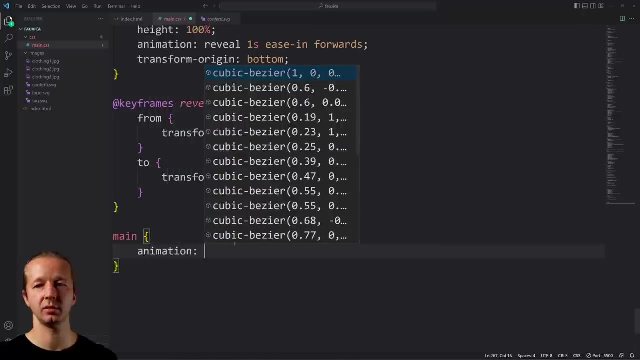 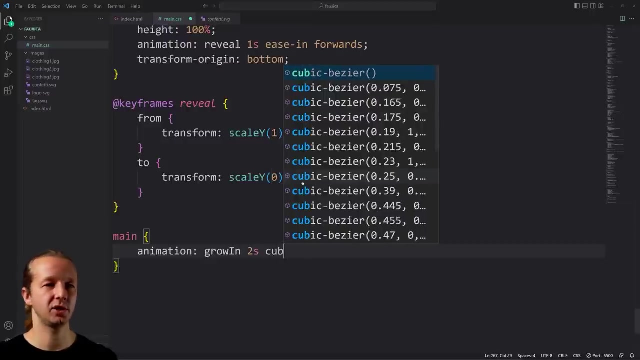 or what wraps around left column, right column, it's main, i'll show you real quick right here. so, main, we're going to say animation, animation, grow in camel case, here two seconds. now we're going to use cubic bezier. i think we're going to use this one right here. 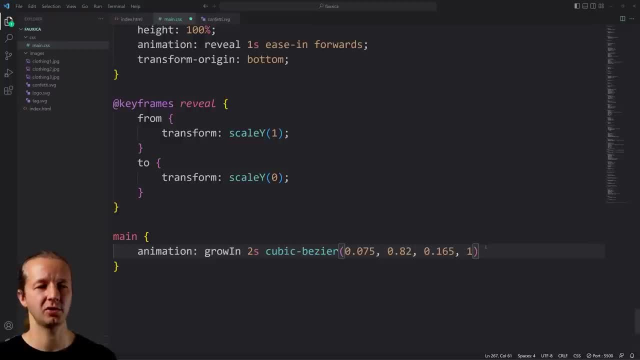 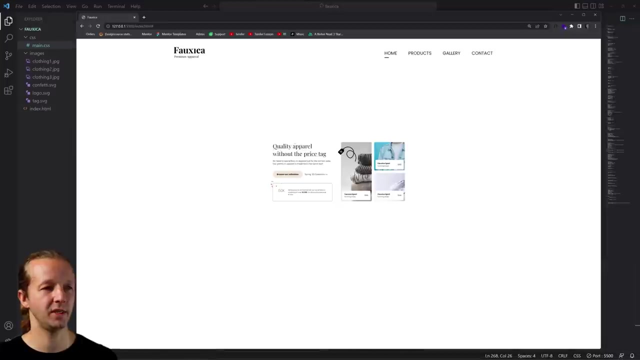 these are just advanced timing functions, and visual studio code has a few of them worked in already. we're going to say forwards, we're going to also change the transform property scale to point four. so if we save this, we scale this thing down quite a bit. so now on animation. 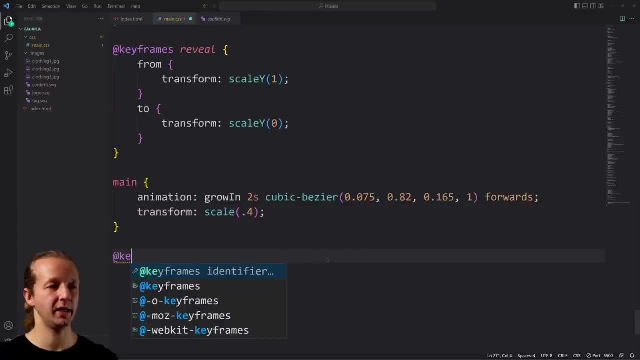 for our grow in at keyframes. grow in, we're going to say to transform. we're not putting from because we didn't specify, because we were specifying by default already in the selector for main transforms. it's already set at point four, so we just put to. 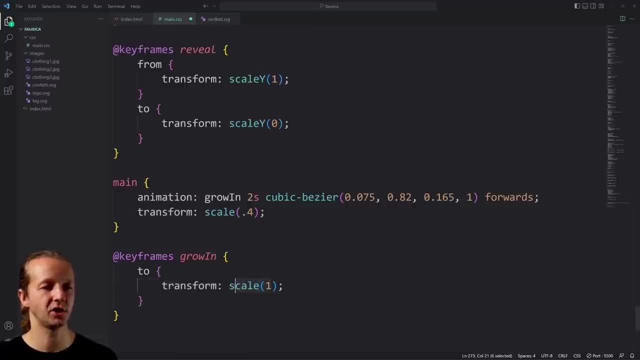 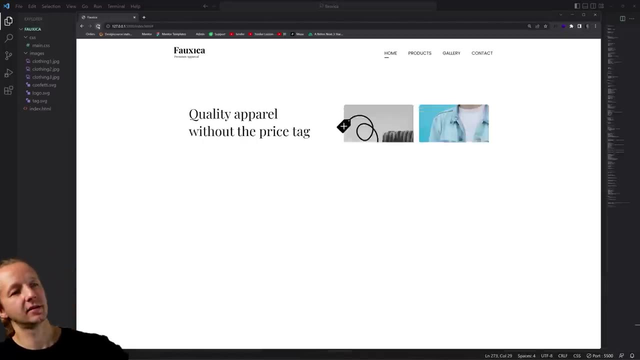 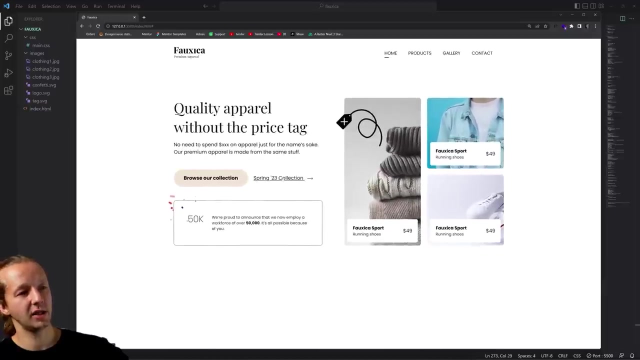 scale one. so we're going back to the original scale essentially. so refresh- look at that, isn't that snazzy. and we have all of our animations worked in here- very fun stuff. so this right here is part of the process. now, I say part of the process, 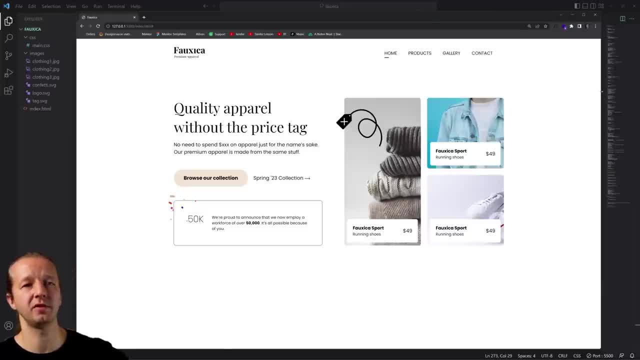 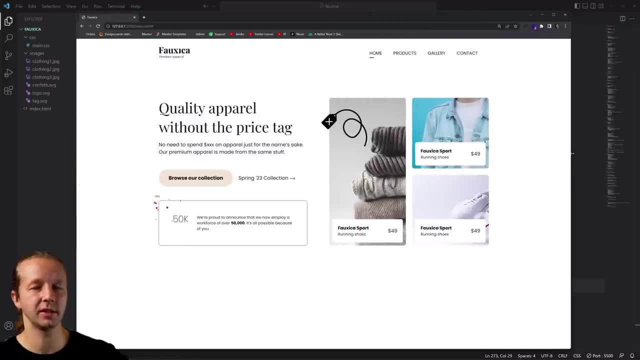 because we did not make this responsive, so if you visited this website on your phone, it's going to look like a mess. typically, you want your designs almost like 99 million times out of. wait a 90. okay, never mind, my brain is fried right now. typically, you want to make sure that your design.